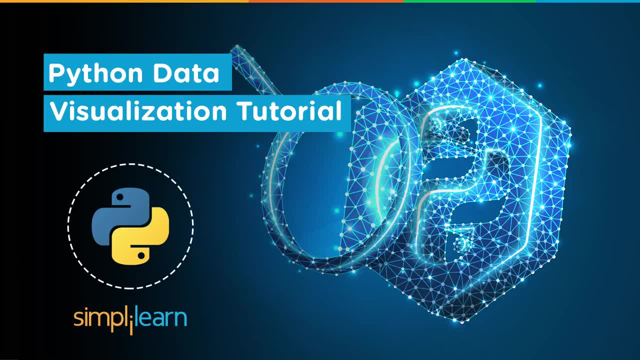 Seaborn. We will explain what is Seaborn to you and then understand Python Seaborn better with the help of a hands-on demo. Feel free to follow along with it. And finally, we will take a look at the Bokeh library offered by Python, which is used to. 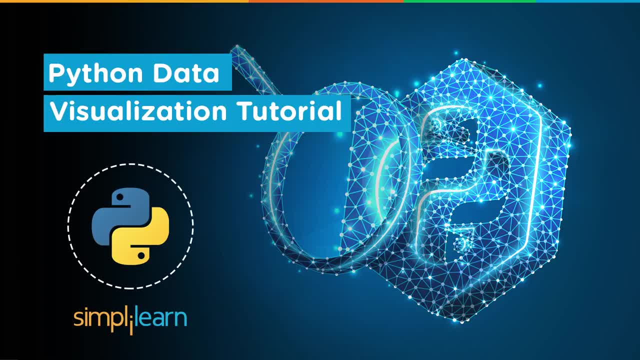 make interactive graphs in Python. We will explain different graphs like scatter charts, line charts, pie charts, histograms, bar plots, etc. in Bokeh and how you can implement them and make them user-friendly and interactive. Okay, so we've made it pretty short in this video, So I hope it seems useful. Have a nice. 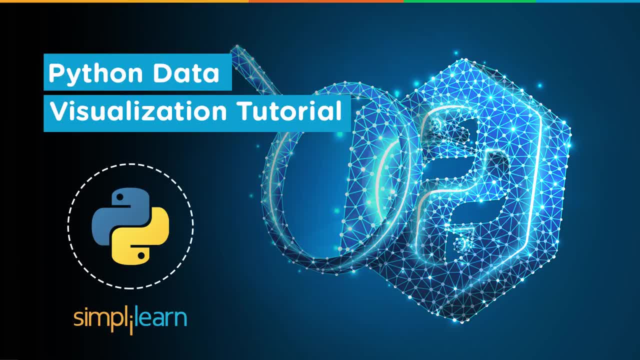 day, Bye-bye, Bye-bye, Bye-bye, Bye-bye, Bye-bye, Bye-bye, Good night, Good night, Bye-bye, Good night, Good night. we will take a look at the layout function in python which is used to make interactive web. 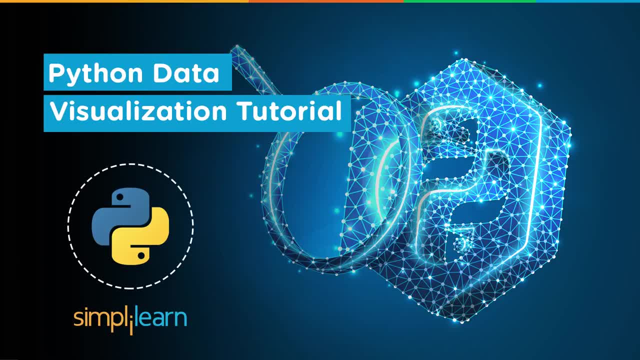 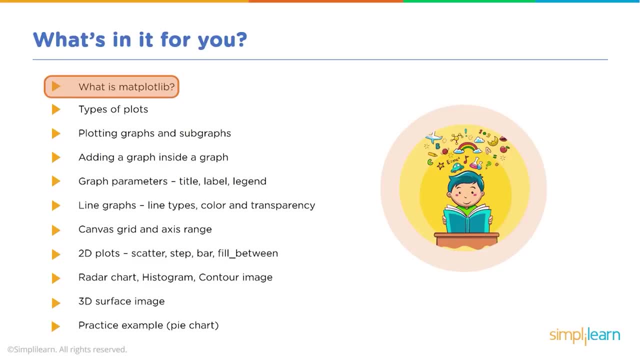 interfaces. so let's get started. today we're going to study the matplot library and the python code, so what's in it for you? what is matplot library? types of plots, plotting graphs and subgraphs. adding a graph inside a graph. graph parameters: title, label, legend, line graphs, line types, color. 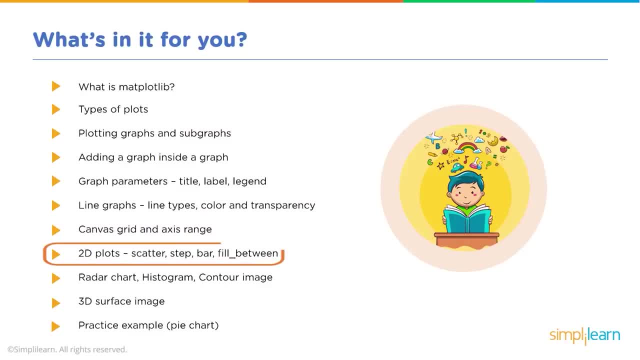 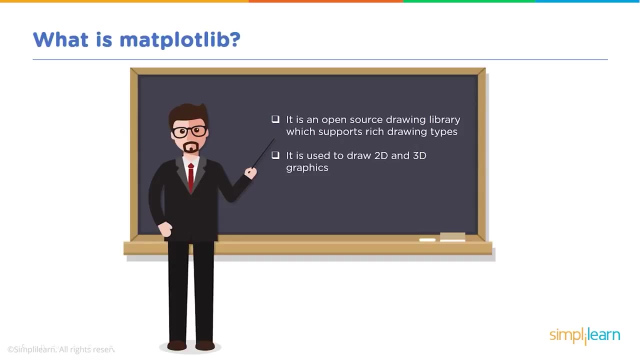 and transparency, canvas, grid and axes range. 2d plots, scatter, step bar, fill between radar chart, histogram, contour image, 3d surface image and then we'll hit a practice example: pie chart. so let's start with: what is matplot library? matplot library is an open source drawing. 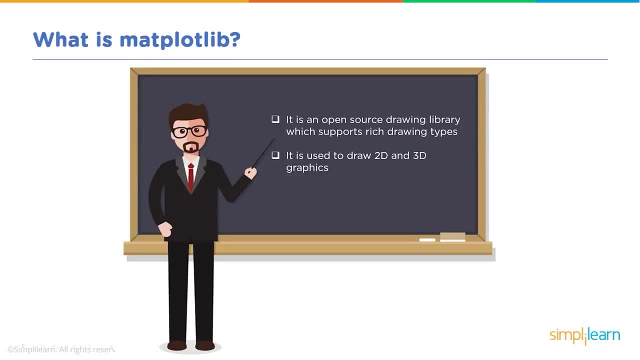 library which supports rich drawing types. it is used to draw 2d and 3d graphics. and there are so many packages in the matplot library. we're going to cover them in just a few minutes. so let's get started with matplot library. we're going to cover the 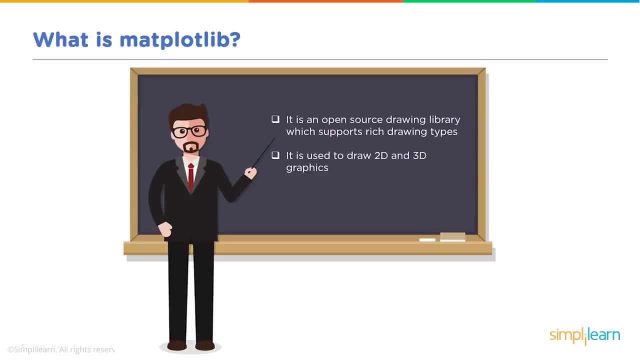 basics, and there are so many packages that sit on top of the matplot library that we can't even cover them all today, but we'll hit the main one. so you have a good understanding of what the matplot library is and what the basics can do. you can understand your data easily by visualizing. 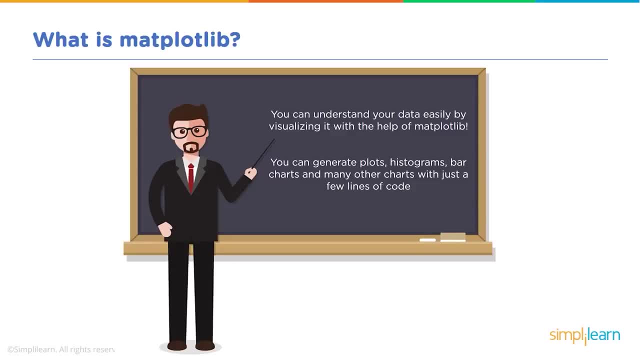 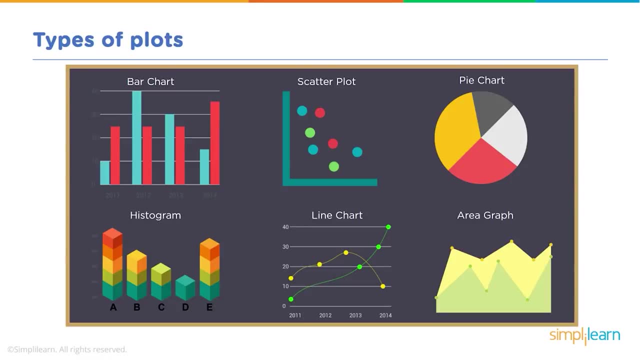 it. with the help of matplot library you can generate plots, histograms, bar charts and many other charts with just a few lines of code, and here we have some basic types of plots you can see here that we'll go into. we have the bar chart, the histogram boy. i use a lot of his. 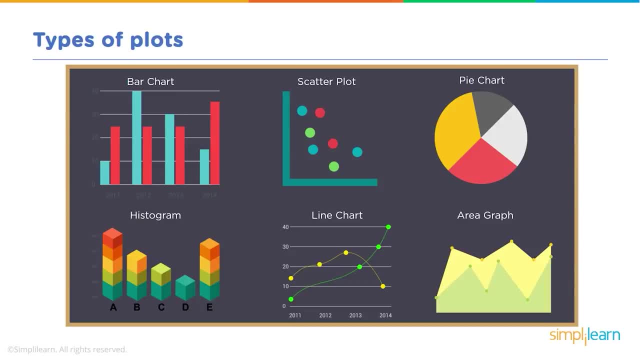 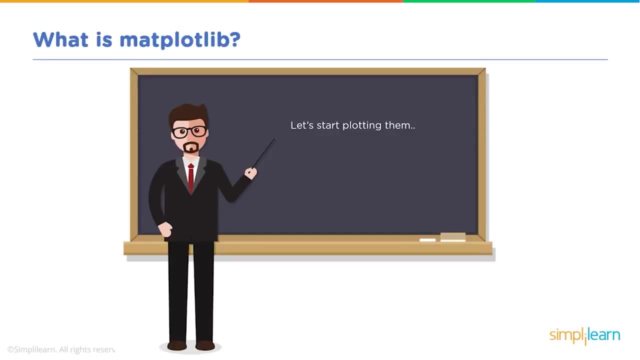 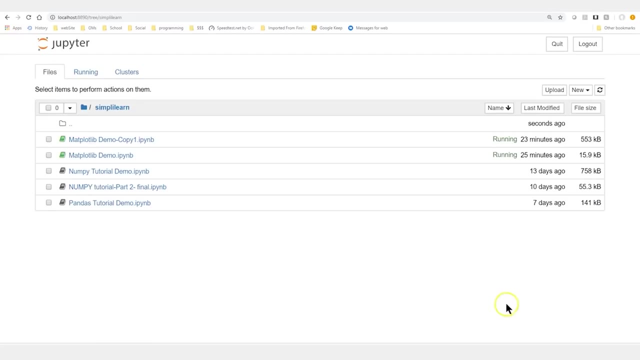 histograms in my stuff- scatterplot, line chart, pie chart and area graph. let's start plotting them and to do this i'm going to be using jupyter notebook. you can use any of your python interfaces for programming or scripting and running it. of course, we here really like the jupyter notebook. 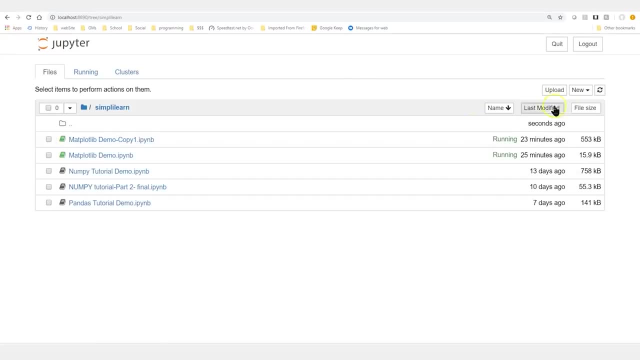 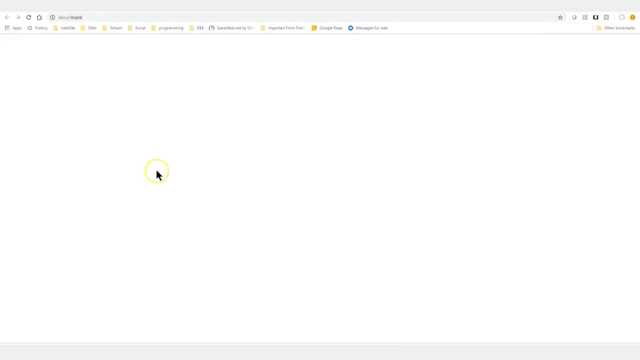 for doing basic, a lot of basic stuff, because it's so visual and in our jupyter notebook, which opens up- in this case i'm using google chrome- you can go up here to new and we'll create a new python 3 and set that up. if you're not familiar with jupyter notebook, we do have a tutorial that covers. 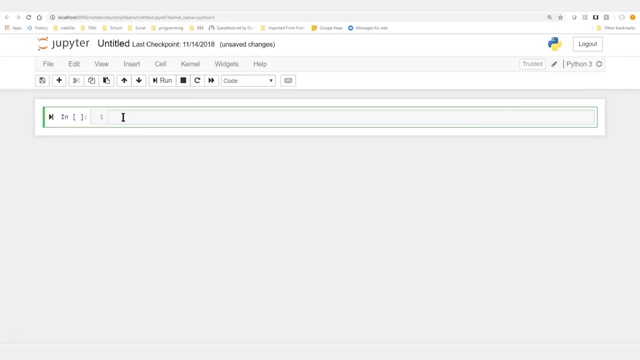 some of the basics of that. you'll look at any of our tutorials. they usually cover a number of them showing how to set up jupyter and anaconda. i myself use jupyter through anaconda, in fact. let's go ahead and open that up and just take a look at this. see what that looks like. you can see your. 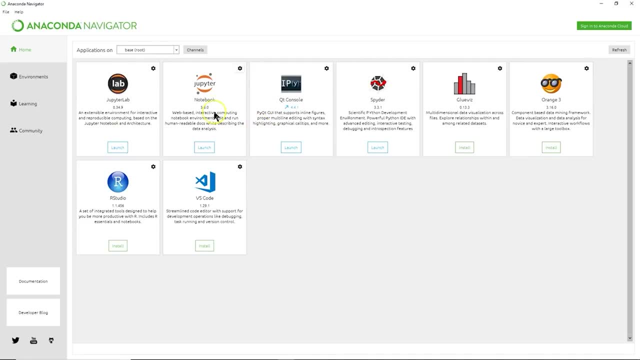 anaconda navigator. if you install it it will automatically install the jupyter notebook. but that also installs a lot of other things. i know some people like the qt console for doing python or spider and other things like that, so i'm going to go ahead and open that up and i'm going to go. 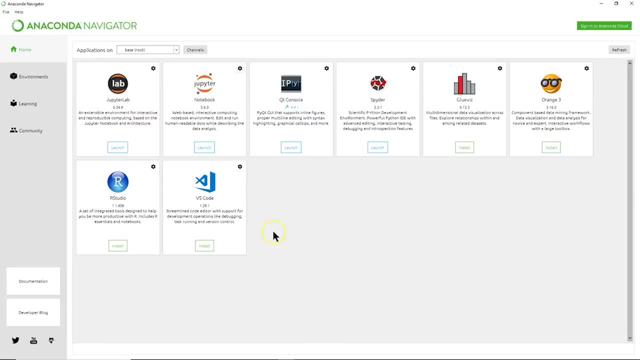 ahead and open that up and i'm going to go ahead and open that up and i'm going to go. i've never used them. i actually use notepad plus plus as one of my editors, and then i use the jupyter notebook a lot because it's so easy to have a visual while i'm programming an even simple 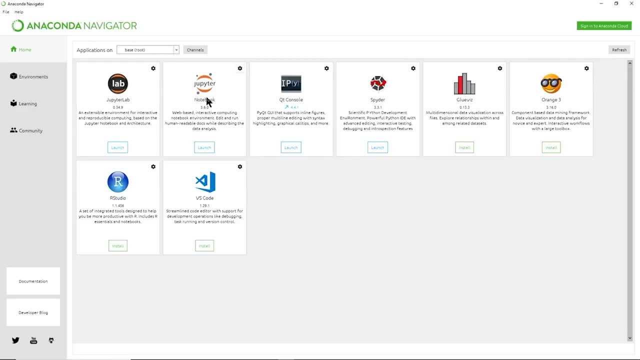 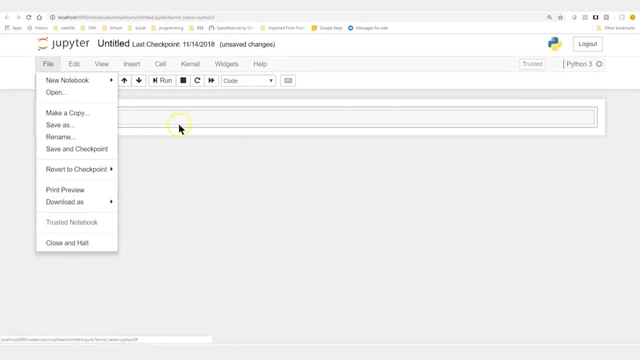 script in python. i'll take it from the jupyter notebook and then do a save, as you can always go under file and you can download as a python program, so that will download it as an actual python versus the ipython that this saves it as. so let's go ahead and dive in and see we got going. 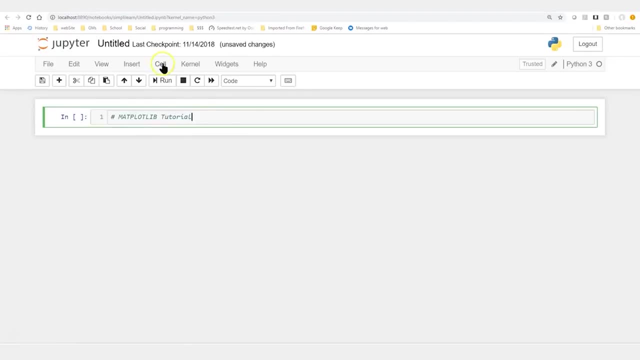 here and let's go ahead and put matplotlib tutorial- and i'm going to turn on the jupyter, this cell, into a markdown so it doesn't actually run it, but you can see it has a nice little title there. that's all jupyter notebook. and then from matplotlib let's import pylab back one, and then 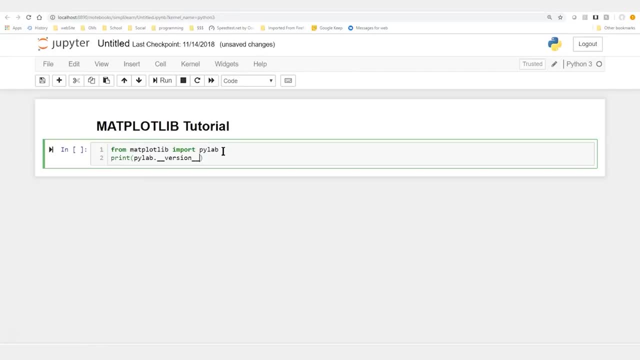 let's go ahead and just print. we'll go pylab in the version. let's go ahead and run this. so we're going to import our pylab module from the matplot library and we find out that we're in version 1.15 .1. always important to note the version you're in. probably i was reading an article that said: 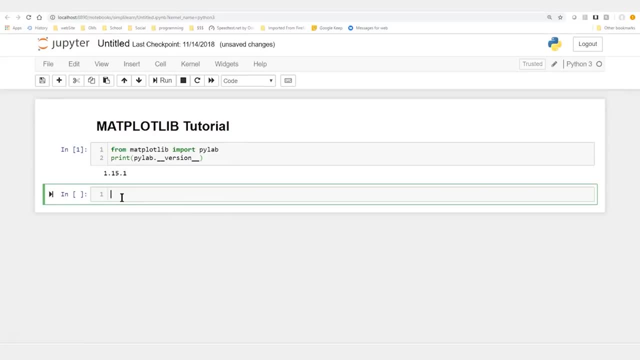 the number one thing that python programmers struggle with is remembering what version they're working in and making sure that they're going from one platform to the other with the same version. and if we're going to graph things, i think we need some data to graph, so we're going to import. 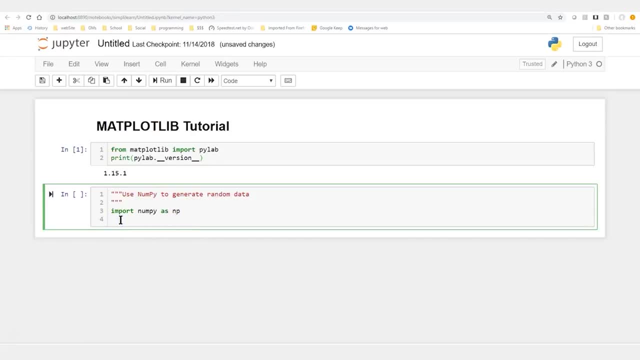 numpy as np. now, if you're not familiar with numpy, definitely go back and check out our numpy tutorial. there's so many different things you can do with it: dealing with reshaping the data and creating. we're just going to use it to create some data for us, and there is a lot of ways to create data. but 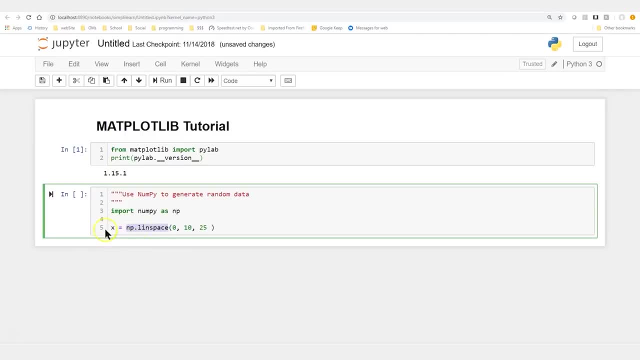 we're going to use the npline space, so we're going to create a numpy array, and the way you read this is: we're going to create numbers between 0 and 10 and we're going to create 25 of these numbers, so we're just going to divide that equally up between 0 and 10.. and if we have x coordinates, we should. 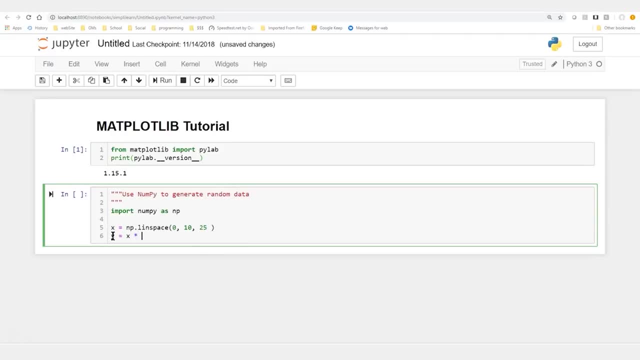 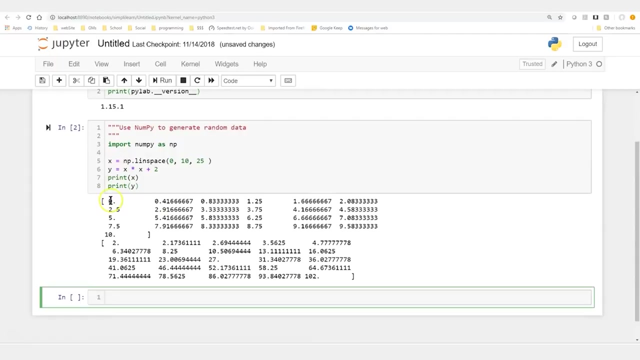 probably have some y coordinates and we'll do something simple like x times x plus 2.. and let's go ahead and print this and print y. let me go ahead and run this and let's see what we got going on here. so we have our x coordinates, which is 0, 0.4, 0.83, etc. and you can look at this as an x- y plot. 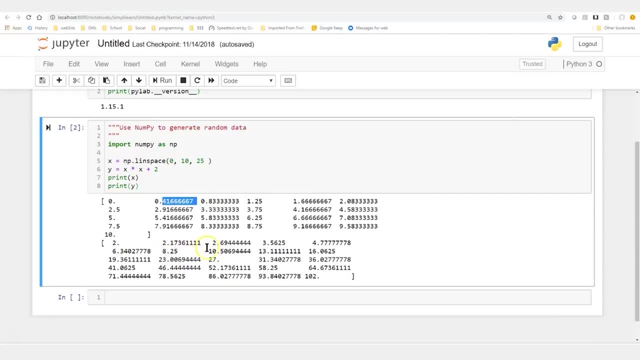 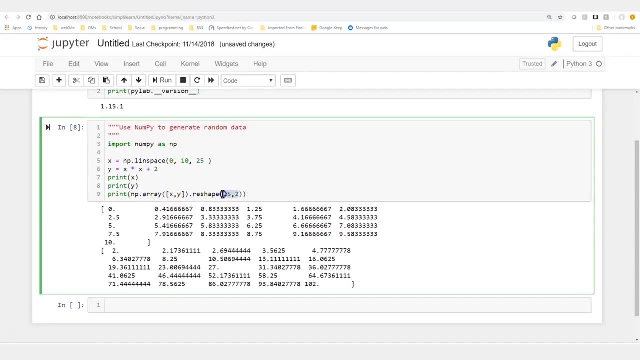 so where we have 0, we have 2, where we have 0.416, we have 2.17. and, just as a quick reminder, we're going to do print np array x, comma y, dot reshape 25, comma 2, and the reason i want to do this is i want to show you something. 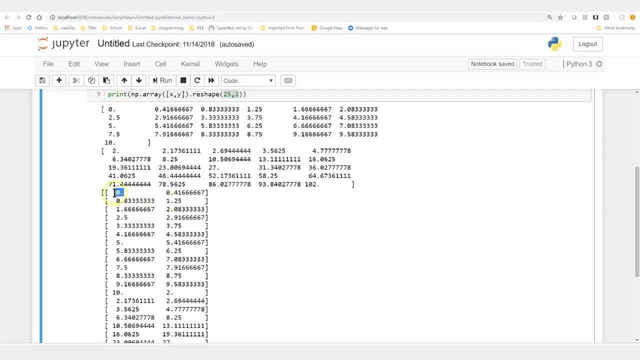 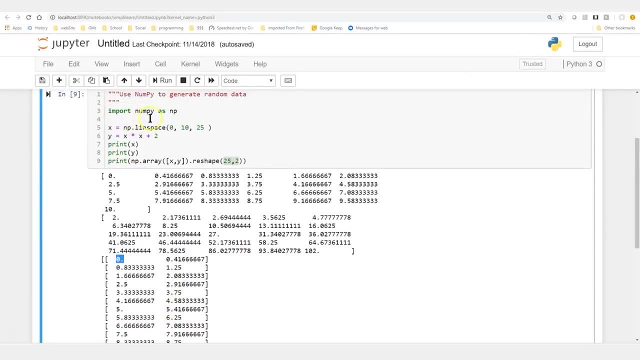 here. a lot of times a program returns x comma y and it's an array of x comma y, x comma y, x comma y, and so when you're working with the pi plot you have to separate it out and reshape it. so if i start off with pairs like this, i can reshape them. if i know there's 25 pairs in there, i can switch. 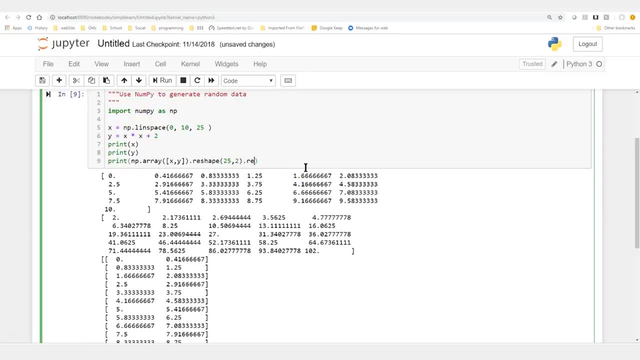 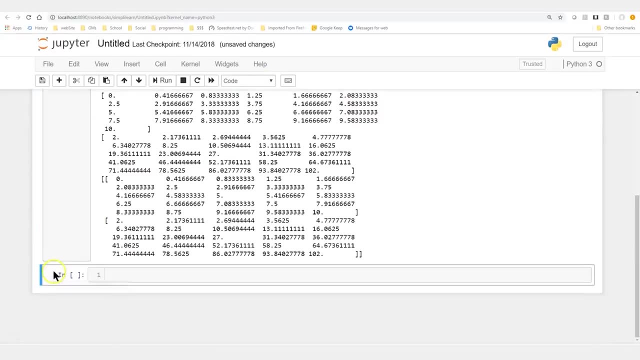 the 2 and the 25 and this is kind of goofy but we'll do it anyways- reshape. so i'm going to reshape my 25 by 2 back to 2 by 25.. And if i run that, you'll see i end up with the same output as the x, y, the two different arrays in here. 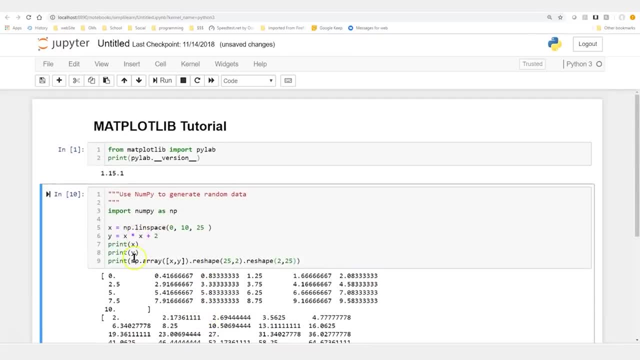 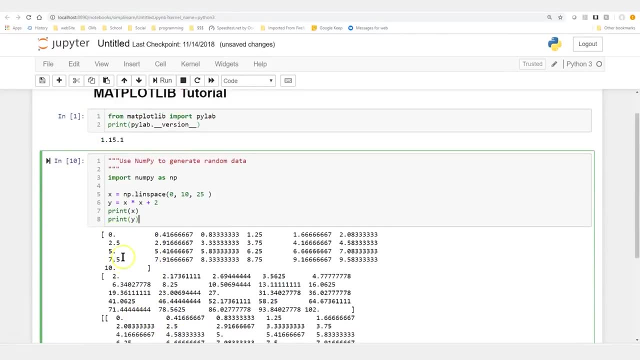 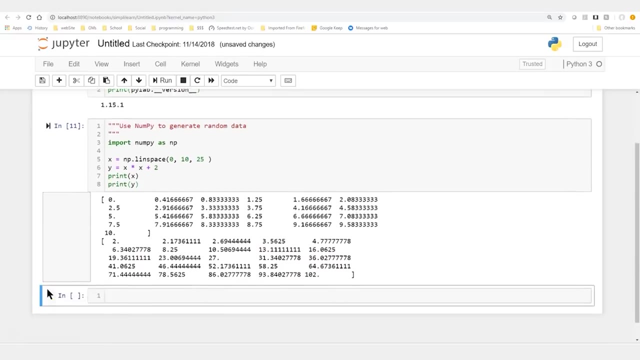 and this is important- that we want x and y separate. again. that's all numpy stuff, but it's important to understand that this is a format that mapplot library works with. It works with an array of x's and they should match your array of y's, so each one has 25 different entities in it. 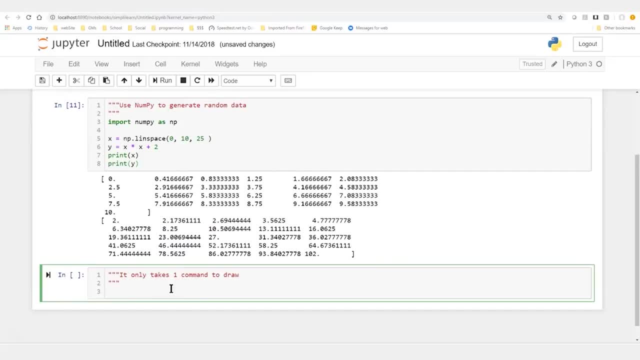 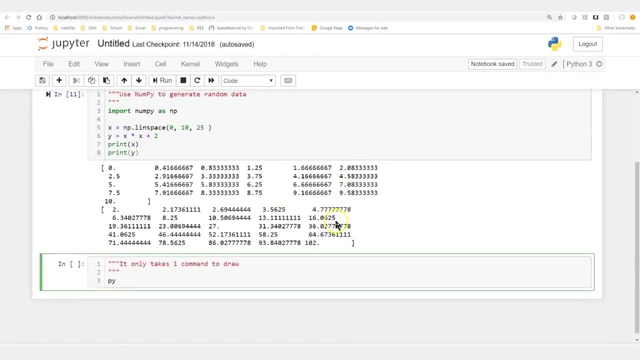 and then for our basic plotting of this data, it only takes to draw graph of this data and so we use our from up here. we imported pi lab. we take our pi lab and the key under there is plot for plotting a line, and then we want our X coordinates and our Y coordinates and we'll throw in R and the. 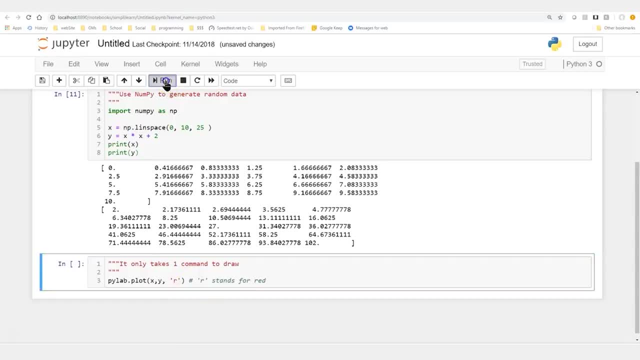 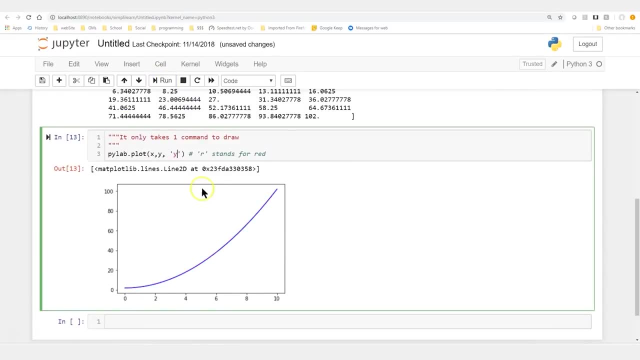 R simply means red, so we're gonna draw the line in red. let me go and run that. you can actually switch this around if you wanted to do different. there's B for blue. we have a lot of fun yellow: hard to see yellow. there we go, but we'll go. 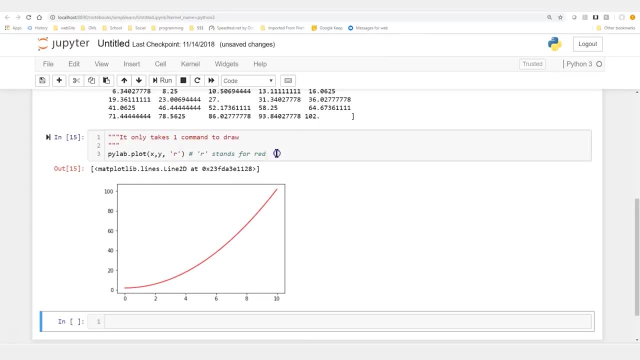 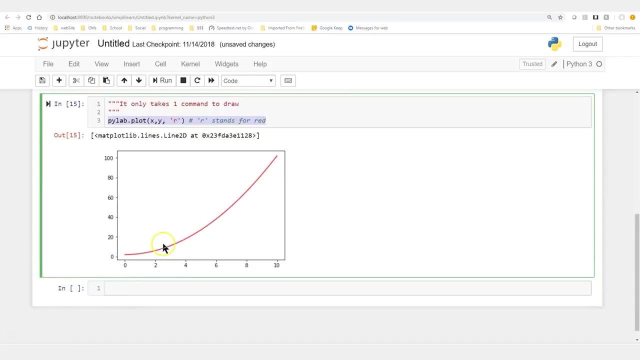 ahead and stick with red run and when you're doing presentations with these, try to be consistent. you know, if the business and the shareholders send you a spreadsheet and they have losses in red, use red for losses in your graph. try to be consistent. use green for profit, for money you don't have to necessarily use. 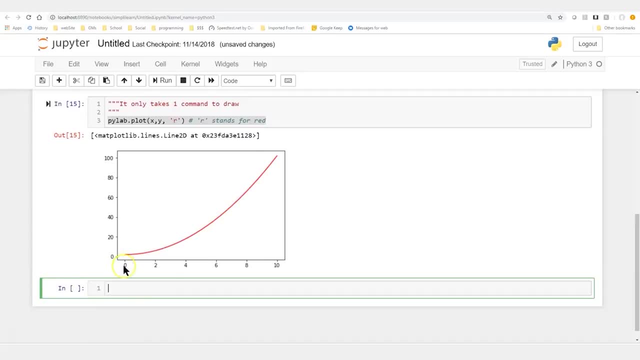 green, but it's whatever they're using, whatever the company is using. try to mirror that. that way people aren't going to be confused. if you switch your data around and every time one graph has red for loss and one graph has blue for loss, that gets really confusing. so make sure you're consistent. 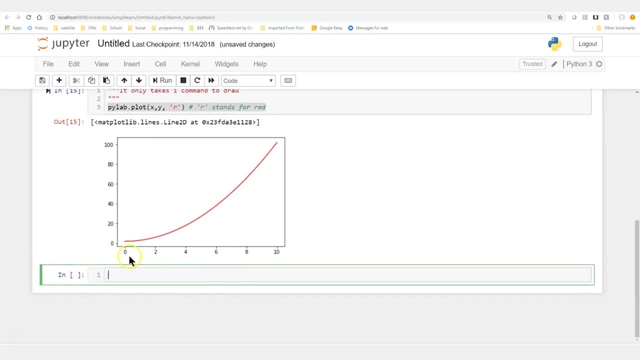 in your graphs and your coloring and something to know, because we're gonna cover this in a minute. this is your canvas size. so we have a canvas here and what we're gonna do next is we're gonna look at sub graphs. okay, so let's take our pi lab and create a sub plot, and one of the things also to know when we're 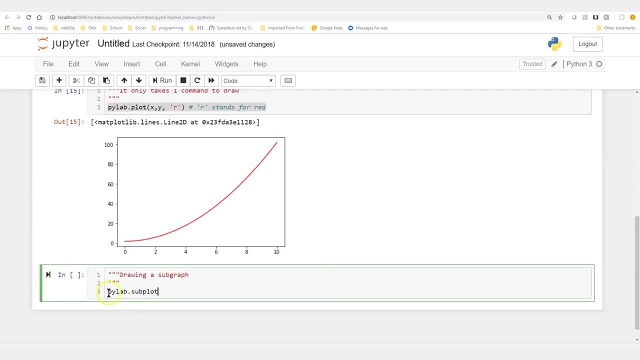 working with the map plotter, map plot library. I'm not setting when I do this. this is my drawing canvas, the pi lab. so once I've imported the pi lab, I'm drawing my images on there- very important to know. and with the subplot we're gonna give it some different. 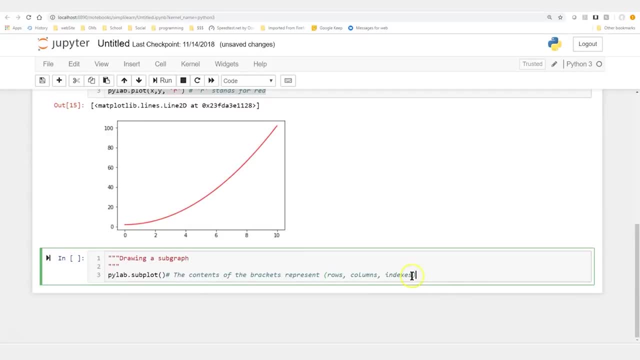 values and we're gonna represent by rows, columns and indexes and let's do one to one, so it's gonna be the first row, second column and the index is like you can stack your graphs and things like that. we don't worry too much about that, indexes, but rows and columns. we want to go ahead and use row one and column two. 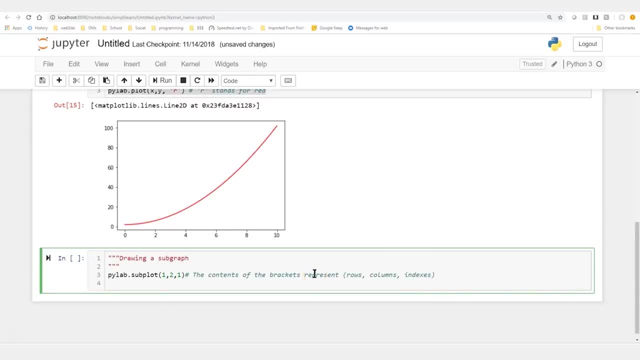 and if we're gonna have one object, we should probably have two. but before we do that we have to plot data onto the subplot. so the order is very important and we're going to stick with their X comma Y, and let's do this. we're gonna. 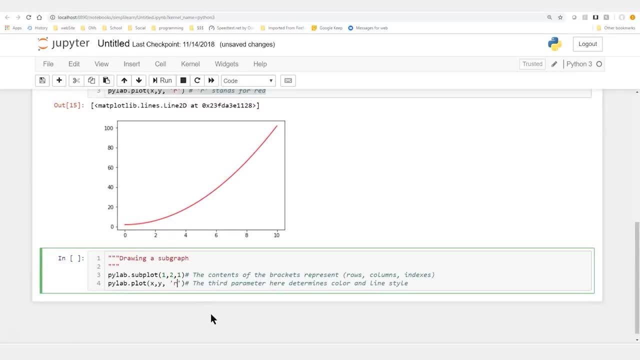 add in a third parameter here. remember we did red- we're gonna add shorthand dash, dash for dash lines. so this plots the data into row one, column two, and if we're gonna do that, let's do up another one pi lab dot subplot. and if we're gonna do row one, let's do column two and index two, and this time we're. 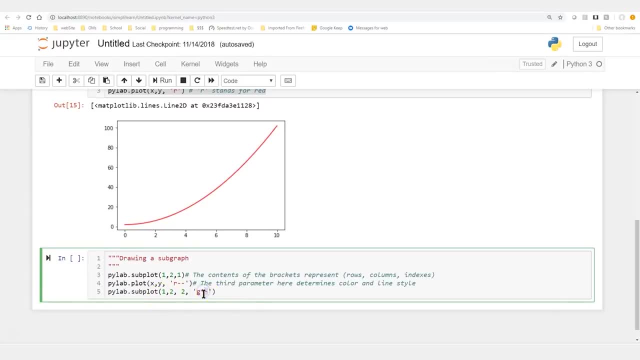 gonna add G for green and this denotes a style. and if we're gonna set up our pi lab subplot, there we go. we gotta go ahead and plot that pi lab plot and instead of X, Y, we want Y comma X. whoops, I messed up. this is in the wrong spot. there we go. we'll move that down here real quick. 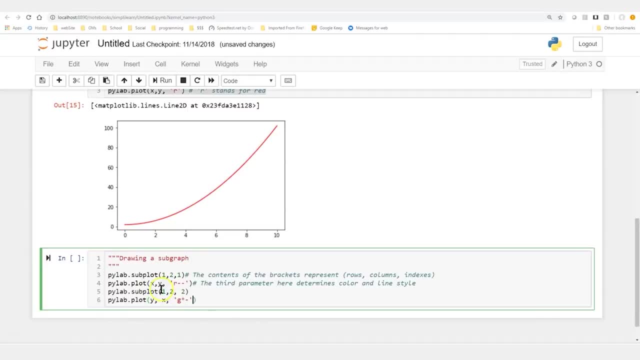 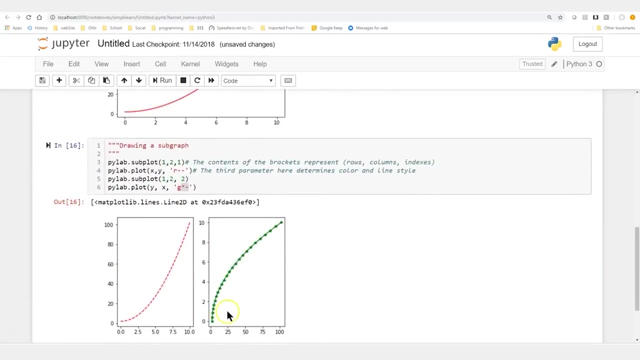 because that goes in the plot part. so the subplot tells it the row, column and index and the pi plot tells it what data. in this case we switch them- and the color and then the style shorthand. now let's go ahead and run that and you'll see, it takes this canvas, splits it in two and now we have two different graphs. 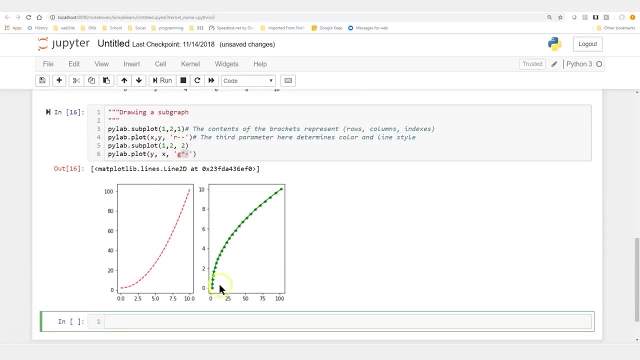 and we have the red one with dashed lines and we have the green one, which is has a little stars going up, and if we take this and let's just um, just for fun, let's change this and run that with an index of one, it puts them both on the same index. it also 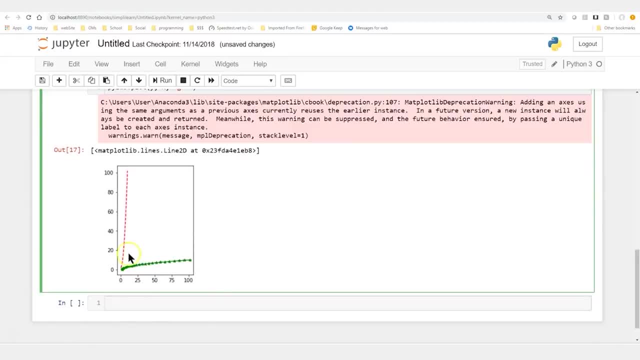 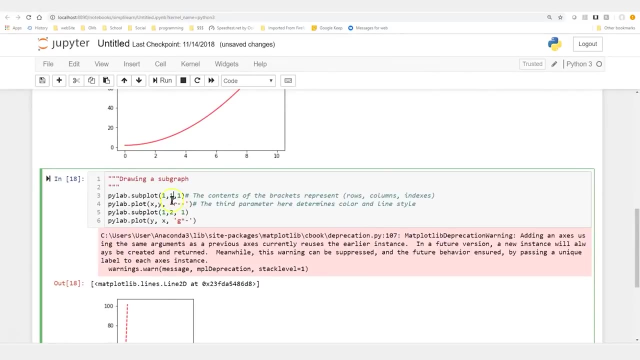 gives me a warning, because it's a strange way of doing two subplots. there's this, depreciated, there's another way to do it, but most people just ignore that warning because it's not gonna go away anytime soon. now that's using the same setup. what happens if we do? instead of this, let's change the column on here. 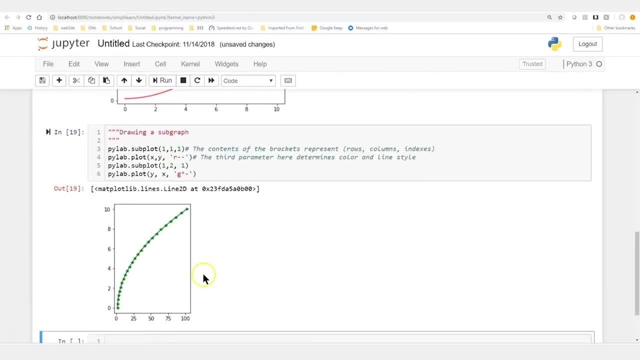 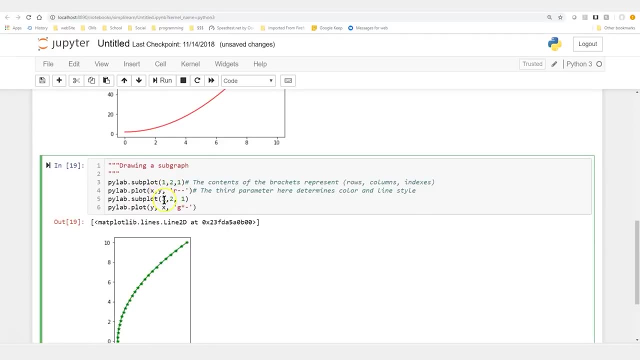 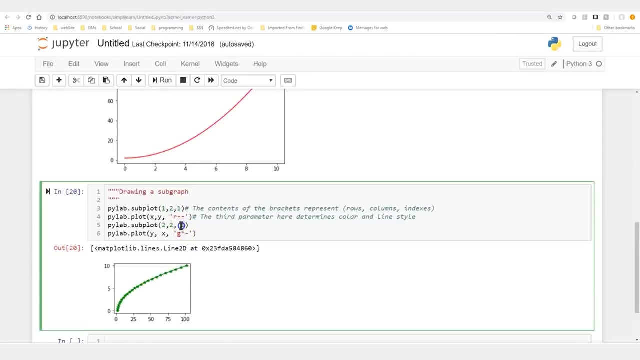 and find out what happens. now. this div is going to leave about 1 and if we do the column- it didn't really like that on the set up- it just disappears. so let's keep our column as 2 and let's change the row on the second one to 2 and run that and 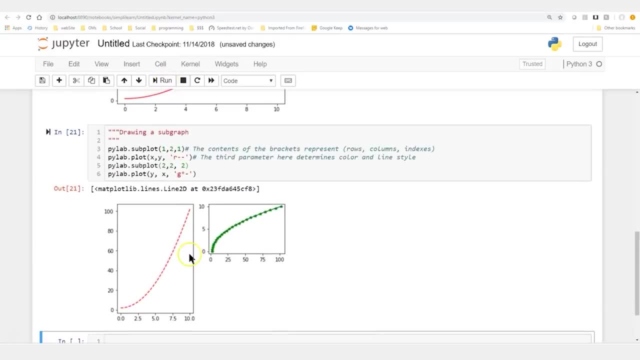 you'll see again. it kind of squashes everything together and cause some issues. so let's take the index. so these need a unique index and you can see here or I've made some changes. I said row 2 and look what happens when I change to. 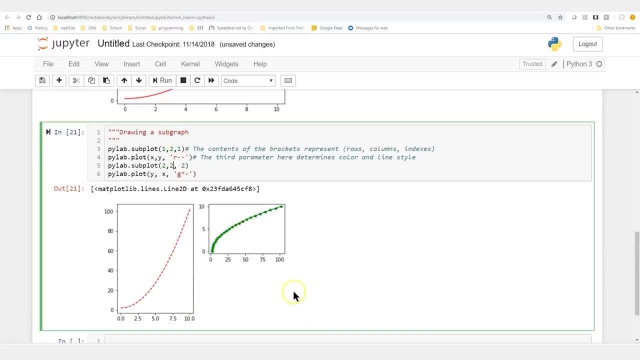 to index 2. I squished it up here so you could put another graph. underneath is what that does, And there's all kinds of different things. You really have to just play with these numbers until you get a handle on them, because you know you have to repeat it 164 times, according to Cambridge. 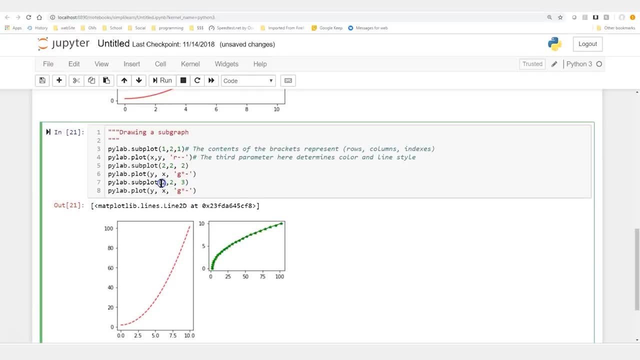 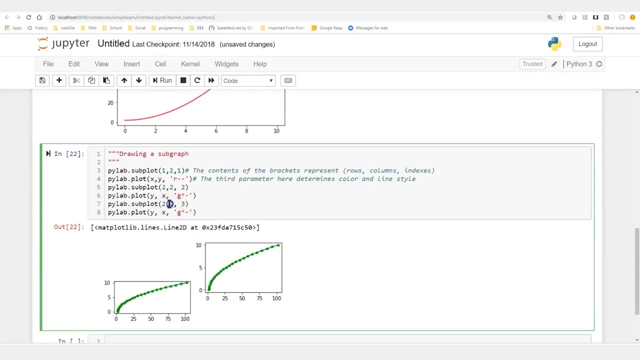 University if it's completely new to you And you can see right here where there we go. 3, run, There we go. But you can see it takes a little bit sometimes to play with these and get the numbers right. I hope they hit the wrong one. That's why Let's go 3 there. 3 there. run, There we go. 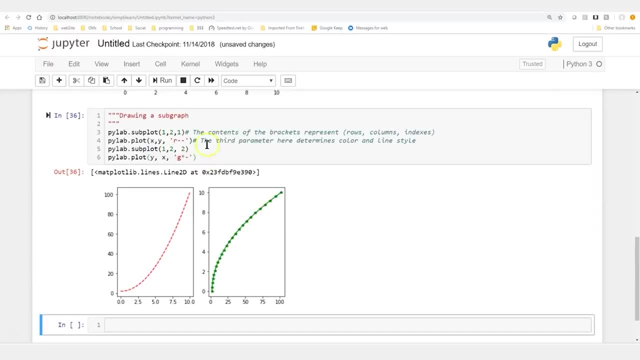 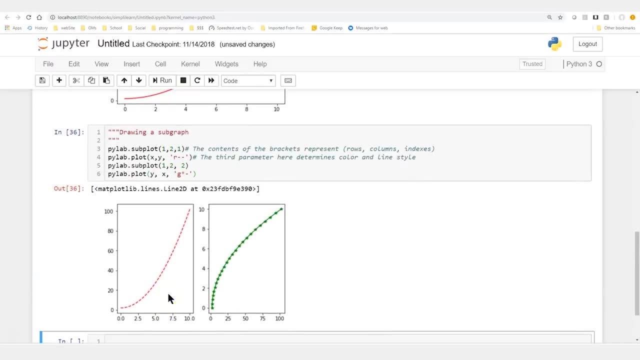 Now it's overlapping, So I have this doubled over here on the right. For now we'll just go ahead and leave this with the, where we have column and row 2 and the two different indexes, so they appear nice and neatly side by side, And then, as we just saw, as we were flashing through them, we can put. 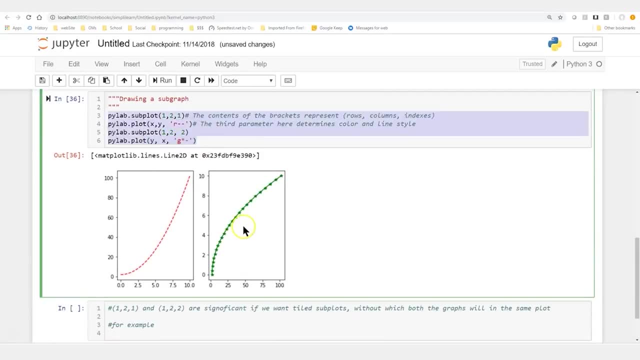 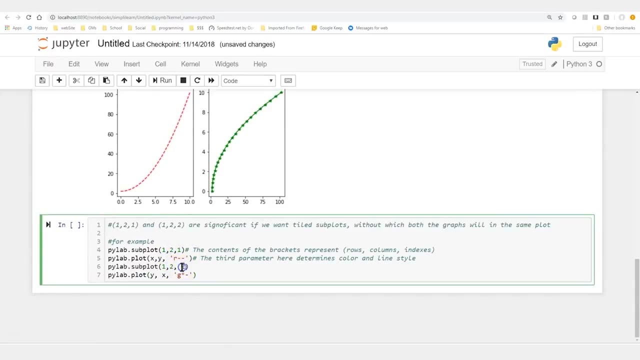 them on top of each other. And let me just highlight that and copy it down here, Paste it down there, And here we have 1, 2, 1.. And then we'll do 1, 2, 1 also for this one, And that puts the two subplots. 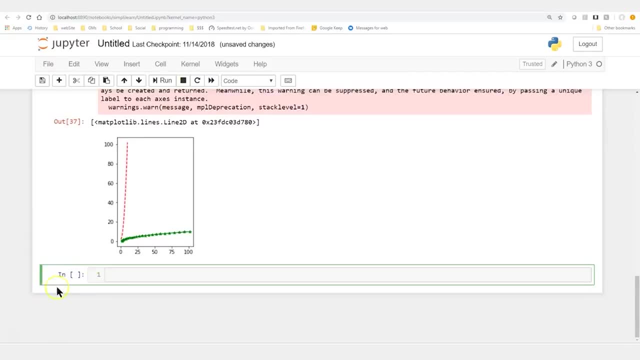 directly on top of each other, And that puts the two subplots directly on top of each other, And that puts the two subplots directly on top of each other Gives us that warning And you can see. we now have two different sets of data graphed on top of each other, And you can also see how it did. 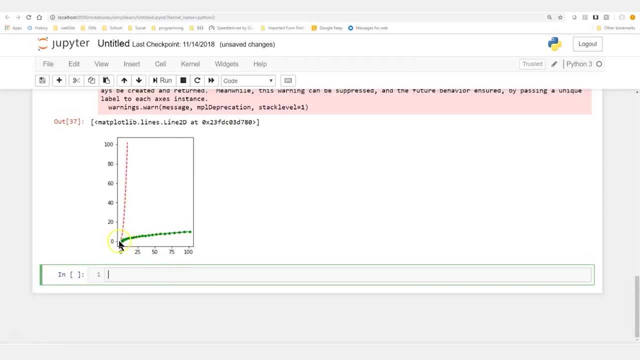 the indexes, Since one of them is from 0 to 10, that's the green one on the x-axis, and the other one is from 0 to 10 on the y-axis. So it took the greatest value of either one and then used those. 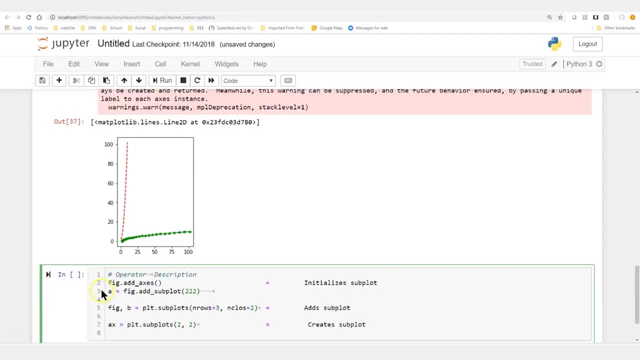 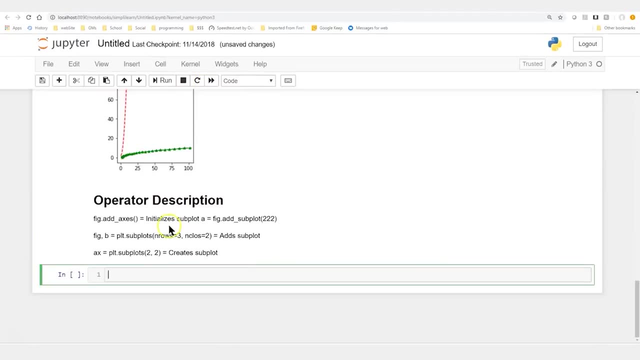 as a shared value. So let's next look at operator description And we'll go ahead and turn this cell into a markdown And run that so it looks nice. So fig, and you remember I talked about the canvas earlier. I briefly mentioned it. We're going to look a little bit more at the canvas later on, But that's what the 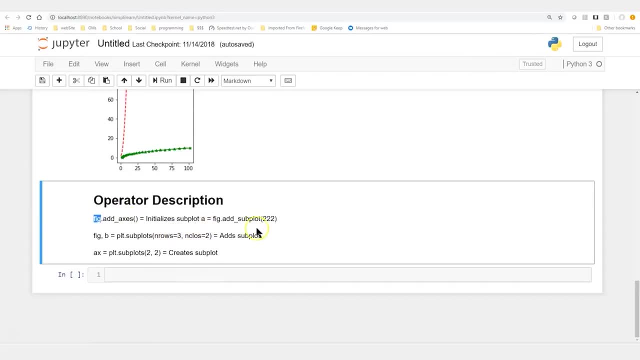 figure is Fig. we're going to add axes, So we're going to initialize a subplot. add the subplot in rows, in columns and all kinds of different things with this that you can do. Let's look at that code and see exactly what's going on, And I want you to notice that there's fig, which is the 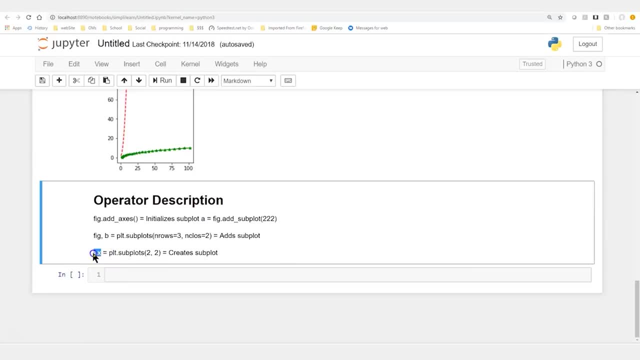 actual canvas in the matplot library And ax is commonly used for the matplot library, So we're going to choose to refer to the subplots. So when we're creating subplots you'll see ax equals plt, subplot. Earlier we did the pylab, So let's go ahead and import pyplot from matplot library And we're going. 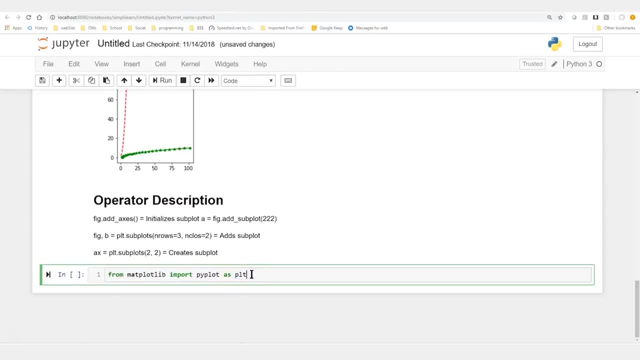 to do it as plt. You'll see that a lot. That's really the standard in the industry is to call it plt, just like pandas is pd and numpy array is np. Certainly you could import it as whatever you want, But I would stick to the standards. 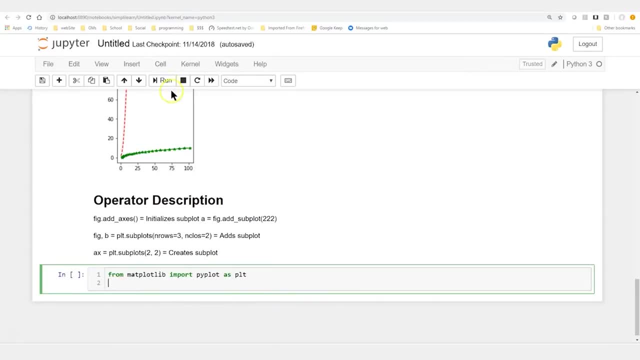 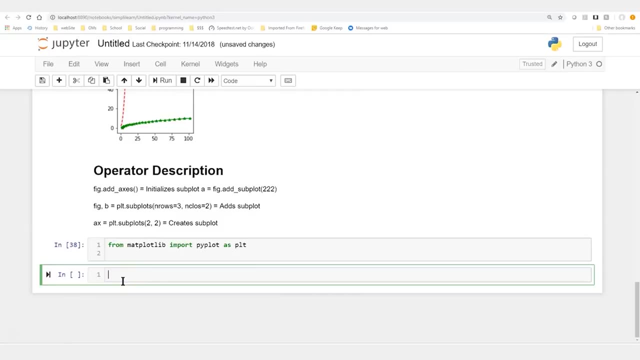 And we're going to do the same graph as we did in the matplot library And we're going to do the same graph as we did above with the pylab but with the plt. So if it looks familiar, there's a reason we're doing this because we want to show you how the figure part works and working with the canvas. 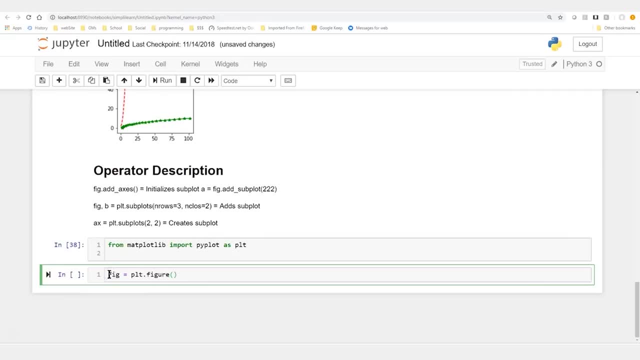 goes. But we're going to do the same plot as we did before And we'll call it fig And we're going to set that equal to plot figure. So there's our figure or our canvas on there, And let's create a. 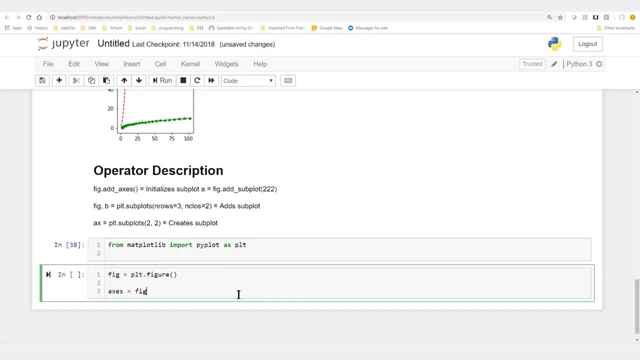 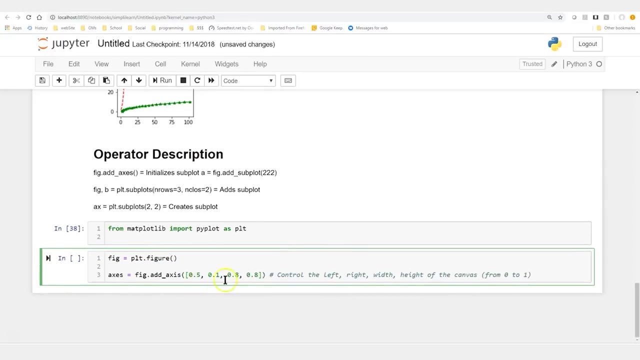 variable called axes And we're going to set that equal to fig dot add axes. And in this we're going to control the left right, the width, the height of the canvas from 0 to 1.. So we can go ahead and I'm just going to put some stuff in there. I got 0.5, 0.1, 0.8,, 0.8.. So when you're 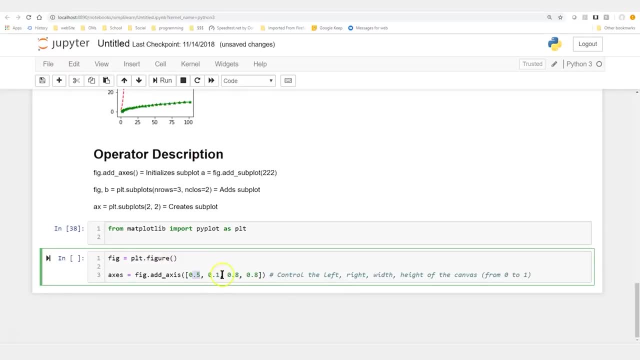 looking at this, this is a 0 to 1, or you could say 50%, 10%, 80,, 80%, But it's a control. It's going to control your left and your right, along with the width and the height. So the width and the height we're going to use. 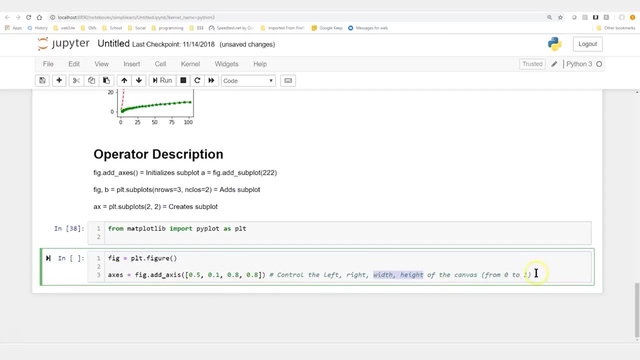 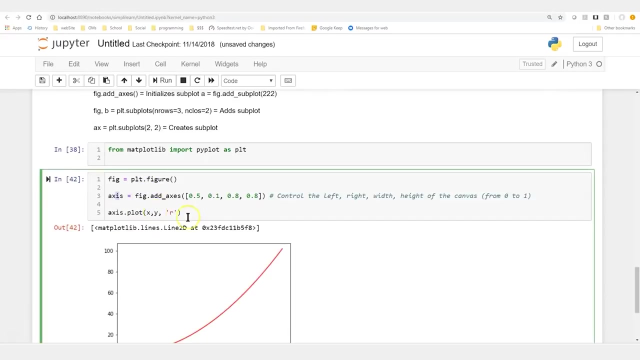 80%, And we're going to have like a little indent on the left and the right, And this will look familiar From above: axes, dot, plot, x, comma, y, And then let's give it a color. How about red? Since we recreated the same graph, let's keep it uniform. Oops, And it helps if I use axis instead of axes. 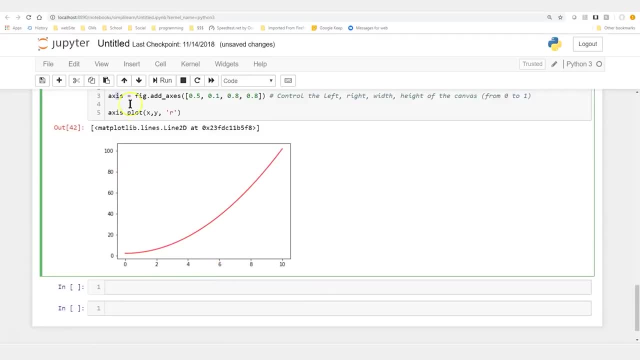 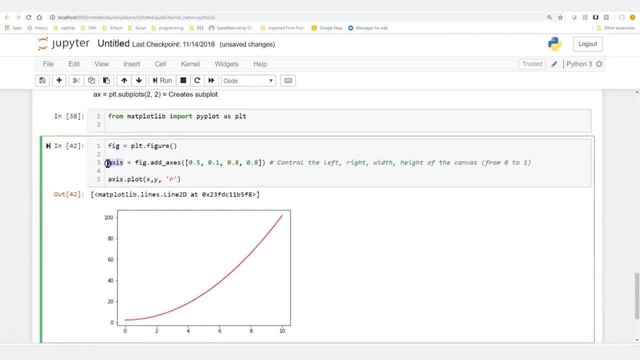 I don't know where that came from, But this looks identical to the one we had up above. So here's our axes: plot x, comma, y of red. Same graph, same setup, But this time we've added a variable equal to the. 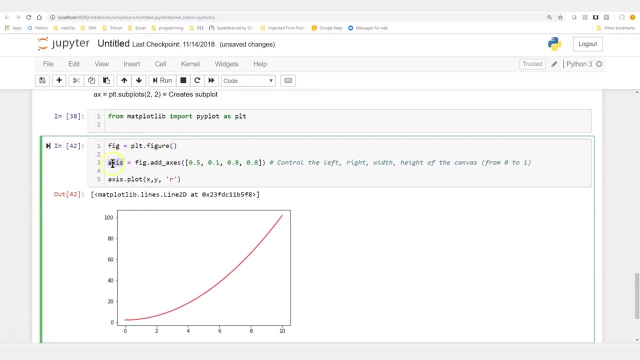 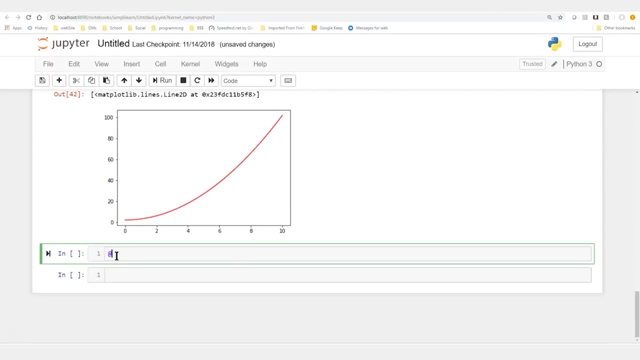 figure, dot, add axes. So our plot figure is our canvas, Our axes is what we're going to working in, And then our axes dot, plot x, comma, y, And again we can draw subgraphs. Let me put that down here, Just like we did before And a little different. 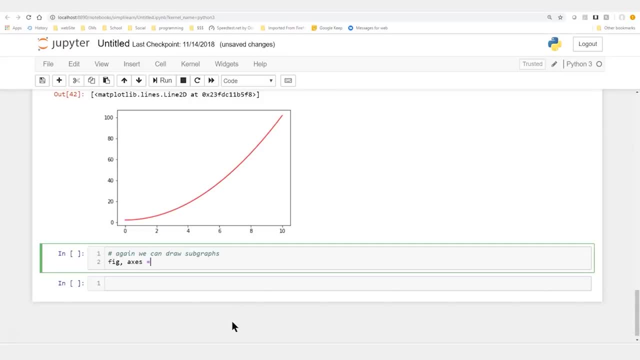 notation: here We're going to have fig, comma, axes equal plt, dot subplots, And in here it's going to be the number of rows. We're going to do one row and columns equals 2.. So if you remember before, that's what we did. 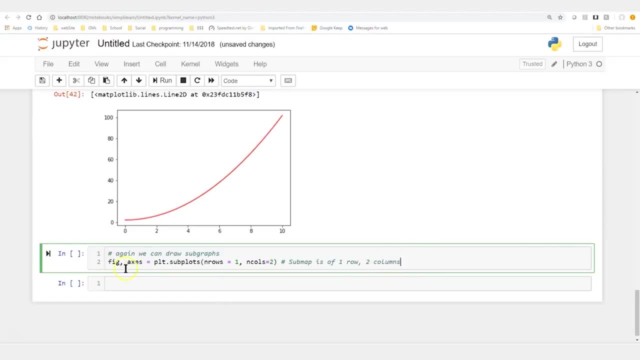 We had one row with two different graphs on it. We're going to do the same thing, But note how we did this. Here's our figure, our canvas and our axes. We're going to create actually two different axes. We're going to create row 1, column 2.. 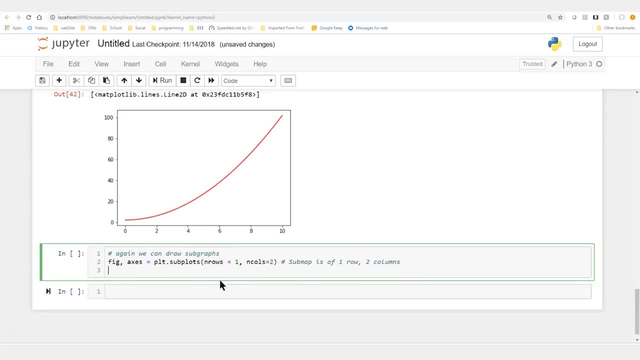 And so axes is an array of information. So we can simply do for: let's do ax in axes. This will now look familiar: Ax dot plot. We're going to do x comma y. We'll go ahead and make it red. 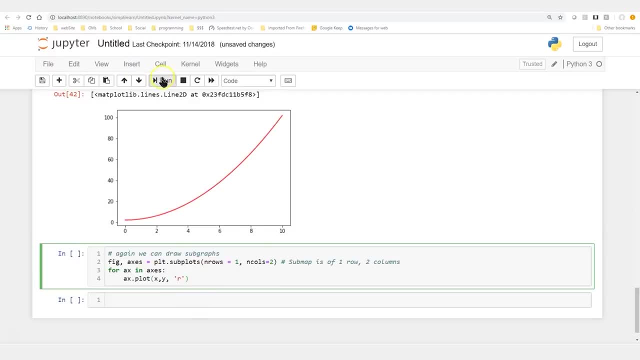 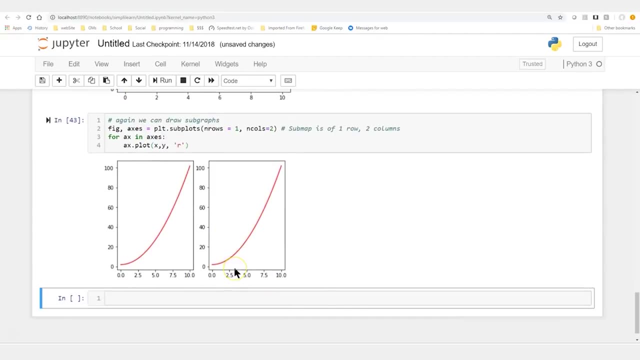 Keep everything looking the same. Remember nice uniform graphs. Everything looks the same And if we go ahead and run this, you'll see we get two nice side-by-side graphs. So just as we had before: the same look, the same setup. 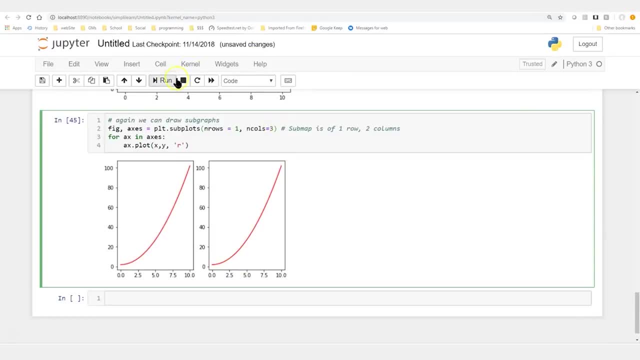 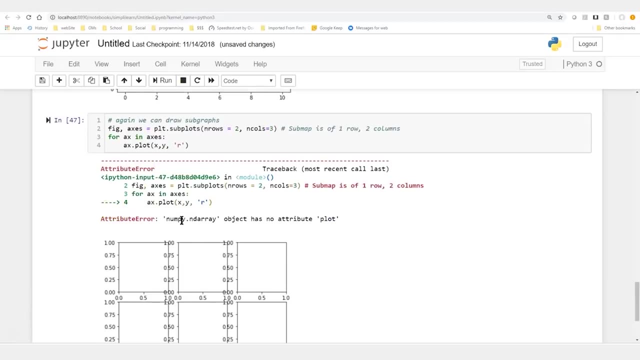 And just for fun, let's change in columns to 3. We'll run that And now you'll see we'll have 3 on there And let's see if we make it a little bit more interesting. We'll do in rows equals to 2. And you can see down here we're going to get an attribute error. 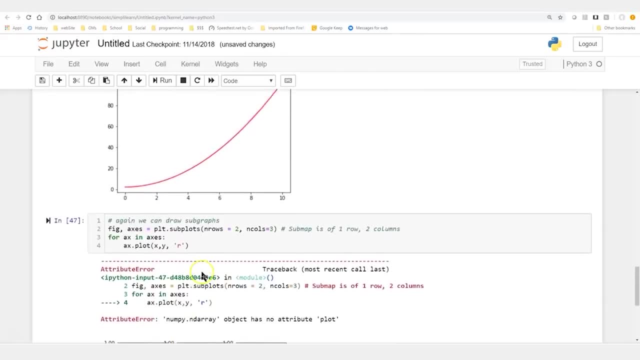 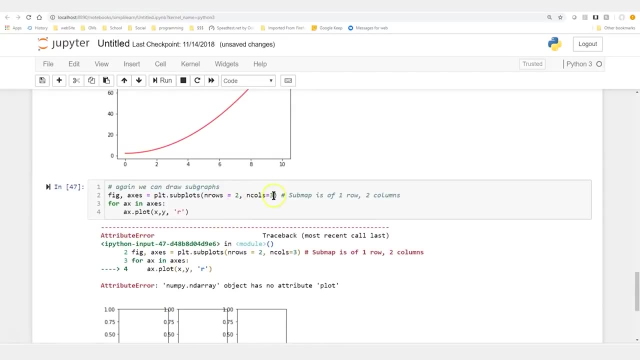 because it's trying to scrunch everything together. So it does have a limit how much stuff you can put in rows, So we'll run one small space. That's important to know. You can fix that by changing the canvas size, which we'll look at in just a minute. 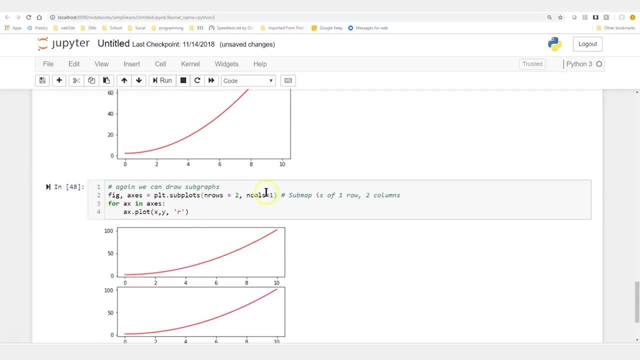 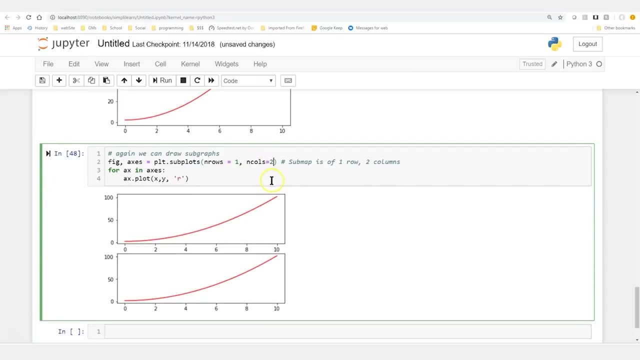 And there's other ways to change it on here. But here we go. We can do in rows 2 and columns equals 1.. You can see two nice images right above each other. We'll go back to the original: One row, two columns side-by-side left to right. 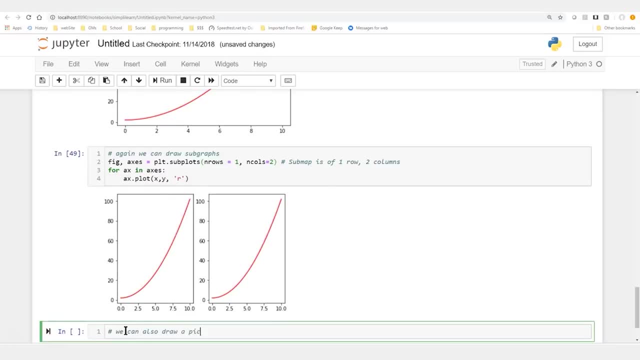 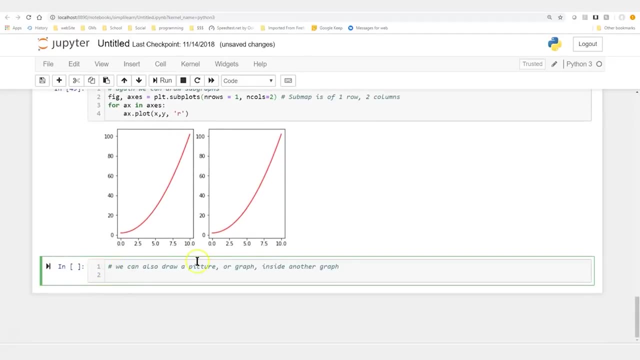 And we can also draw a picture or graph inside another graph. That's kind of a fun thing to do. It's important to note that we can layer our stuff on top of each other, which makes for a really nice presentation. So let's start by fig. We'll create another fig here. 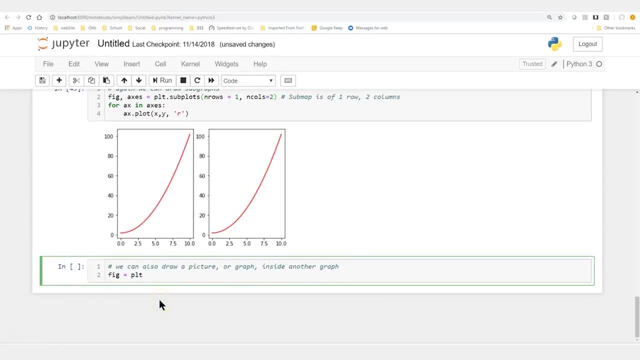 So we're going to start over again with our canvas. We set that equal to pltfig here. So there's our new canvas And let's do axes. We'll call it axes 1 and 2.. Axes 1 equals fig dot. add axes. Remember this from earlier. 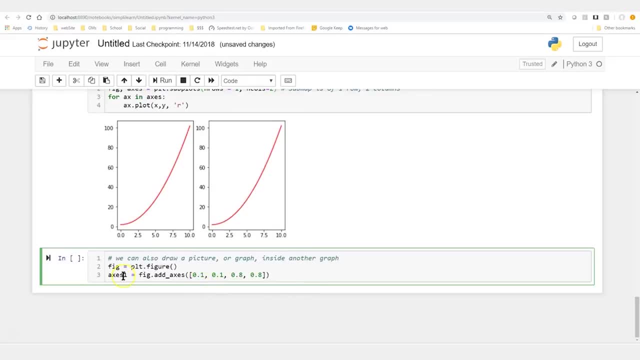 And this here similar numbers we used before Saying how big this axes is. this figure in the axes is: So this is going to be the big axes And let's do: axes 2 equals another fig. add axes And then 0.2, 0.5, 0.4,, 0.3.. 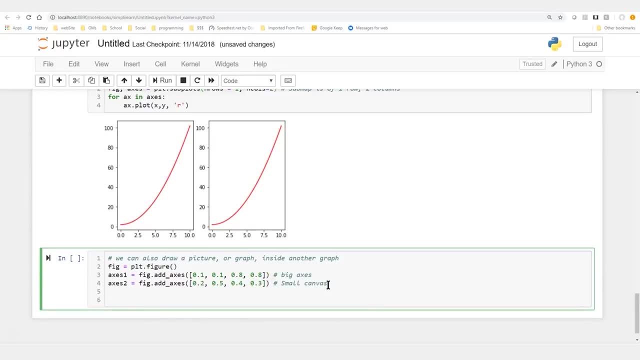 And if we're going to do this, they need data on them. So let's go ahead and plot some data on our axes. So axes 1, dot plot, And we'll make this simply: x comma, y comma, make it red. And then let's go axes 2, dot plot. 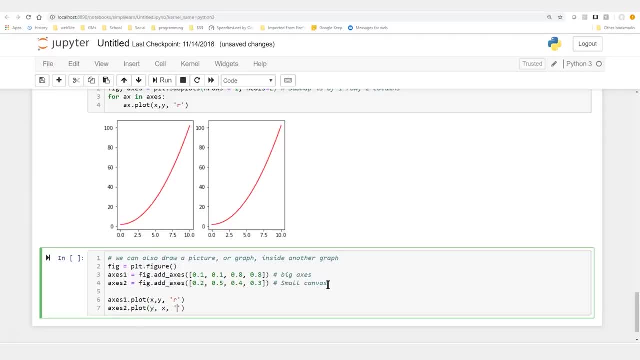 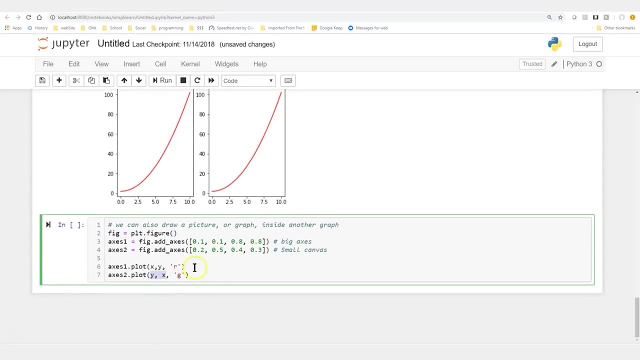 And let's reverse them: Y comma x comma green. There we go, Doing what I told you not to do. You shouldn't be swapping axes around and plotting your data in five different directions, because it's confusing. Let's go ahead and run this and see what this looks like. 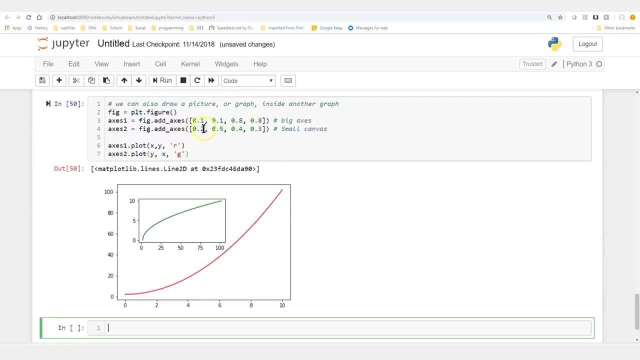 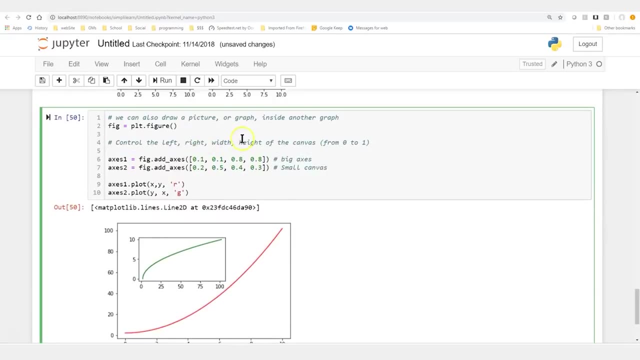 And then let's talk a little bit about this. We talked about the 0.2, 0.5, 0.4,, 0.3.. And let me just grab the annotation for that. That's left, right, width and height. 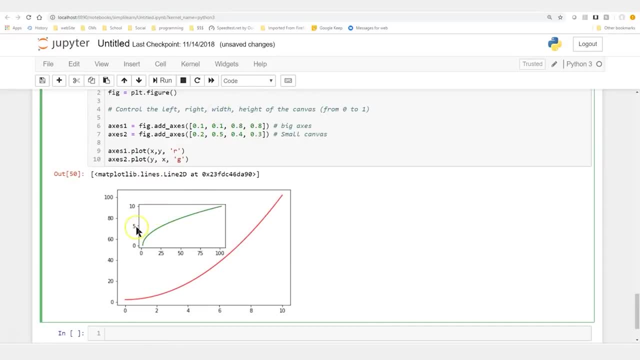 So we have in here that this is going to be left right. So here's our left as 0.1 in 0.5.. You know what? Let's just play with this a little bit. What happens when I change this to 0.1?? 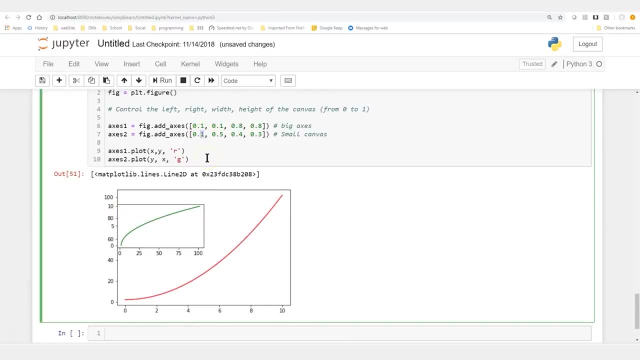 It moves it way over to the left. So there's our 0.1.. So we can make this 0.4.. Run that, There we go, So you can see how you can move it around the branches on here: 0.2.. 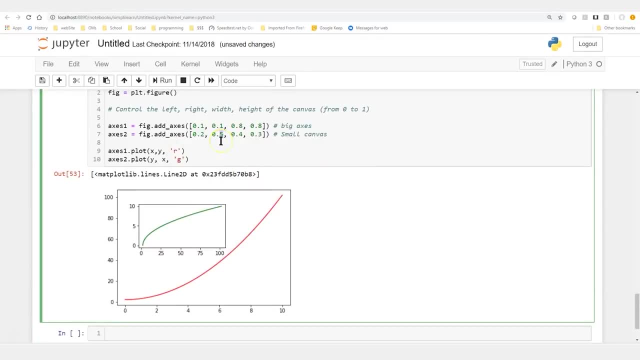 0.5 is the left, so that's our right. So let's see what happens when we do point: Oh, let's make this 0.1.. And that actually they had it down as left right. I thought this was wrong. 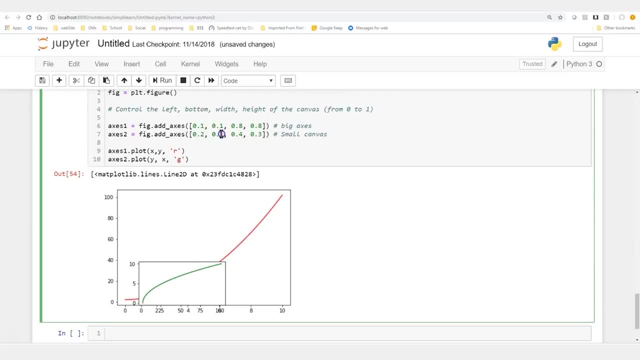 It's actually how far from the bottom- Let me switch that on here- Bottom, There we go. So we had it here on this. We can go ahead and put that back to 0.5 and run that, And this is 0.3.. 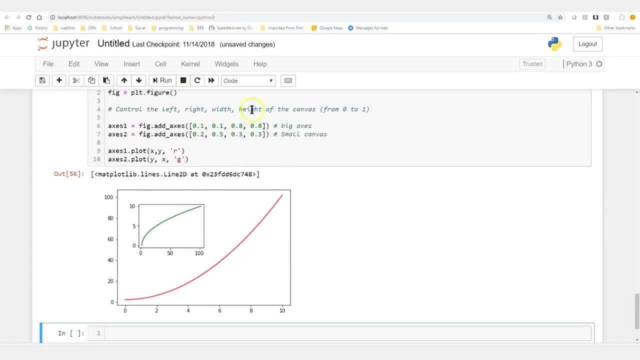 Let's make this 0.3 also, And that is the width, And then of course there's the height. We can make that really tiny. Actually, let's do 0.2.. Let's run that And you can see it changes the height on there. 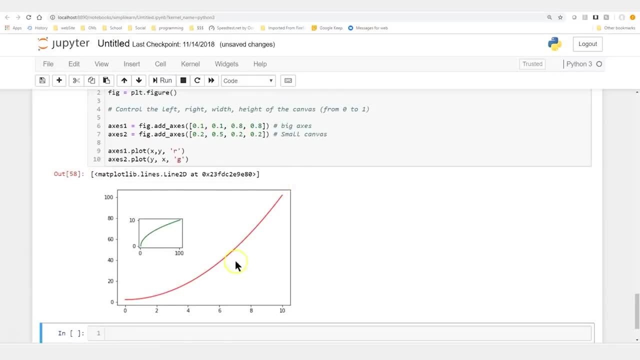 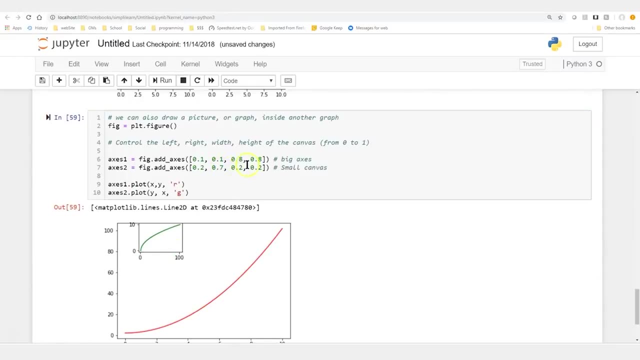 We can make it even smaller: 0.2 by 0.2. And, as you can see, you can get stuck playing with this to make it look just right. It can sometimes take a little bit, Certainly once you have the settings. 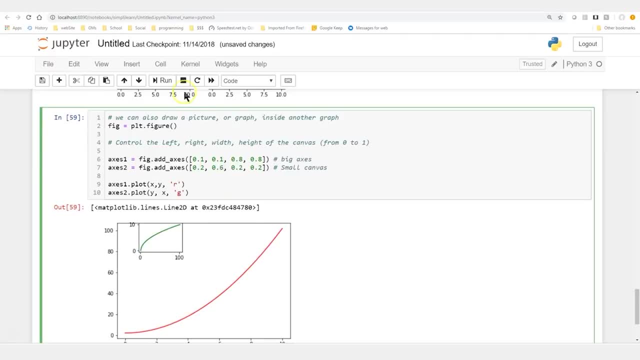 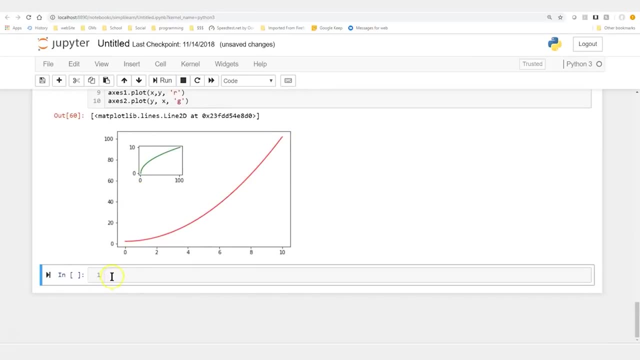 if you're doing a presentation, you try to keep it uniform unless it doesn't make sense for the graph you're working on, Try to keep the same colors, the same position and the same look and feel. And I mentioned earlier, we can adjust the canvas size. 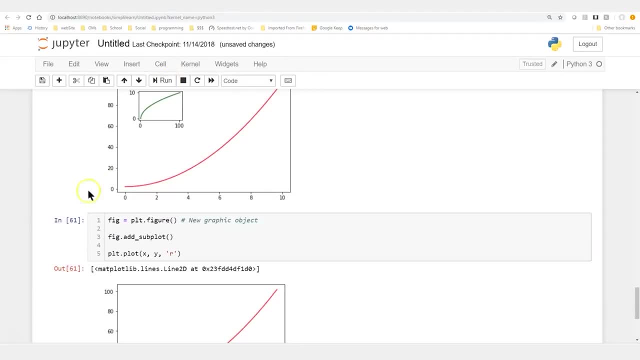 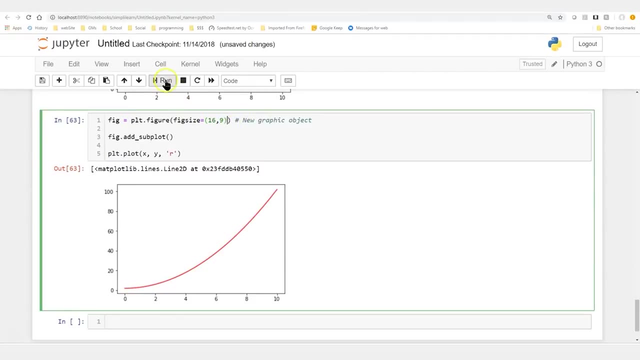 So this is from earlier. I just copied it down below. We're going to replot the same data we've been looking at And what we can do is we can change the figure size to 16 by 9.. Let me run that and show you what that looks like. 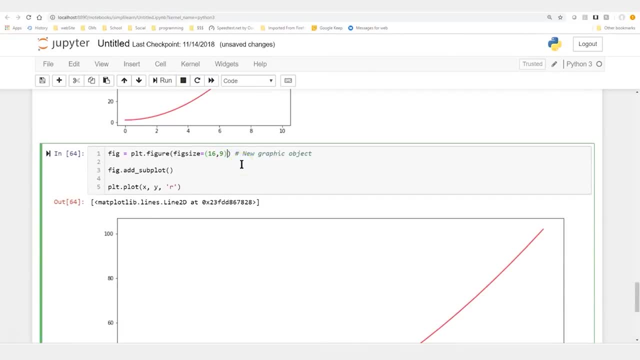 So it fills the whole screen. And then, if you are normally when you're working on the screen, you don't worry too much about this. But we can set the DPI to 300.. Run that. There it goes. This is your dots per inch. 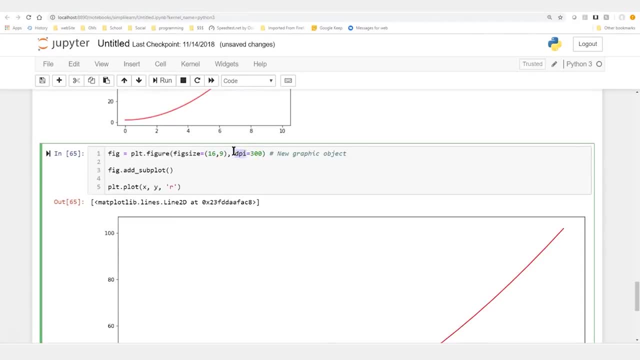 And if you are doing an output of this and you're printing a hard copy, you want the higher quality. I would suggest nothing under 300. if it's a professional print You might get a little less than that, but whenever I'm doing professional graphics and printing them out on something, 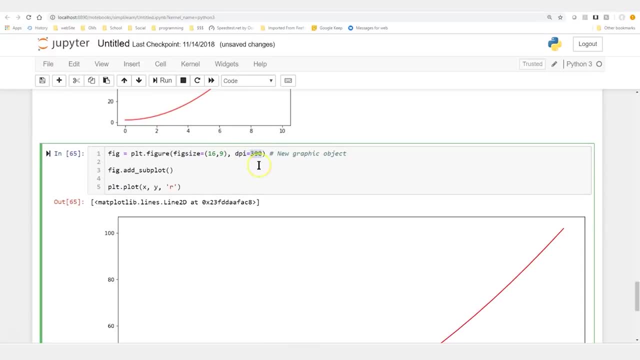 300 dots per inch is kind of the minimal on there. You can go a lot higher too, but keep in mind, the higher you get, the more memory it takes and the more lag time and the more resources you use. So usually 300 is a good, solid number to use in your dots per inch. 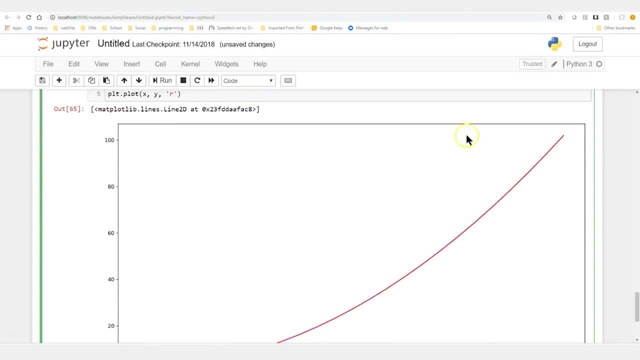 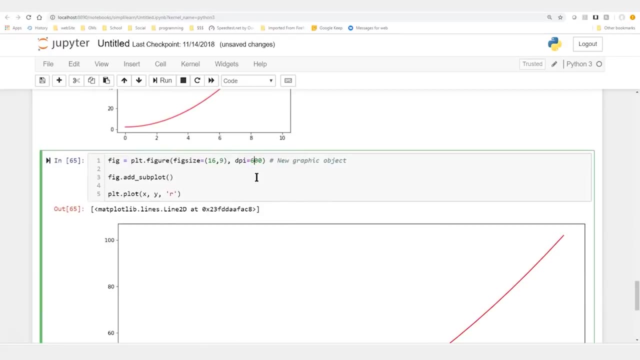 And you can see it draws a nice large canvas here which is 16 by 9. And then the DPI is 300 on here, so it's a little higher quality. Just out of curiosity, I wonder how long it takes to draw something double that size. 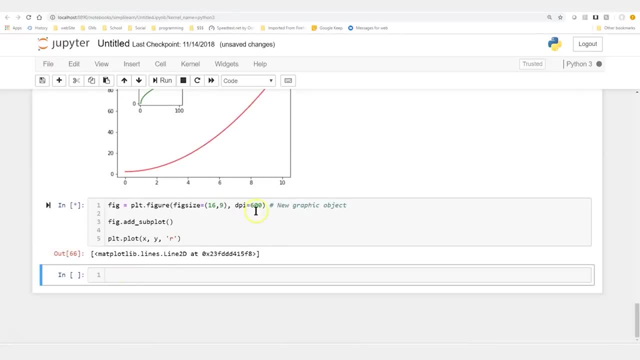 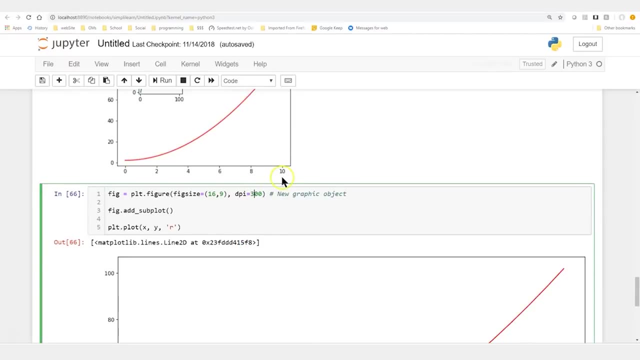 600. And you can see here where, at 600 DPI, it's going to take a while. There it goes, Just because it's utilizing a lot more graphics, And let me just go back to the 300.. No, we'll actually do. 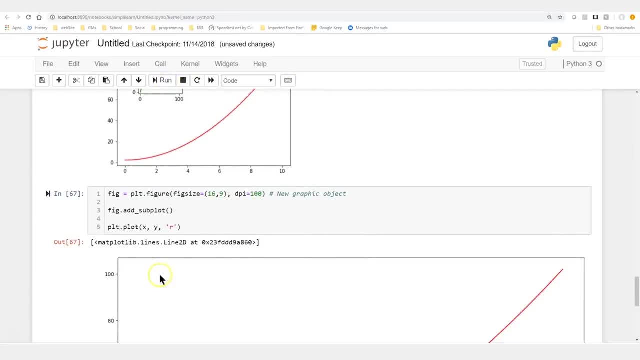 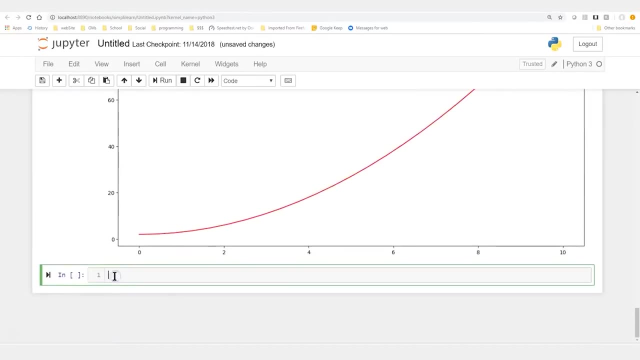 let's do a 100.. You're not going to see a difference on this because it is web-based. graphics are pretty low And up here you saw I did this with the plot figure. This works the same if I do figure axes, subplot, figure size. 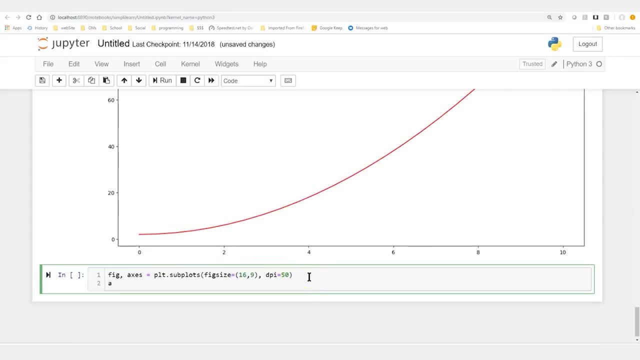 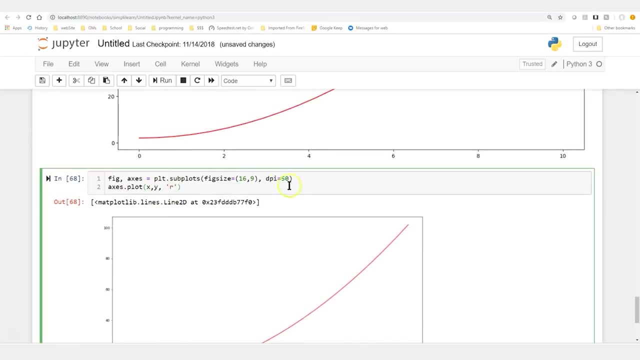 and then we'll go ahead and do axesplot x, y comma. we'll stick to red. Let's go ahead and run this And you should get almost the same thing here. Here's our axes on the subplot on here with the fixed size and the DPI. 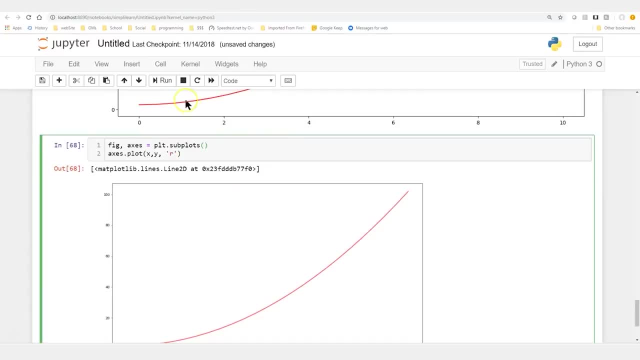 Let me take this all out. Let me just remove all that real quick, Run it again. There we go. Now we're back to our original figure And let's look at some of the other things you can do with this. One of the things we can do is we can set a title for the axes. 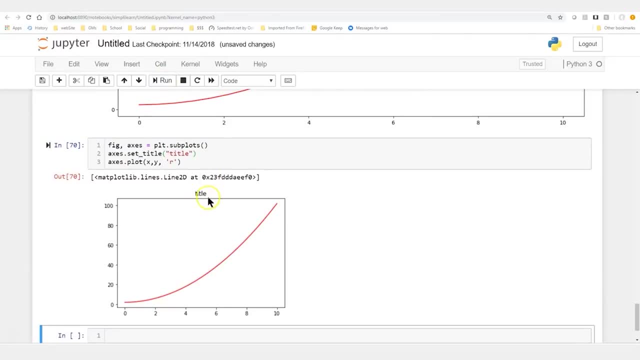 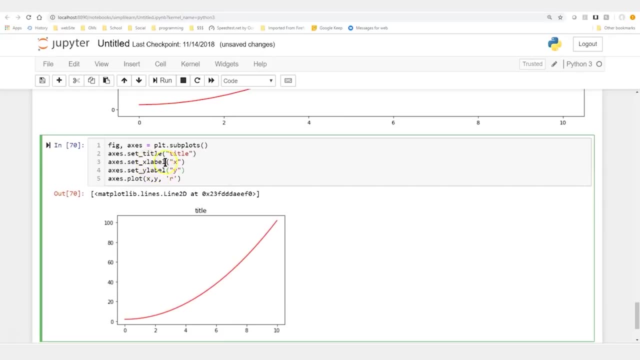 So axes set title. You'll see right here, since I put this on the axes, it's the main title for the whole graph And if you're going to have a title you should also label. So we can label our x label. 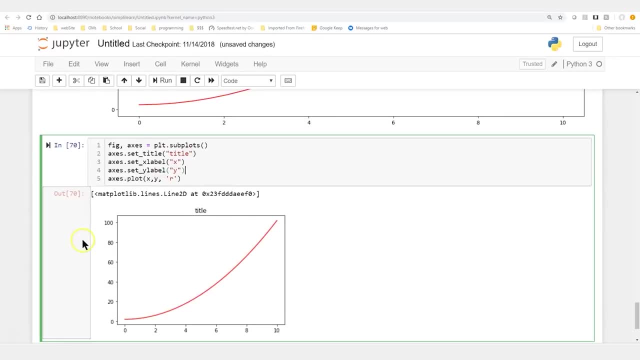 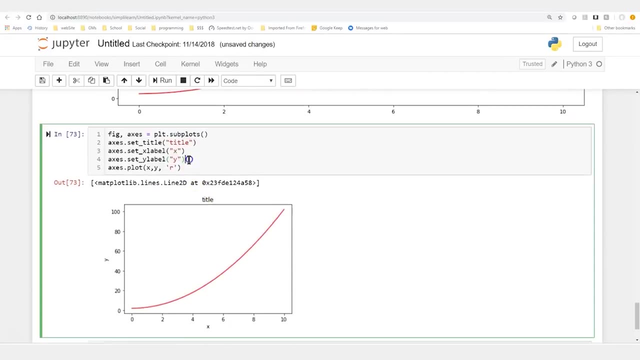 and we can set our y label. In this case, we're just going to call it x and y, Keep it nice and uniform, And if we run this, you'll see that we've added a nice x label and y label. Whoops, where'd they go? 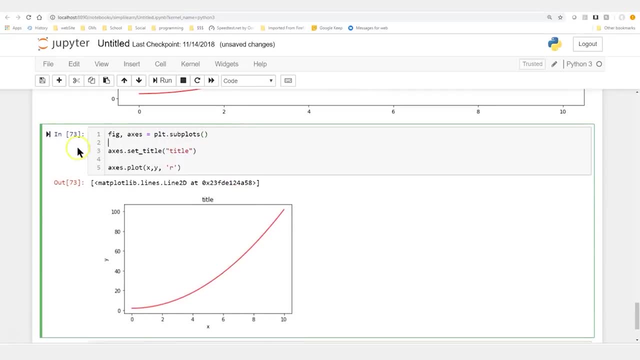 And it turns out in this environment that you have to put it before the title. So let me go ahead and put it before the title, And there's our x, y and let me run that, And of course we can also do up our size a little bit. 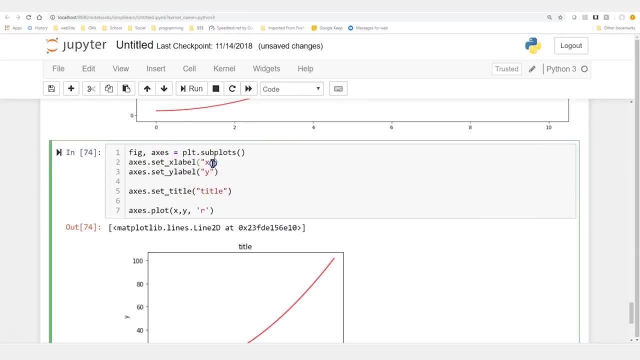 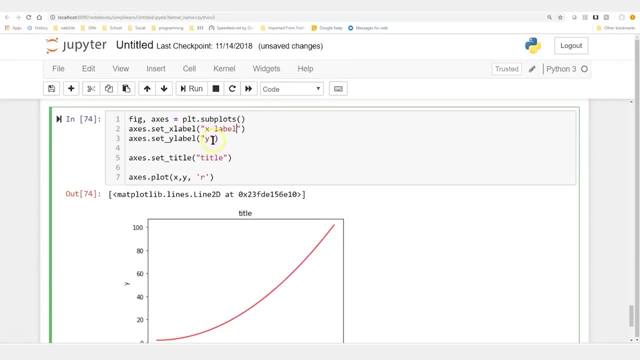 so you can see what's going on a little better. So here we have x label x. If you come down here, you'll see our x label and our y label. We can, of course, change this to x label. You can change this to y. 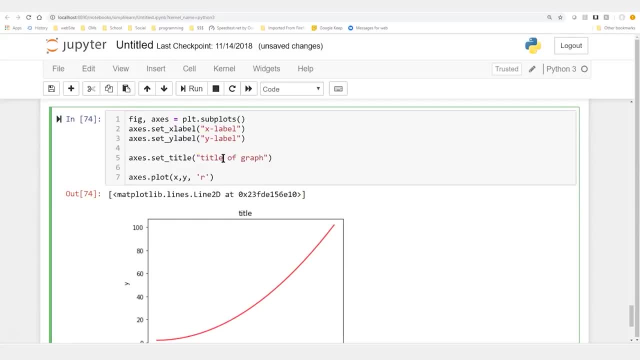 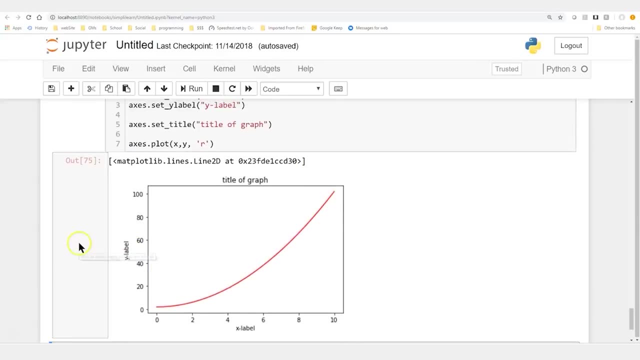 It can be whatever you want on here, of course, And our title graph. There we go Run. So here we have our title graph, our y label and our x label, all set up on our nice little plot. And then, before we move on to the next section, 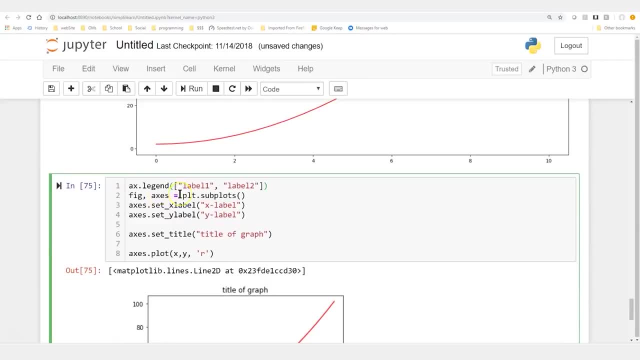 let's do one more thing on here. We have a thing called the legend And we're going to do. we're going to set our ax legend, label 1, label 2 up here. That's the first thing. We don't have the format for it. 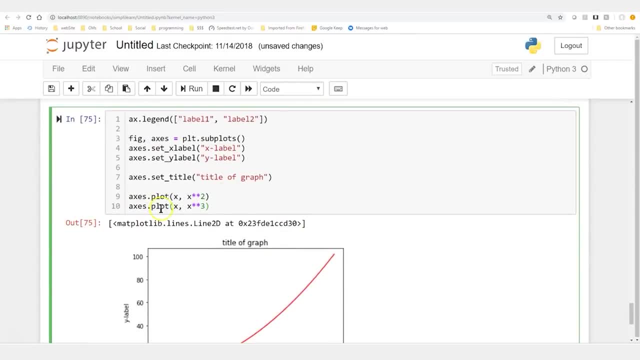 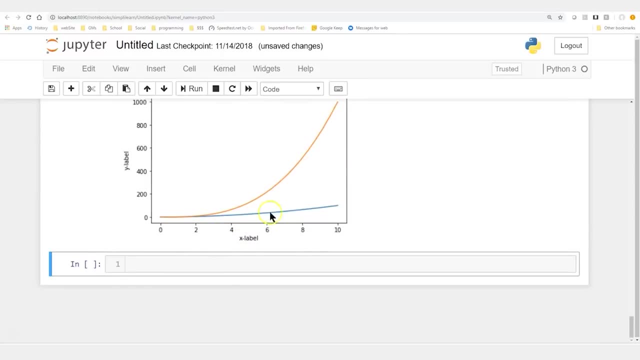 but let's go down here and actually use it. I'm going to do two different plots. We're going to have axes plot x by x times x squared and x cubed, And if I run this you'll see it puts two nice graphs on the setup on there. 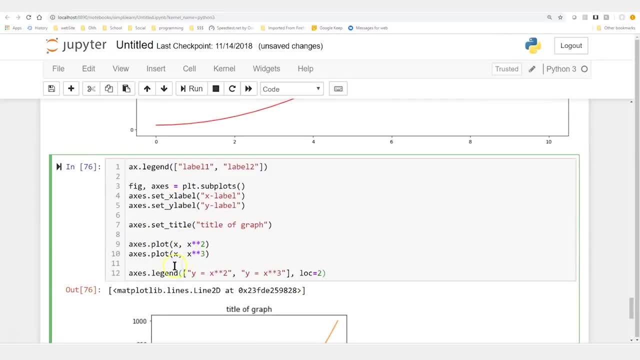 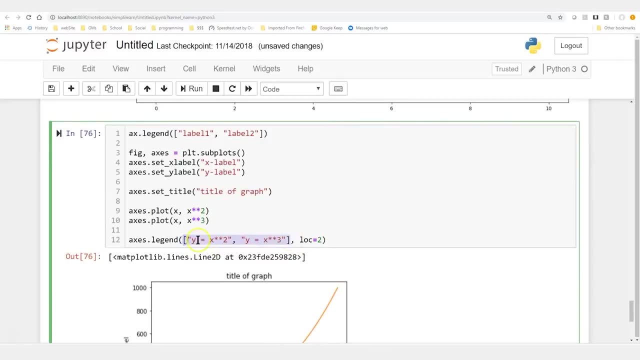 But it's nice to have a legend telling you what's going on. So for the legend we can actually do axes, since we have the two plots- legend, And on here we've created an array And we have y equals x squared. 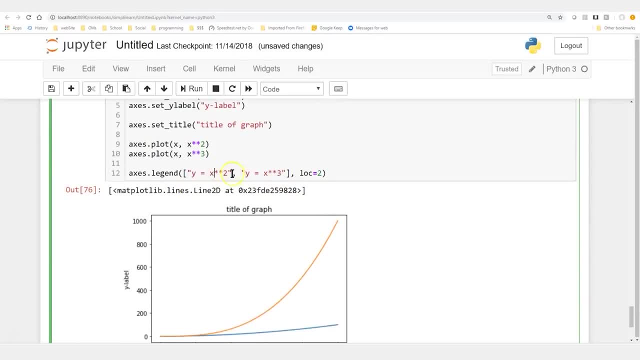 y equals x cubed, And we can actually put this as whatever you want. Those are just strings. And then location 2. And let's go ahead and run this and see what that looks like And you can see it puts a nice legend. 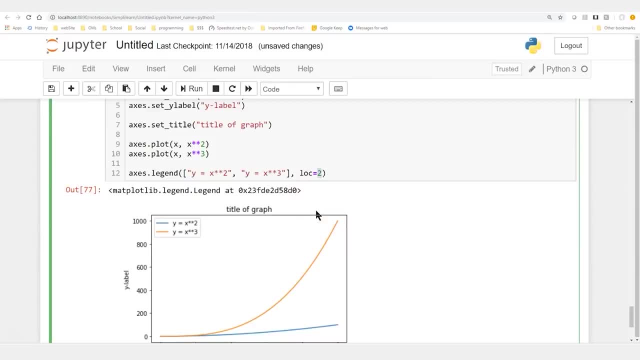 on the upper left-hand corner, Location 2.. We can do location 3 and run it And it drops it down to the bottom, Location 1.. I can't remember where that's at There we go upper right, So each one of these is a number. 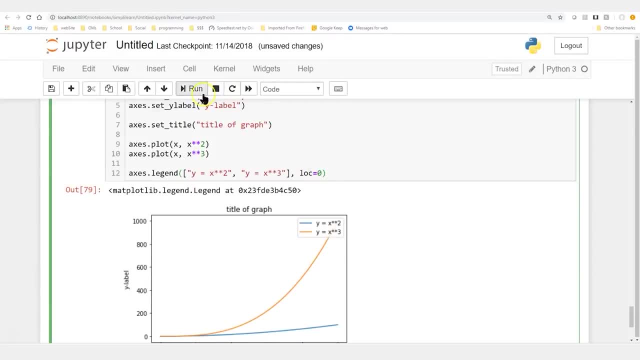 that refers to the different locations on the screen 0. Kind of have to play with them or look them up to remember where they're at, But it does work. It just kind of moves around depending on where you want your legend data on there. 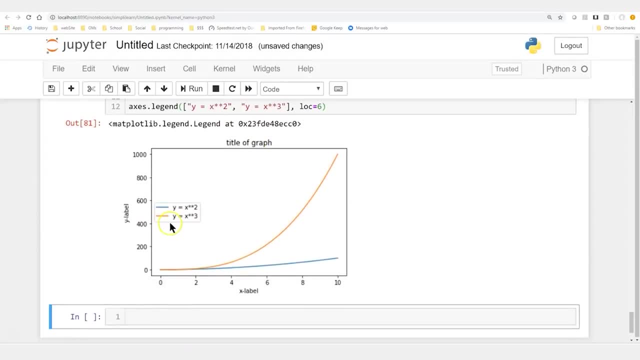 So on this section we cover the title of the graph, the y labels and legends. This is we're getting into some starting to look really fancy here, So we now have something we can actually put out. You'll see, the title of the graph looks a little fuzzy. 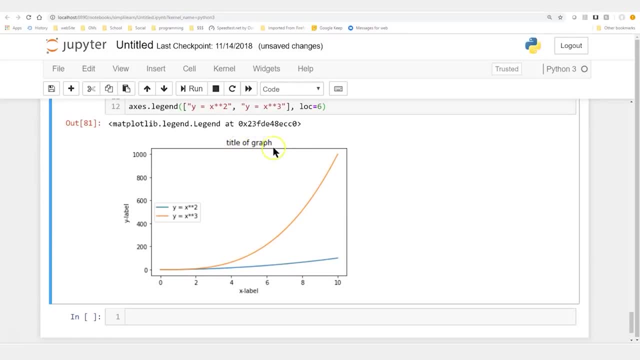 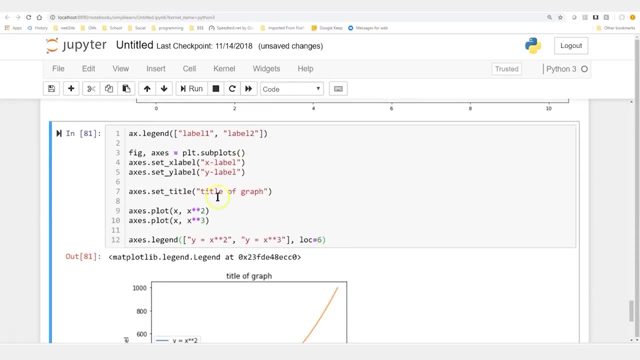 So I might, in a web setup, put the DPI up a couple notches, Maybe put it at 200.. 100 might work fine. Just so you know something to notice on here when you're playing with these different things. 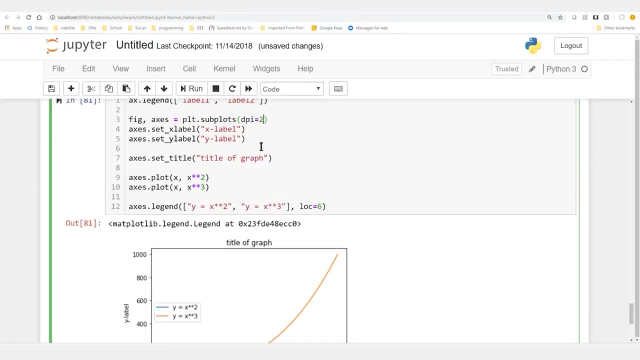 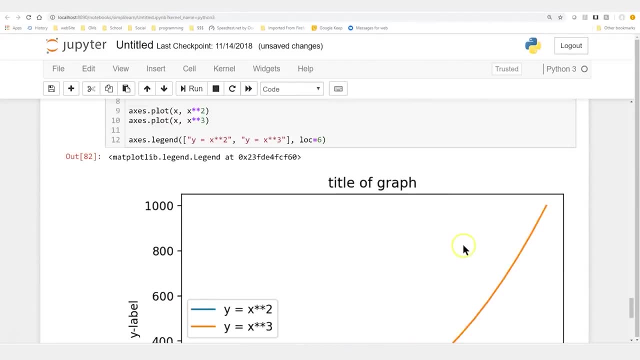 We've got our subplots. DPI equals- oh, let's do 200 to see what that looks like. So you can see it now is a lot clearer. It's also larger, So it's a nice little feature you can throw in there. 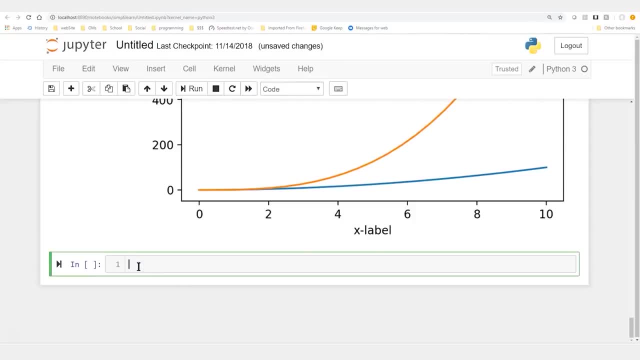 with your DPI dots per inch. So the next section is: let's look at some graph features. We're going to look at line color, transparency, size and a few more things on here And, oops, I forgot the main title. 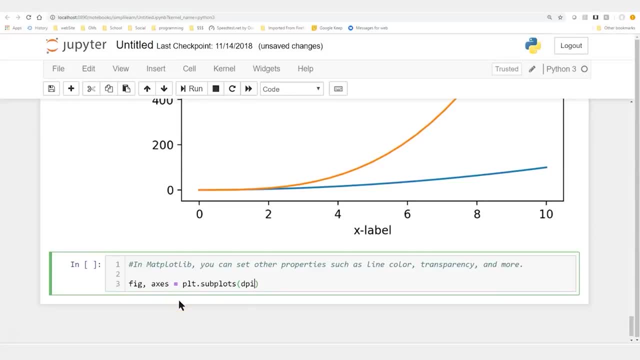 So we have our figure and our axes equals our plot and subplots, And I'm going to go ahead and say DPI equals 150.. So the graph comes out nice and large and easy for you to see And let's go ahead and do three plots on here. 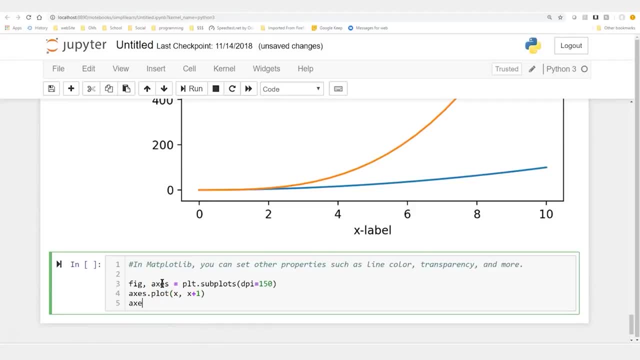 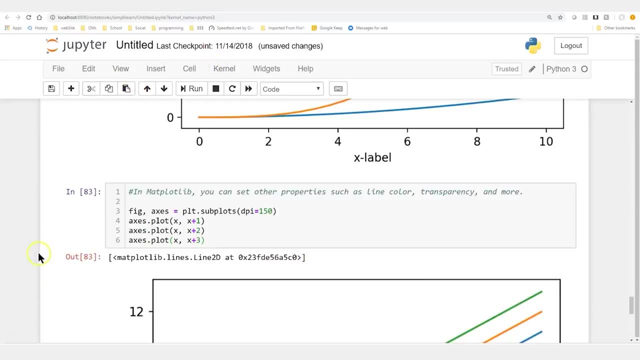 We'll do X by X plus one, So it's just going to be a straight line Plot X plus X plus two And axes dot plot X, X plus three. So it looks like we're doing nearest neighbor setup or showing how it located data. 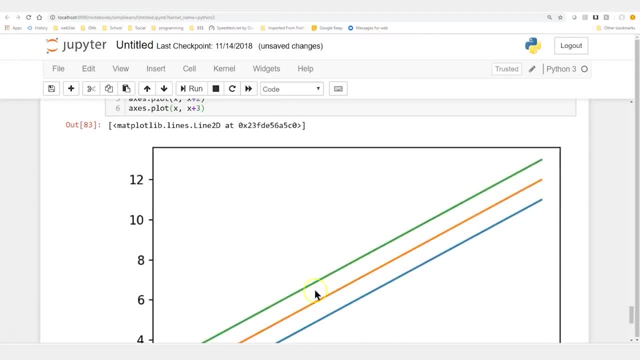 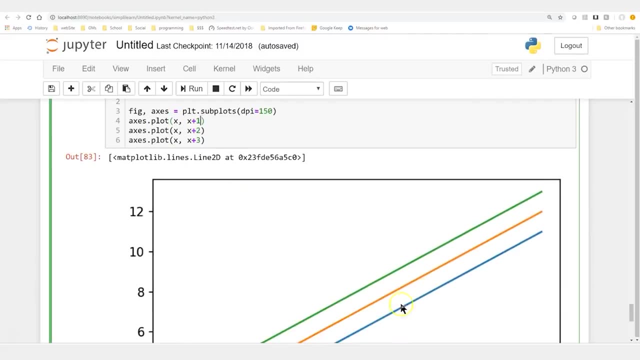 and putting your lines on there between the nearest neighbors. There we go. So it draws a nice little graph with three lines on it. One of the things we can do is we can control the alpha on this Oops And you can actually see the. 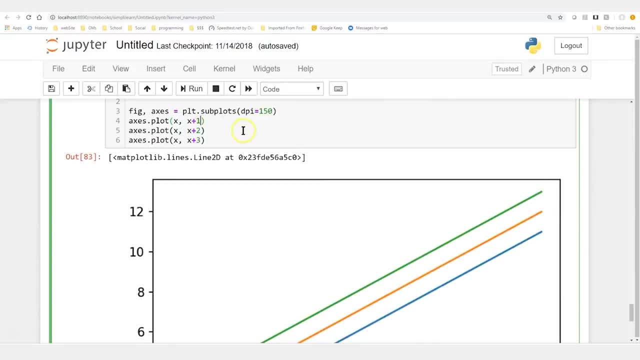 when they did these lines, it automatically pulls in different colors for your setup. So there's some automatic automatic things going on in there And a lot of times we do that comma R. but we're going to do color equals red. another notation on here: 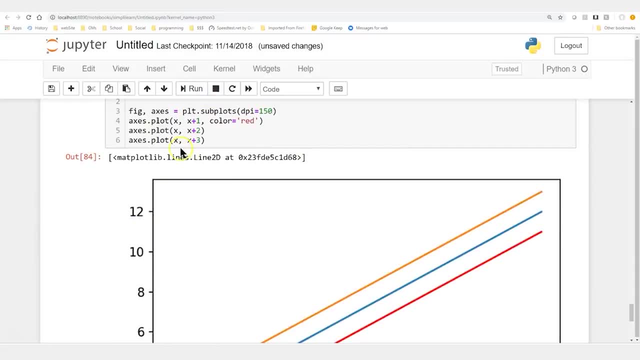 Let's go ahead and run this Now. we have a bright red line down there And with the map plot library you're not limited to red. You can also use the one of many different color references, as you see here with the pound sign. 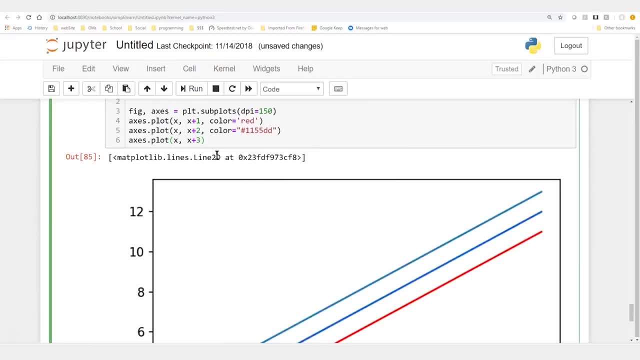 one one, five, five DD, which just is just blue. And we can do the same thing with another color on here which turns out to be green, And I can just as easily do this: Green, blue. Oops, there we go. 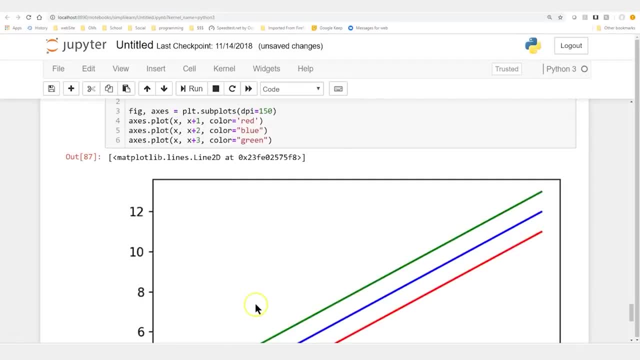 Blue and run that And you'll see. here we have red, blue and green, And what I want to do is I want to make this: we're going to set what's called the alpha on this And we're going to set this equal to 0.5.. 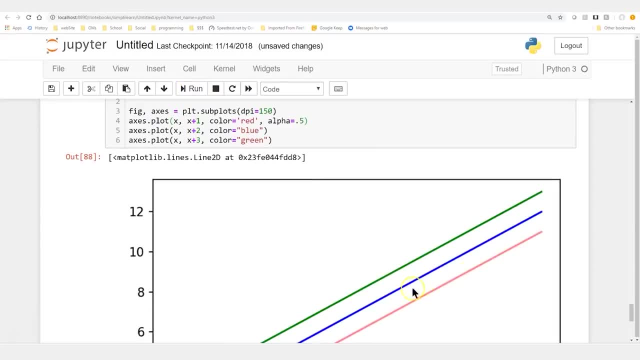 So this is halfway C3.. Halfway through, when I run this And it's almost going to look pink because you can see through it And let's change this just a little bit, just to make this kind of fun, Let's square it. 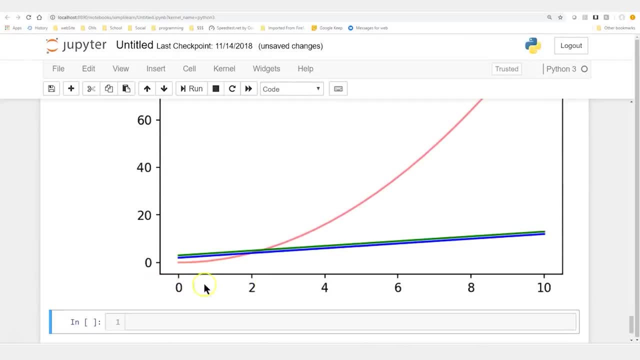 There we go, run it. So now we have this nice square that comes up And you can see when it crosses it, because I plotted these two lines after it and they have no alpha. the red is behind those lines or, in this case, pink. 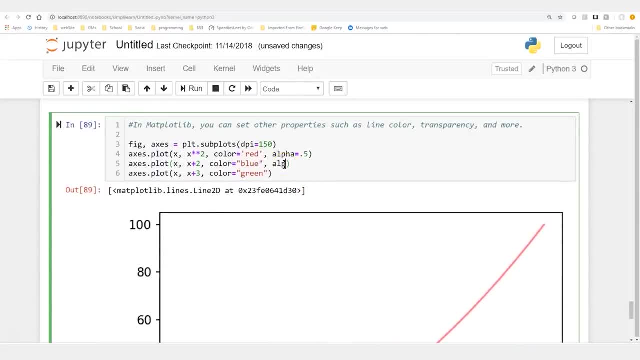 because we did the alpha halfway through. So let's go ahead and do this. Alpha equals 0.5.. And oh you know what, Instead of squaring it, let's take it to the 0.5 power. That'll be kind of interesting to see what that does. 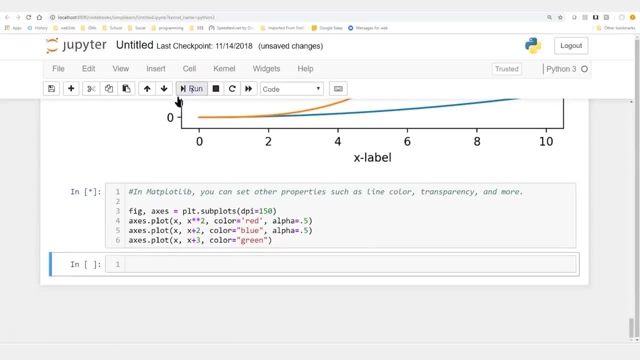 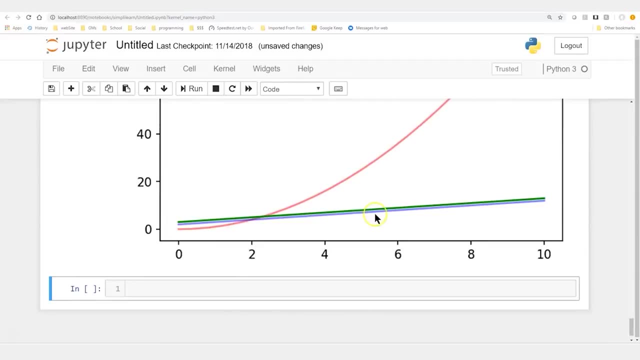 We'll just go to keep it squared There. we go And run that And let's go back and look at this where it crosses over, And the first thing you'll see right here is on the blue. it's kind of light blue now. 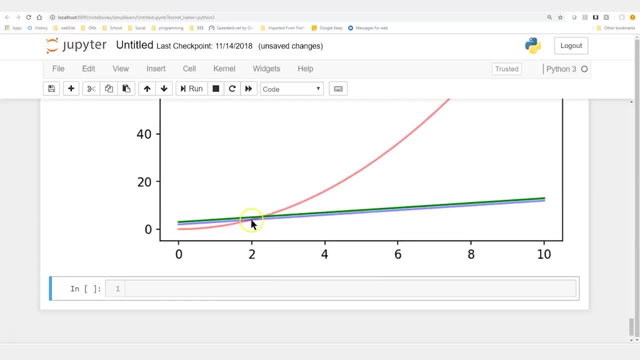 you can see how the two colors add together. You get almost a purple on there. So I can clearly see where the red crosses the blue line And then the green just blanks it over, because I didn't do any opaqueness. no alpha on there. 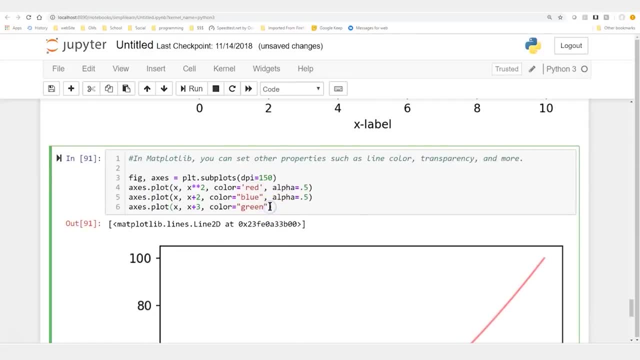 So this is great if you have lots of data that crosses over and you need to be able to track those lines better, And we'll go ahead and do this 0.5.. And we'll run that- Oops, I did equals 0.5. 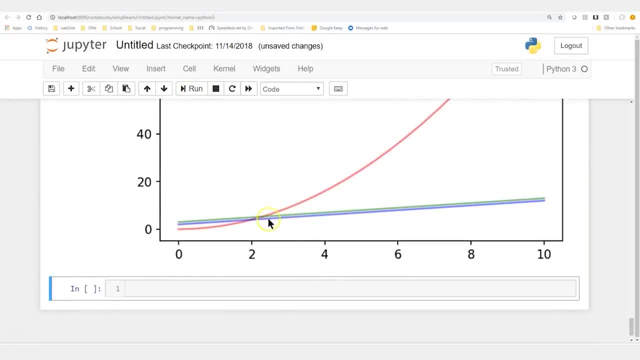 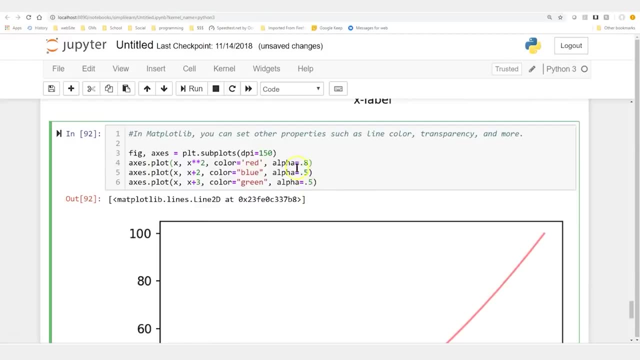 And let me go ahead and run that And so you can see right here now you can easily see the red line how it crosses the green and the blue down here, And if we want to, we can do this, as the default is 1,. 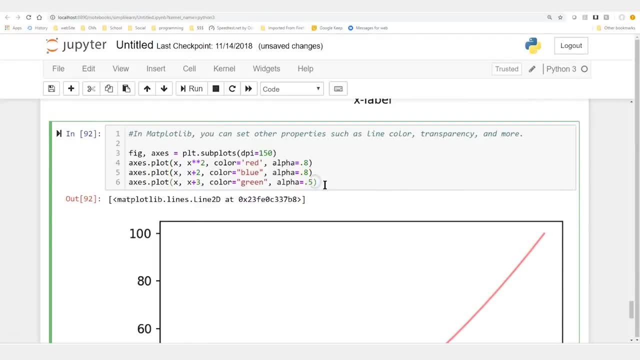 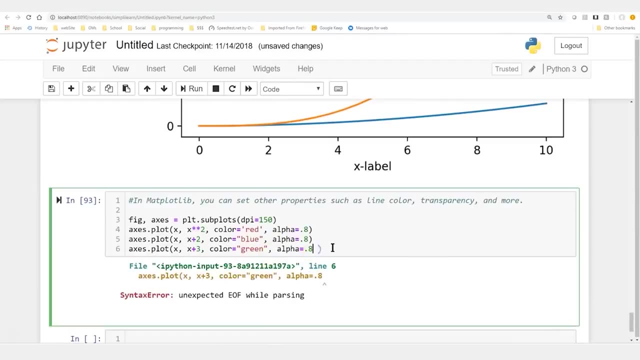 is solid, So we can change this all to 0.8.. Let me just do that. Oops 58, 8.. There we go, Run Oops. I must have hit a wrong button there. Let me try that again. 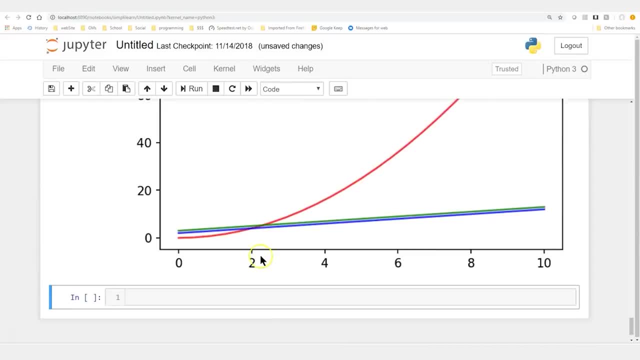 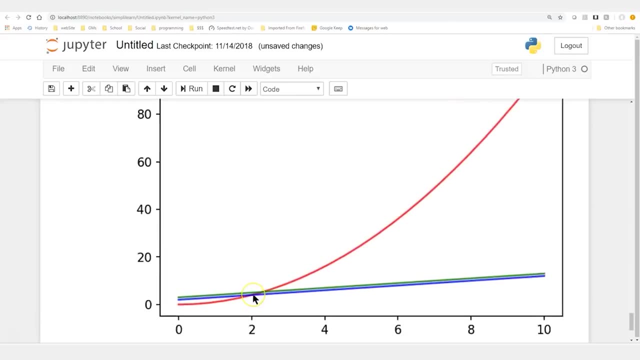 I accidentally got rid of a bracket And let's go ahead and run that And we come down here and look at this. You can still see where it passes behind them, but the green dominates and the blue dominates because we're now at 80% instead of 50%. 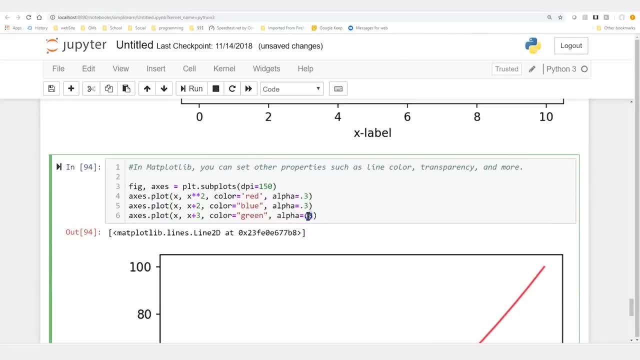 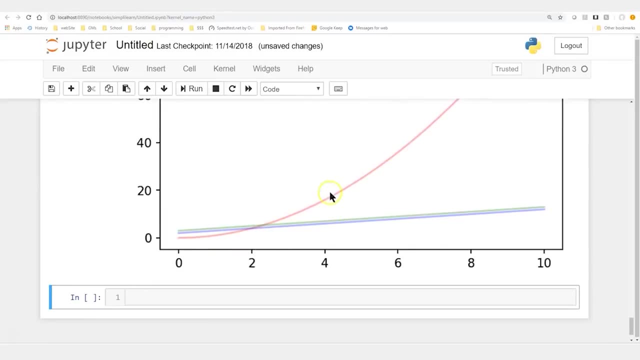 And you can do less. That's kind of fun, Although at some point the lanes kind of fade. So 0.5 is usually the best setting on there. We have a nice pastel here at 0.3, and you can easily see where they cross over. 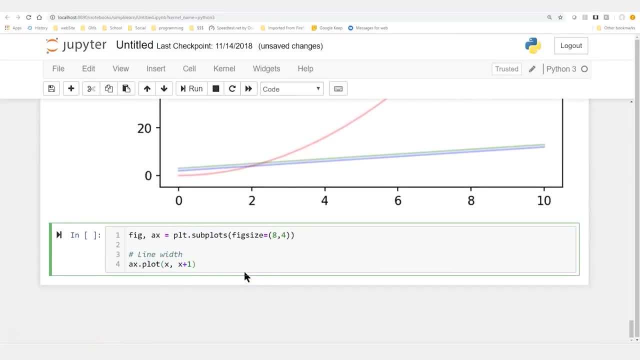 And just like you can play with the colors, we can play with line width. And let's do, let's try DPI 100 and see what that looks like on my screen Equals 100.. And we'll go ahead and just take our AX plot. 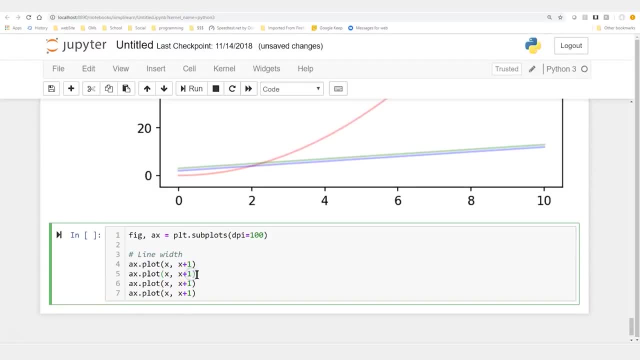 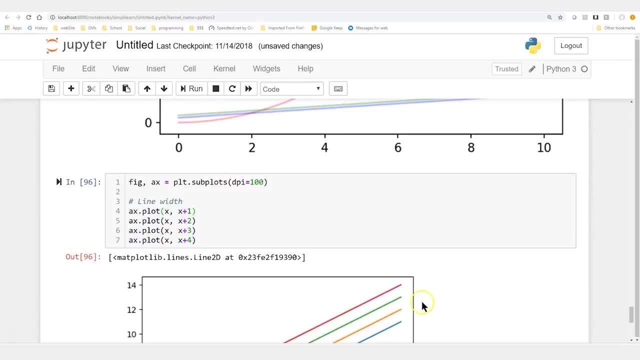 Let's do four of these lines, just so you can see how they look next to each other. Real quick here. There we go, And if I run this they should all appear the same. It automatically does different colors on there, So let's do color equals blue. 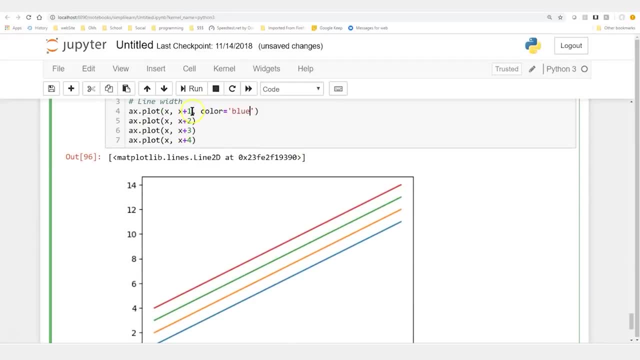 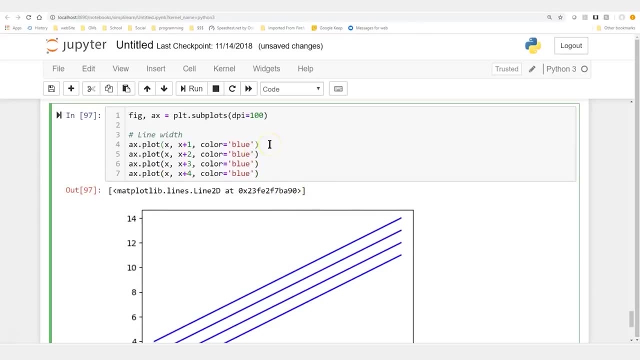 I forgot my quotation marks. There we go, And we'll go ahead and just make these all blue just for purposes of being nice and uniform, And then what I want to do is I want to do the line width. Line width equals 0.25.. 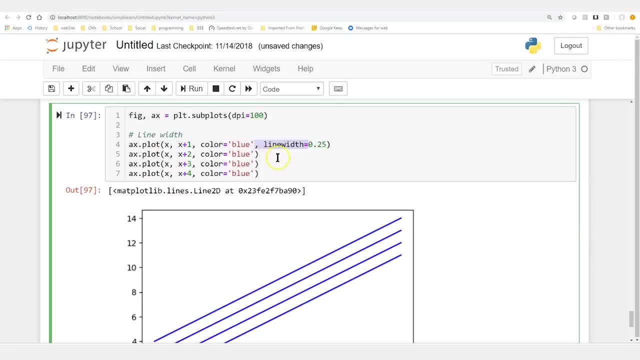 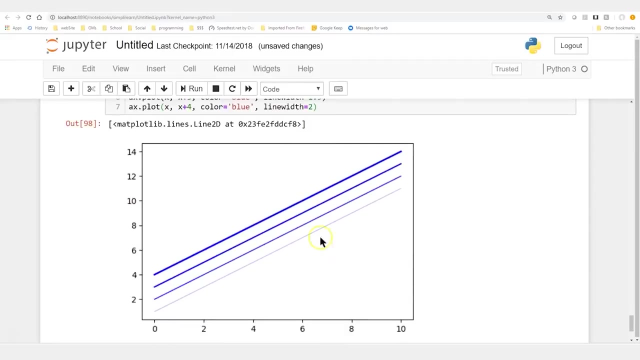 And let's just copy and paste that down here. Let's do equals 1.. About 1.5.. And let's do 1, just make this equal to 2.. Let's see what that looks like. Now we do that. you can see it goes from a very thin line. 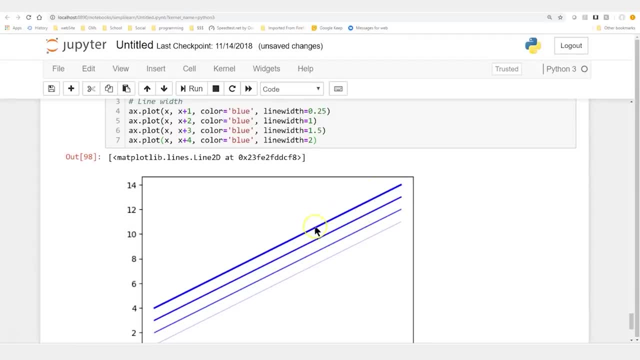 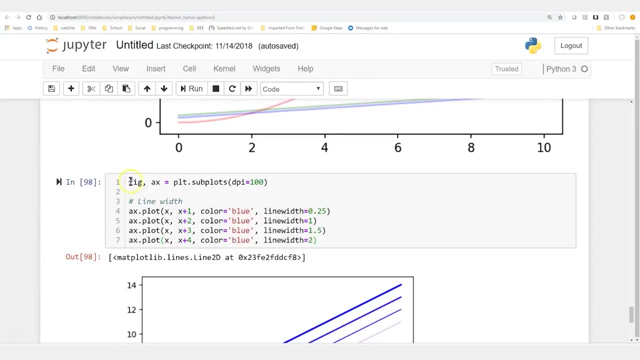 a 0.5, a 1, our 1.5 and 2, which is twice the width of the 1.. And if we're going to do different sizes, we had different colors, we had our alpha scheme. Let's take this whole thing here. 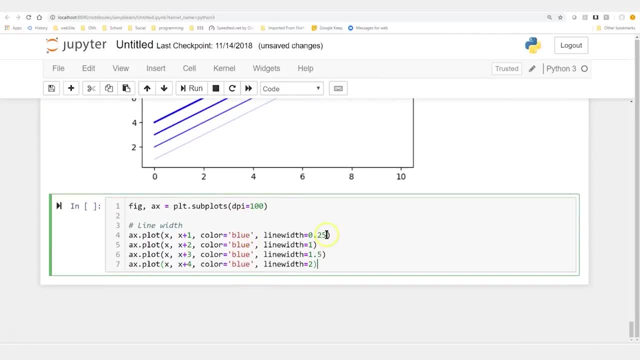 Let's paste it down here and do another one. But instead of line width, let's look at styles. Something to note here: you can actually abbreviate this with LW, So line width can also be. let's just do everything: 0.2.. 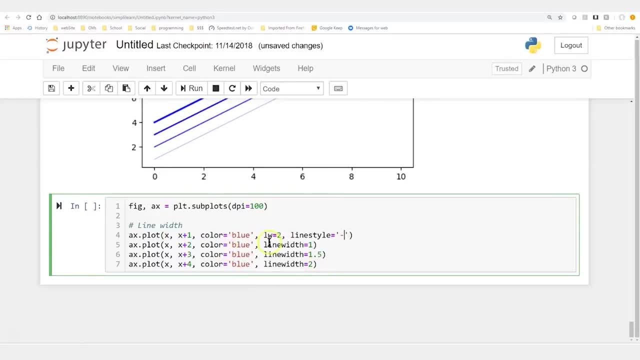 And let's set up a line style. We'll do the first one dashes, And let me just paste that down here, So I'm not doing a lot of extra typing. There we go, Take this out, So we have our dashed. 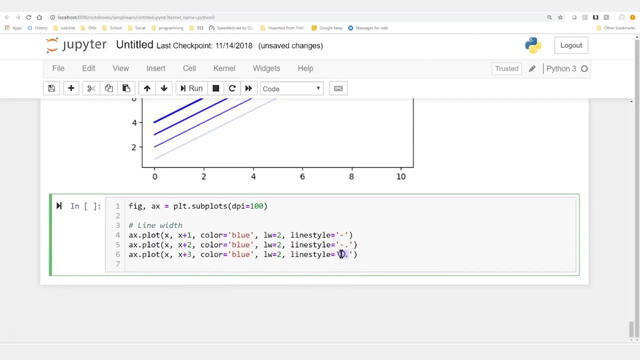 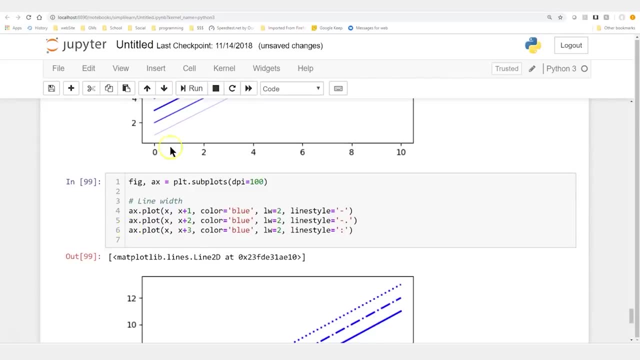 We can do a dashed dot. We'll just do the dashed dot here And a colon here. There we go, And there's a lot of different options. We'll look at a few more as we go down for different ways of highlighting data. 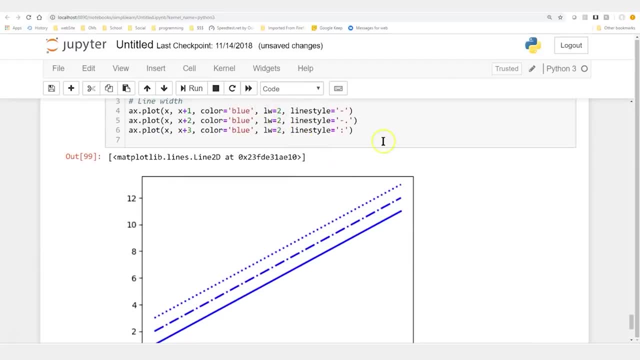 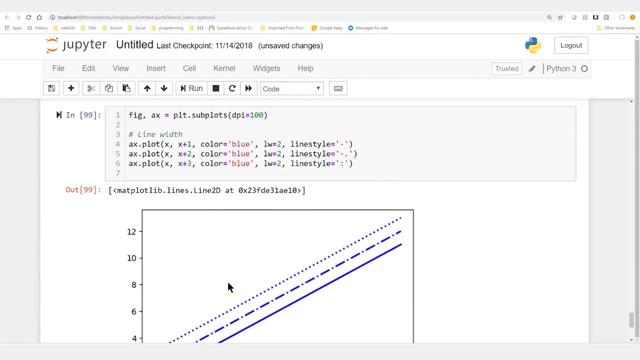 But when you look at this, we have everything as a line width of 2.. And now we have a straight line. We have a dash line or a dot dash And a dot, dot dot line. And then another thing we can add on here is we're going to do: 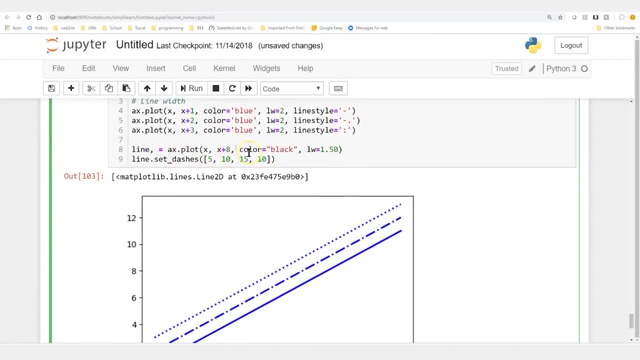 here's our ax plot: And we did x, Let's do x plus 4.. So it goes right on the top. Then do color black line width 1.5.. So it's a smaller line And we're going to take the line and we're going to set dashes. 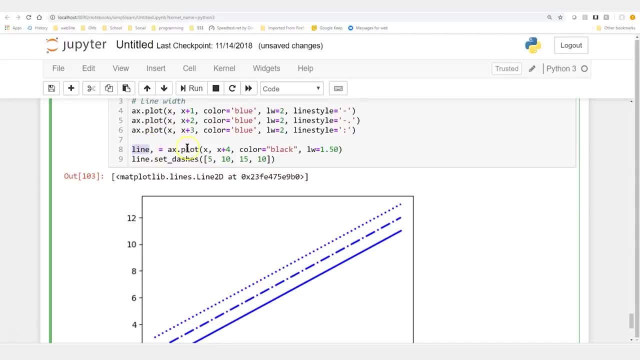 So look how I've changed some of the notation here for my line and my dash. I can set my ax plot, So I can set my line comma equal to ax plot, And then I can change the line settings this way, And when I run this, 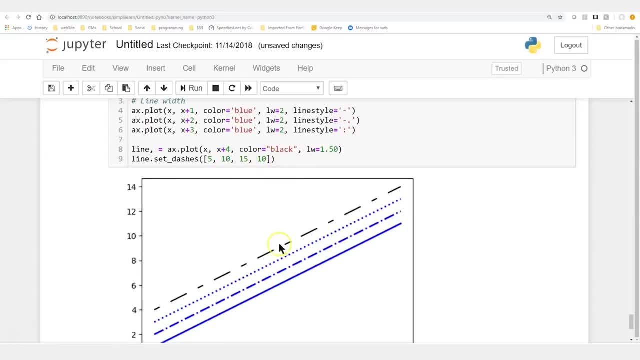 let me run that on here. you'll see. the 5,, 10,, 15,, 10 creates a series of dashes that are varied in length. In this case, they alternate between a short dash and a long dash, And we can play with these numbers. 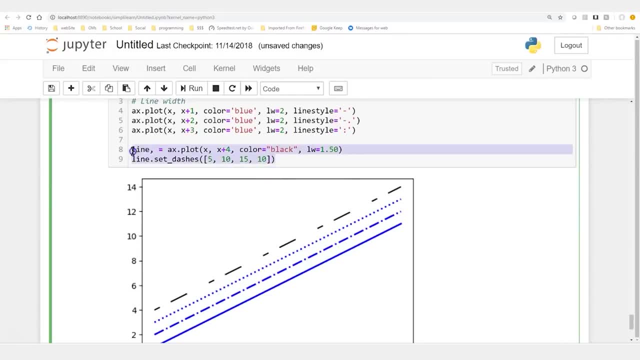 Curiosity always has me. What happens when you play with the numbers Just to see what they look like? let's do this. Let's paste this down here. I'll do two of these, just because they're kind of fun to play with. 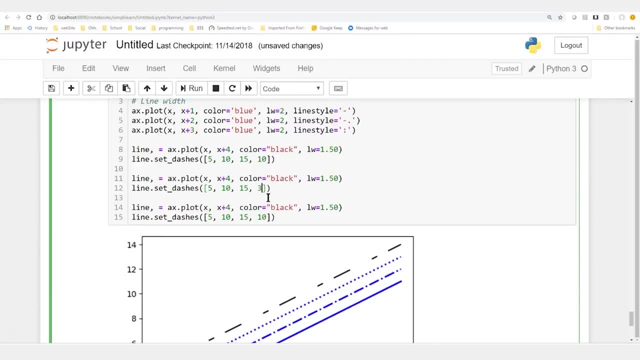 And let's change this from 10 to 3.. And we're going to change this one from 15 to 4.. And let's run that And you can see the differences in the lines. Oops, a little bit confusing on there. 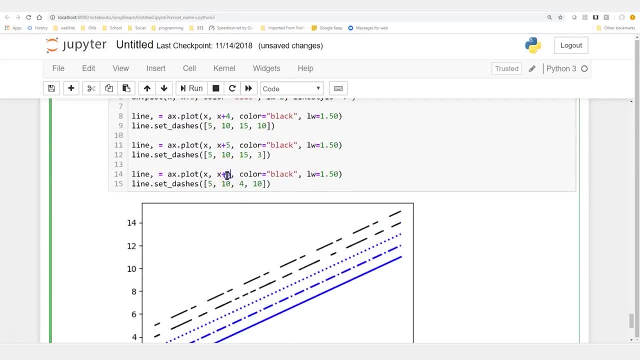 because I forgot to change the lines are all on top of each other, So let me change that really quick here And let's run that. And now you can see here's our original dash line alternating. But when I change these numbers on the second one, 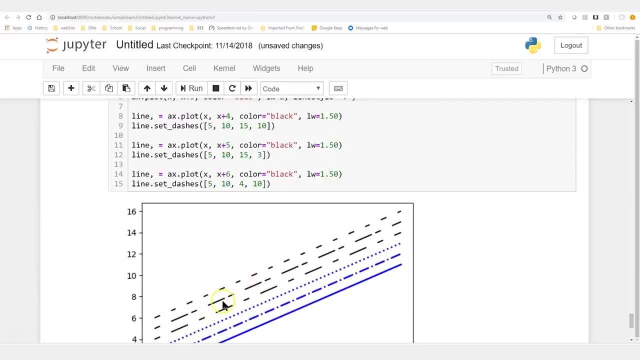 the very end value to 3, you can see. now we have the dashes of 5.. Let's see. I'm going to guess this is the dashes of 5. Skip 10.. Dashes of 15. Skip 3.. 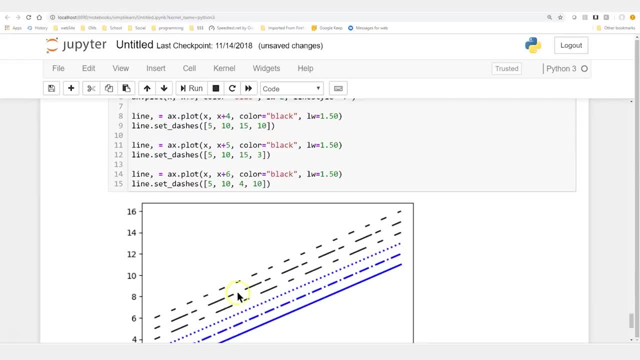 And then it goes back to the beginning. Dashes: 5 dashes Skip 10.. 15 dashes: Skip 3.. And, of course, the last one. we just switched up a little bit. It looks a lot more uniform because I'm using two sets of 10.. 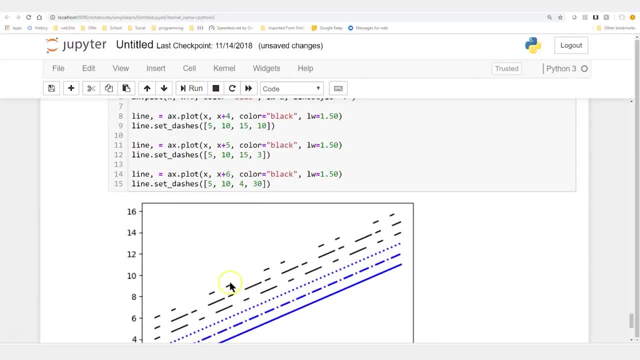 Or if I did something like this and changed it to 30, it really becomes pronounced as far as the numbers go, So distances between them, And instead of 4, let's go, let's put 30 here also 30 by 30. 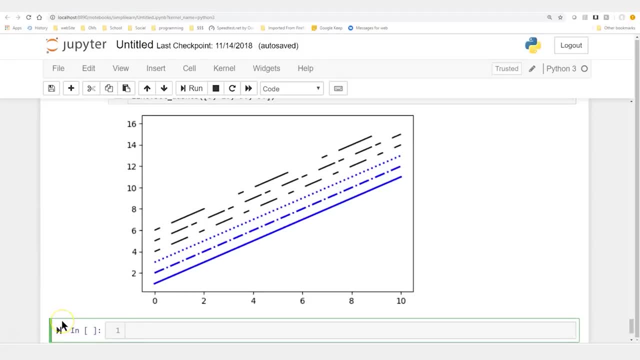 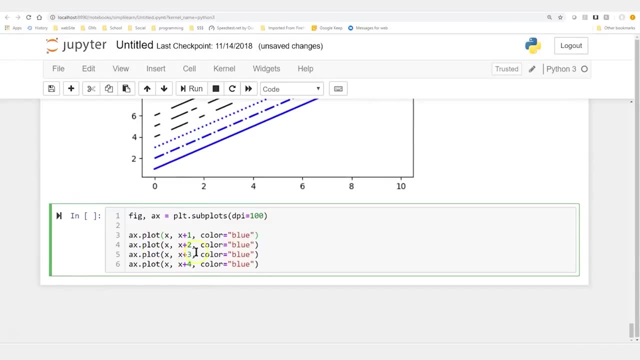 There we go, Really pronounced on that one. And let's look at one more important group for plotting our data, And in this we're going to. here's our plot. we started with with the x plus 1, x plus 2,. 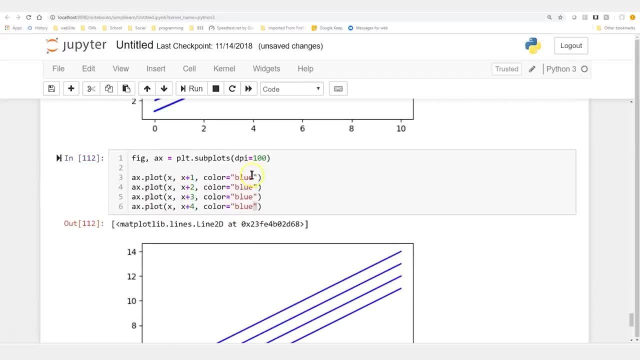 x plus 3.. And did it in blue. on this one, Three or four different blue lines And this property, we want to add the actual plots So you can see where the plots are on the graph, And for that we might have marker equals 0.. 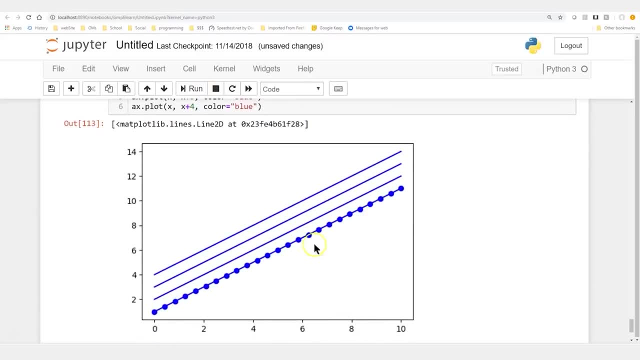 If we run this, you'll see it puts a dot for each of these And there's 25 dots because we have 25 x values, So we actually have 0, and each of the different values of x and y are then plotted here with the dots. 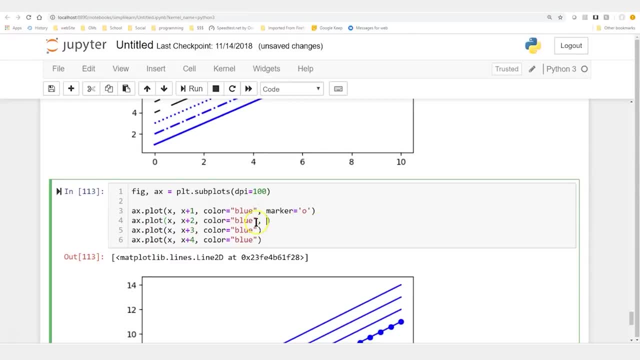 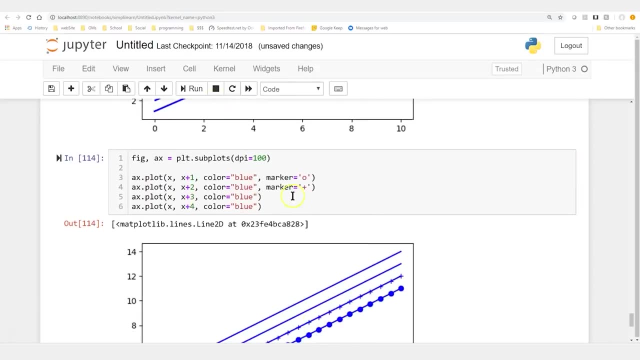 And we don't want to just limit ourselves to dots. We can also do plus sign. That's another option. Dots is most common. I actually like the dots the best. If we do the plus sign, you can see it puts a nice cross here. 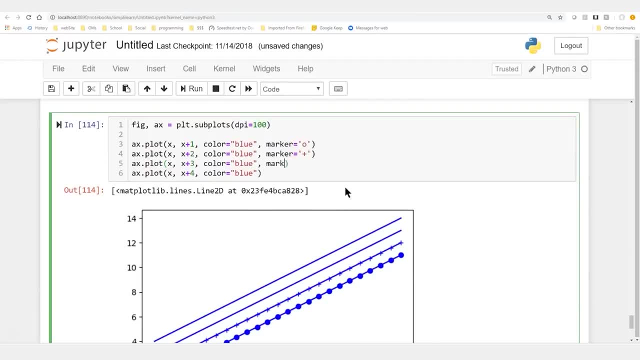 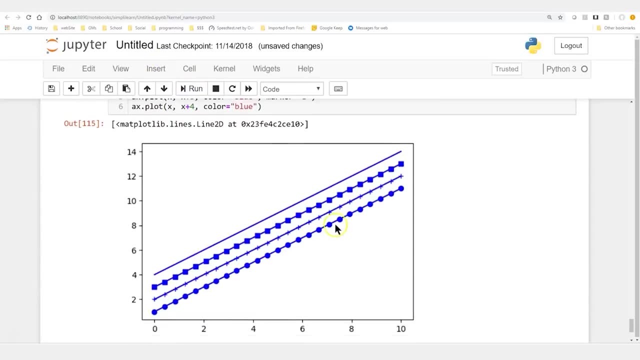 There's our plus sign on there And we can do a marker. There's a number of different markers you can use And I think this one was it. S is another one, which is a nice square And that's actually a good one. 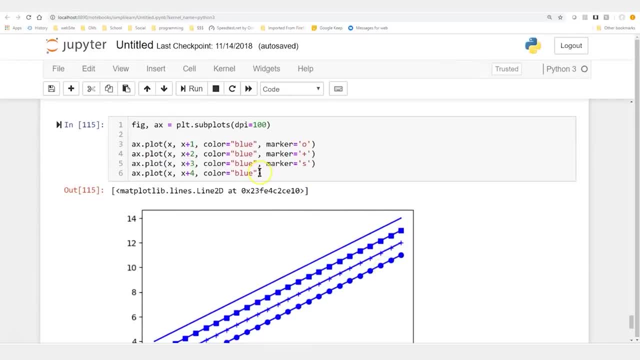 S for square O for period. Okay, that's just kind of weird. So you can see that probably on these markers. another one is number 1. So if you run that, you'll see we now have these little hatch marks. 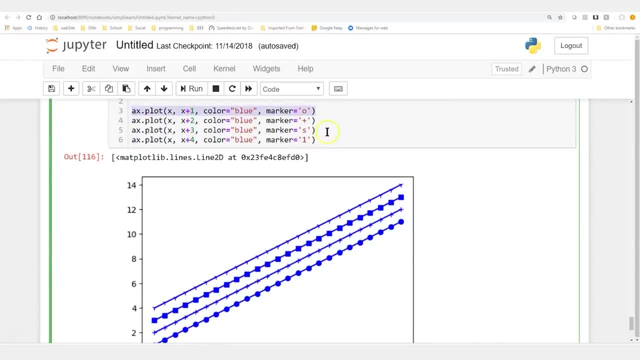 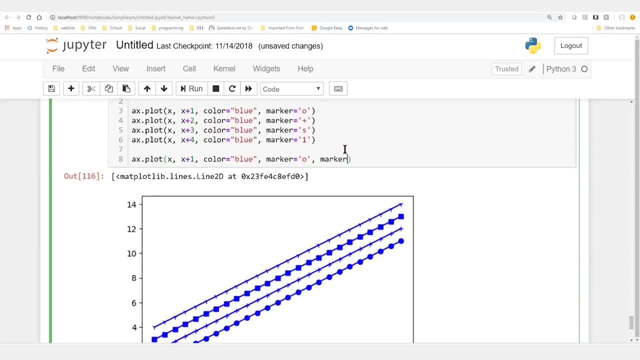 And let's take- oh, let's just go with the O on this one. By the way, this works with square really nicely. Some of the stuff we're going to do here on just a second Let's do: marker size equals 2.. 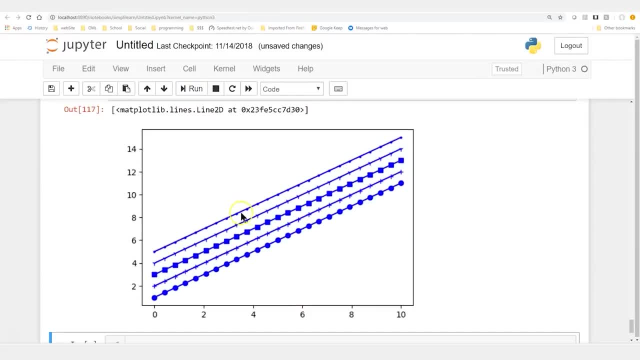 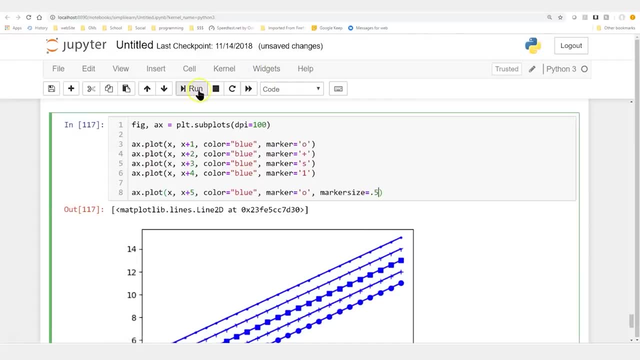 And change that to 5 and run that And you can see here it puts a nice little tiny dot versus this size dot here, And this is interesting because it said 2.. I thought it would be bigger, But if you do .5,. 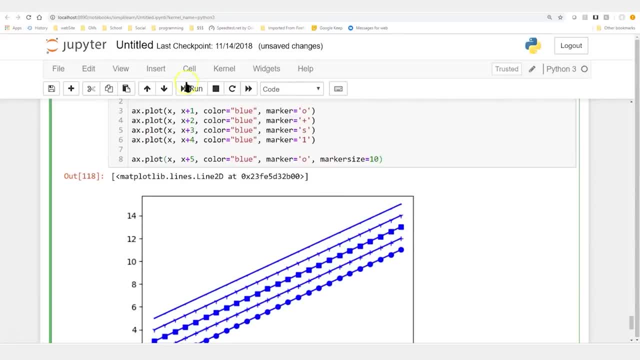 it gets even smaller. And let's just do 10 to see what that looks like. Run: That looks huge. So marker size: A lot of these are dependent on the DPI in the setup, So there's things that switch around As far as the way the size shows up. 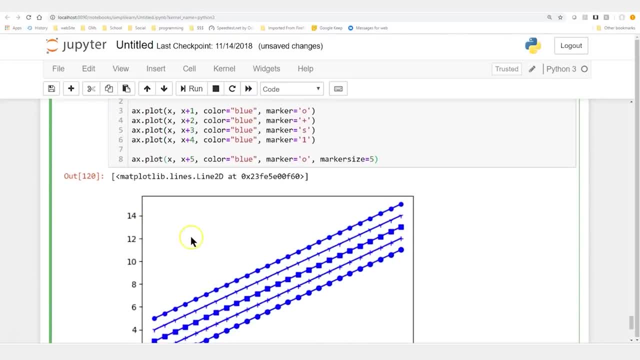 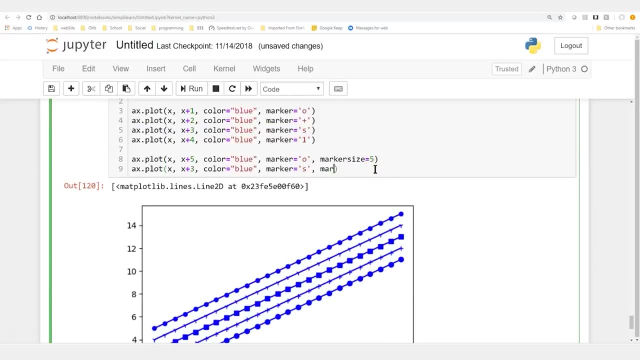 You've got to be a little careful. when you change one setting, it can change all the other markers. And then let's take our square on here And we'll do. we have marker size. We also have marker face. We'll set that equal to red. 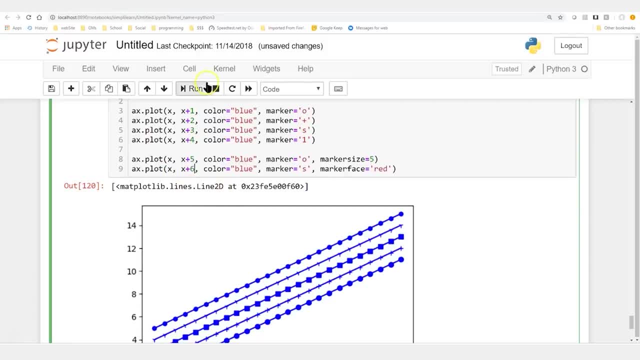 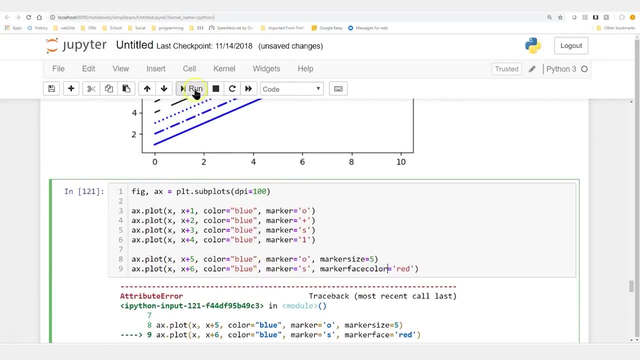 Of course we may change the, so it's up one notch. We'll run that. Whoops must have mistyped something on here And I did It's marker. face color equals red, And so when I run that you can now see I have the squares on here. 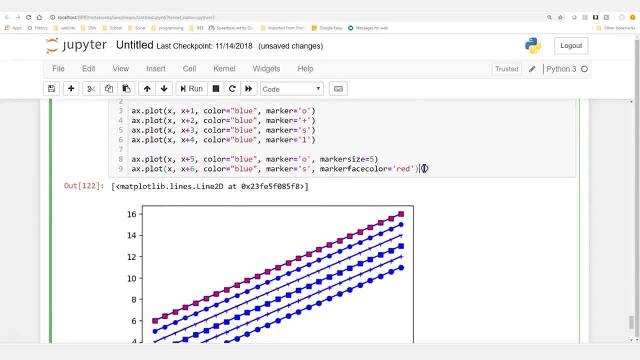 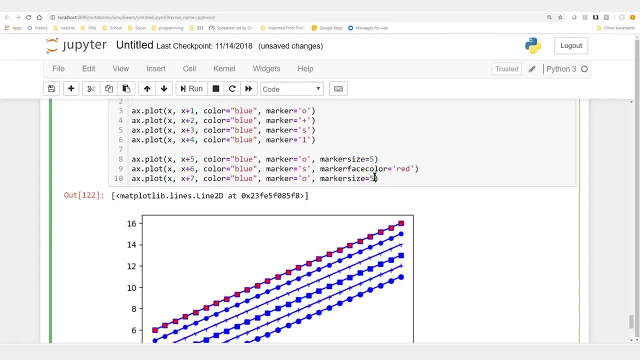 With the marker face color. Of course, we can mix and match these. Come down here and we'll make this instead of let's make this plus seven And we'll make this size 15.. Marker face color. equals And we'll do what. 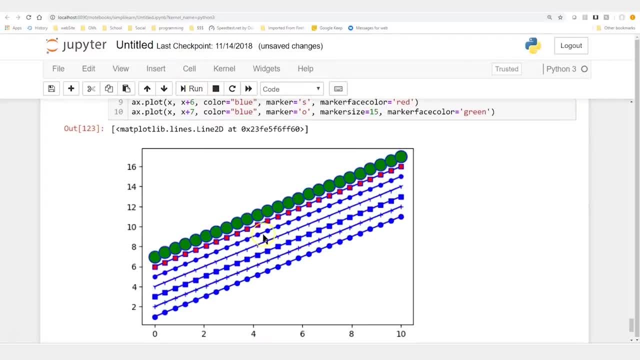 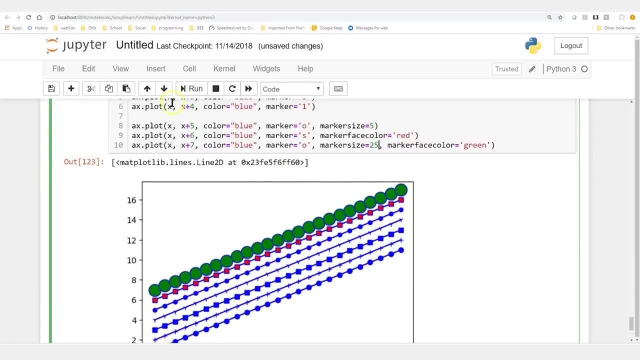 Green. Just because There we go, Run Very hard to actually see what's going on there. Still 25 dots. They kind of overlap, As you can see. they print them over each other And, of course, if we really wanted to make it look horrible, 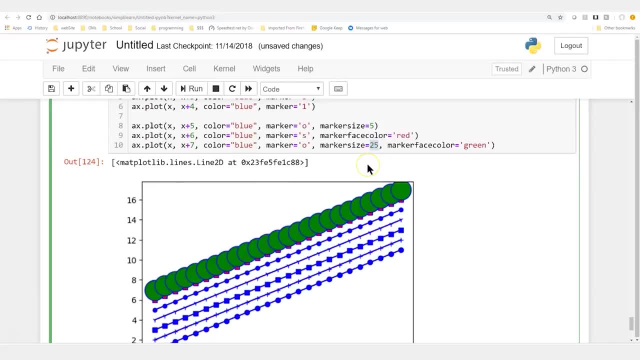 we could just make that really huge. Generally, though, you'd want something a little bit smaller and cuter. We'll just try doing it this way. There we go. That's too small to even see the face. So four: You can start to see the face on there around four. 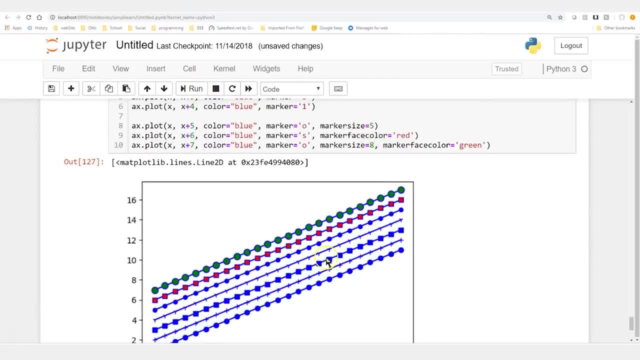 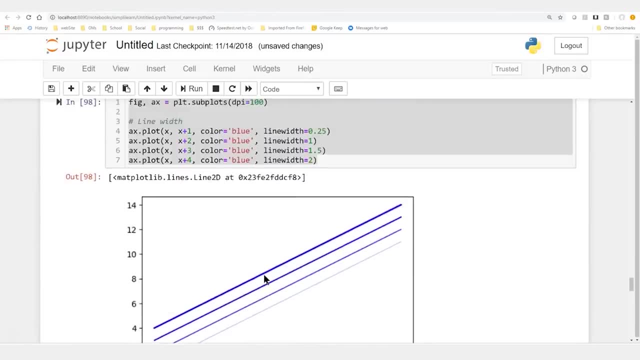 Maybe an eight. Eight might be a good number for this. There we go. Eight Again. that all just depends on what you're trying to show and display. So we've covered a lot of stuff here As far as our lines. 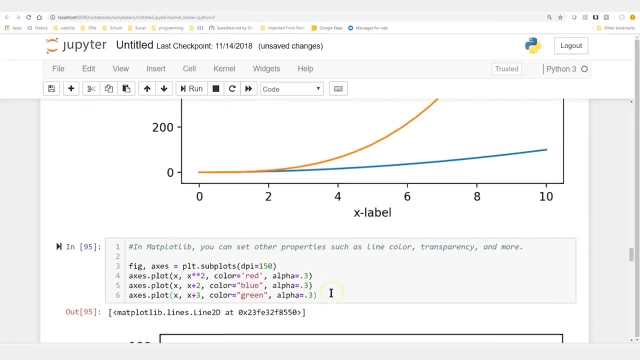 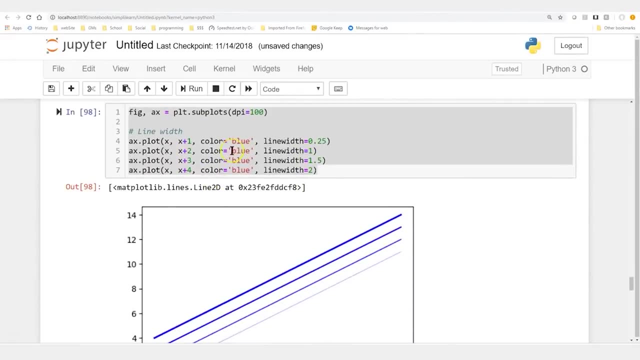 we've covered opaque with our alpha setting on there. Okay, Let's give it some nice pastels. You can see how they overlap and how they cross over. We covered the line width, different size on there, different formats for the line itself. 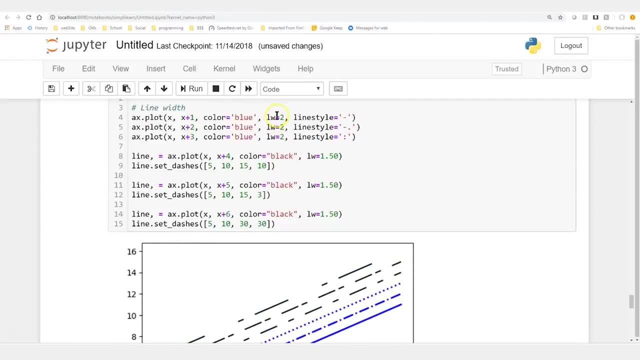 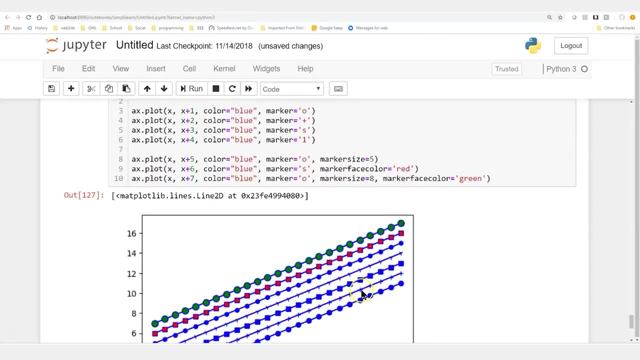 And these are all. you can combine all these So you can have: our line width equals two, line style equals dash. You can bring this down here. also to the markers. And then we added markers in Just standard, a circle, a plus sign. 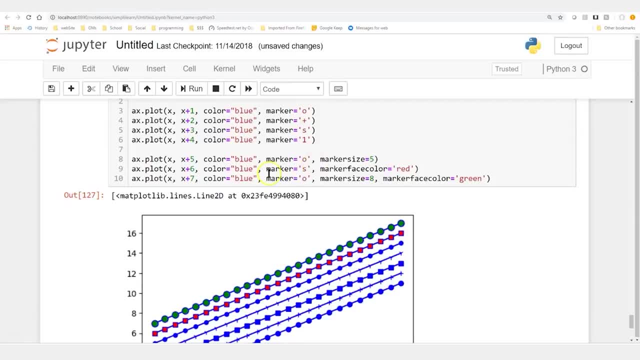 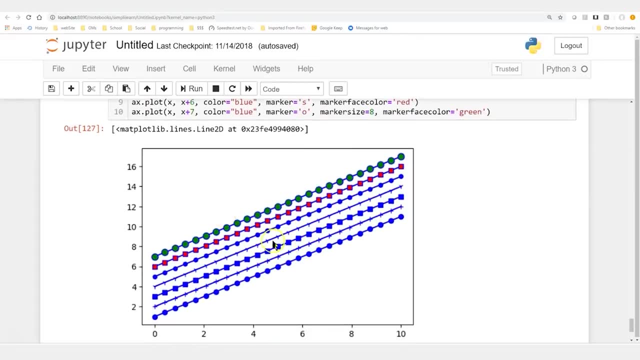 the square a little tick which uses a one. Then we add a marker size and a marker color face And we combine those. You see different series of representations And we also briefly mentioned color where you didn't have to use. 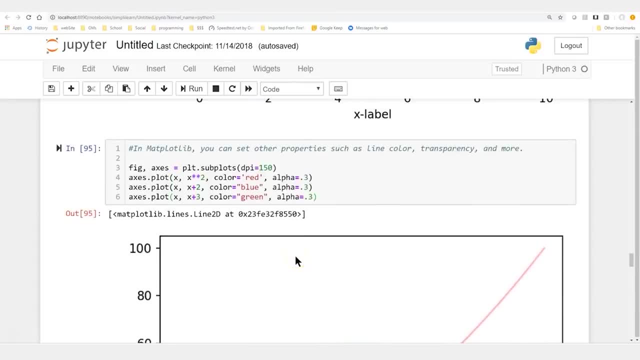 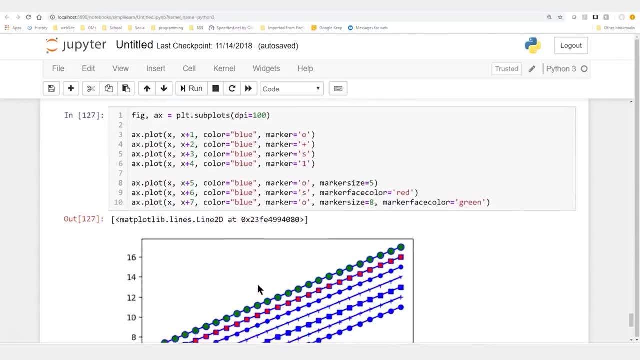 Like in here, we used color black. Someplace up here you'd have to find it. We used the actual number for the color as opposed to. I changed it to red and blue So you can get very precise on the color. 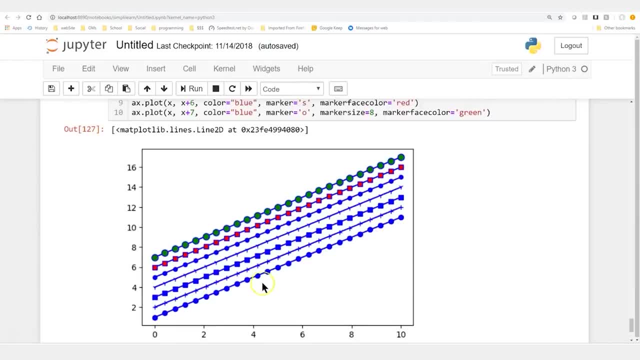 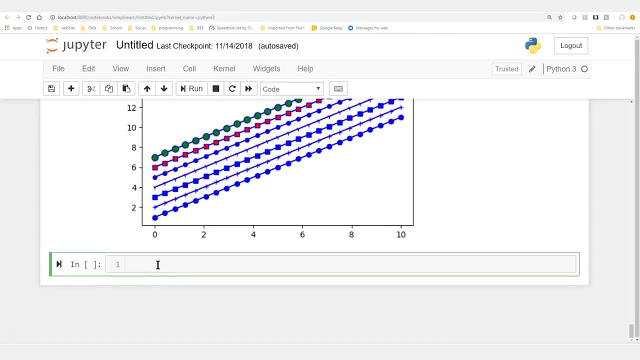 If you have a very specific color set that you need to match your website or whatever you're working on. All of those are tools in the Matplot library, So we have one more piece to formatting the graph, So we want to show you. 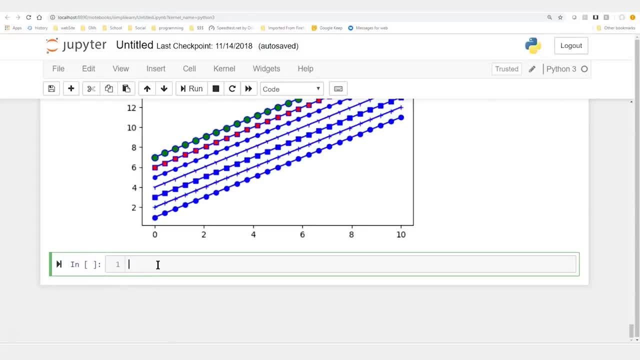 And then we have two big sections. We're going to go over the different graphs that they have, along with a challenge problem. So let's go to the last section we're going to look at is limits. We're going to limit our data. 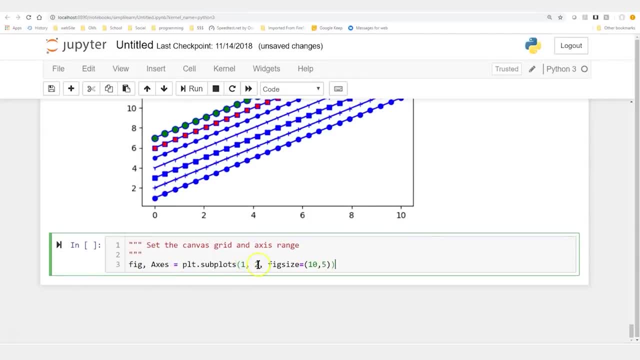 So this first part I'm just going to paste in there. We're going to create our subplots: one, two, So one row, two columns. We're going to do a figure size of 10,5.. This should all look familiar now. 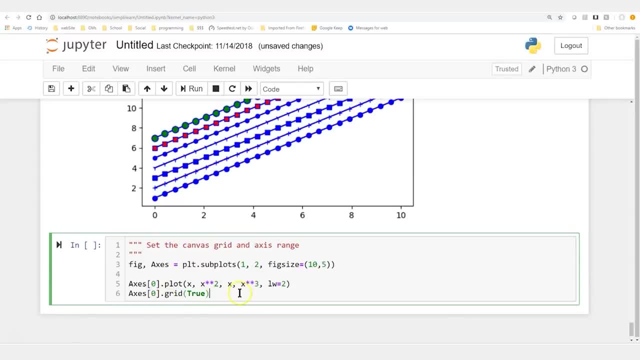 since we've done a number of them And we're going to go ahead and plot- And this is an interesting notation you should notice here- Our axis is zero, So one we've used instead of you can just iterate through them. 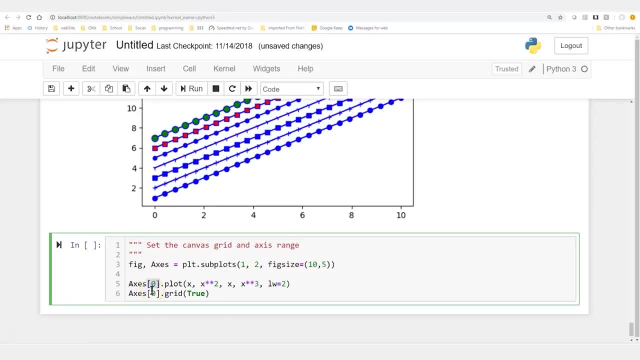 but they're just an array, So it's an array of zero. It's still the axis of the first axis out of two. And we're going to plot x, x squared, x, x cubed, line width two. So we're going to go ahead and just plot two graphs right on top of each other. 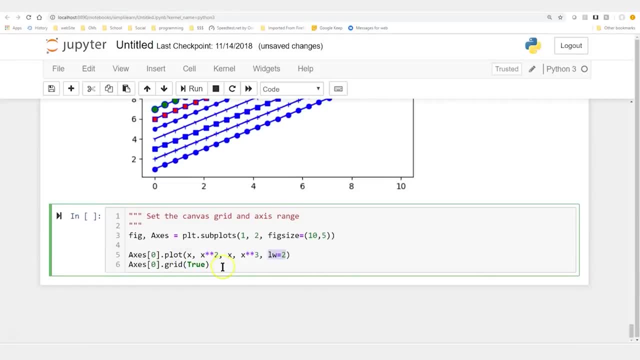 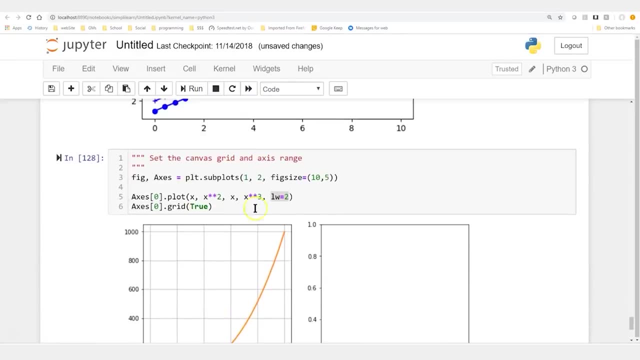 without doing multiple plots on here, And we'll set the grid equal to true on here. Let's go ahead and run that And you can see here our two plots with the x value going across, And I'm going to do something similar. 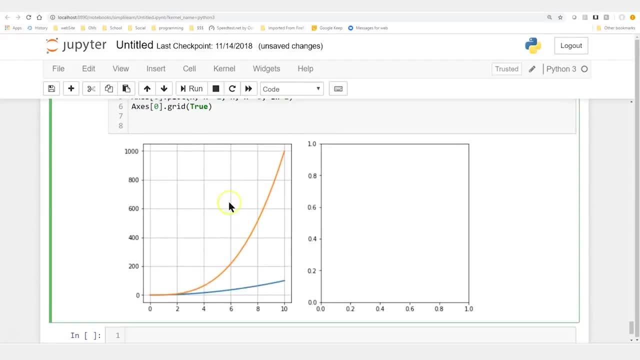 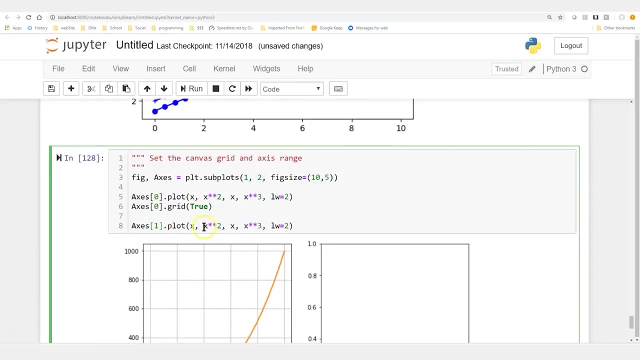 and, by the way, if you look at it, you can see the grid on there. That's all. that is Easier to spot the data going across. We're going to take the same data for axis one, So we have our plot of x. 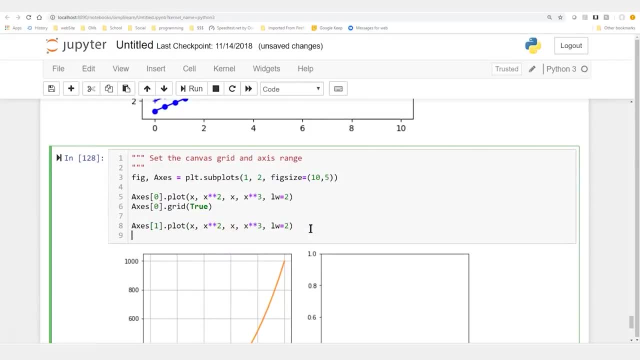 x squared x and x cubed. line width two. And this time we're going to take our axis one and do y limit. It's actually set underscore y limit. This is the y axis, So it's going to be an array of two values. 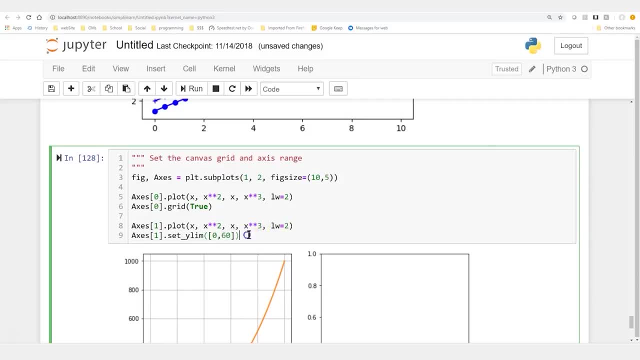 And we'll do zero comma 60.. I'm just making these numbers up. The guys in the back actually made them up. I'm just using their numbers And we're going to set the x limit. And we'll set the x limit as. 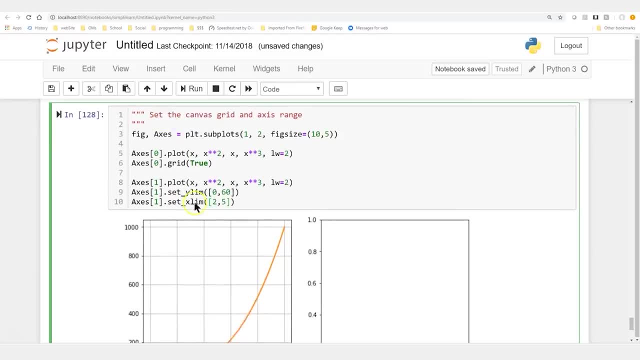 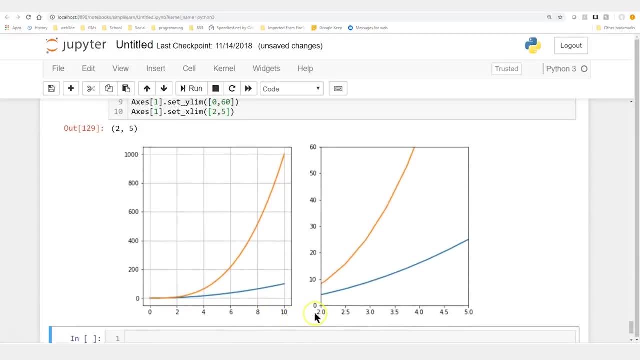 don't forget our brackets there. two comma five. So it's the same data going in, but we're setting a limit on it And let's go ahead and run that And let's see what it comes out of. And here we have the y limit zero to 60.. 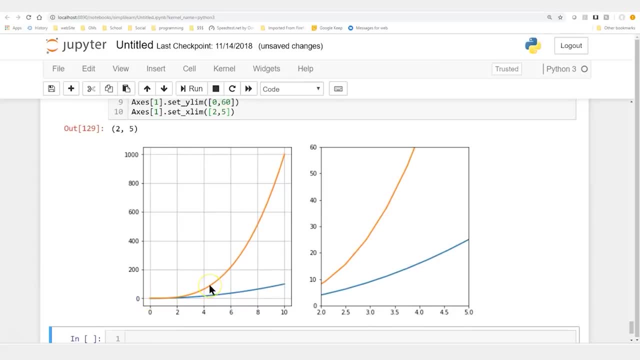 So we're looking at just the lower part of this curve here up to here And we have the x limit, two to five. So that starts right here at two, And you can see very different graphs. This is kind of nice. 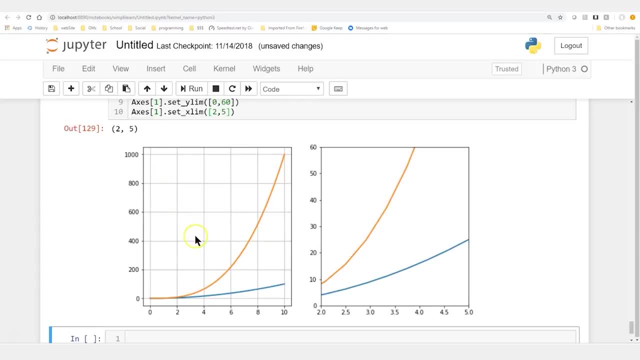 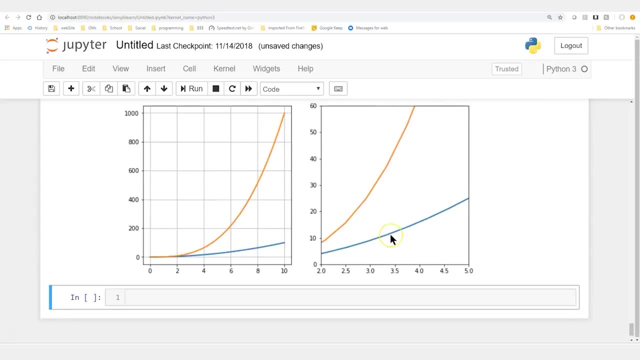 because you could actually put one of these on top of the other if you wanted to draw focus to one part of a graph. Remember how we did that earlier: one inside the other. But just a quick note: you can easily limit your graph and kind of reshape the way it looks, quite easily. 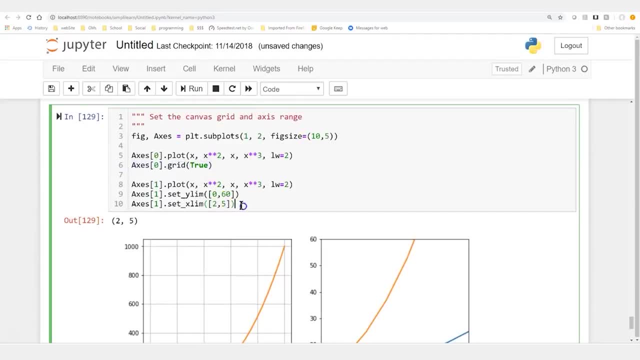 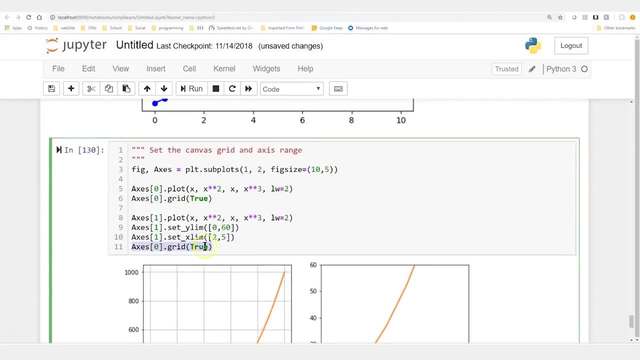 And we can also add that grid down there. if you want a grid, We'll run that and add the grid in there. Oops, I guess you have to do the grid beforehand. Switch. that. There we go. Sometimes the order on this is really important. 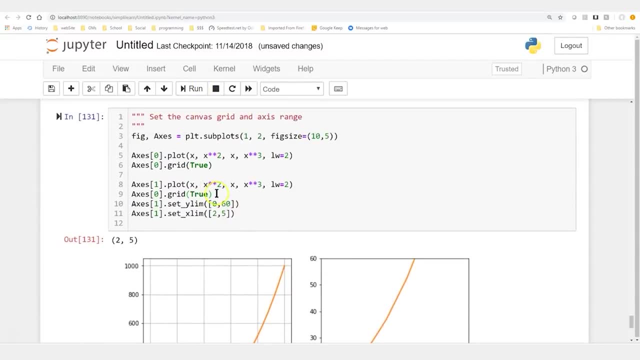 So you may double check your order when you're printing these things out. It also helps if I change it to one, So in this case it might not be the order. I wonder if we'll go back here as one. There we go. 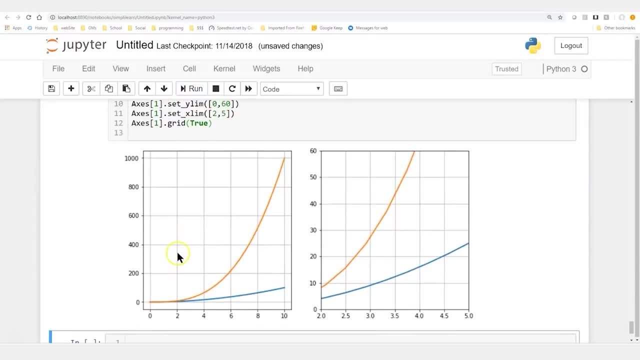 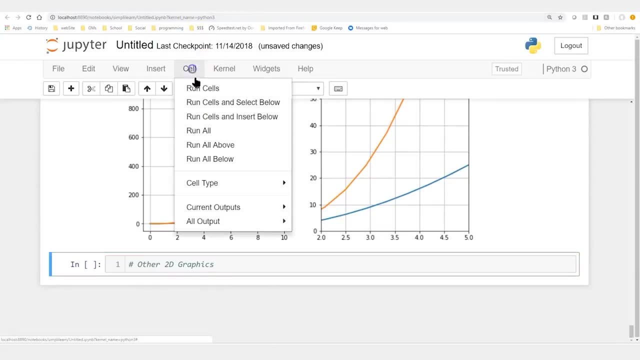 So it doesn't matter the order and grid, But you can set the grid for easy viewing here. Nice setup on there, But you can see how we can limit the data. So let's start looking at some other 2D graphs and make this cell a markdown. 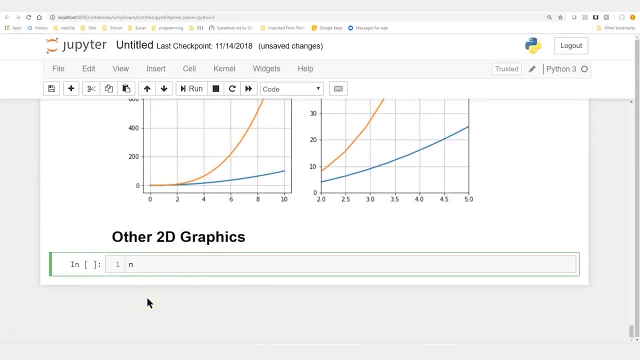 So we run it. It has a nice pretty title to it And let's go ahead and create some data with an NP array. We'll do 0 to 5 on here. There we go, And let's look at 4 common graphs. 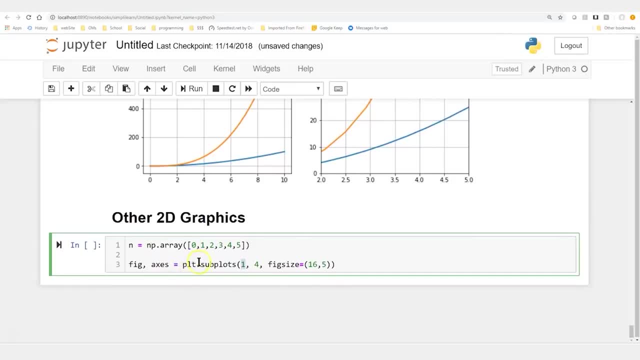 We'll put them side by side, So we'll do a figure. Our axis equals plot, subplots, 1, 4 columns and then figure size. Hopefully it'll fit nicely on here. It seems to do pretty good on here And I'll go ahead and just run that. 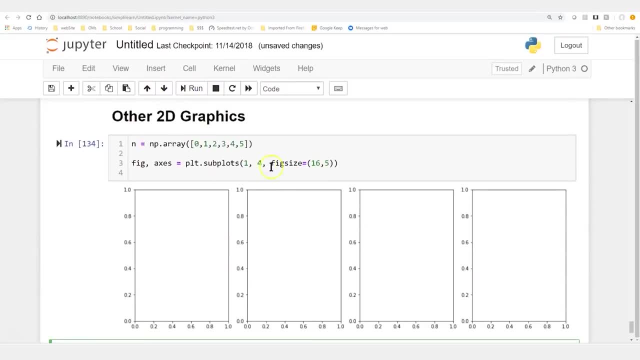 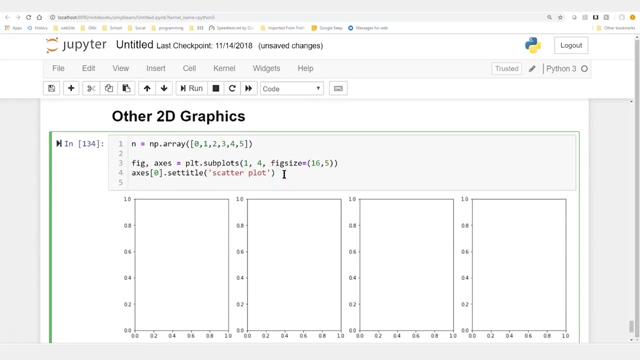 since we're in there Run. You'll see I have 4 blank plots on here And we'll start with axes of 0.. Let's set title And we want this to be a scatter plot. A scatter plot just means it has a bunch of dots on it. 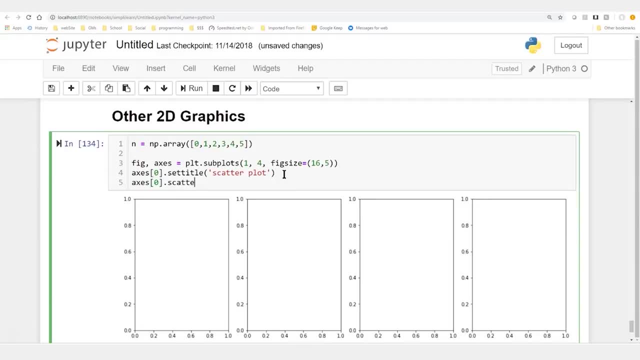 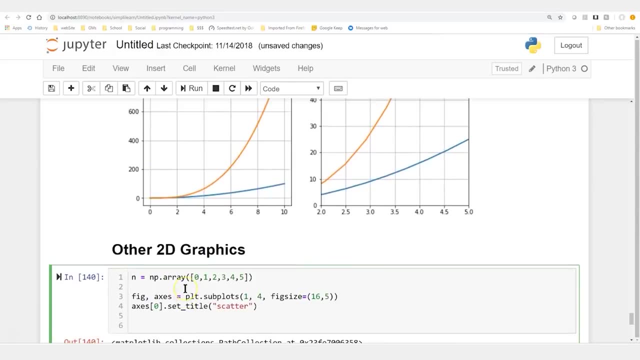 So here's our axes of 0.scatter- Easy to remember. Scatter a bunch of plots on there. We'll do our n, Or we can do x or n. There we go And let's go ahead and do axes. set title: scatter. 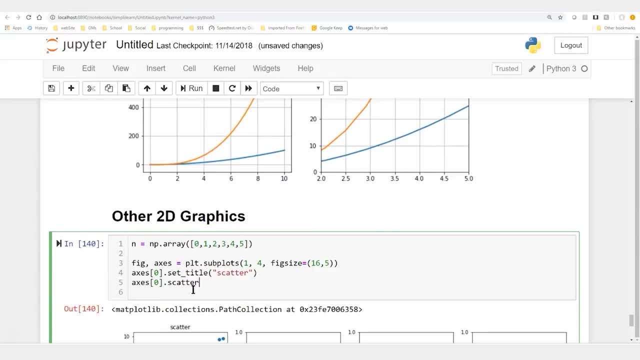 Already did that. We're just going to do scatter. That's how you do it on there. That is how you create a scatter plot, simply with the scatter control. And we'll do. let's do the variable x, x plus. Let's throw some randomness in here. 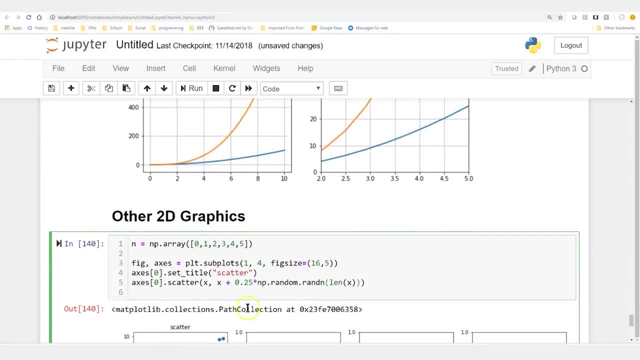 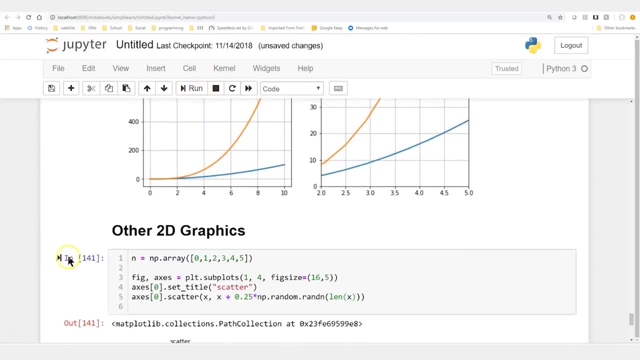 Usually scatter plots are have a lot of random numbers connected to them. That's why they do them on there, And so the bigger the x gets, the bigger the randomness. So 0.25 times the randomness And what we should end up down here. 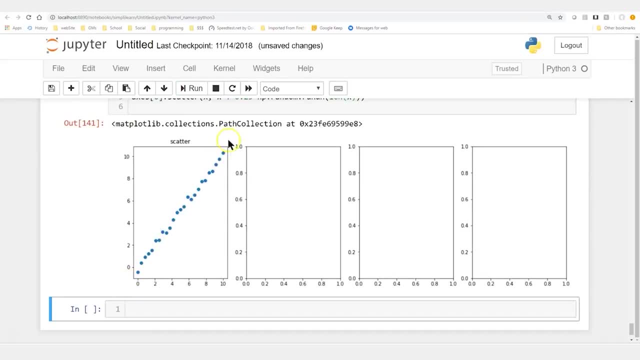 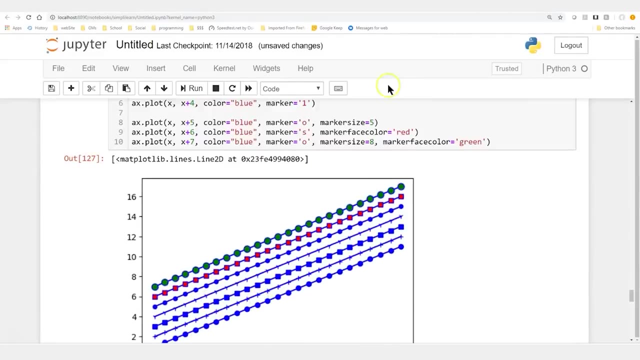 is with the scatter plot And you can see as you go up. it just kind of has some random numbers and moves up and down the line, But plot's just the points. So if you remember from back up here where we did marker, 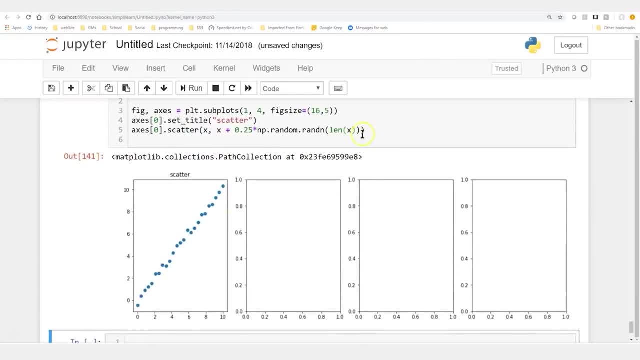 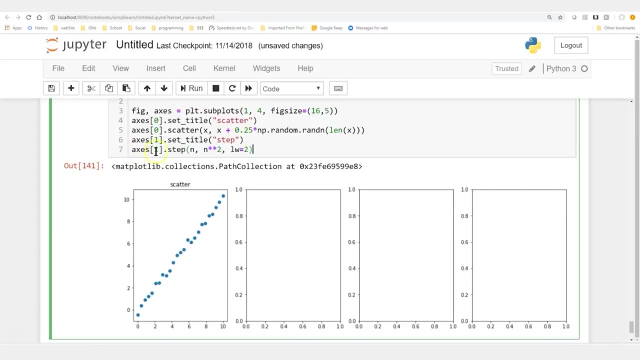 this is plotting, basically just the marker, So it's a scatter plot. Probably less used is a step plot. So for x is 1, we'll go ahead and do a step plot So you can see what that looks like, And this time we'll use our n value. 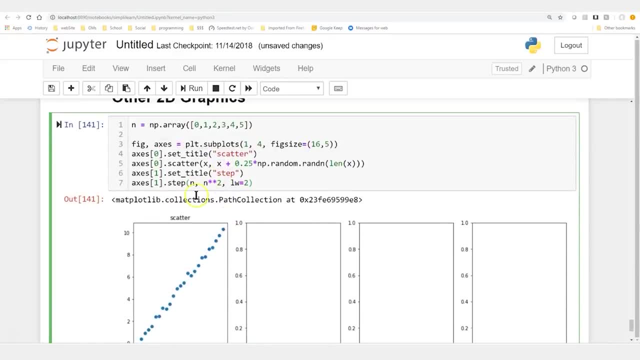 instead of x. We generated that n value up here, And so for this we have n n times 2, our n squared n times 2, n squared Line width equals 2.. And if we run that it creates a nice step up. 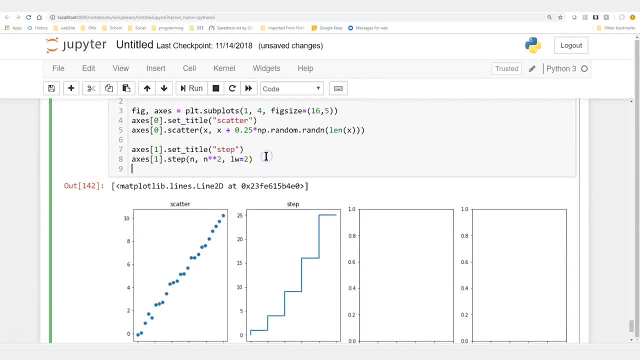 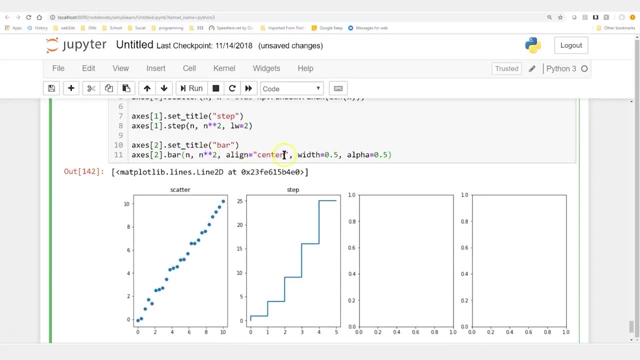 Let's see. So we've got a scatter plot, We've got a step plot, Let's do a bar plot And we'll use the same formula- n, n, squared alignment centered, Because you can have them left or right. 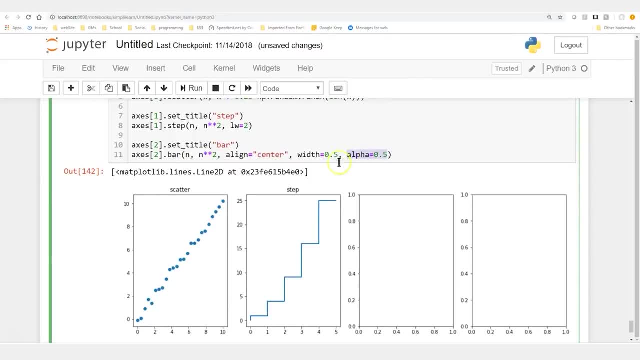 Width 0.5 and alpha, If you remember correctly. that's how opaque it is. Let's see what that looks like on there. So we have some nice- you can see here a nice bar plot. It should look very similar to the step plot. 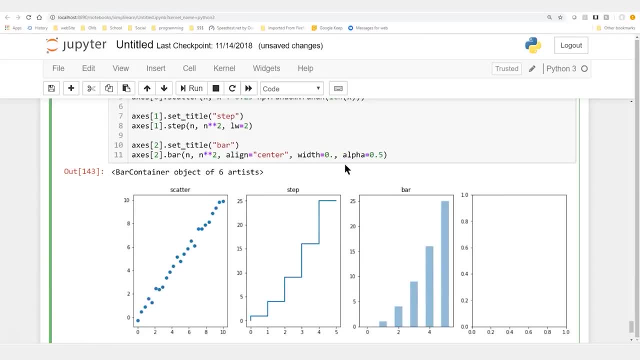 but colored in And we can change the width. Let's see what happens when we do 0.9. Run And if we take width out completely, run that You can see it starts coming together on there And we can change the alpha. 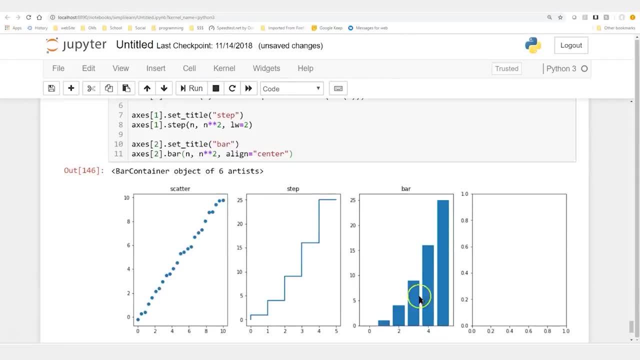 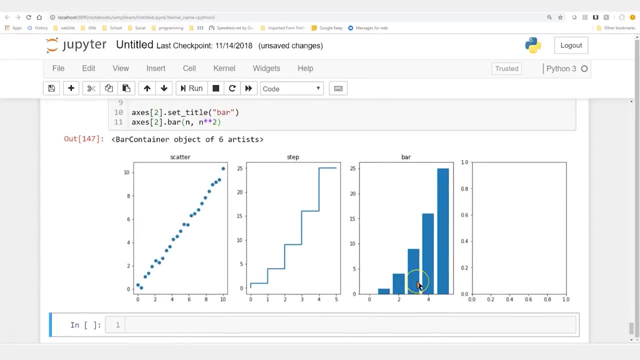 We can take the alpha out too And run that. See, now you have the solid colors, And if we take out the center and run that everything, you really can't see the shift on here, because that's actually the default on this. 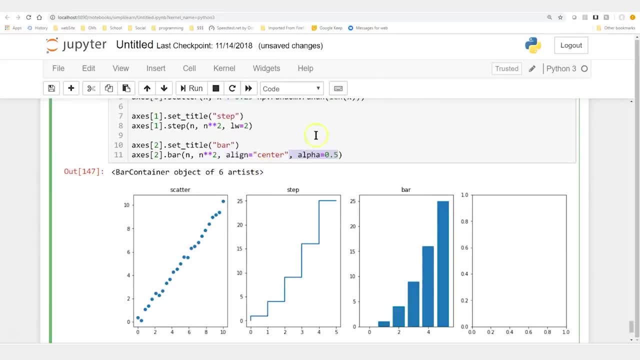 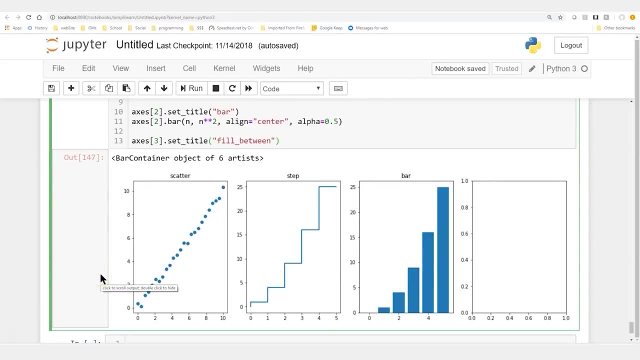 But these are common settings for the bar graph. Let me just put it back in there. There we go: Alignment, center and alpha. Now I can't say I've used the step graph very much. There are certain, I guess. 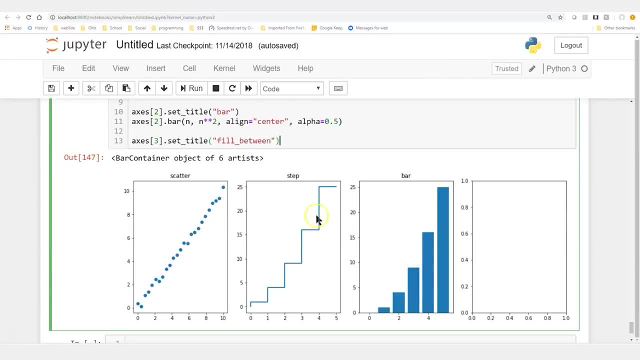 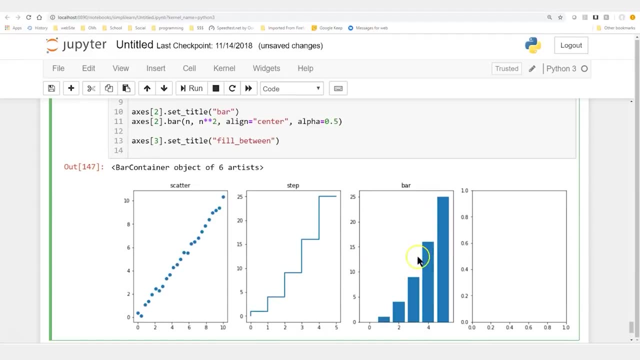 domains of expertise that require a step graph, But the scatter plot and the bar graph very common, Especially the bar graph, and we'll look at histograms here in just a minute. So I use histograms a lot, Especially in data science, But this is nice if you have very concrete objects. 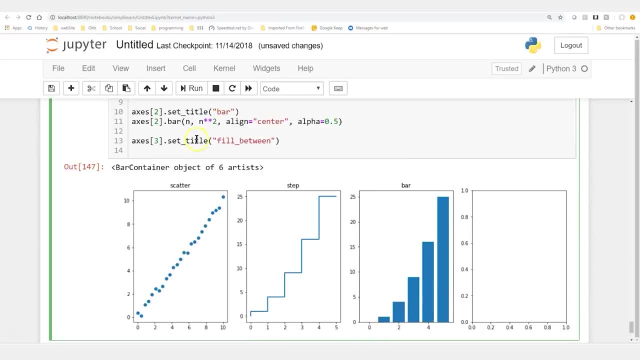 How many people are wearing yellow hats, That kind of thing. But if we're going to do that, let's go ahead and do the last one, which I see a lot more in the sciences. I'm certainly using the data science, but more 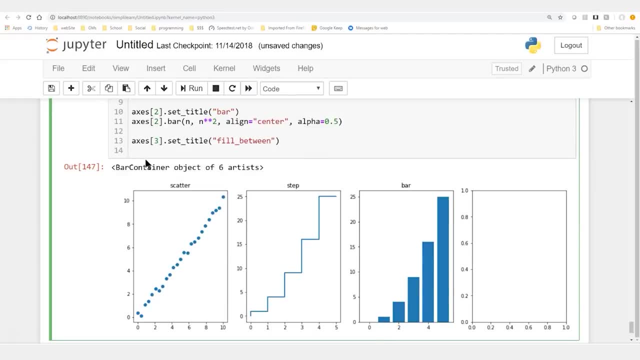 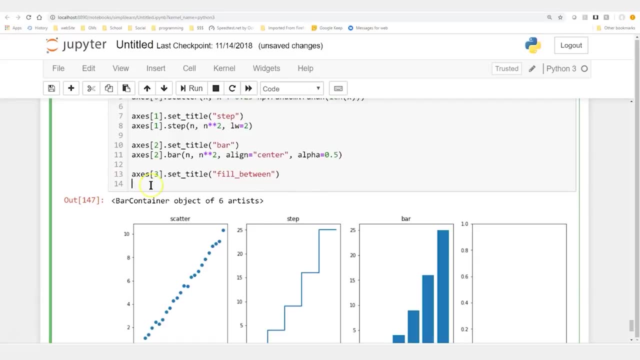 like for mapping. I saw a publication on solar flares And they were discussing the energy, And so filling in the graph gives it a very different look. So we're going to do the fill between, And it's just like you think it would be. 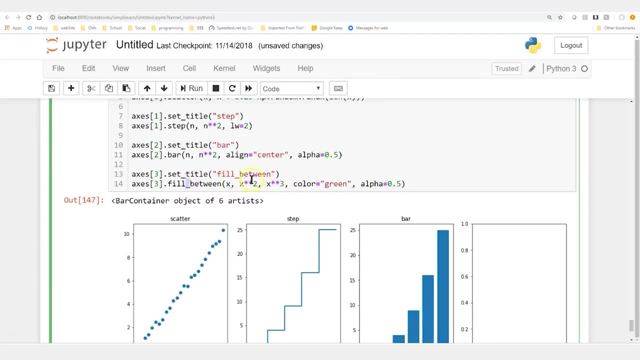 It's fill between, but with a underscore between them, And we'll do x and x squared and x and x cubed, And we'll do color green and alpha again, Just in case you had other data you wanted to plot on there. 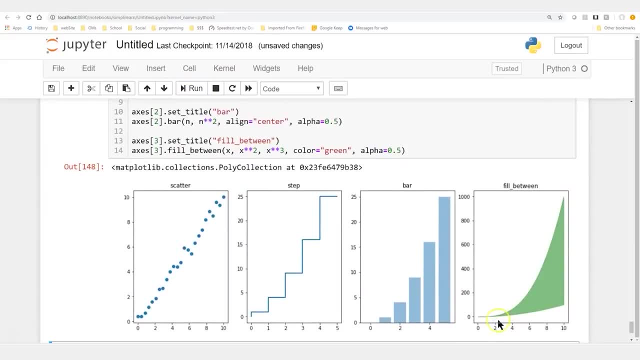 You can see it forms a nice squared coming up here. And also if you look at the, the bottom one is your squared value, The upper line is your cubed value And then it fills in everything in between. If you remember from calculus, 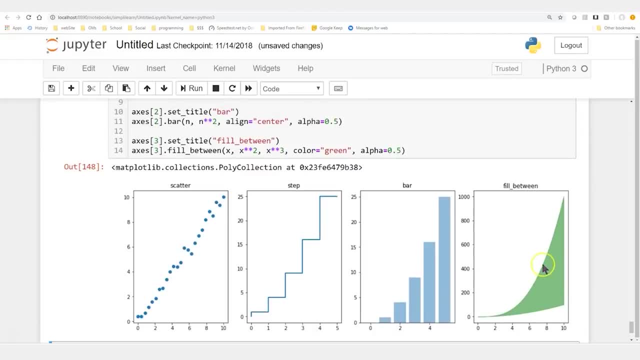 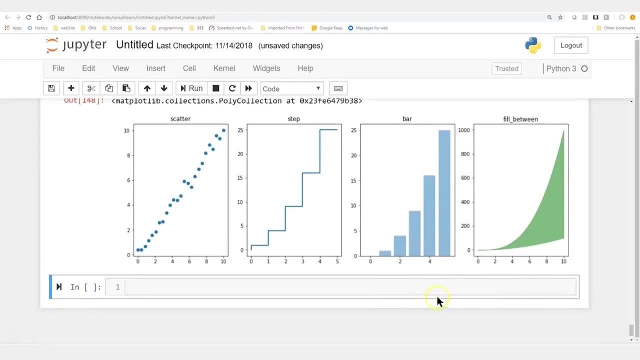 this would be if you had like a car, a motor, and efficiency. they would talk about the efficiency going up and the loss And you're looking for the space or the area between the two lines. So it gives you a nice visual of that. 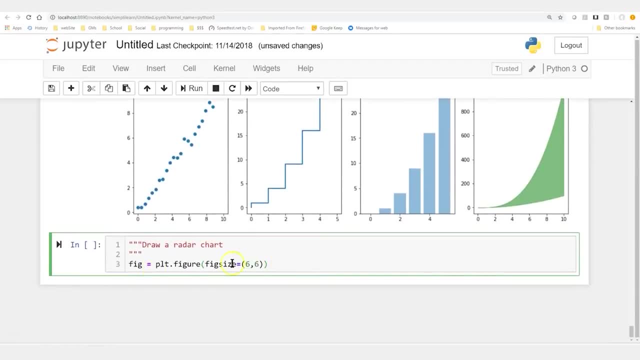 And let's look at a few more basic two dimensionals. So we're going to have our figure, figure size on here. We're going to do a radar chart. To be honest, I've never used a radar chart, either in business or in data science. 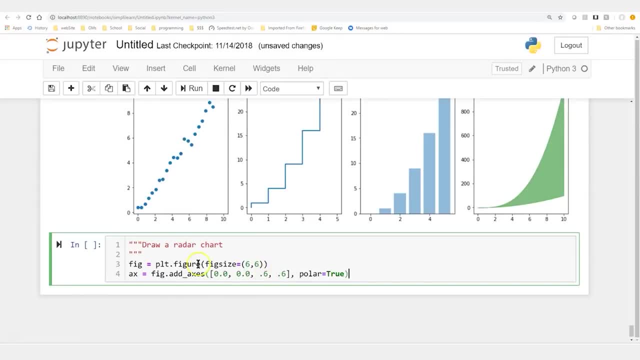 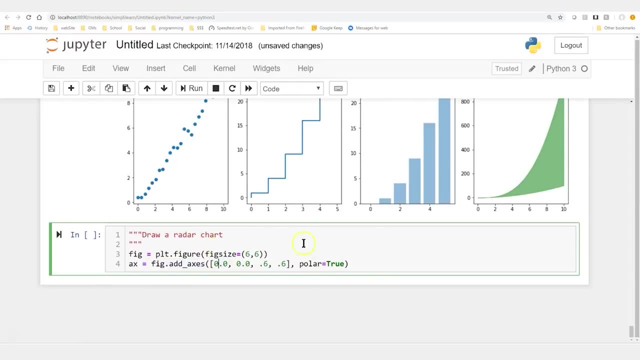 I can't find a reason to use one now. So the first line for doing a radar chart, we have to add axes in the figure And with this this actually creates our. let's run it so you can see what it creates. 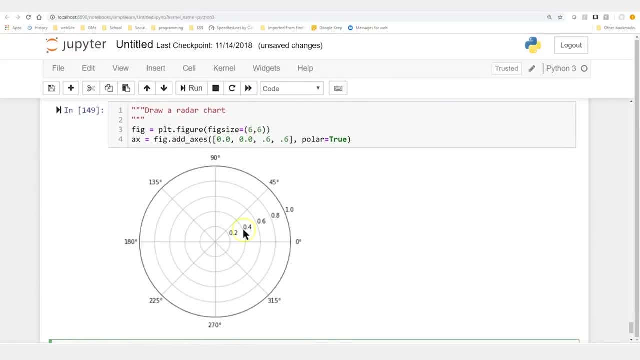 It creates a nice looks like you're on a submarine and you're tracking the hunt for red October or something like that, And it needs all of these. The polar is the fact that we're doing polar coordinates 00.6.6. 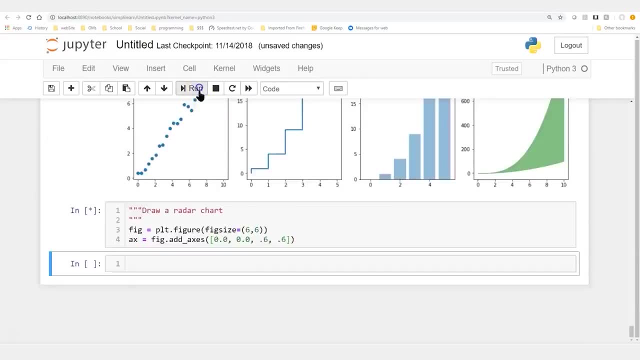 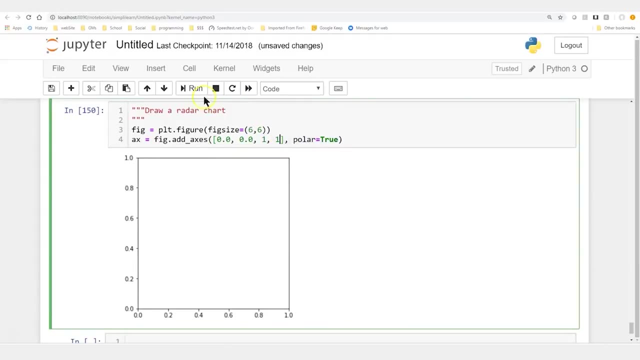 has to do with this. The size: if you take out any of these things and run them, you get just a box. If you take out the other half, you pretty much get nothing in there. And if you change these numbers, change them a little bit. 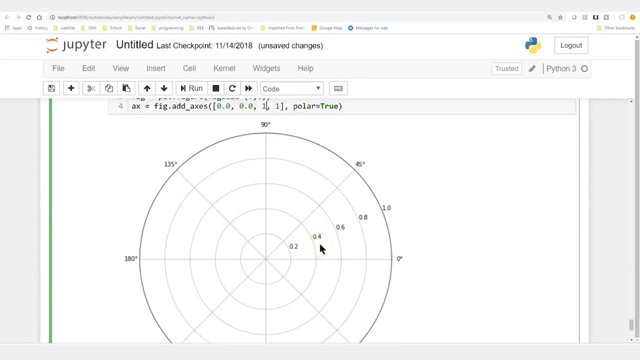 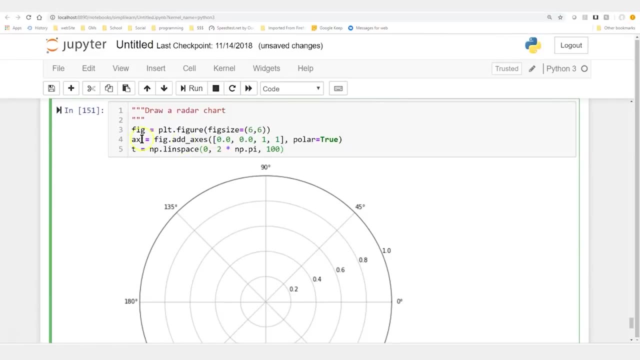 you can see it gets bigger. They had 0.6 on here. I'll go ahead and leave it as one, because that's just kind of fun. But that's all about the size on here, the height and the width, And then let's create some data. 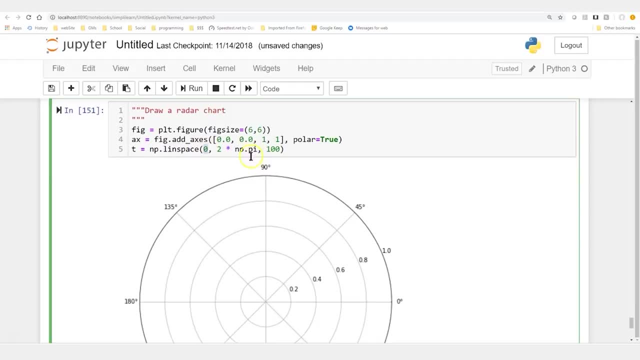 T equals NP line space And this is 0 to 2 times NP, times pi. So, if you remember, that is the distance across and we're going to generate 100 points. So this is just a thing of data we're putting together. 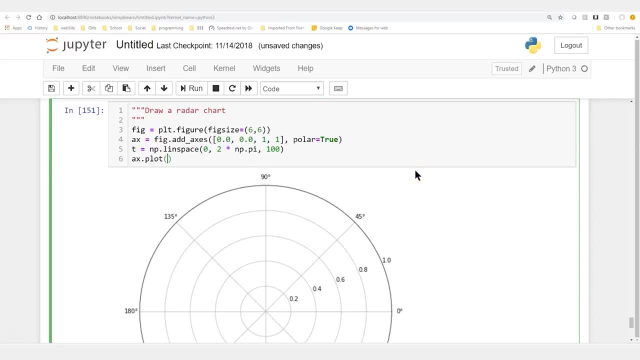 Then we can simply do an ax dot plot And in this case let's do t comma t, which would be a diagonal line on a regular chart, And we'll give it a nice. color equals blue and line width equals 3.. Let's see what that looks like. 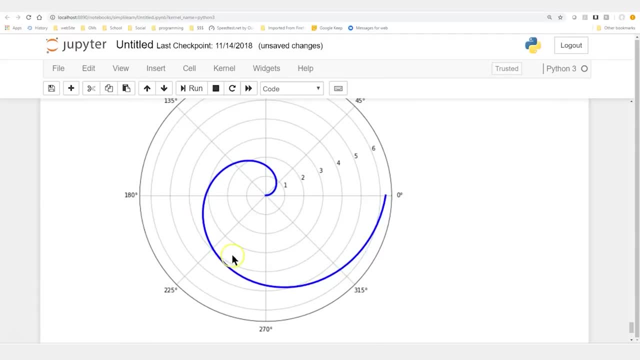 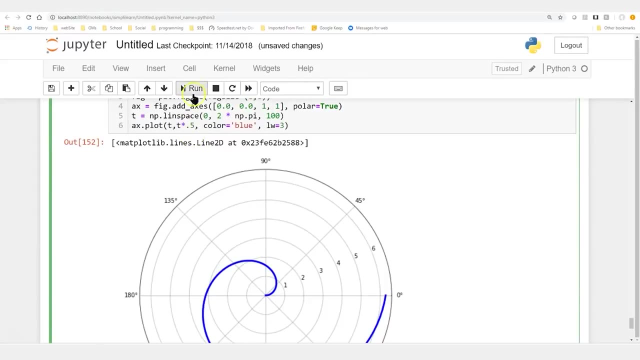 And we can see here a spiral coming out. And remember, this would be just a diagonal line on a regular chart. What happens if we take this and instead of t times 0.5, there we go And you can see it slightly alters the way it spirals out. 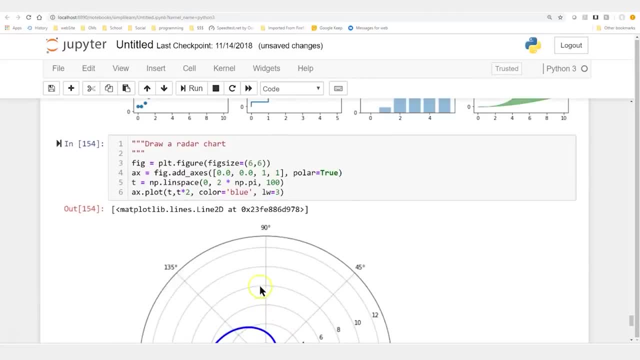 We can do t times 2.. It spirals out a little quicker, So it's kind of just a fun. Like I said, I've never used a radar chart. It's a column, But you can always think of radar in a submarine. 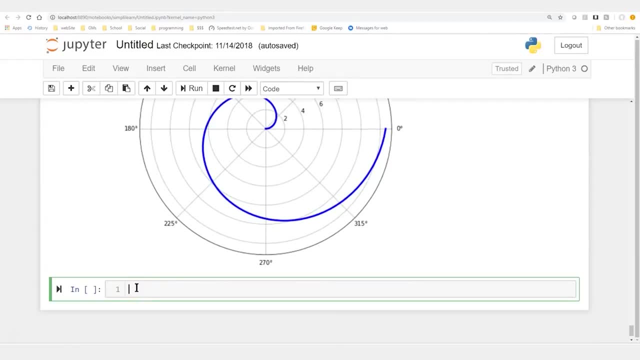 It kind of looks like one of those, or in an airplane. And none of this would be complete if we didn't discuss histograms. Oh my gosh, do I use a histogram so much? And we'll use our numbers We have set as np to generate: 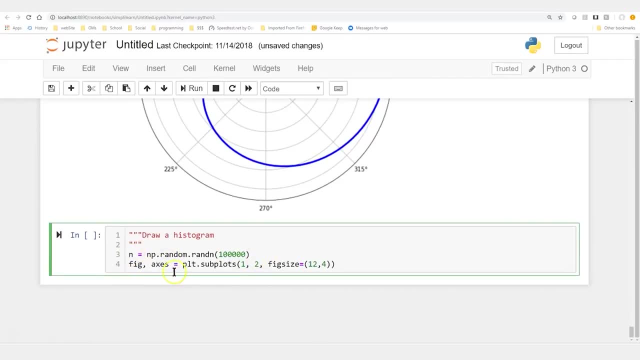 Oh, it looks like we have 100,000 variables. we're going to set equal to n And, of course, we create our figure and our axes: Subplots 1,, 2, figure size: 12,, 14.. So we're going to look at two different variations. 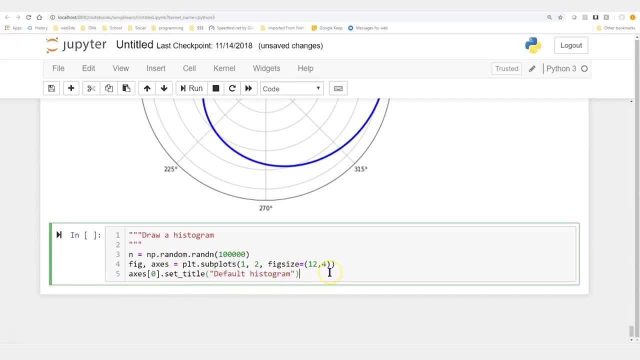 of the histogram And we'll set a title, default histogram, Set our title there And then this is simply hist for histogram And we'll just go ahead and put in our n in there. And let me run this and see what that looks like. 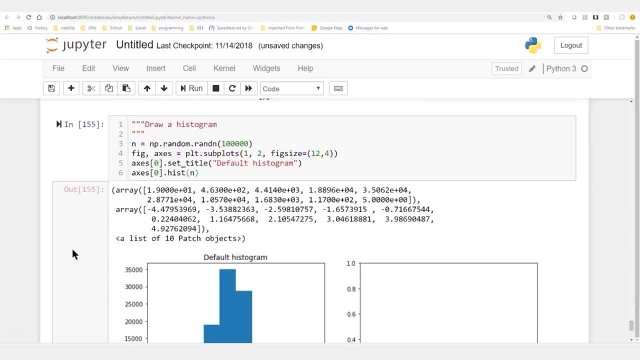 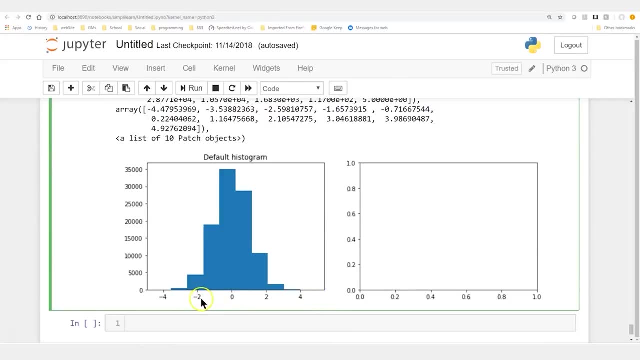 And let's talk about what is going on here. So we generated an array here of data, 1,000 random arrays. It looks like they're mostly between minus 4 and 4.. And then it adds up each one. It says 0, you have 35,000 that are 0. 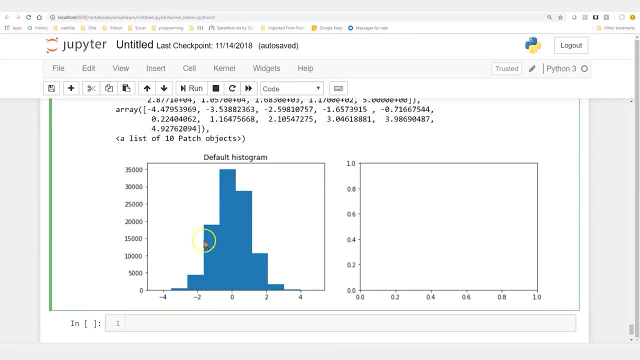 So that's what's most common on here, And we have 20,000 that are somewhere in this range right here between the minus 2 and- well, it looks like 1 and minus 2.. And somewhere between 0 and 1,. 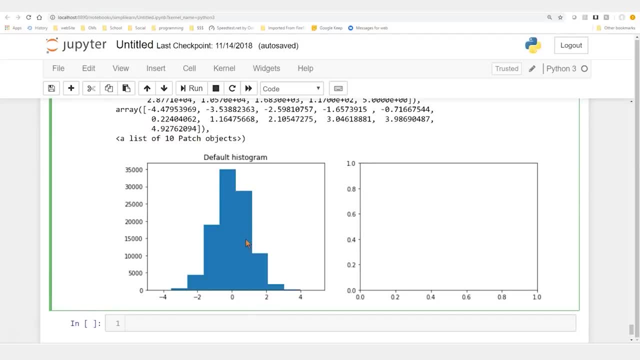 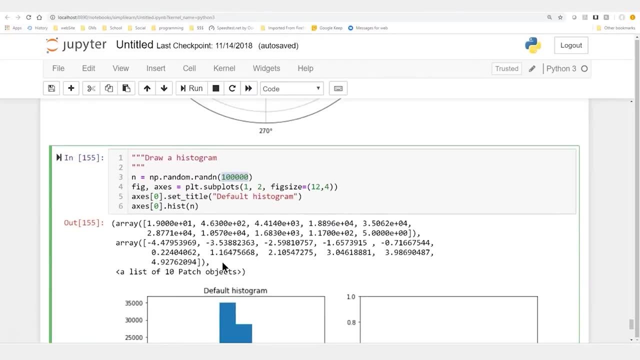 there's 30,000 numbers. So all this is saying is: this is how common these variables are, And this gives you- this will point you in so many directions when you're looking at data science- to go ahead and run your histogram, So you should always have your histogram. 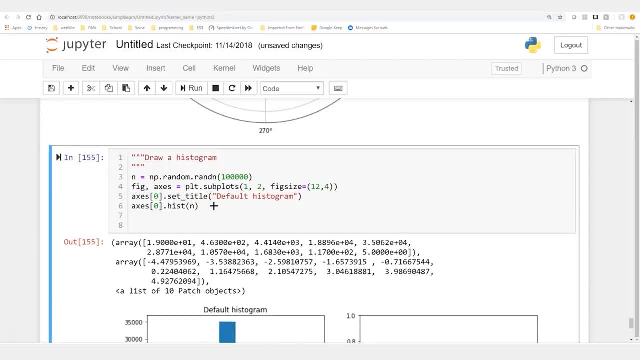 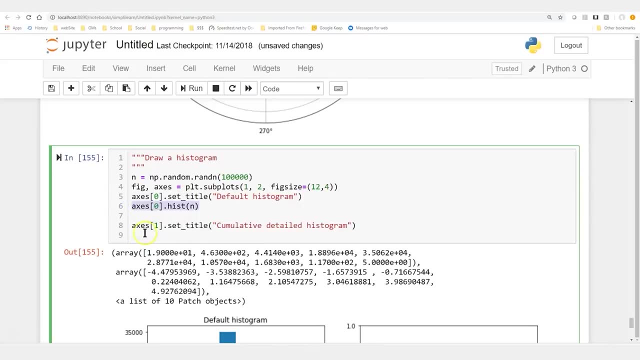 And you can always put limits and all the other different things on your array, Just like you did on the other graphs on there, And then we're going to do a cumulative detailed histogram And all it is is a histogram. Let me just do that. 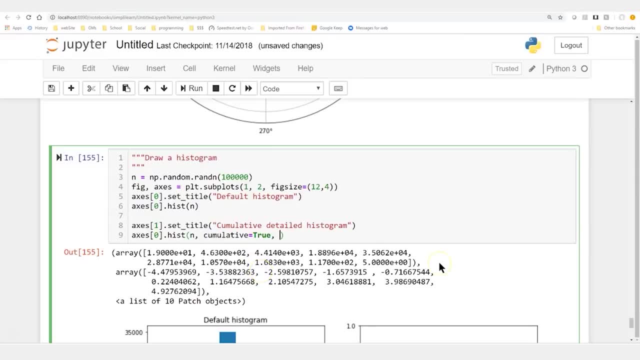 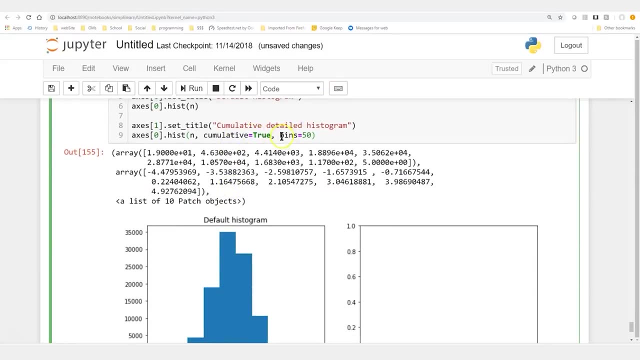 And we set cumulative equal to true And bins equal 30. And I really want to highlight the cumulative equals true is important, But we can now choose how many bins we have In the first one it kind of selected them for us. 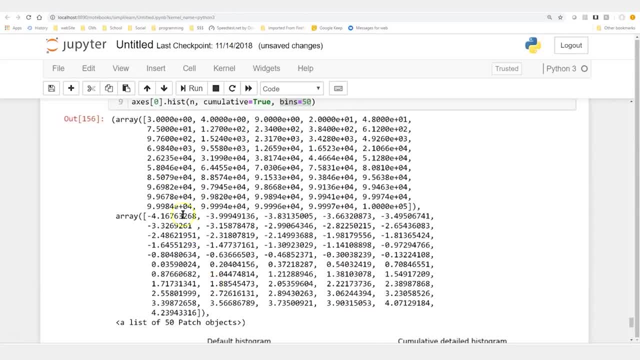 In this case. let me go ahead and run this And you'll see it has. it prints the data out for us. And here's: our whoops must have missed. oh, there we go. It doesn't help that I put it over the old one. 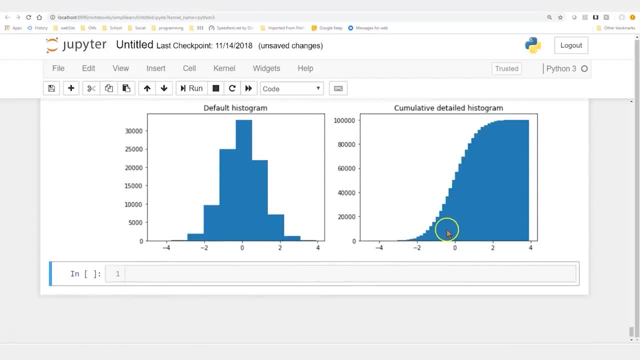 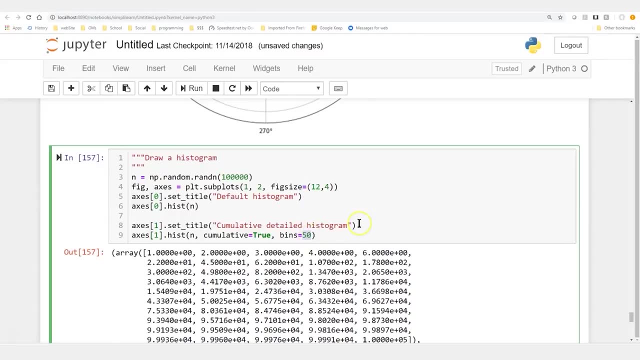 There we go. Okay, So now you have your default histogram And now we have a cumulative histogram And we should have 50 steps in there, And let's just find out if that's true, Not so much by counting them, I'm not going to count them. 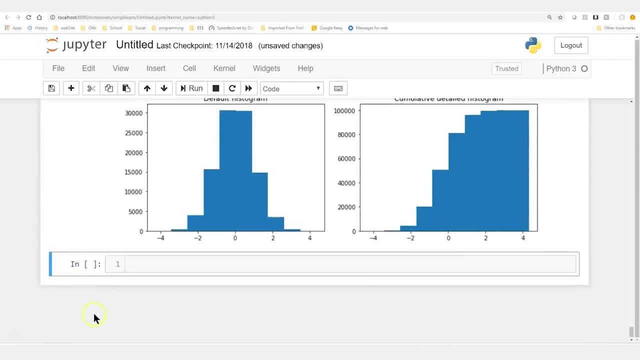 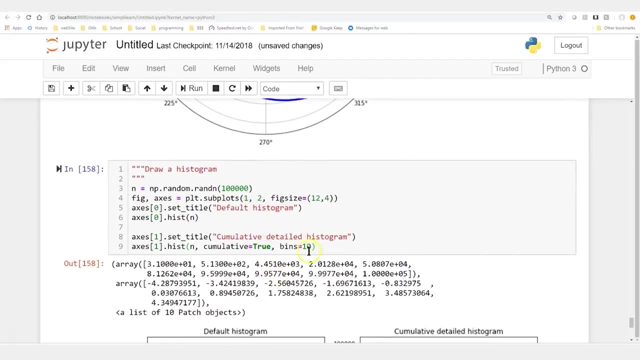 If you want to, you can count them. Let's just change it to 10 and see what happens, And we see, here we have now 10 counts of that And we could set that for five And run that, And then we have our five on there. 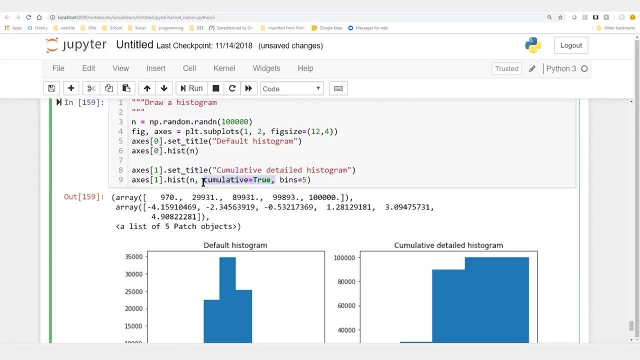 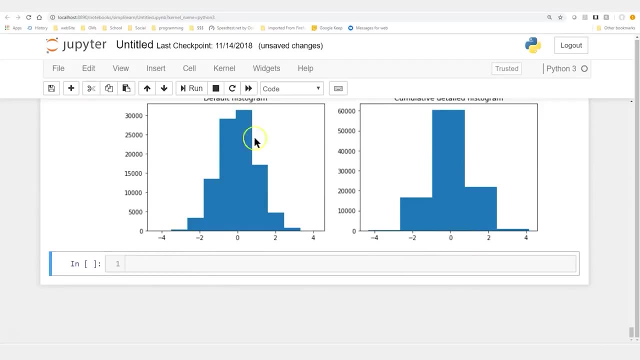 And we can go ahead and take the cumulative equals true out, Just so you can see what that looks like, And let me run that on here too. That looks just like it did before. I think there's what one, two, three, four, five. 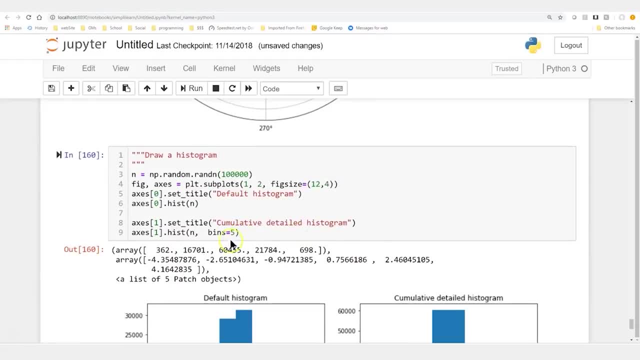 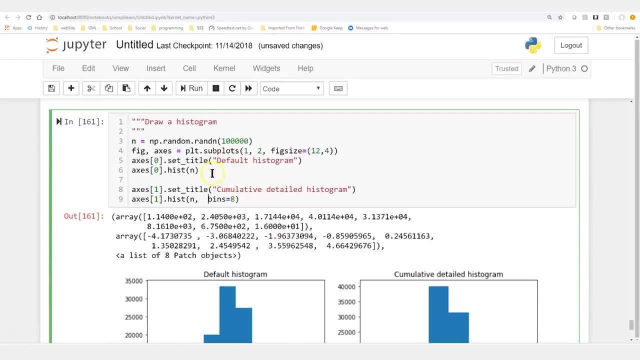 six, seven, eight, Eight different bins on here. That's what the default came out of. Put that back in there, Run, And so now it should look almost identical- And it does, And then we can put the cumulative back in. 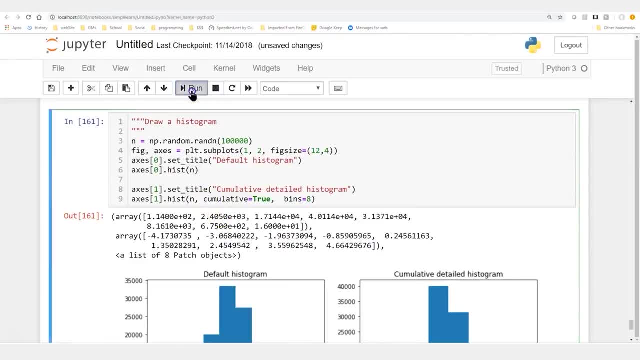 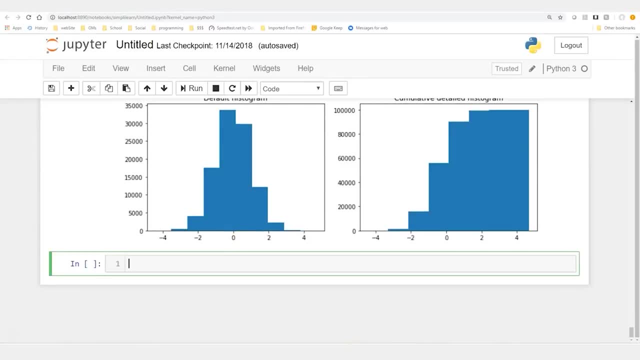 See what that looks like with the cumulative And run that And we can see how that shifts everything over and has a slightly different look. Wait, It shifts it all to the right. No, It doesn't actually shift it to the right. 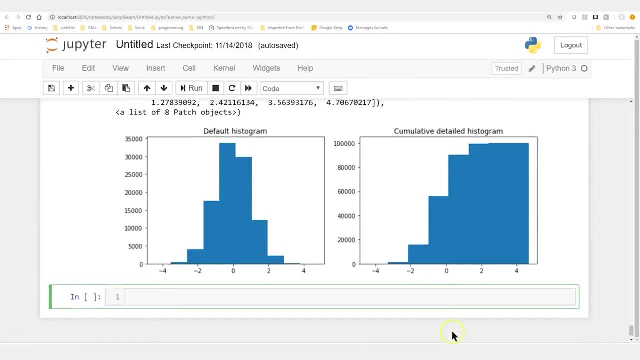 It's cumulative, So it's the total of the different currencies, And so what that means is like, if you consider this, like for the year of rainfall, we have, like, day one, you had a little bit of rain, Day two, we have more rain. 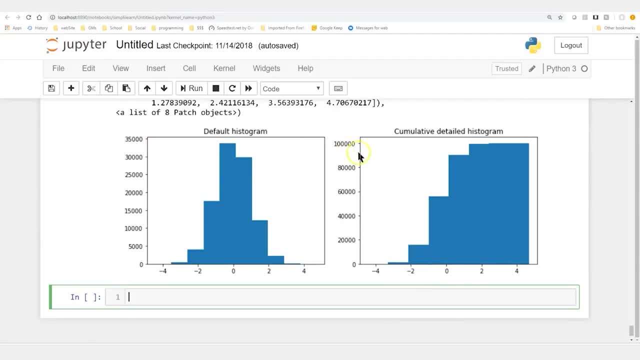 And so if you look at the number, this is 100,000, 35,000. So it's a cumulative, detailed histogram of the occurrence as it grows. And rainfall is a good one, because that would be a cumulative histogram of how much rain occurred throughout the year. 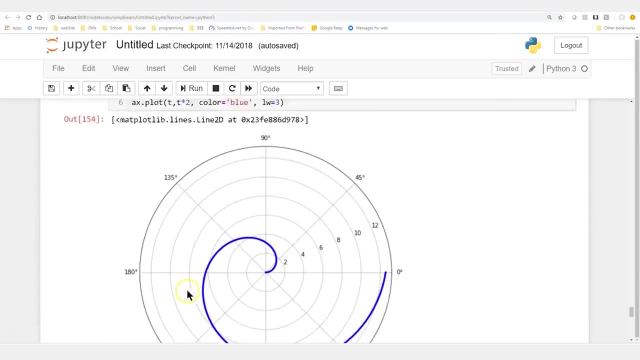 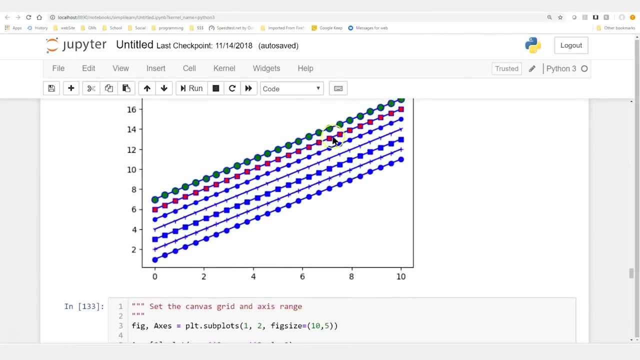 And we're going to look at two more graphs. We've already looked at a bunch of them. We looked at our radar graph. We've looked at scatter step bar, fill in Basic plots. We've looked at different ways of showing the data. 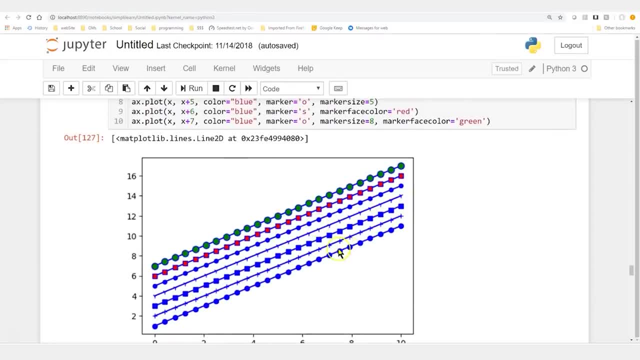 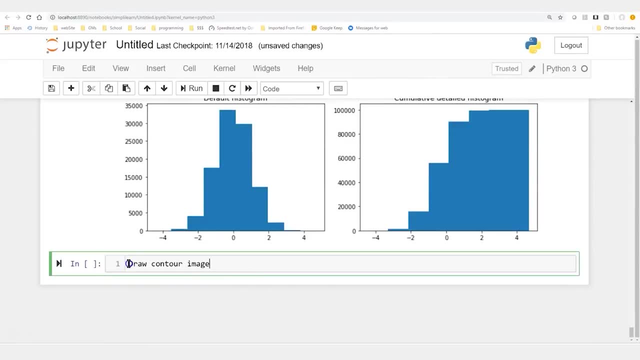 You know we can increase the size of the line, the look, the color, the alpha setting. So let's look at contour maps. Just put that in there. There we go, Draw a contour map. And before we draw a contour map, 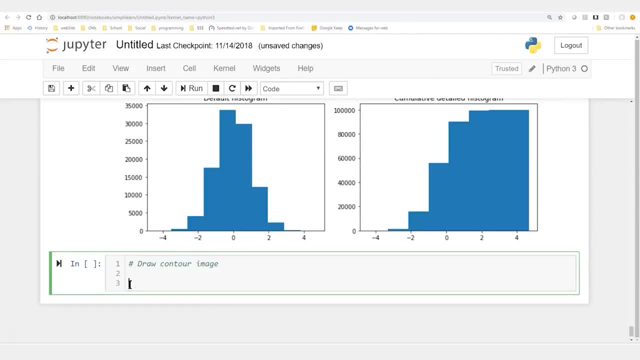 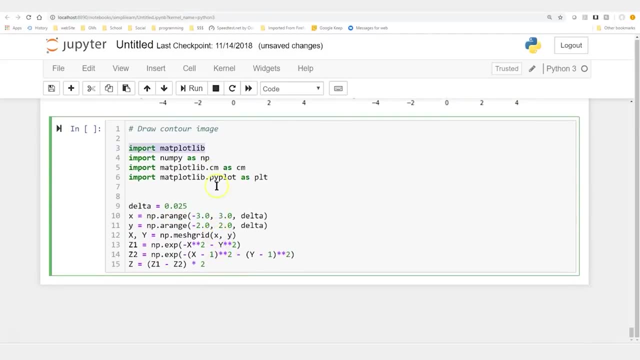 we need to go ahead and create data for it, And if you have contours, your data is all going to have three different values, So let's go ahead and create the data. here We have our you'd import your map plot library. 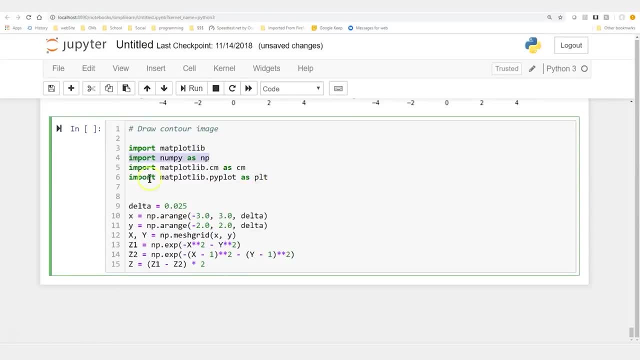 your numpy. so we have our numpy, We have our numbers array And we'll import mapplotcm And that's your color maps. So you have all these different color maps you can look at. There's like hundreds of color maps. 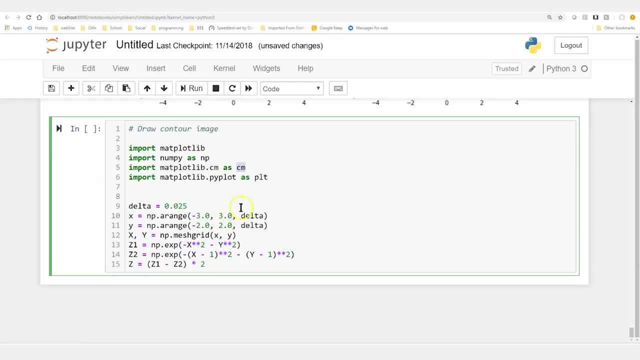 So if you don't want to do your own color, you can even do your own color map. They're pretty diverse- And of course, our PLT, our pi plot, And to generate our different data, we're going to create a delta .025.. 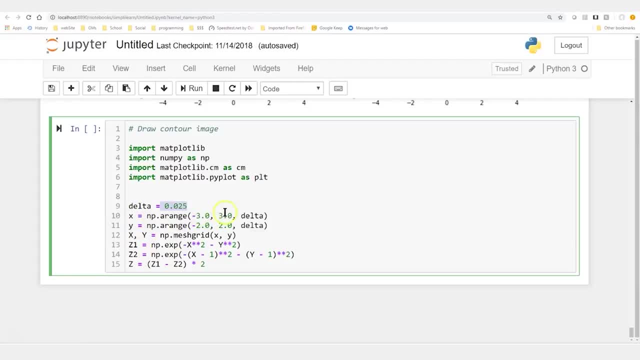 And we'll start with x And we're going to create an array between minus 3 and 3 increments of .025.. And we'll have our y, We'll do something similar And then we'll create our xy into a mesh grid. 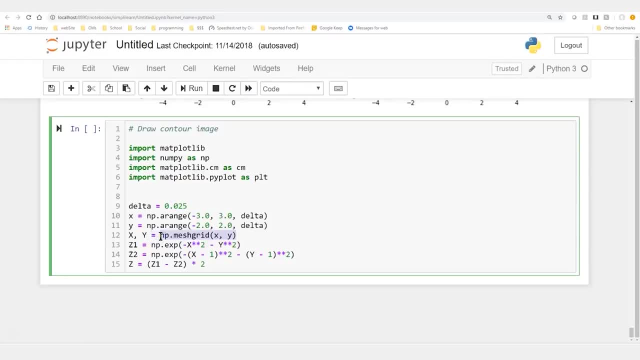 Again, these are all numpy commands, So if you're not familiar with these, you'll want to go back and review our numpy tutorial And we'll do an exponential on here, Minus x squared, minus y squared, for our z1.. We'll do a z2.. 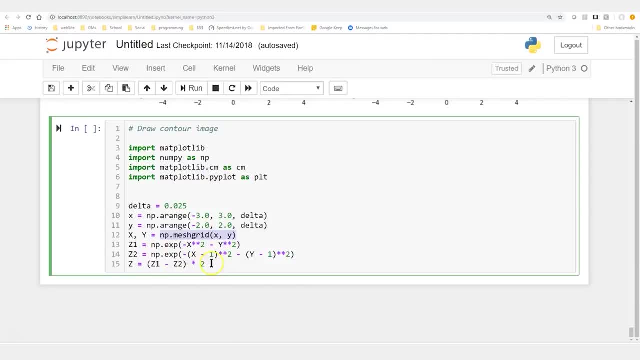 So we have two different areas And z equals z1 minus z2 times 2.. So we've created a number of values here And let me go ahead and run this And let's plug that in so you can see where those values are going. 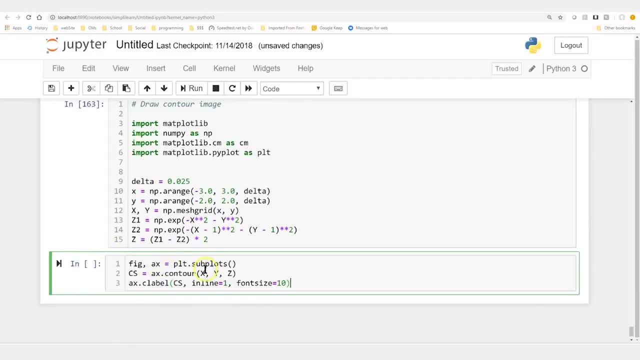 So, once we've set these, we're going to create our figure and our x from our PLT subplots. We're going to create the variable cs And this is going to be our contour. So, right here, cs is our contour surface. 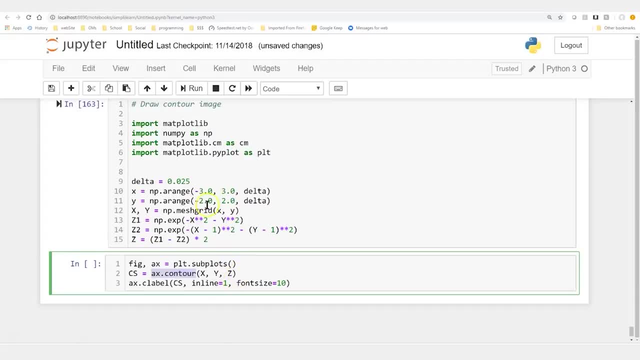 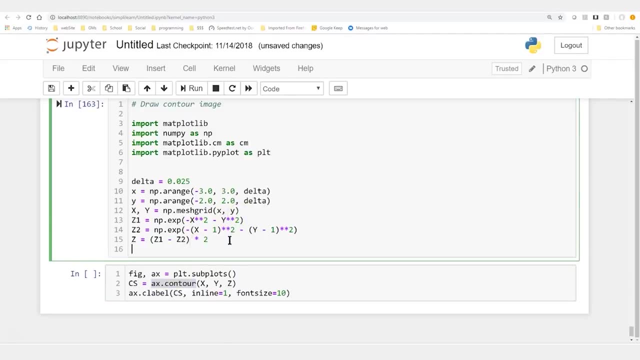 And we're feeding it x, y and z And, if you remember, x- y, we created as our x and y components using our mesh grid, And you know what? Let's do this Just because it's kind of good to see this. 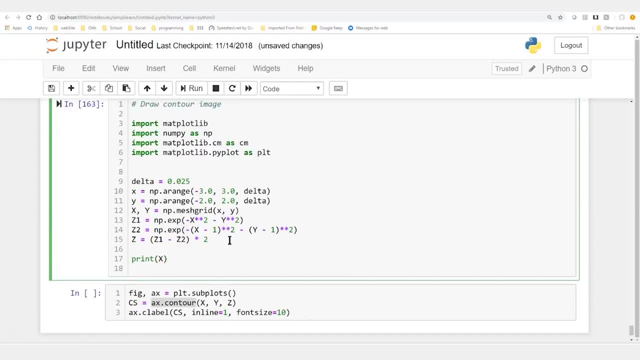 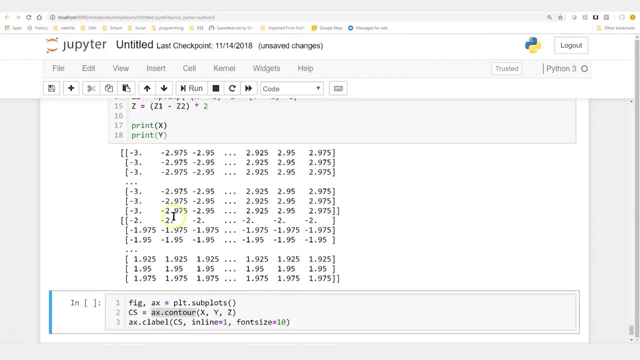 Let's go ahead and print x And let's print y, And I always like to do this when I'm working with something that's either is really complicated- in this case, is what we're looking at- or you don't understand yet. 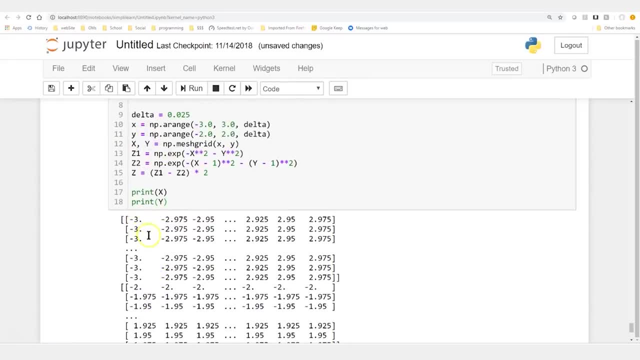 So we've created a mesh grid, We have x, y, And when we're done with this, we end up with: here's our x and this set of values, and our y. So these are our x and y coordinates, And then we've also created z based on our x and y. 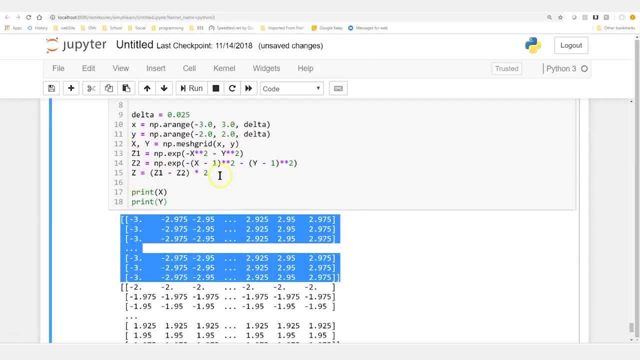 So we have x, capital, X, capital Y and capital Z as our three components, X and y being the coordinates, while Z is going to be our actual height, since we're doing a contour map. So we created our contour map from our x, y and z coordinates. 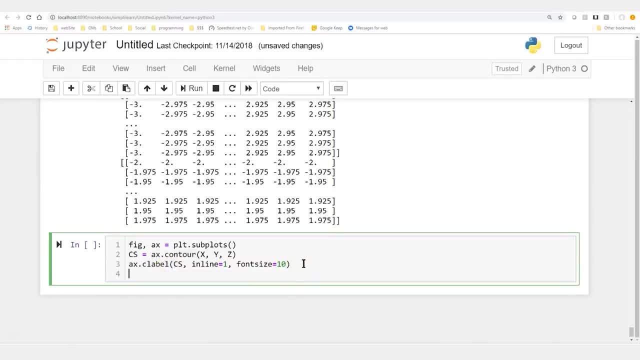 We want to go ahead and put in a C label. Maybe we want to go ahead and do a title on here. We'll put that in our set title And this is a contour. There we go, contour map, And let's go ahead and run this and see what that looks like. 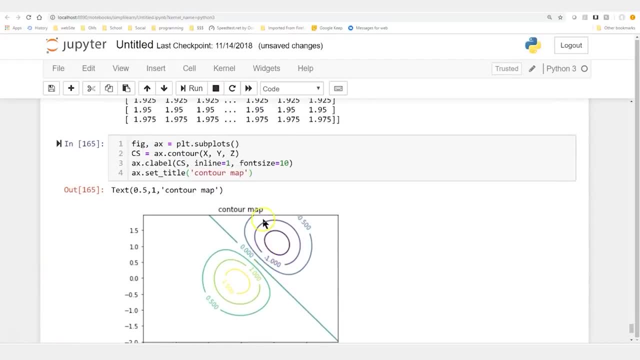 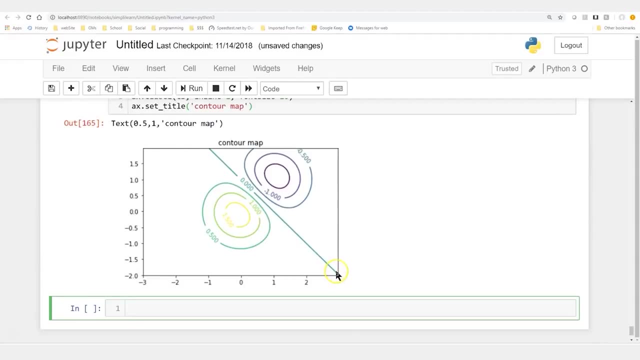 And you'll see we generated a nice little contour map. There's different settings you can play with on this, But you can picture this being: you're on a mountain climb And here we have a line that represents 0, maybe that C level. 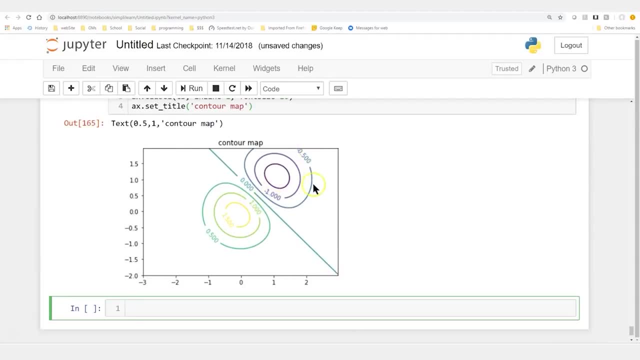 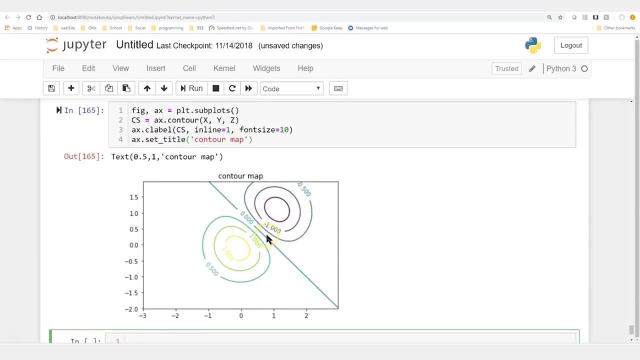 And then, moving on up, you have your contours of 0.5 and minus 1 and different setups, little hills, I guess. if it's minus that's like a pit. So I guess you're going down into a pit at minus 5 and minus 1.. 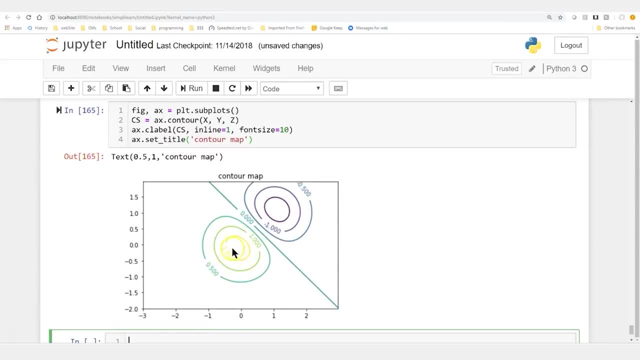 But on the other side you can see you're going up in levels. So here's a mountaintop and here's like a basin of some kind, And in data science this could represent a lot of things. This could also be representing two different values, and maybe profits and loss. 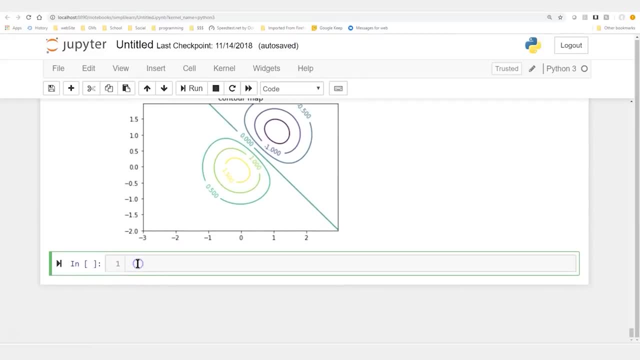 I don't know if I'd ever really do that as a contour map, but I'm sure you can be creative and find something fun to do with a contour map. And then we're going to look at one last map, which is the 3D map. 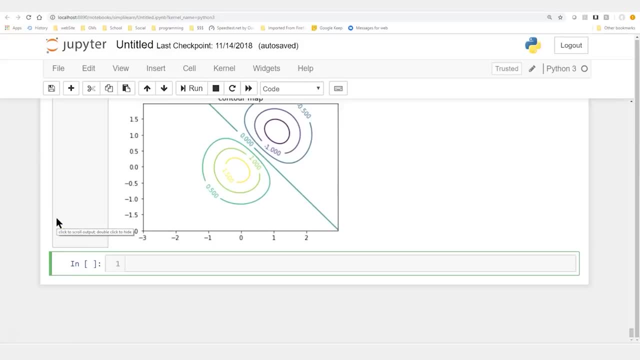 And those can be really important as a final product, because they can show so much additional information that you can't fit on two-dimensional graphs. There we go, draw a 3D image And so we're going to import from our MPL toolkits. 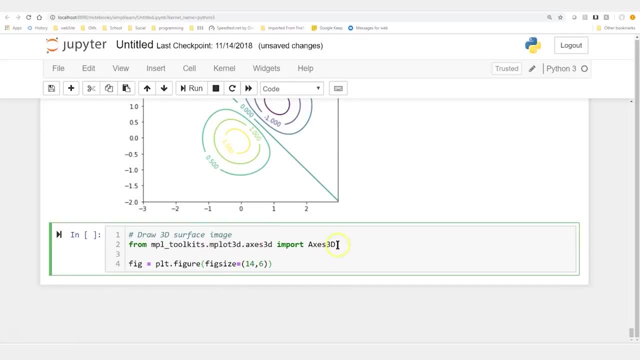 the Mplot3D and the Axis3D. We're going to import Axis3D. This is what's going to let us work with the 3D image And this should look familiar. We're going to create another figure, just like we did before. 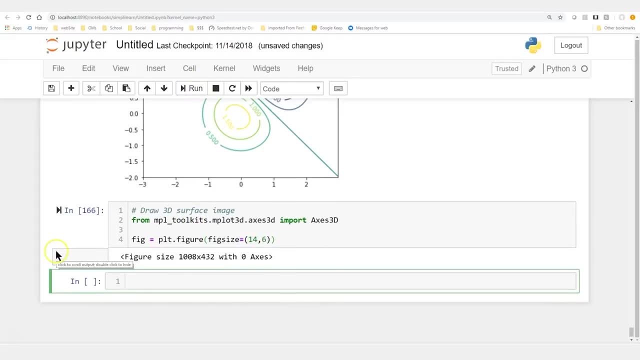 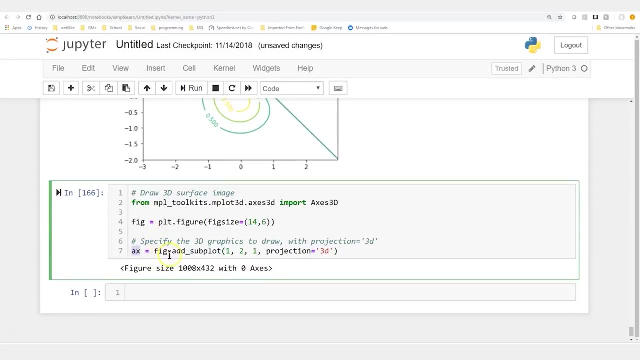 Figure size 14 by 6, that's a good fit on the screen. We'll go ahead and run that. So we have our figure and let's go ahead and take our ax and we're going to set that equal to figaddSubplot. 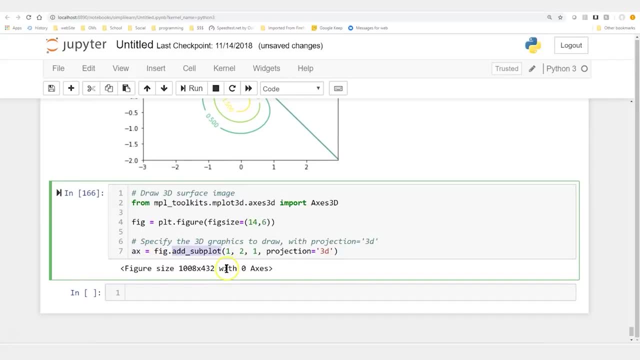 That should also be familiar from earlier And we're going to work with this sets- the settings for the projection, And we're going to use 121, projection 3D, And we'll see what that looks like in just a minute And we just created some three-dimensional data here before. 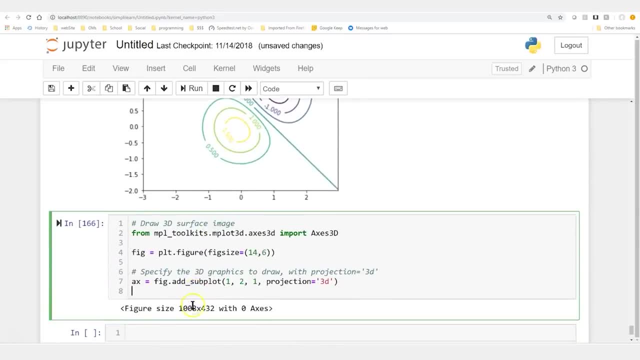 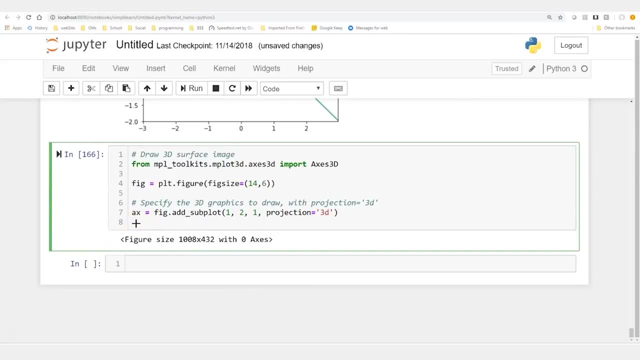 where we had X, Y and Z, capital, X, Y and Z. So we're going to reuse that data. We're just going to use that, since this is also a three-dimensional image. So let's use that for a three-dimensional graph. 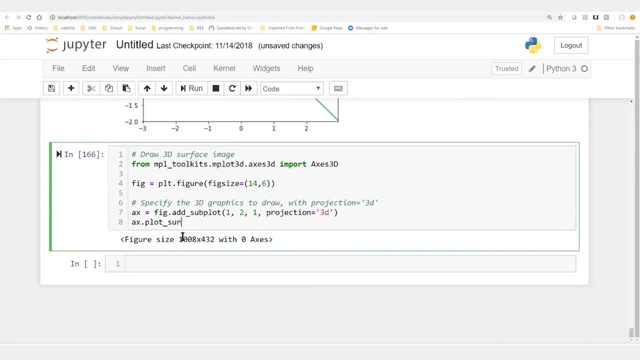 And we simply do axplot, underscore, surface and a capital X, capital Y, capital Z. So there's our data coming in And we're going to add some settings in here. We're going to do rstride 4, cstride 4, and line width 0.. 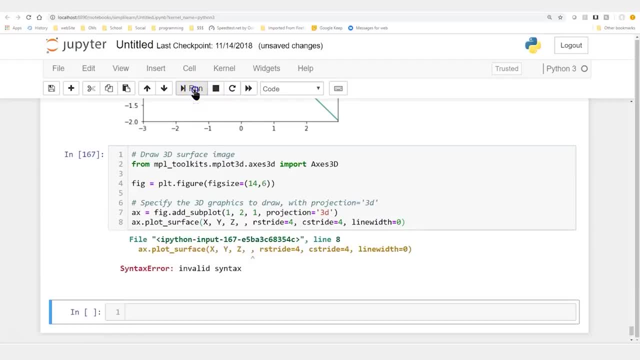 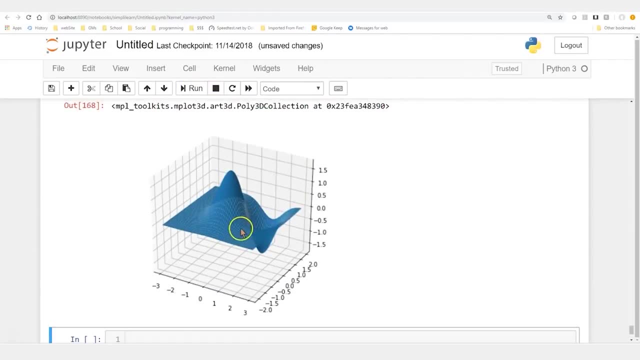 And I'll show you what that is here in just a minute. Let's go ahead and run that so we can see our graph- And of course it helps if I don't add an extra comma in there- And you can see it generates this really beautiful three-dimensional graph. 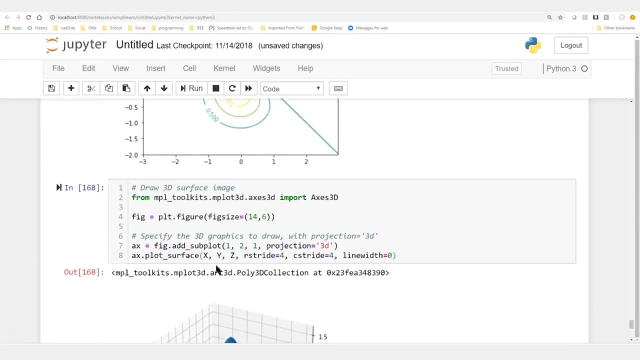 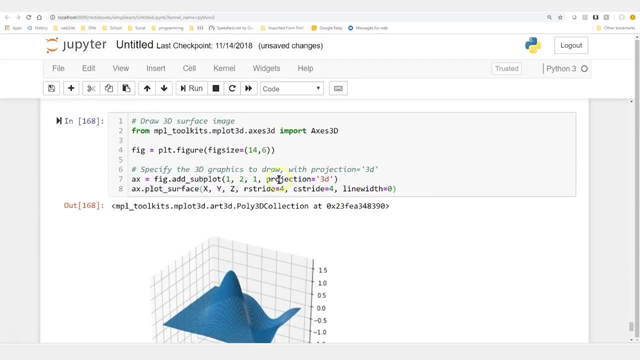 So let's take a little bit of time to explore some of these numbers we have going in. here We have the rstride 4, the cstride 4, and the projection 3D. Projection 3D is the important one, because that's telling us that this is a 3D graph here. 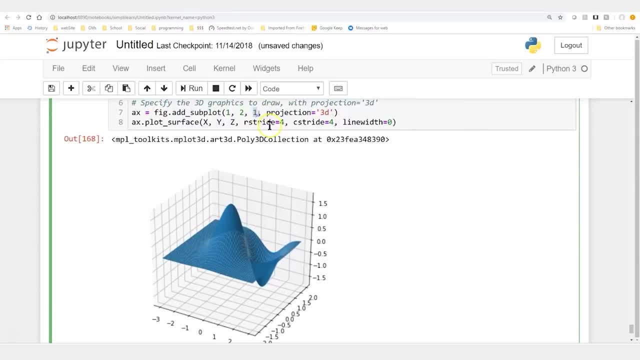 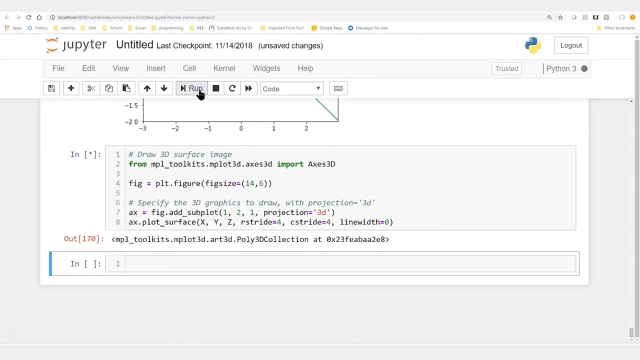 So what are these first numbers, 1,, 2, 1.. Let's just change one of these. I'm going to change this to 5. And it's going to give me an error. Let's change it to 1.. 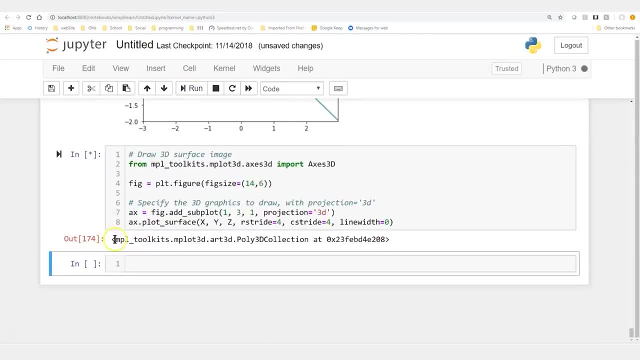 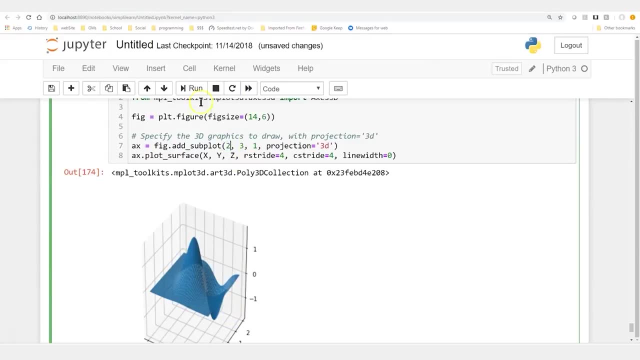 And that didn't work. Let's change this middle one to 3 instead, And you're going to see how it starts reshaping the size and how it fits on the screen And we'll change the first one to 2.. And we'll run that one. 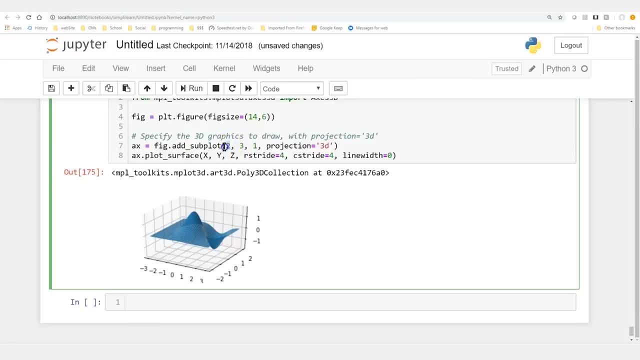 And again it's changed the dimensions and the size and how it fits on here. Play with these numbers so you get a nice look and feel for it. Part of it is the tilt and the angle. We'll do 7 on this one. 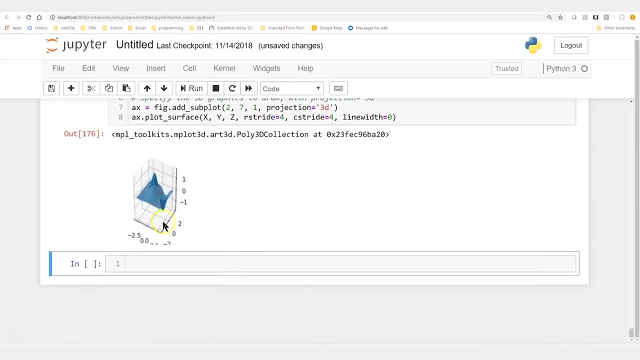 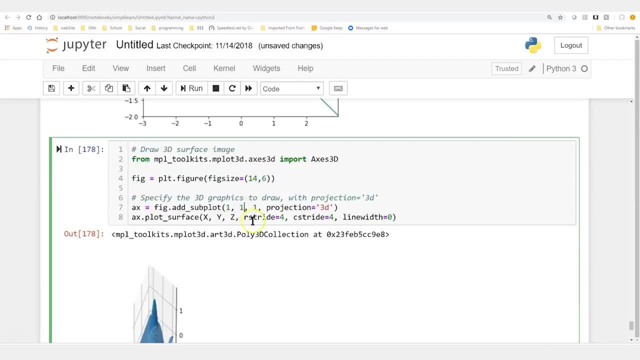 There we go. You can see it really shifted it there. But again, that changes the size and how it fits on the canvas. But we'll leave it at the 1, 2.. And just so you get a good look at what we're talking about here. 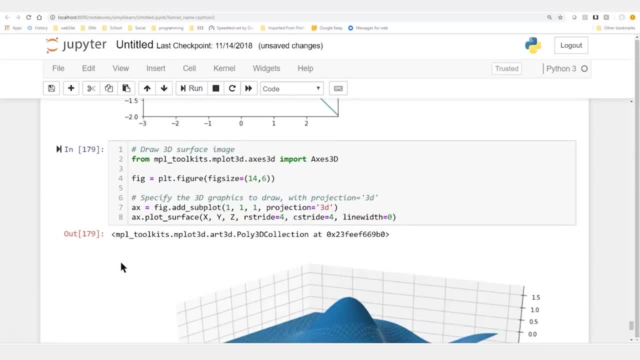 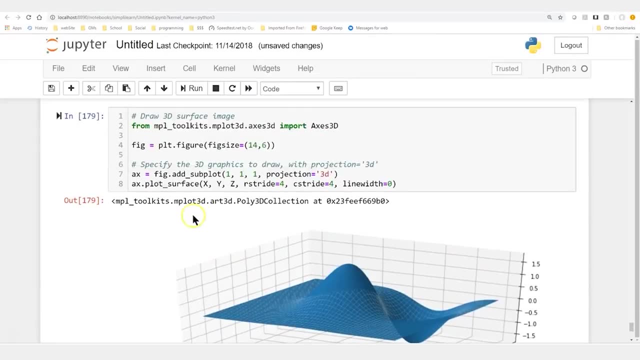 this is column width and index from before. If we do 1,, 1,, 1, you can see that it now spreads it out all the way across. It uses the whole setup on there. So this has to do with the size and how big you want it to be. 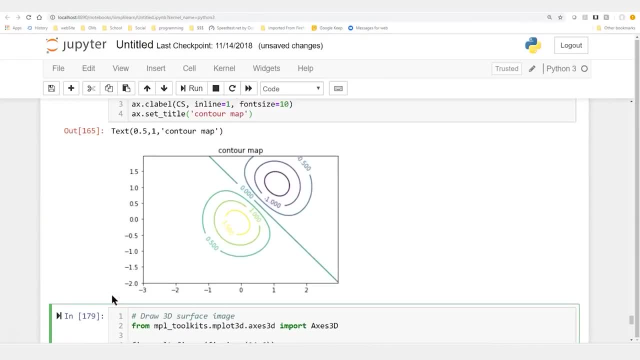 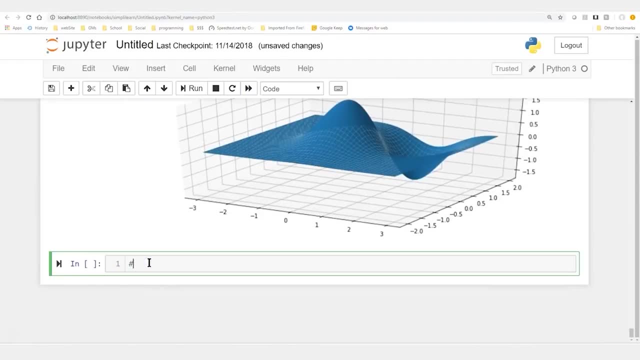 Now, there's one term that we didn't cover in this yet, but we've used it throughout the whole setup, And I'm just going to type that down here, even though we're not going to go into detail, And that's the term heat map. 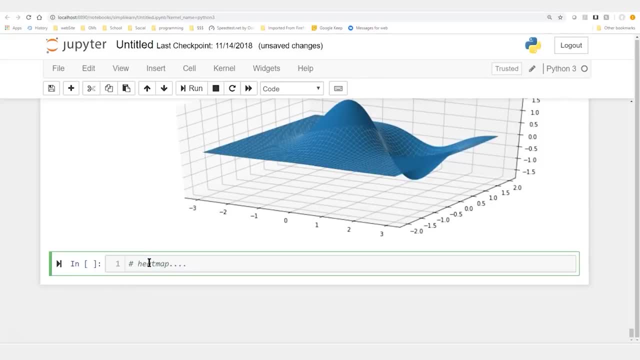 You might see that as kind of starting to lose ground as far as a common reference, But there sure are a lot of people who still talk about heat maps. What is a heat map? Well, it is simply a color map. That's all it is. 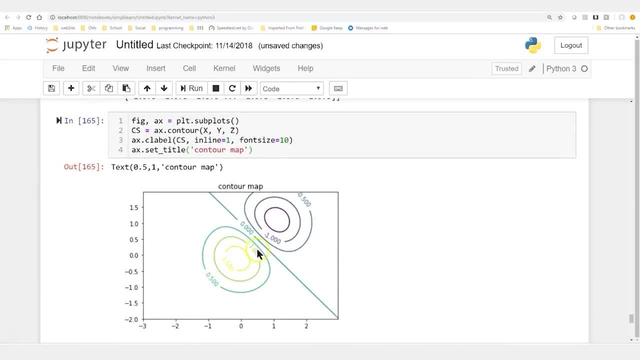 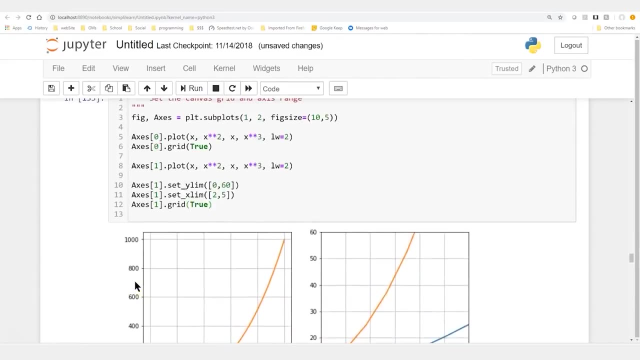 So if you ever see the term heat map, that refers to the fact this is in different colors representing different heights. That one isn't a heat map. But you can see up here we switched into. Let me go back up here. Here we go. 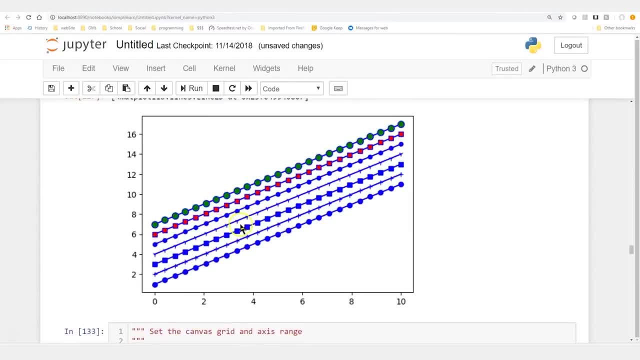 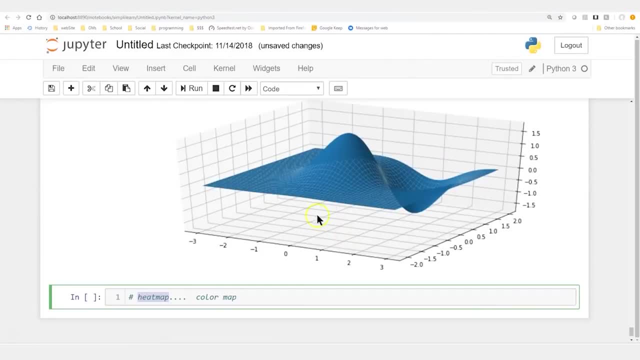 This one has different colors for the different values. A lot of times you'll use like: instead of X and Y, you might do a heat map where you have a fourth value And the fourth value represents the color, And you'll see this 3D image in a nice color. 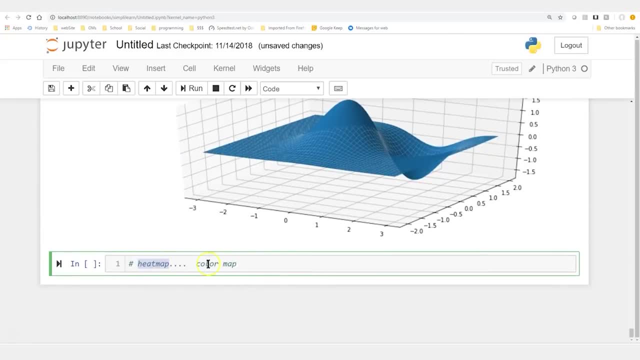 represented by a heat map. That's all it is. So if you see the term heat map, that only means we're plotting some of the data in color to make it stand out, or to give it a fourth dimension, in this case. So we've covered a lot of things on map plot. 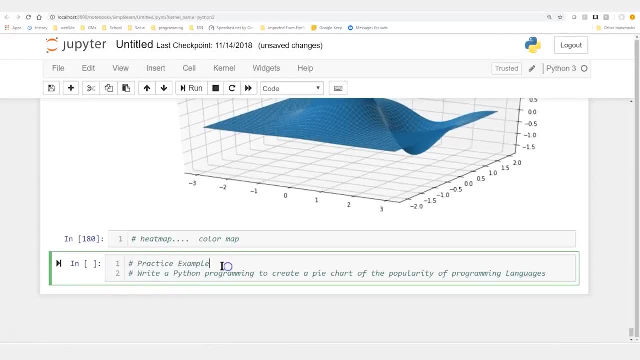 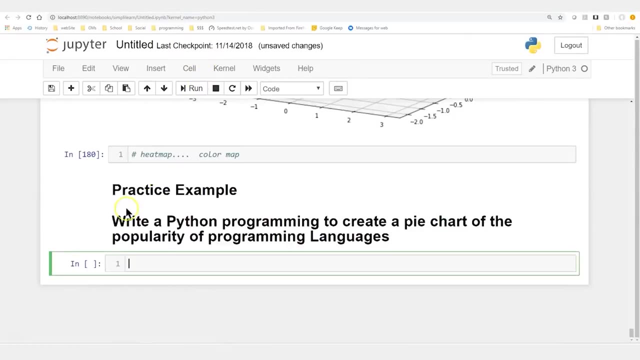 And that brings us. We've covered all the basics. So that brings us to practice. example, And this is going to be the challenge for you. And let me go ahead and change our cell Cell type, mark down and run that so it looks pretty. 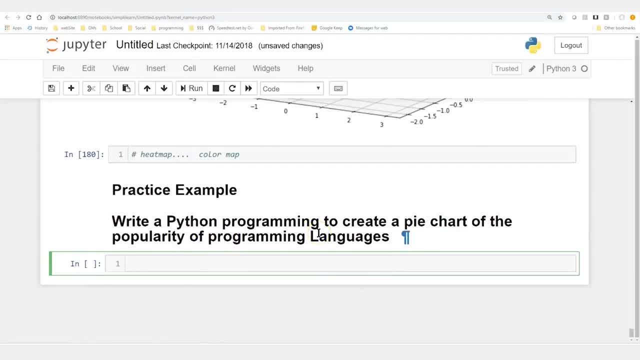 Practice example: Write a Python program to create a pie chart of the popularity of programming languages. Okay, excellent. And if you're going to have a challenge, we need some data, And I'll just throw in our import, our map plot library at the beginning. 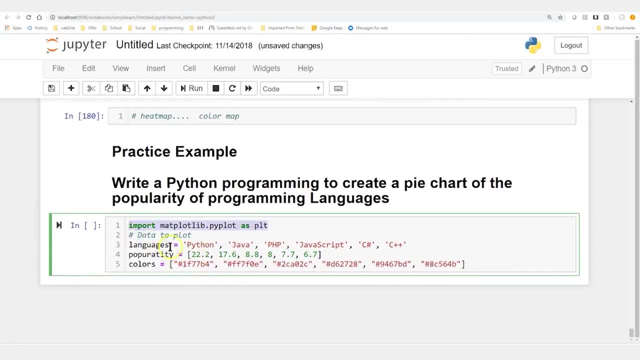 You should do that automatically, And so, for our data to plot, we're going to have our languages, We're going to have Python, We're going to have Java, PHP, JavaScript, C, Sharp, C++. So those are six categories. 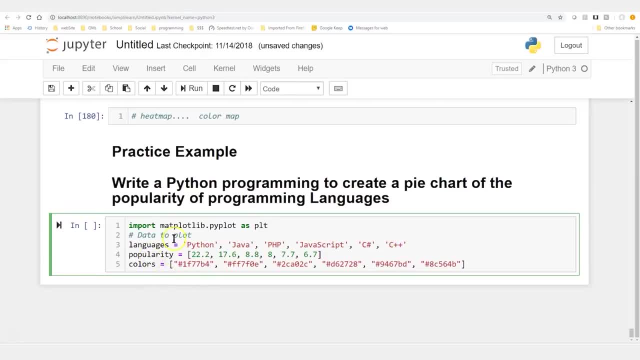 And then we have our popularity. Oops, misspelling there Popularity. We'll give the first one: 22.2%. Java 17.6.. And I don't know if these are real numbers they pulled. My guess is that they might have just been made up, because I don't know if Python is really that much more popular than the other ones. 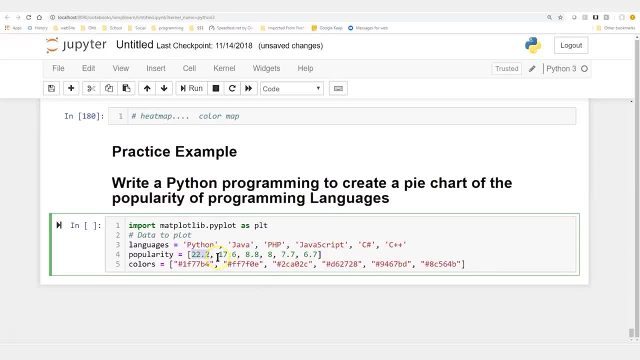 Maybe specific to data science, because Python is very popular in data science right now because it has so many options. The only other program that is highly used and exclusively for data science is R, So Python is big And Python also does a lot better. 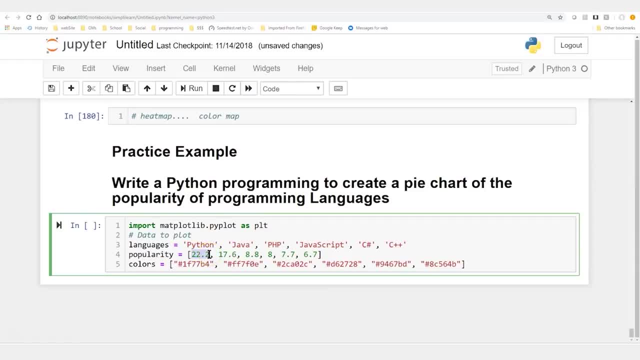 It's a full programming language where R is primarily for data science. They didn't even put R in here. So we have Python, We have Java, We have our PHP And you can see the different values they've given it or different percentages. 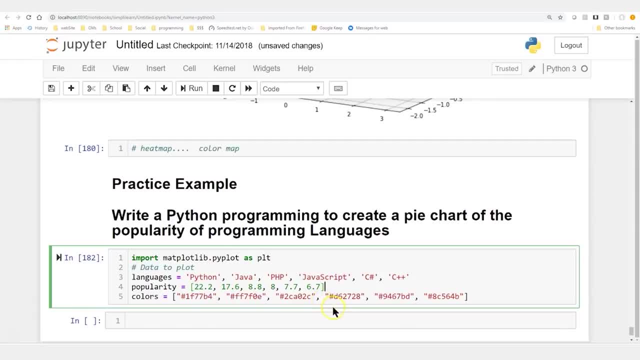 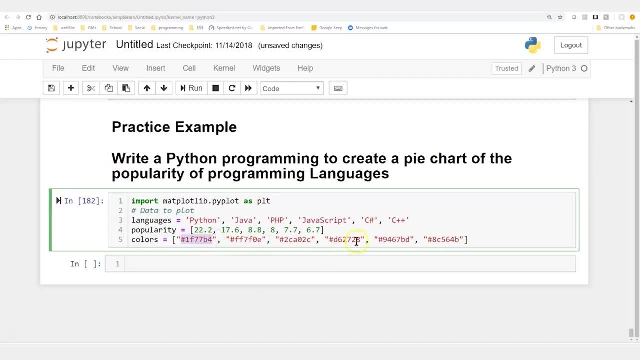 And I did add these up. It does not add up to 100%, It adds up to 71% or something like that. And then we're going to give colors And we've chosen these guys in the back brought in these colors. 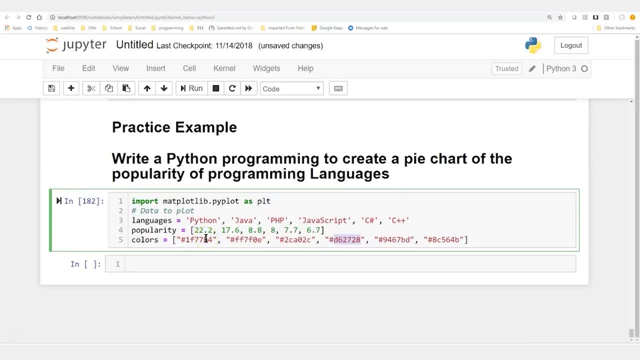 I'm not sure what these colors are. We'll find out in a minute, So it'll be exciting. But you can see they're using the actual color values You can pull off of a color wheel or something like that. You could have just as easily done blue, red, green if you're too lazy to pick the exact colors. 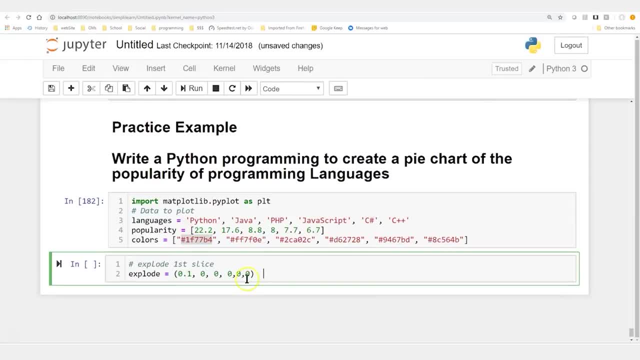 And then let's go ahead and solve this and see what we got here. We're going to do something a little fancy just because we can. The first thing we're going to do is we're going to use a variable called explode, And you'll notice that there's six variables in here. 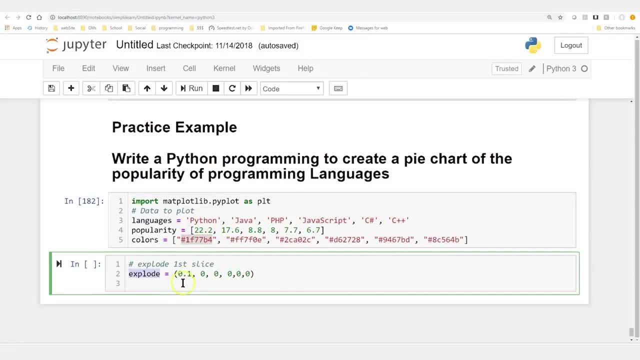 So that matches our six different categories, And the first one we've done is 0.1 and then 00000.. So 0.1, when we put this in here under the explode in the plot, it will actually push that square out. 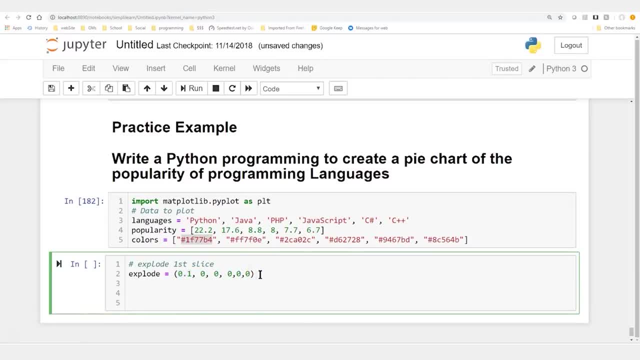 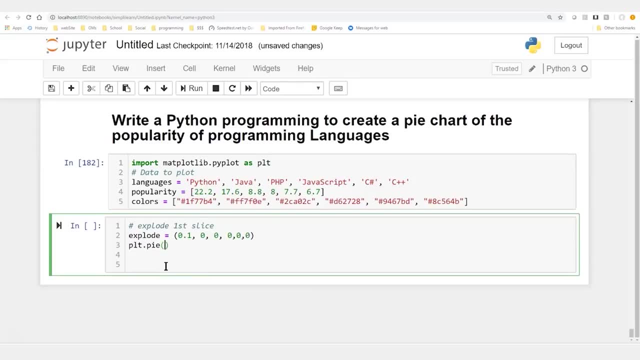 So it's a really cool feature to highlight certain information on a pie chart, And this is simply pltpie And we're plotting popularity. There we go, And before we add in all the really cool settings for this, let's go ahead and run it. 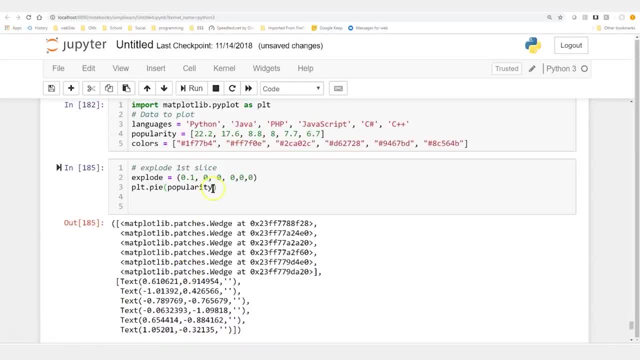 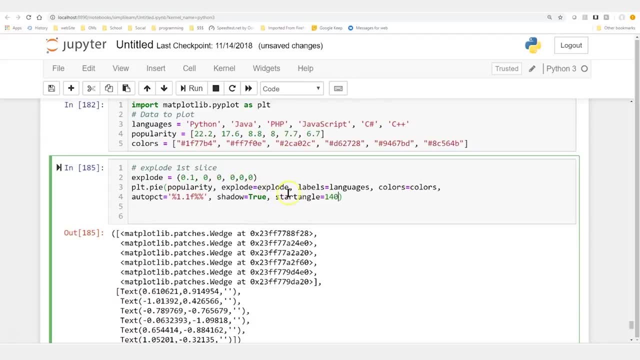 And you'll see we generate a nice flat pie. Not too exciting there. And then we'll go ahead and put in all the extras. I talked about explode, where we can explode one of the values out. So here's our. explode equals explode. 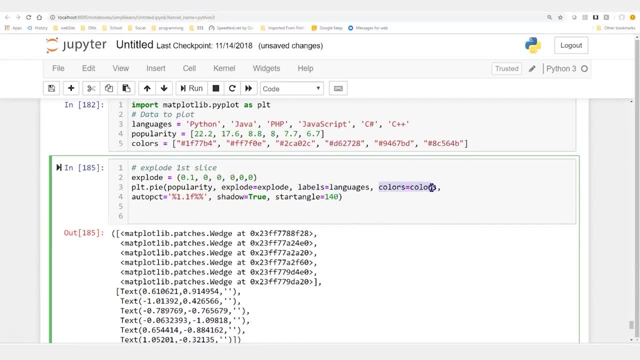 Labels is languages, because we want to know what the different colors mean. Here's our colors, equals colors, Our auto picture And this is standard print format. So that's a Python setup on there And that's just going to put the value on the pie slice. 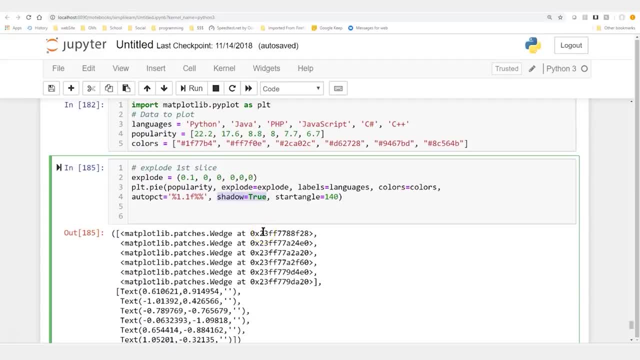 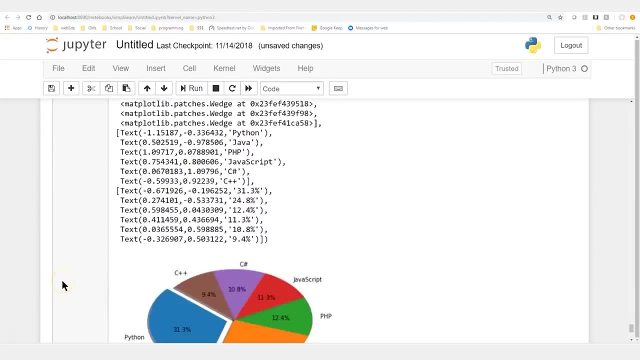 And then we're going to add shadow, because it just looks cooler with a shadow, It gives it a little 3D look And we'll do a start angle of 140.. Let's go ahead and run this and take a look and see what comes out of that. 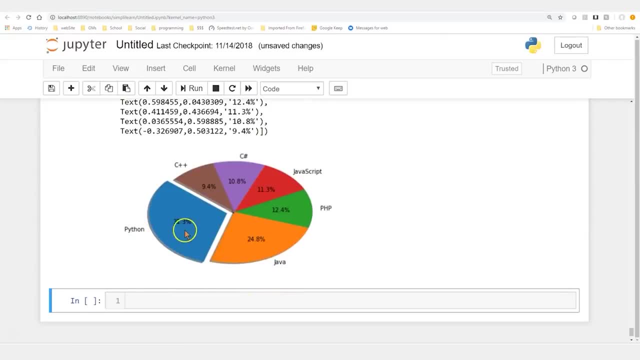 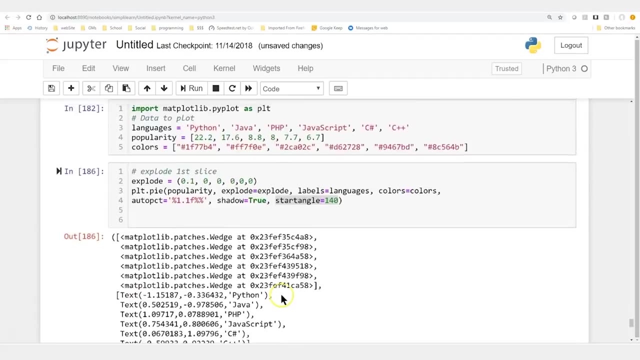 And look how that changes the whole setup. So here's our labels, There's our value we put on there, There's our slice that's pushed out, There's our shadow with 3D effect, And then we started at 140.. 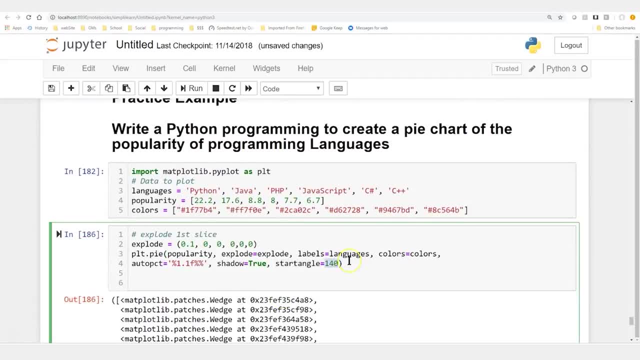 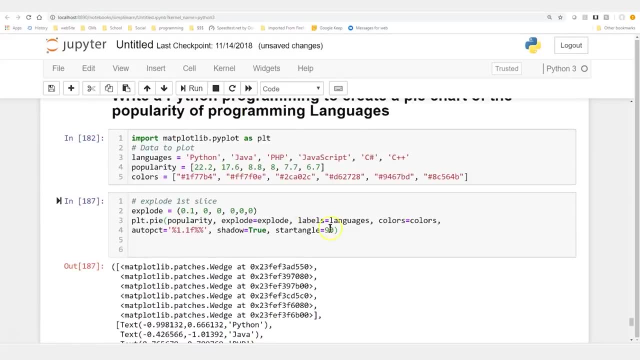 We could also rotate this. Let's just do this angle 90. And if we run it you'll see the blue pie slice has moved up a little bit And we could actually just take the whole starting triangle out and run. It'll default to zero. 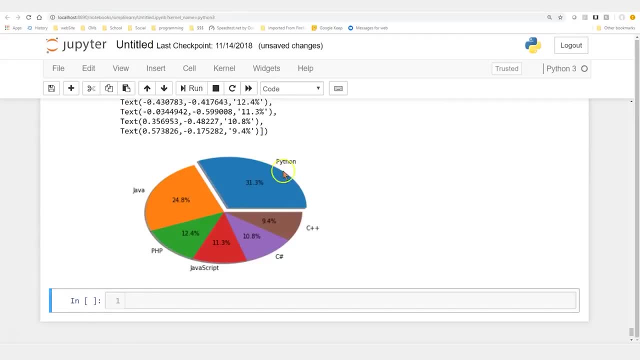 And this is what it looks like if it defaulted to zero. So, depending on where you want the highlighted slice to appear, usually you want that to appear on the left, because people read left to right, And so it draws a focus onto, in this case, Python and how great Python is. 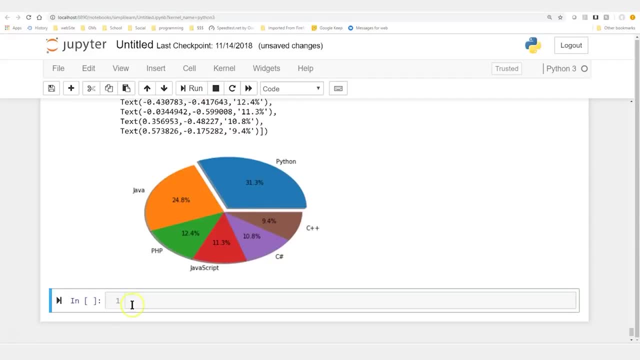 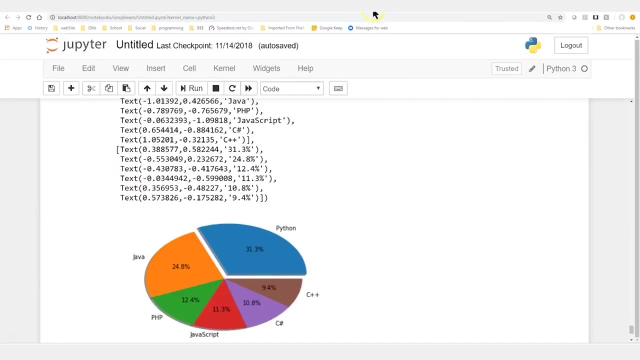 I'm a little biased. We're teaching a Python tutorial, So it should be understandable that we're looking at Python. And one last reference before we close. You can go over to the matplotlibrarycom. We've got pyplot set up And if you go underneath the different functions on there, 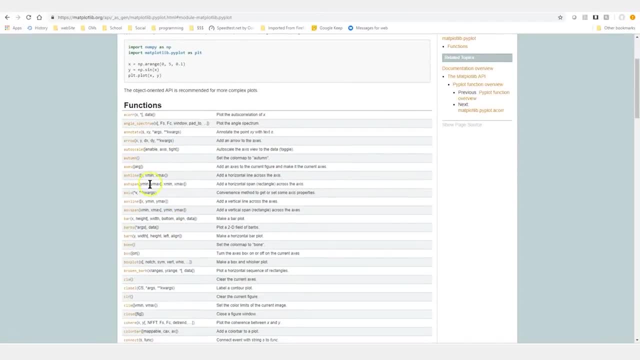 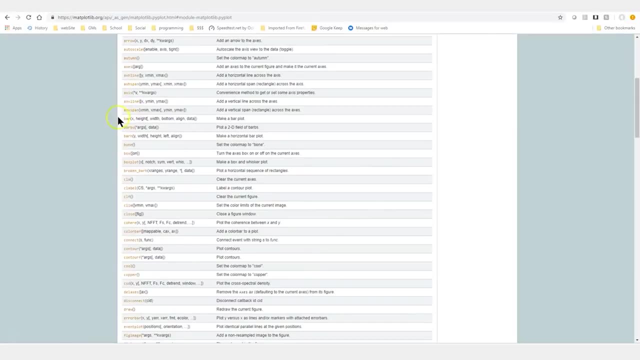 you can look this up on their website. you'll see a full list, And this is why it's so important to go through a tutorial like this, because this list is just so massive. I'm trying to figure out like: here's our bar plot. 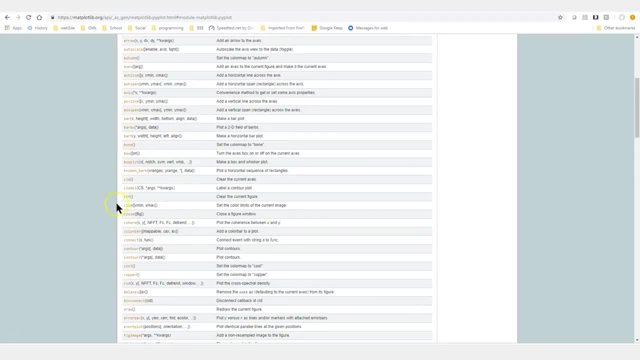 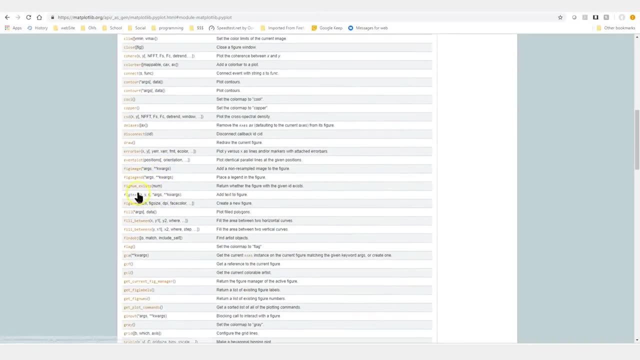 There's a bar h, You can add barbs. There's a box plot. we didn't cover C labels, totally different kind of for your contour plot. you can set up in there. If you go down here we have our figures we used on there. 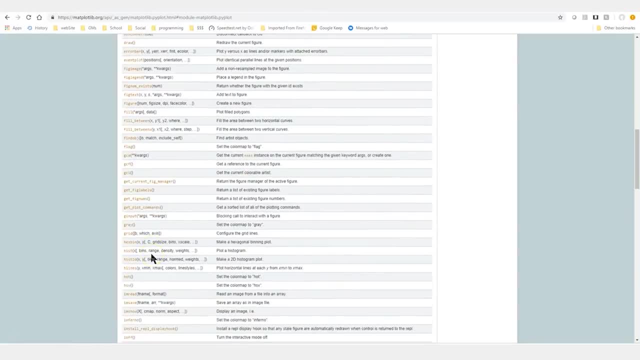 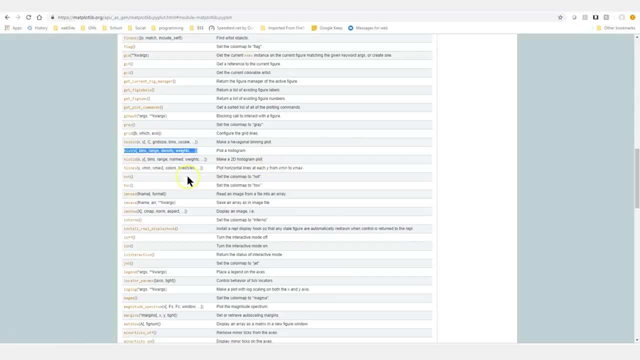 I showed you the basics of how to do the figure. You'll see some closer references on those. There's a histogram down here, HIST. There's also the HIS2D makes a 2D histogram plot H lines. All of this, these are all the different commands that are underneath of here. 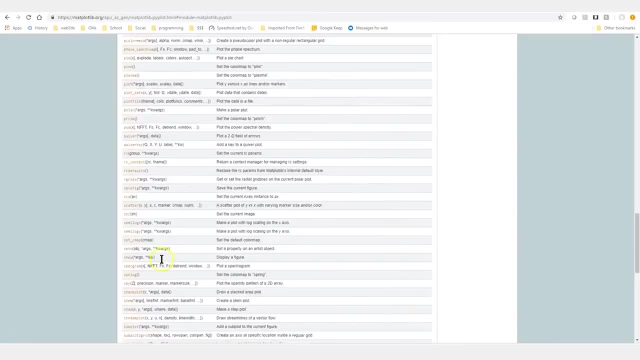 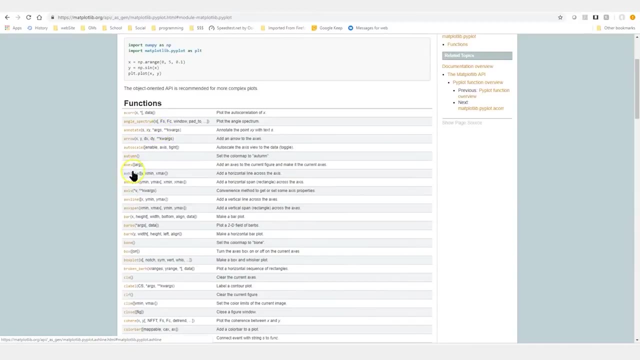 And you can see it's pretty extensive. We've covered all the basic ones so that you now have a solid ground to look at these different options. So when you come to these functions, some of them are going to look a little off or not off. 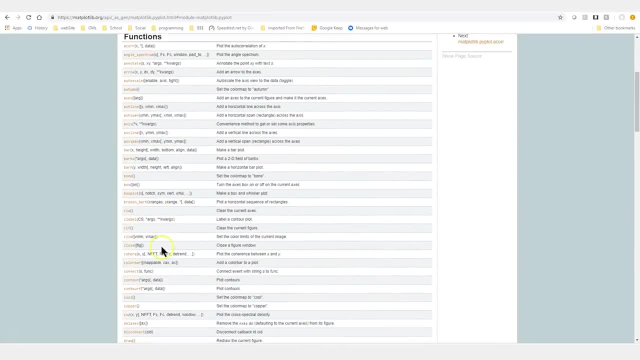 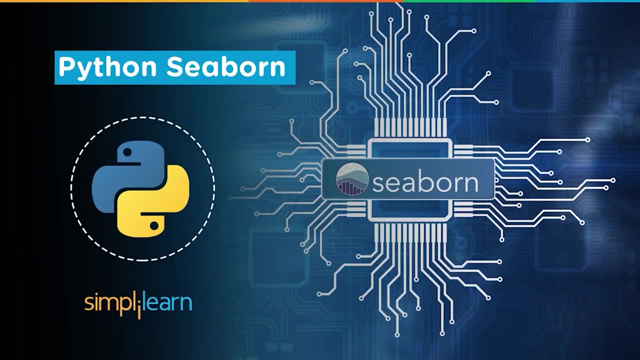 Some of them will look unfamiliar, but you'll still have the availability to probably understand most of this and have a basic understanding of your Matplot library. We will learn how to visualize data and draw insights with different charts and graphs using the Seaborn library. 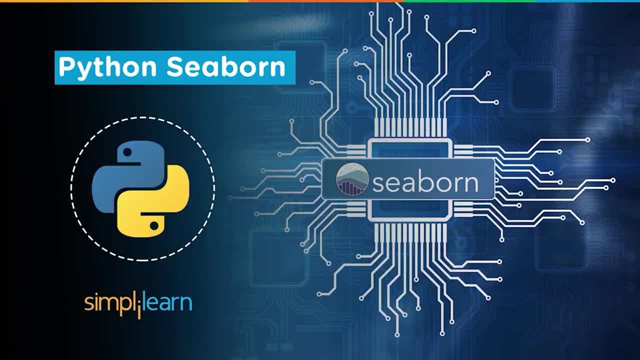 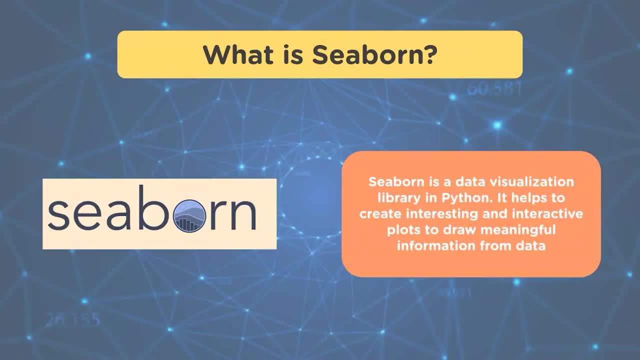 These visualizations are often referred to as plots in Python. So what is Seaborn in Python? The Seaborn library in Python is a widely popular data visualization library that is commonly used for data science and machine learning tasks. It is built on top of the Matplotlib data visualization library. 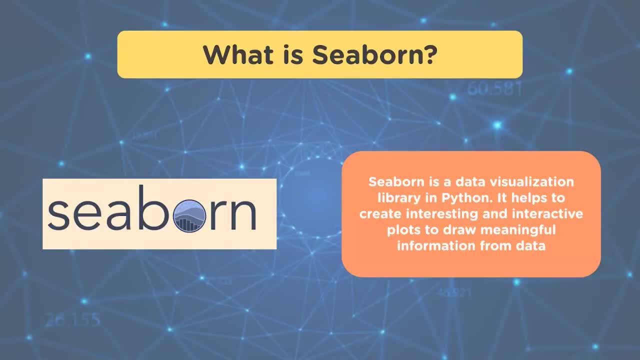 and allows you to perform exploratory data analysis. Using Seaborn, you can create interactive plots to answer specific questions about your data. It helps you find trends in your data that you can't notice just by looking at the data. Now to understand the Seaborn library in detail. 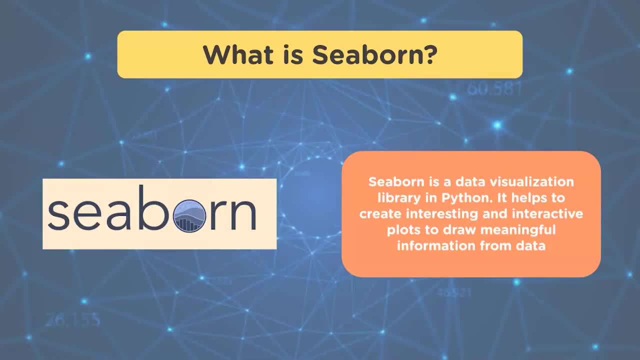 and how to create different plots and know the data better. we'll be using two datasets in our demo. The first one is the empty-cast dataset and the second is the popular iris flower dataset. Now let's head over to our Jupyter notebook. 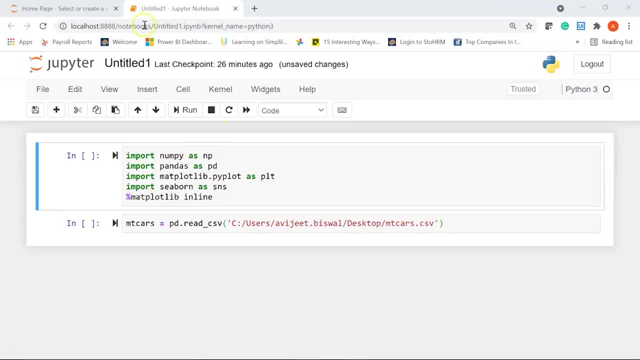 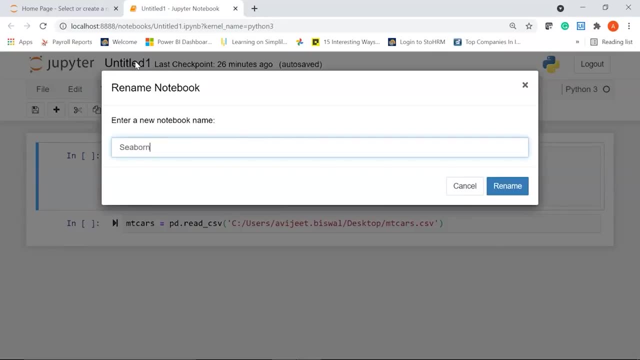 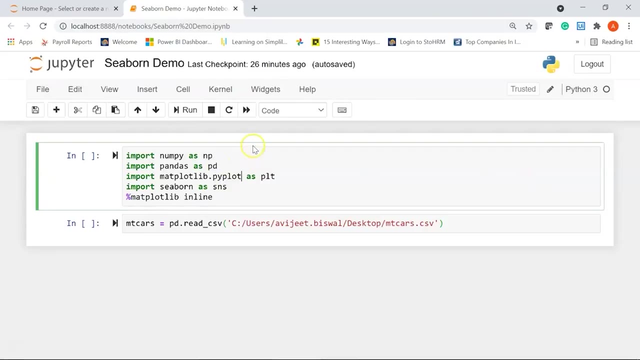 and start with our demonstration. So I am on my Jupyter notebook. Let me go ahead and rename the notebook. I'll say Seaborn demo. We'll rename it. Alright, You can see. I have the first two cells already filled in. 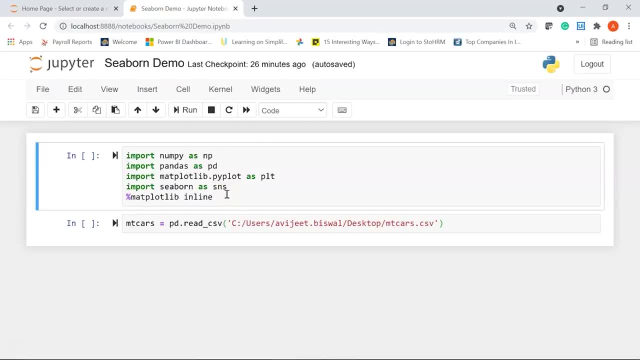 So while working on an exploratory data analysis project using Python, you will need numpy, pandas, matplotlib and Seaborn libraries for data manipulation and visualization. So let's import these libraries first. So I have already written: import numpy as np, pandas as pd, matplotlibpyplot as plt. 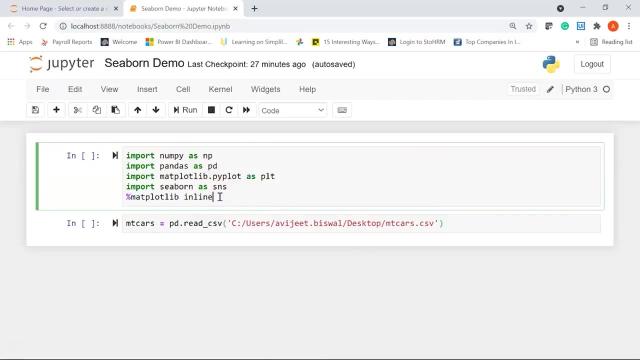 Seaborn as sns. Alright, So I'll hit shift enter to run this first cell. Alright. Now, using the read underscore csv function that is present in the pandas library, I am importing my dataset. that is mtcars. I'll tell you what mtcars is about. 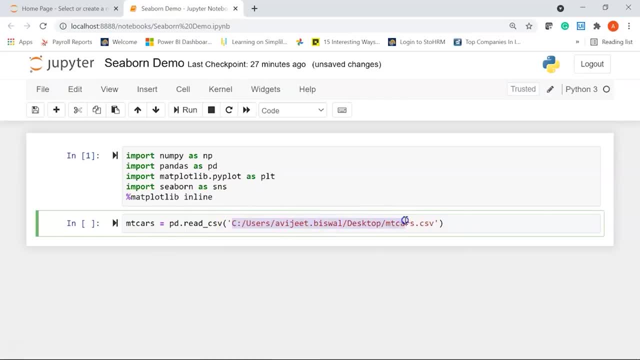 This is a csv dataset, and here I have given the location where my dataset is present. Let's run it Alright. Now let me go ahead and print the first five rows of my mtcars data frame. For that I am using the head function. 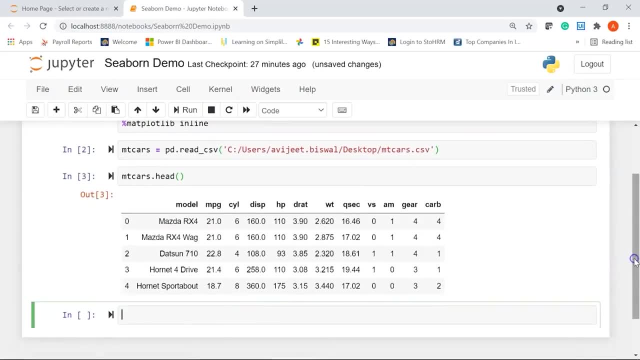 If I run it, okay, you can see here it has given me the first five rows. The index starts from zero till four, So total five rows of information and you can see these are the columns that are present in the mtcars dataset. 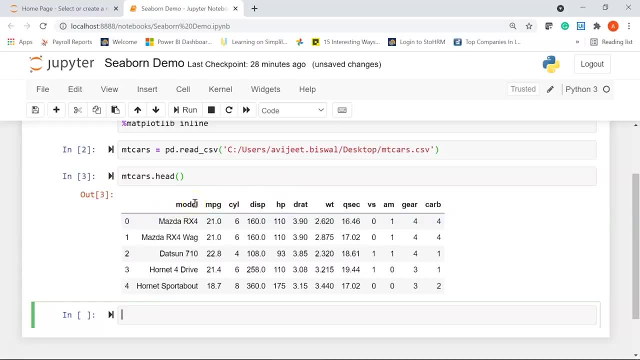 The first is the model of the car. Now just let me give you a background about this dataset. So the data is taken from the 1974 Motor Trend US Magazine. It has information about fuel consumption and 11 different aspects of automobile design and performance of 32 cars. 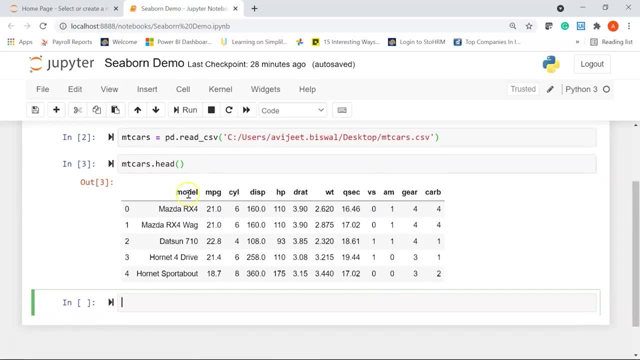 Alright. So here we have the first column as the model of the car, and then we have MPG, which is miles per gallon, Then we have CYL, which stands for the number of cylinders in the vehicle or the car, Then we have DISP, which is displacement. 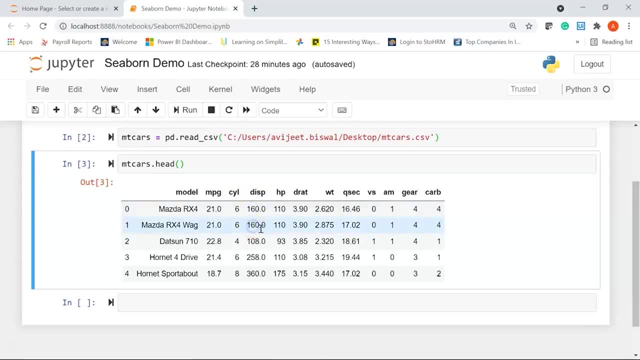 in cubic inches. So these all values are in cubic inches. After that we have HP, which is gross horsepower, Then we have something called as DRAT, which is basically the rear axle ratio. Then we have WT, which is the weight of the car in pounds. 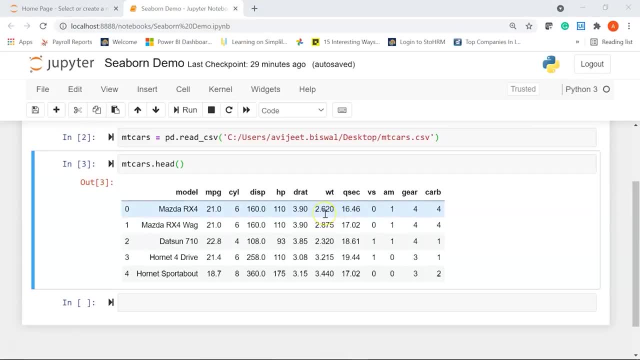 So think of it as weight multiplied by 1000 pounds. Alright. and then we have QSEC, which is one fourth mile time. This is a measure for acceleration. Then we have something called as VS. This is the type of engine for each of the vehicles. 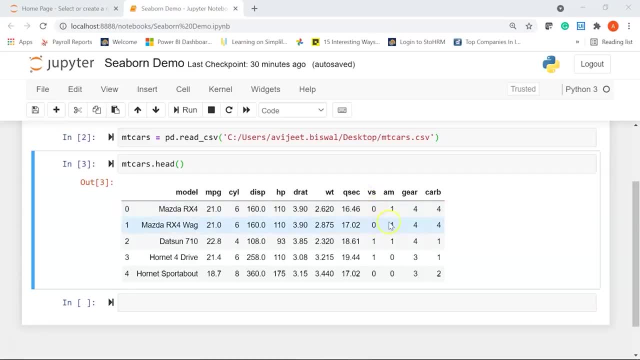 So 0 stands for V shaped engine and 1 stands for straight engine. Then we have AM, which is basically the mode of transmission. So 0 is for automatic transmission and 1 is for manual transmission. Then we have the number of forward gears. 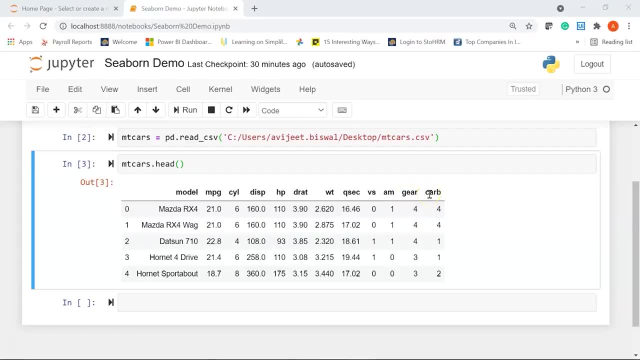 present in the vehicle. Then we have something called as CARB or C-A-R-B. This stands for the number of carburetors. So carburetors is a device for supplying a spark ignition engine with a mixture of fuel and air. Alright, 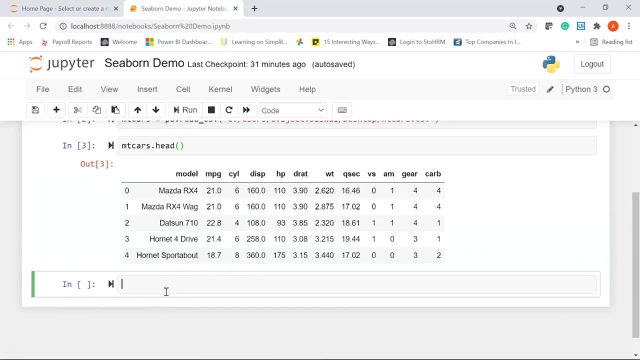 Now we will use the info function to print the summary of the data frame. So the info function returns information regarding the index data type column data types. Then we have the information about non-null values and memory usage. So I will write my data. 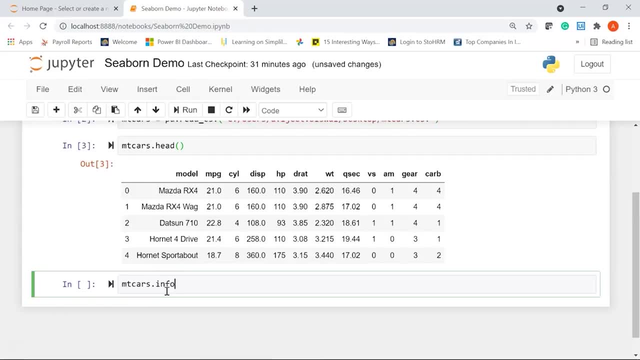 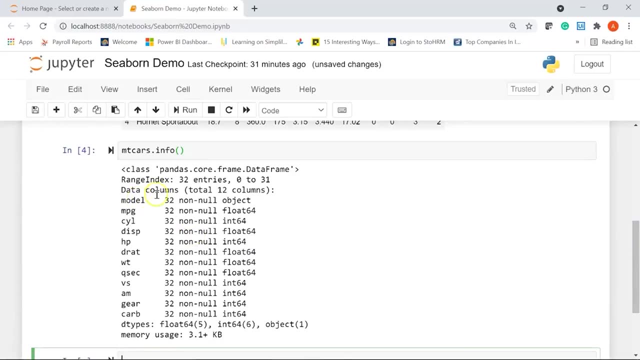 frame name, which is empty cars dot. I am going to use the info function. Let's run it and here you can see. we have all the columns. There are total 32 entries, from 0 to 31.. So data about 32 cars. Then here you. 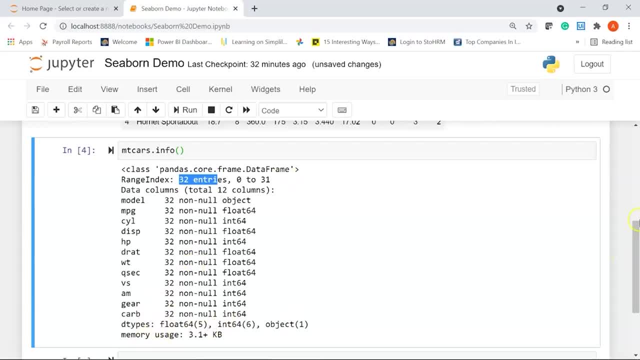 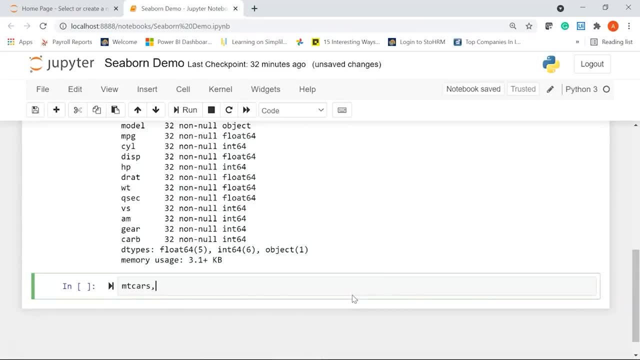 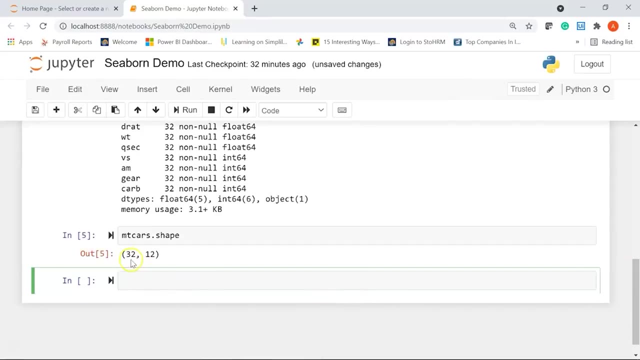 can see the data types and the memory usage. Now, moving ahead, let me just print the shape of the data frame. that will give you the number of rows and columns present. I will use the shape attribute. You can see here there are total 32 rows and 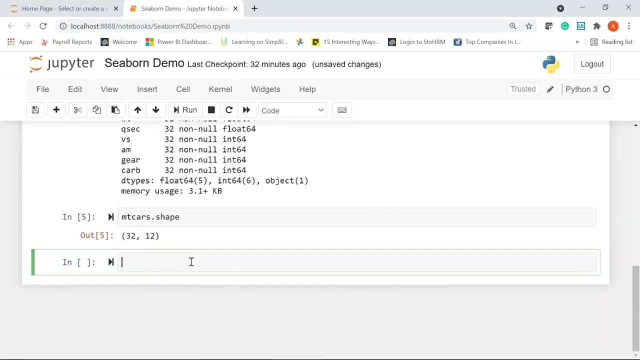 12 columns in my data set. Now the Seaborn library provides a range of plotting functions that makes the visualization and analysis of data easier. So we will cover some of the crucial plots that are available in Seaborn. So let's start. 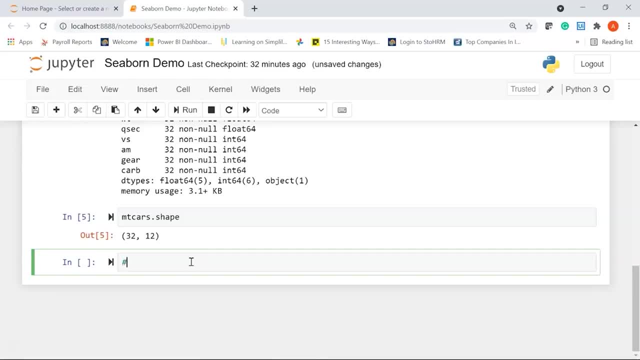 with a bar plot. I will give a comment as bar plot. Now, first understand what a bar plot is. So a bar plot gives an estimate of the central tendency of a numeric variable with the height of each rectangle. It provides some indication of the uncertainty. 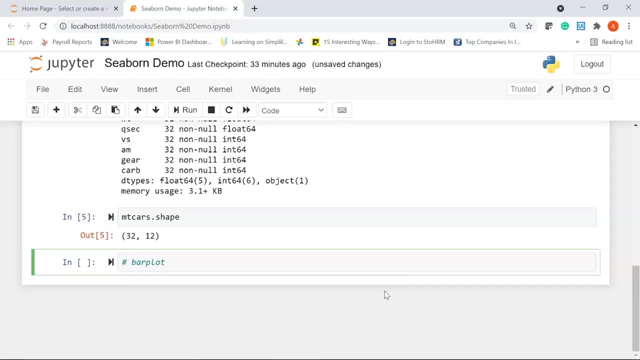 around the estimate using error bars. Now, to build this plot, you usually choose a categorical column in the x-axis and a numeric column on the y-axis, So we will create a bar plot between the number of cylinders and the miles per gallon. So let's start. 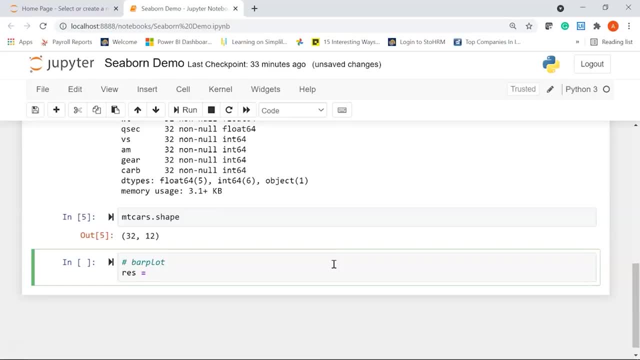 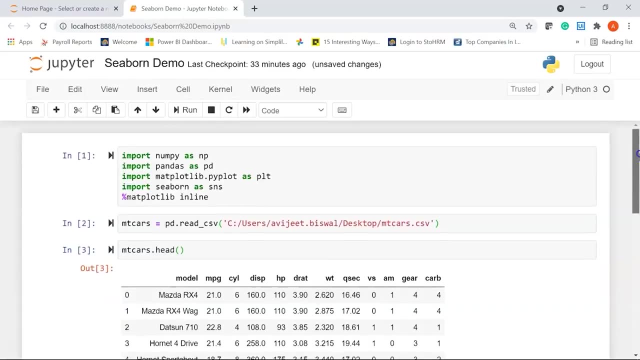 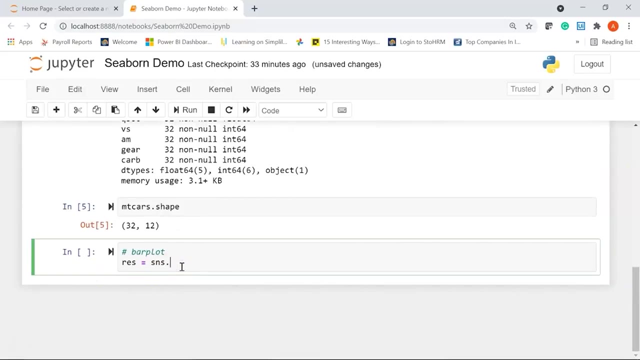 I will declare a variable called res, which essentially stands for result. Then I will use sns, which is for the Seaborn library. I will say sns dot, followed by my bar plot function and inside the function I will pass in my data frame name that is, empty cars. 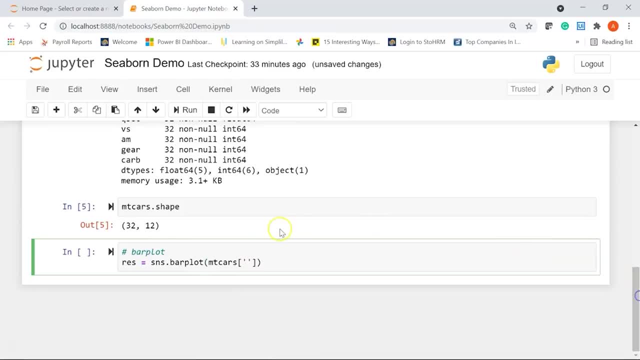 and then for x-axis, within the bracket, using quotation, I will give my column name as cylinder. So this is going to be my x-axis and for y-axis I will say my data frame name- empty cars, then square bracket, followed by my y-axis column. that is miles per. 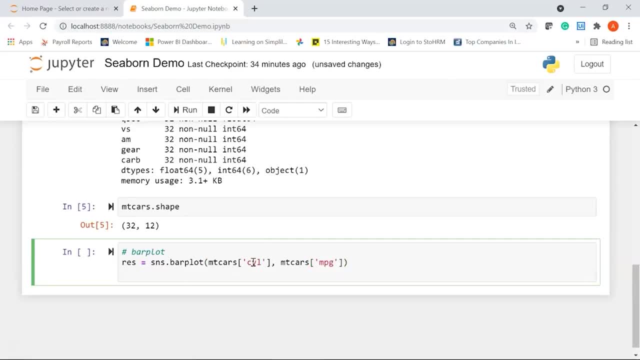 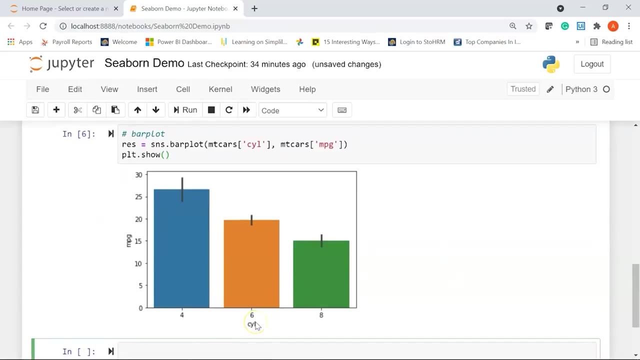 gallon. Now to display, I am going to use the matplotlib function. I will say plt, dot, show. Let's run it and we will see the result. There you go. So here you can see. on the x-axis we have the number of cylinders. So in our data we have 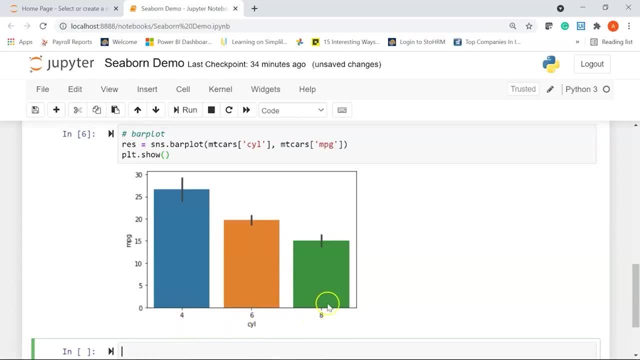 vehicles with 4, 6 or 8 cylinders, and on the y-axis you can see the miles per gallon. Now what essentially this graph tells us is that when the number of cylinders in the vehicle increases, my miles per gallon or mpg for the vehicles. 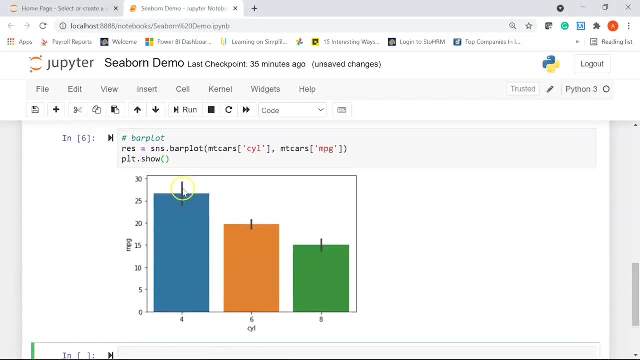 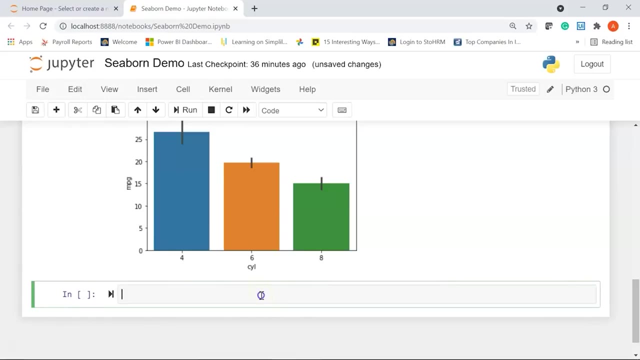 decreases and you can see these black lines. So these lines indicate the uncertainty around the estimate using error bars. Alright, Now you can create the same barplot using another way. Now we will exclusively define the x and y-axis columns and also pass the name of the. 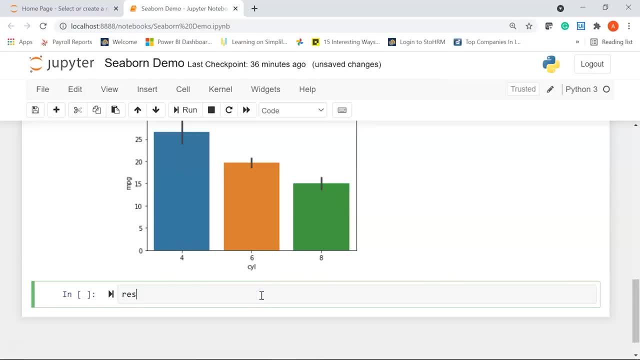 data frame using the data argument. Let me show you how to do it. I will use the same variable name res, which stands for result. I will say sns dot barplot. Now, inside the barplot function, I am going to exclusively define my x-axis. 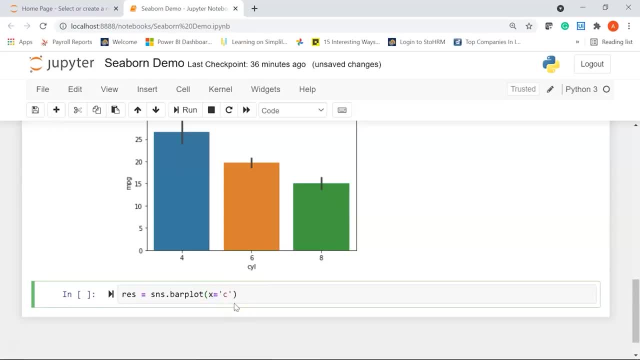 I will say x, equal to, I will pass in my column as cylinder. then I will say y-axis, which is miles per gallon, and then, using the data attribute, I will pass in my data frame name that is empty cars. and finally we will write plt dot show. 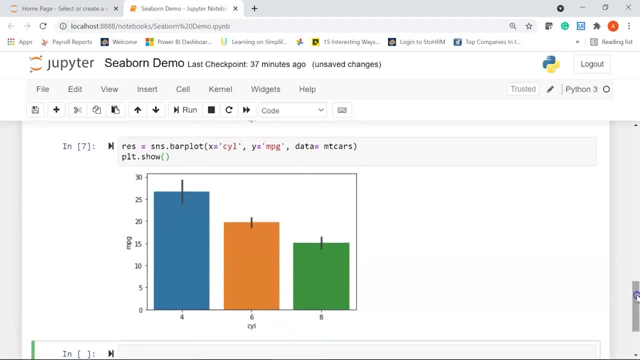 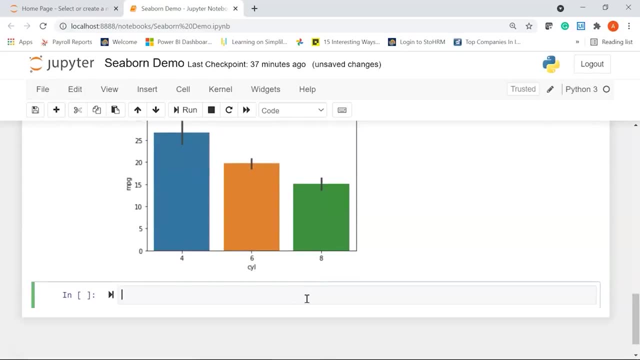 Let me run it. You see, here we have the exact same barplot as the above one, So this is another way to create a barplot. Now, python cbon allows the users to assign colors to the bars, So the bar chart that we are going to create. 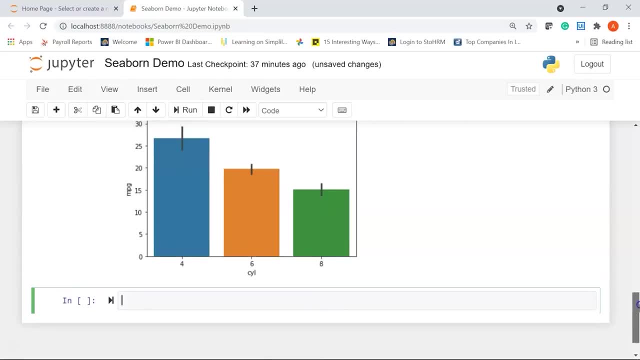 will convert all the bars to a particular color. So for that I am going to use the color argument. So I will say: res equal to sns, dot, my function, that is barplot. I will say x equal to cylinder, my y-axis will have mpg. then I will say: 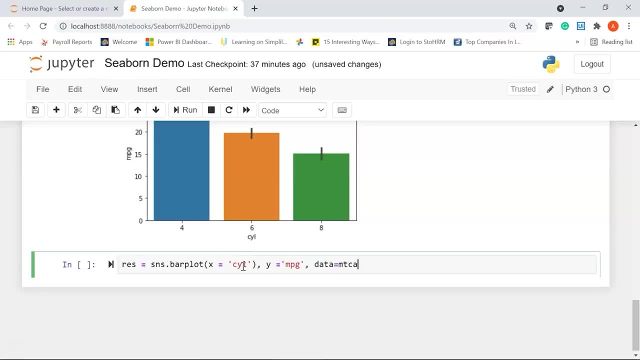 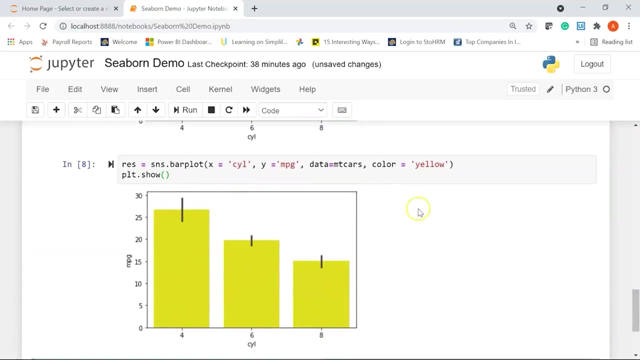 data is empty cars. give a comma and my final attribute: I will say color equal to. I will say yellow, close the bracket and and then I am going to write plt dot show. If I run it, you can see here: all the bars have been converted to yellow color now. 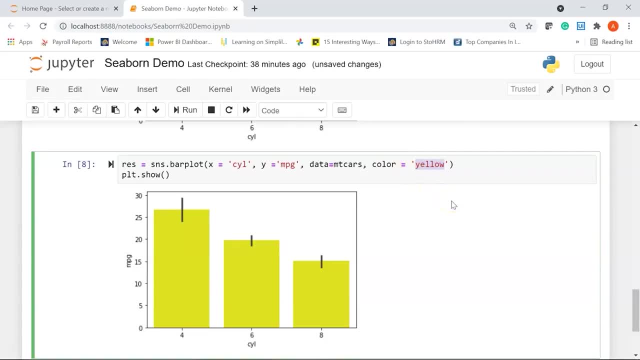 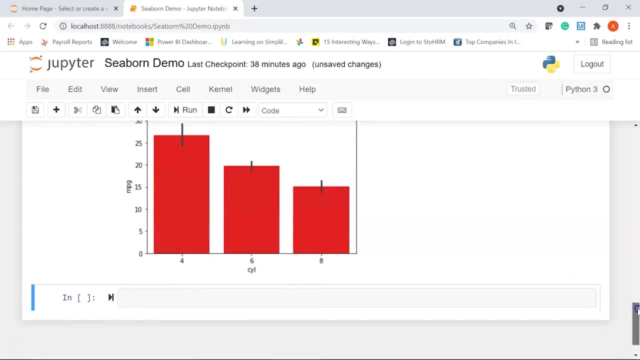 You can change the color argument. Let's say, I will make it to red If I print it. you can see here: all the bars have been changed to red color now. Alright, Now cbon library also has the palette argument, which you can use to give different colors to the bars. 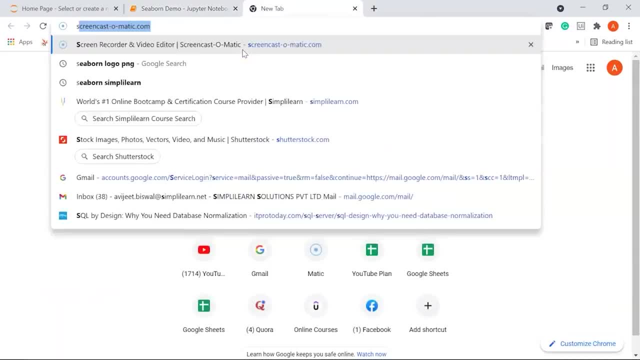 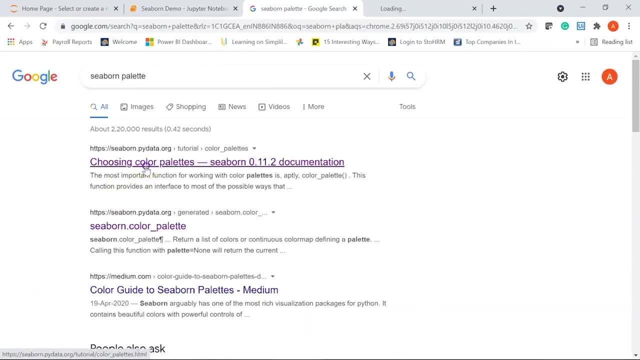 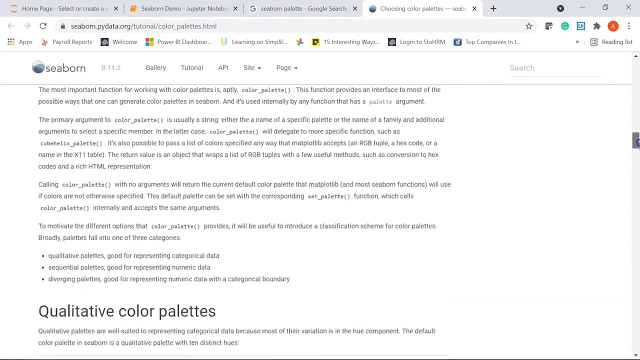 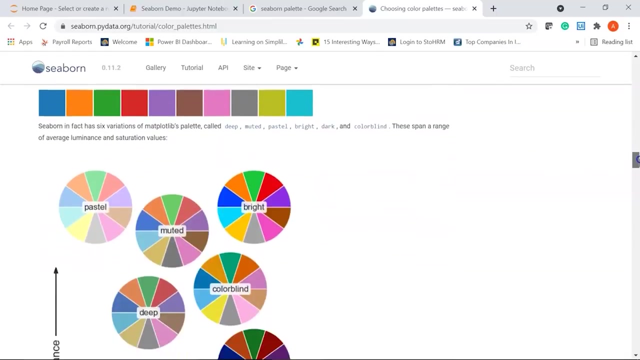 So if you go to Google and search for cbon palette, You have a nice link here. So here you have. there are different palettes provided by cbon. you can see here sns dot color palette and these are the names of the palette. You can use whichever palette you want. 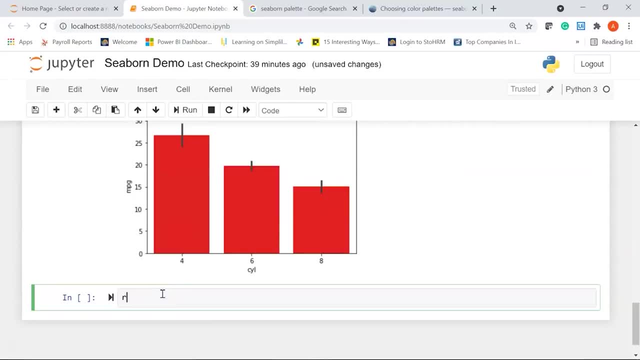 Alright, So I will say res equal to sns dot bar plot. We will use our first method of assigning a bar plot, So I am using my data frame: empty cars. This time we are going to change the x and y labels. Let's say I am using my x label as: 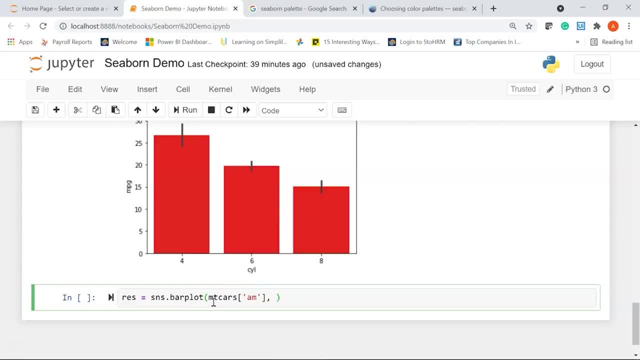 transmission, whether automatic or manual transmission, and then in my y axis I will have miles per gallon. Then I am going to say: palette equal to. I made a spelling mistake here. Let's say: our palette is set to. this is the name of the palette I will write. 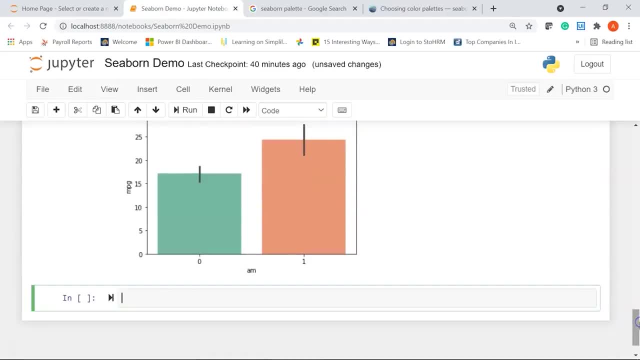 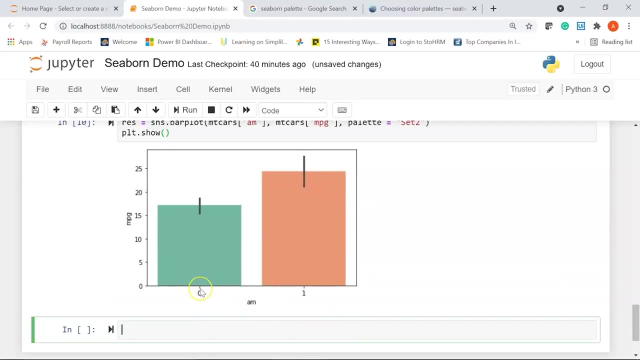 plt dot show. If I run it, you can see. here we have the two modes of transmission: 0 is for automatic transmission of the vehicle, 1 is for manual transmission and you can see the miles per gallon for each of the modes of transmission. If you want, you can change the. 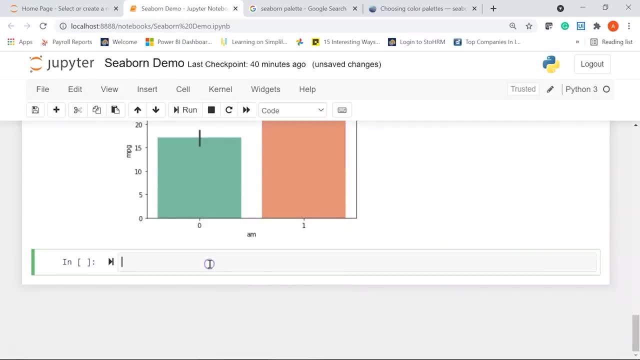 palette colors. let me just copy this. I will paste it in my new cell and instead of set to, let's say we will use another palette called as rocket, and I am also going to alter my x and y labels. Let's say, in my x label I will have 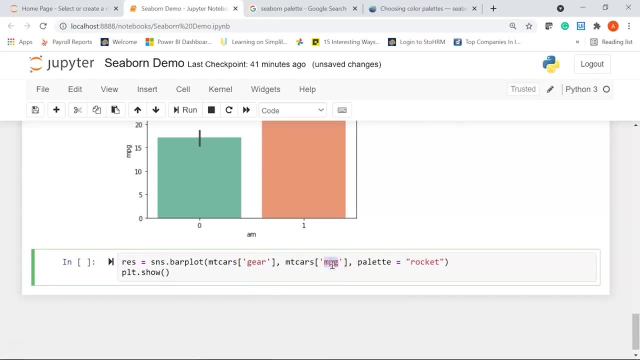 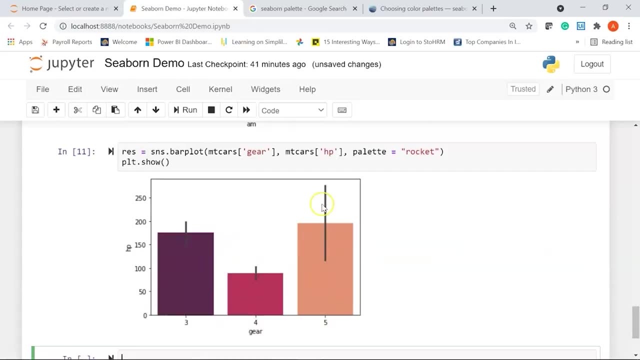 gear and my y label will be horsepower, If I run it, we now have a different palette and the bars are of different colors. On the x axis you have the gears 3 gear, 4 gear or 5 gear vehicle, and on the y axis you have the horsepower. 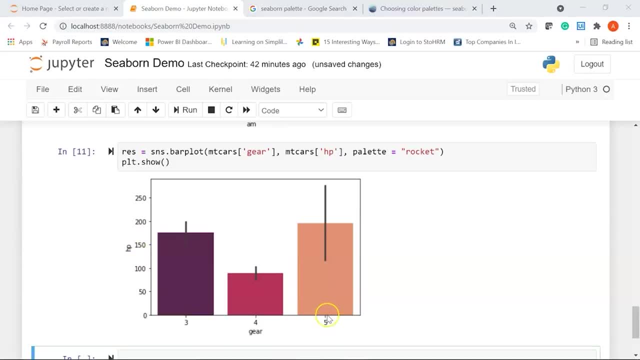 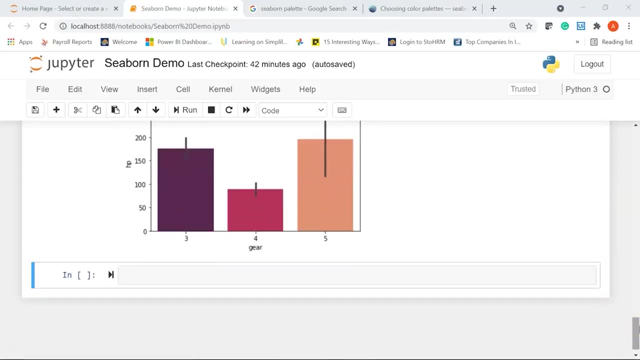 So from the graph you can see the horsepower is low for vehicles that have 4 gears, while it is high for the vehicles that have 5 gears. Now let's understand how to create a count plot. So the count plot function in the python seaborn library returns the count of. 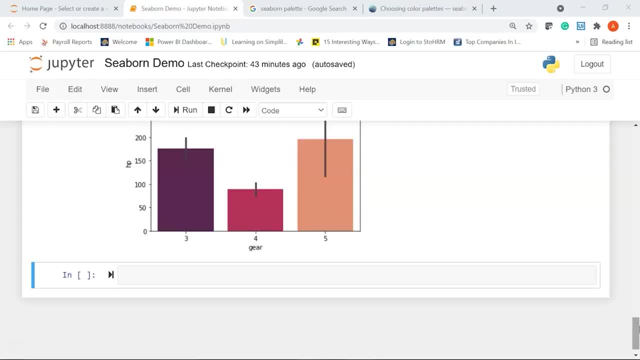 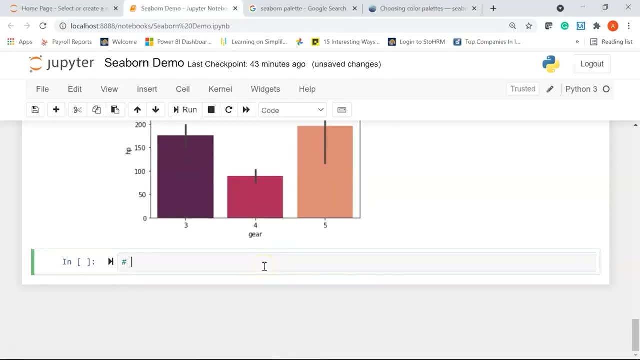 total values for each category using bars. We will create a count plot that returns the total number of vehicles for each category of cylinders. I will just give a comment here as count plot. Alright, So I will start sns dot. I will use the count plot function and I will define. 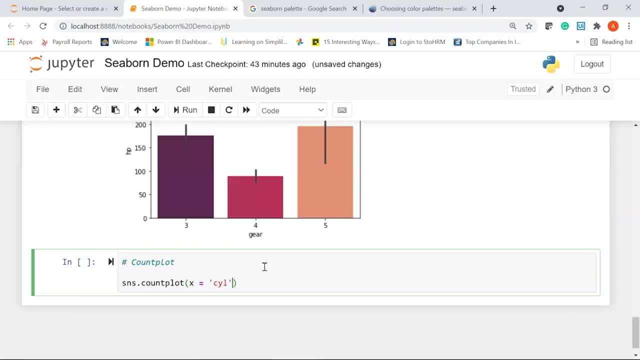 my x axis as cylinders. My y axis won't have any label or any column because y axis will only show the count. Then I am going to use my data parameter or the argument and pass in my data frame name that is empty cars. Let's say I will set the 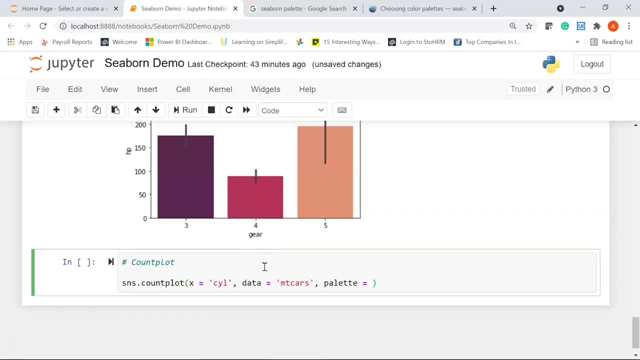 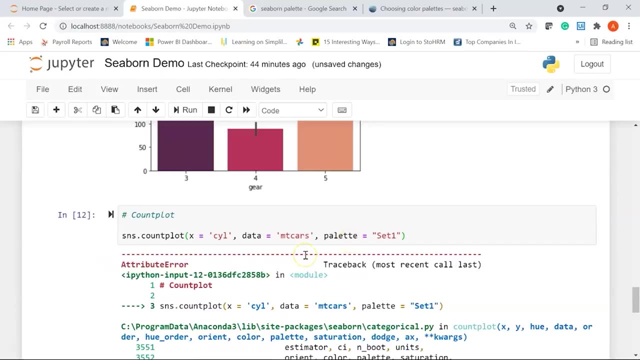 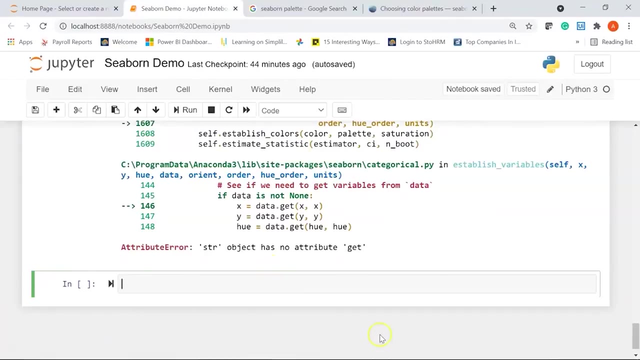 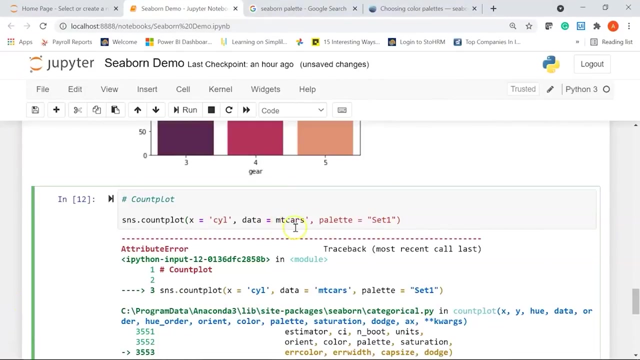 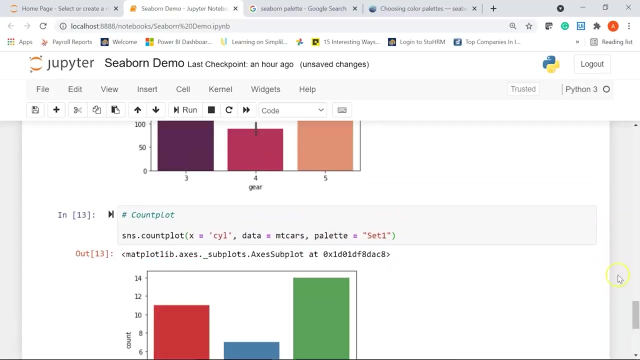 palette to set one. Let me run it. Okay, there is some error. let's debug the error. It says str object has no attribute get. Okay, So this should be without the single quotes. Make sure the data frame name is without the single quotes. Let's run it again. 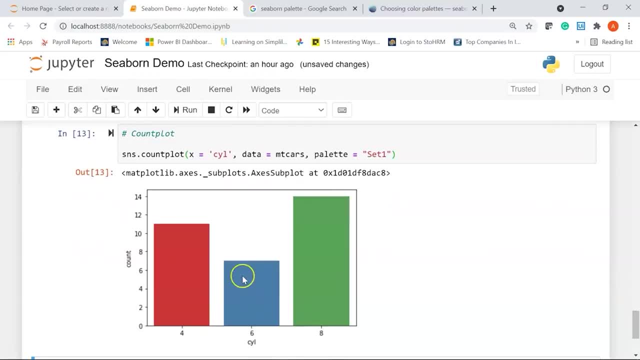 There you go, So you can see here. this is a nice count plot that shows the number of cylinders on the x axis and on the y axis. you have the count. you can see here there are more number of vehicles that have 8 cylinders and there are. 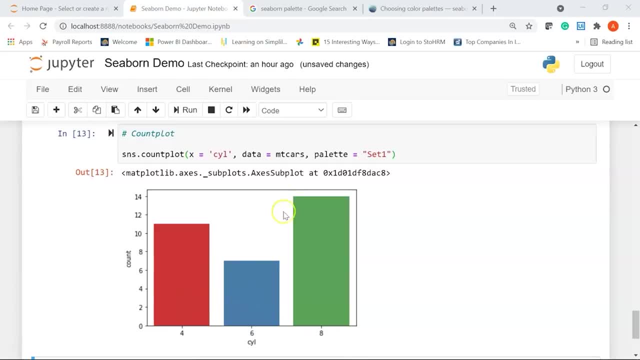 less number of vehicles or cars that have 6 cylinders, and actually you can count it as well. So you can see here there are 14 cars that have 8 cylinders, there are 11 cars that have 4 cylinders and there are 7 cars that have 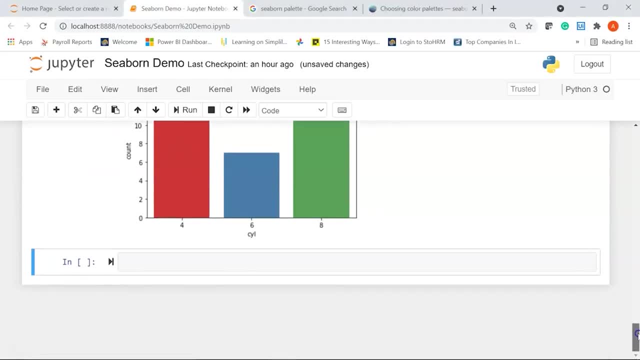 6 cylinders. Alright, Now moving ahead. the next count plot will show the number of cars for each carburetor. So for that I am going to say sns count plot. my x axis will now have the variable carburetor. I will see data equal to: 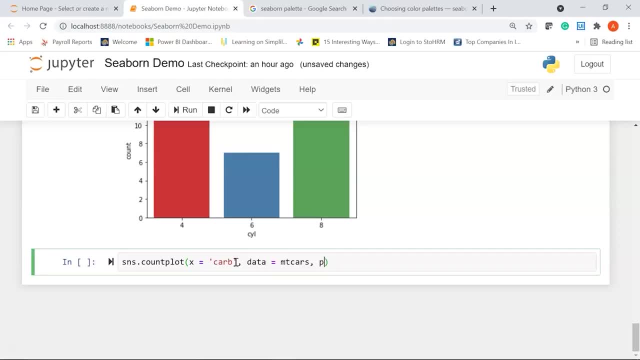 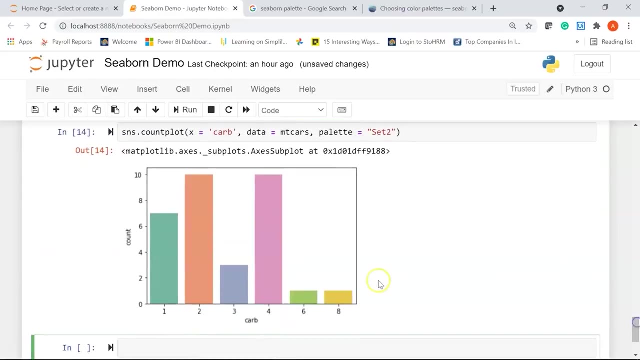 empty cars and my pallet. I will set it to set 1 or let's say set 2. Now let me run it. you can see it here. on the x axis we have the different number of carburetors: 1,2,3,4,6 and 8. 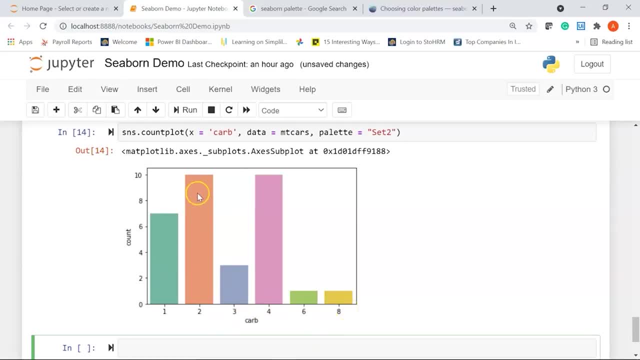 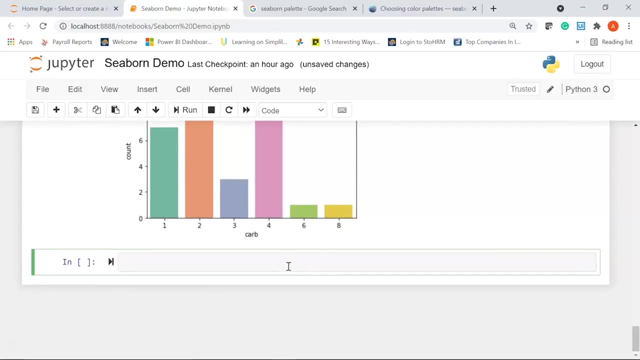 and you can see we have more number of cars that have 2 and 4 carburetors and there are very few vehicles that have 6 and 8 carburetors. Cool, Now moving ahead. So the python seaborn library allows you to create horizontal count plots. 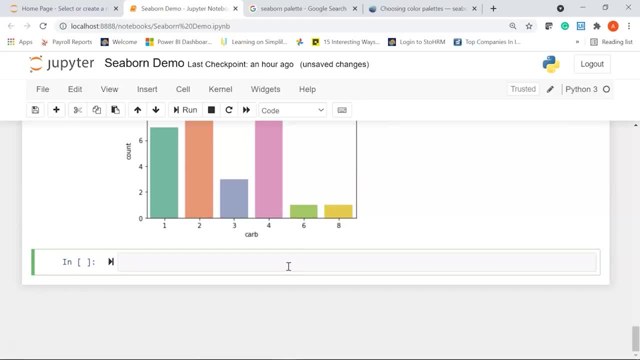 where the feature column is on the y axis and the count is on the x axis. Let me show you how to create a horizontal count plot. I will say sns dot count plot. I am going to define my y label or the y axis as gear. I will say data equal to. 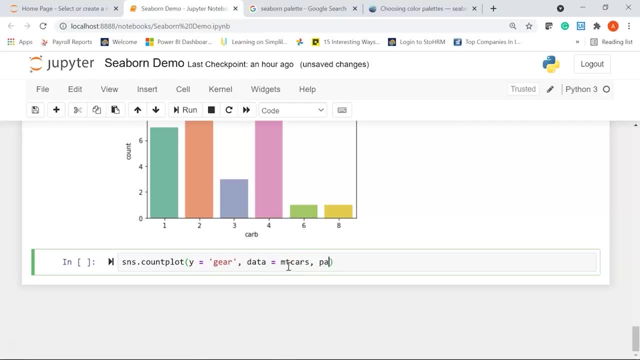 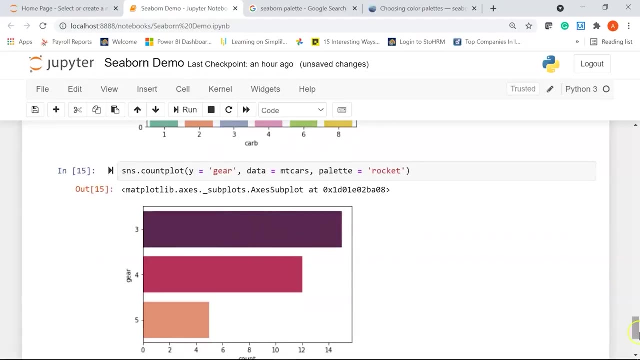 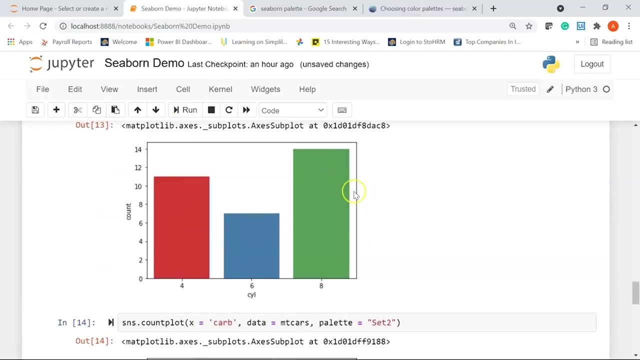 empty cars and set my pallet to, let's say, rocket, Let me run it. ok, you see here this is a horizontal count plot. if you compare it with the above one, these were all vertical count plot as in the bars were vertically aligned, but here you can see the bars are all. 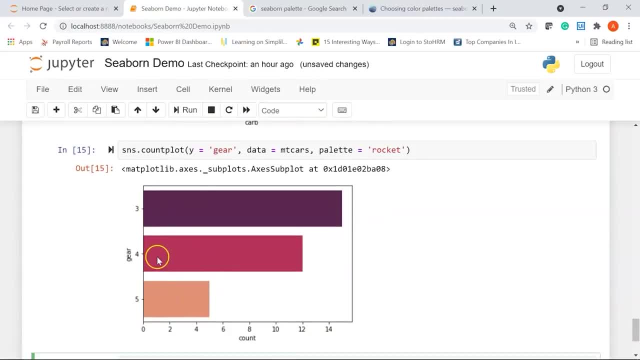 horizontally aligned and on the y axis you have the gear column and on the x axis you have the count. so if you mark here properly you can see there are 15 vehicles with 3 gears, there are 12 vehicles that have 4 gears and there are total 5 vehicles with. 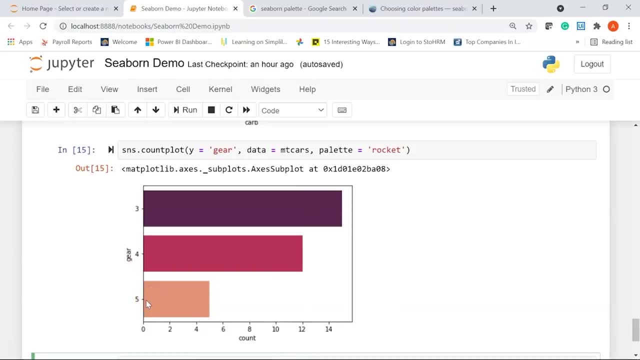 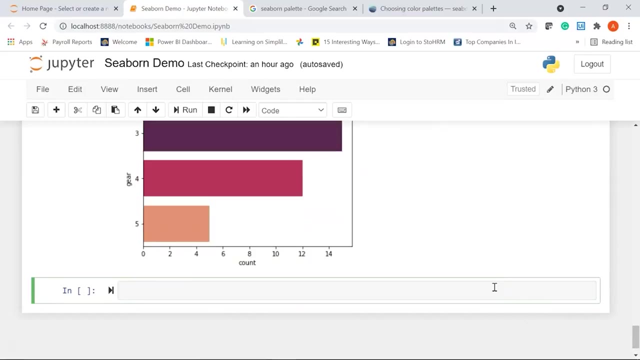 5 gears. now you can also create a grouped count plot using the hue parameter. so the hue parameter accepts the column name for color encoding. now let's build a count plot that shows the number of cars for each category of gears, grouped by the number of cylinders. 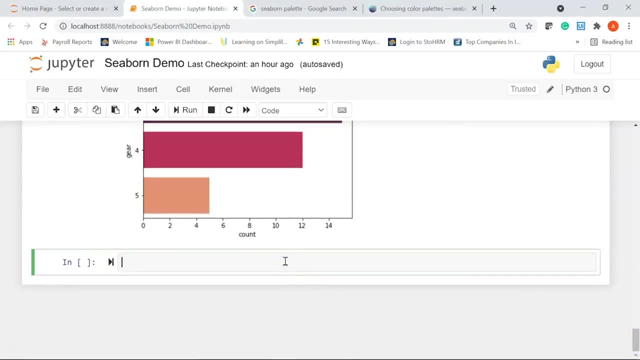 so we are going to group based on the number of cylinders. let me show you how to use the hue parameter. for that I will say sns, dot, count plot. in the x axis I will have my gear column. then I am going to pass my hue parameter. that will have the 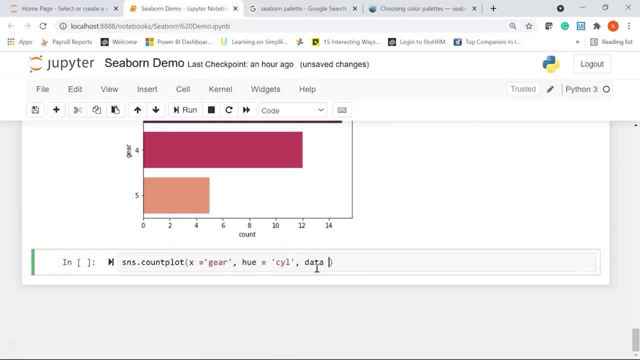 cylinder column or the number of cylinders for each vehicle. I will pass my data frame using the data argument as empty cars and say pallet. I will set my pallet to set 1. let's run it. if I scroll down you see here we have a count plot. 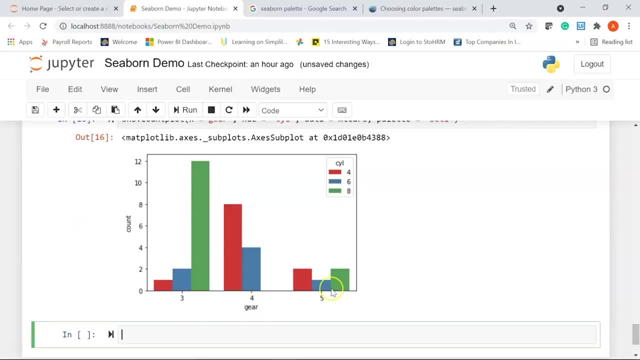 on the x axis you have 3,4 and 5 gears of the different vehicles and for each gear you have the bars that represent the number of cylinders. so for vehicles that have 3 gears, we have majority of the vehicles having 2 cylinders. similarly, for 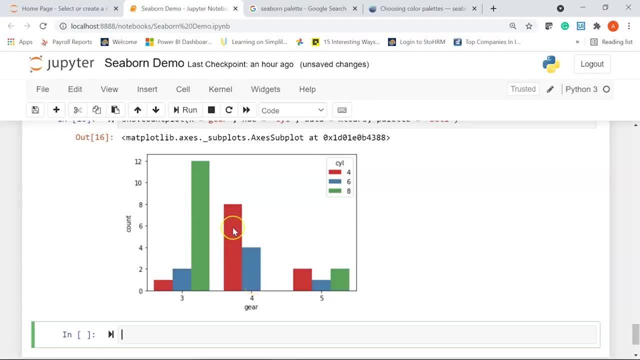 vehicles that have 4 gears. we have most of the vehicles with 4 cylinders and if you compare for the cars that have 5 gears, so we have equal number of vehicles that have 4 and 8 cylinders, and then we have 1 vehicle that has 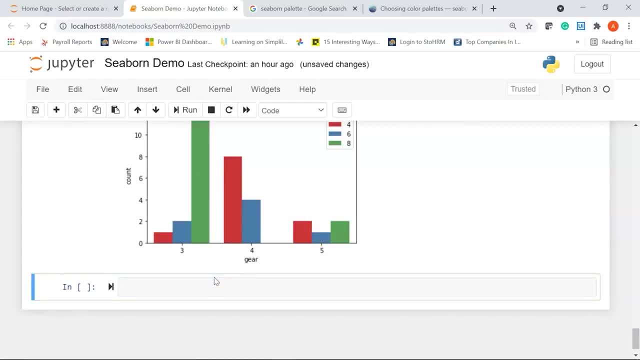 6 cylinders. cool, now moving ahead. so the seaborn library supports the distplot function that creates the distribution of any continuous data. let's create the distribution of miles per gallon of the different vehicles or the cars. the mpg matrix measures the total distance the car can travel. 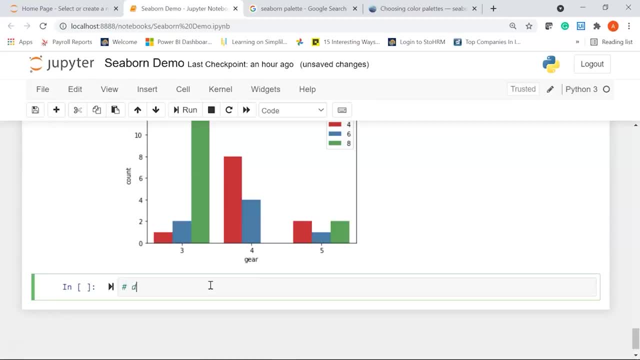 per gallon of fuel. so here I will give a comment. as distplot, which stands for distribution plot, I will say sns dot distplot. I will pass in my data frame name that is empty cars. give a period and say mpg, which is my column name. then I am. 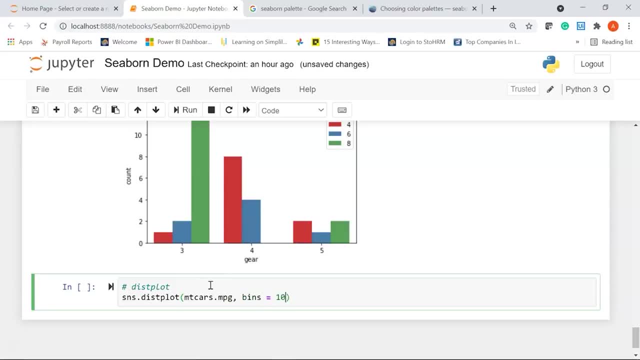 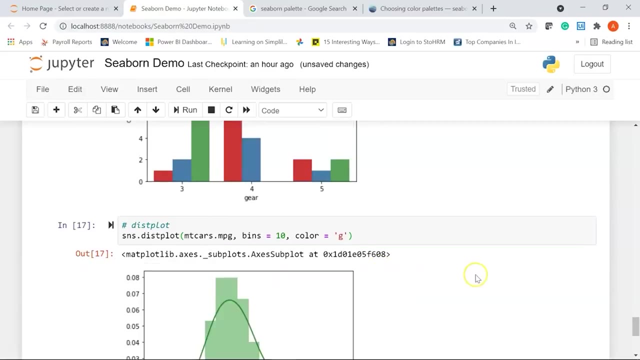 going to define the number of bins that I want. let's say 10. and then I will use the color argument and I will say: let's say g, which is for green. let's run it now. there you go. if I scroll down, you can see we have a nice. 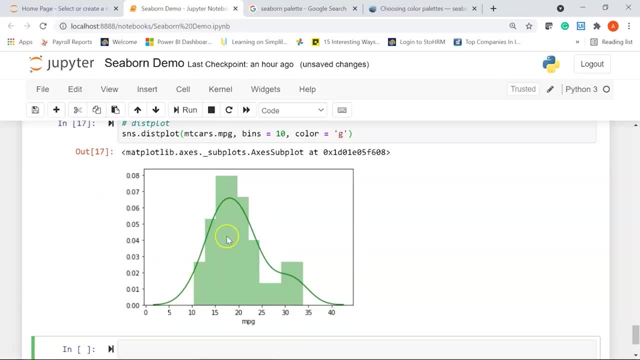 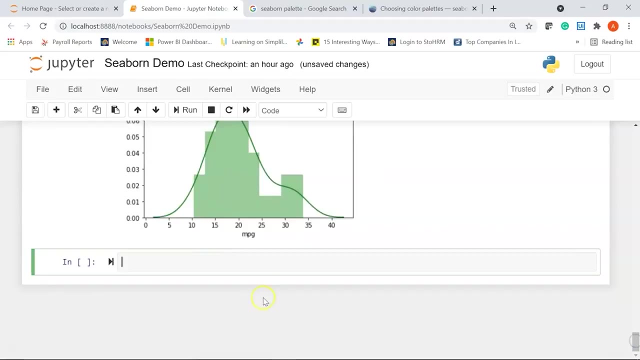 distribution plot. so these are all histograms and you can see we have a smooth curve and this shows the distribution of miles per gallon that is present in our data set. alright, now moving ahead, you can also create heat maps using the seaborn library. so the heat maps will. 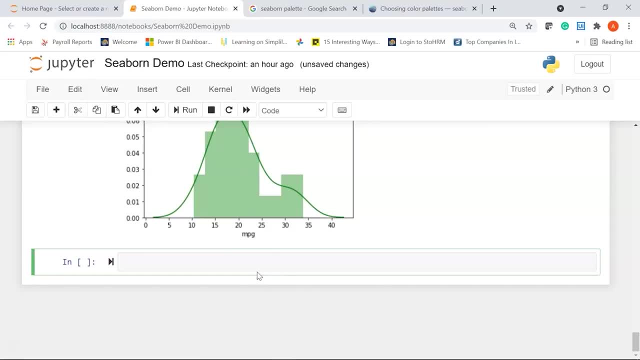 let you visualize matrix like data, the values of the variables are contained in a matrix and are represented as colors. you can create a correlation heat map, which is a graphical representation of a correlation matrix representing the correlation between different variables. so in our example, we will create a heat map where you can. 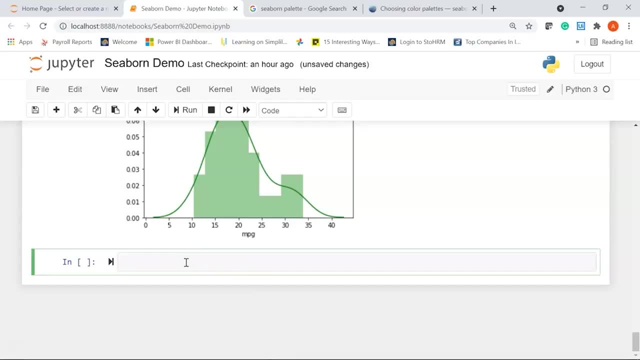 find the correlation between each variable in the empty cars data set. just give a comment. as heat map, I will say sns and I will use the heat map function. I will pass in my data frame name, that is empty cars, followed by my function called corr, which is for: 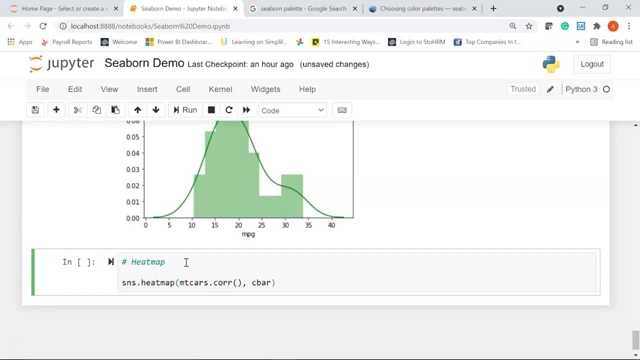 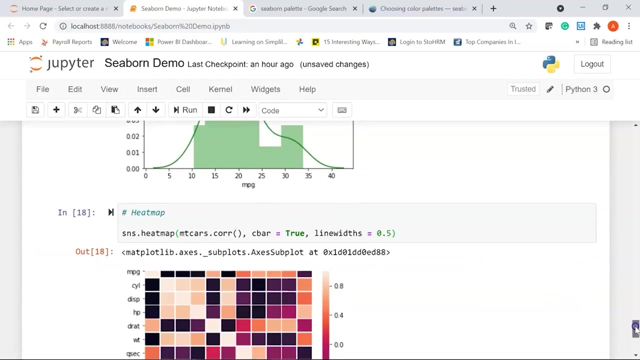 correlation. then I will say: cbar is equal to true, so the cbar argument is used to draw the color bar. then I will say line widths. I will pass it as 0.5. let's run it. there you go here. you can see, we have a nice heat map. 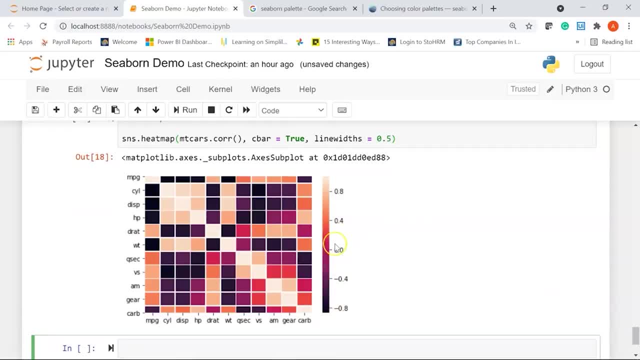 and on the right side you can see the color bar that starts from minus 0.8 and goes up to plus 0.8. so this ranges between minus 1 and plus 1 and the bars, or the bars you can see- that have a lighter color. 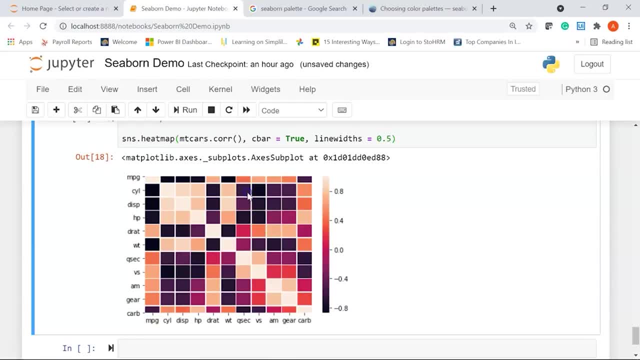 have a positive correlation and the ones that are dark have a negative correlation. so for example, you can see here for cylinder and mpg the color is really dark, which is around this region minus 0.8. this means when the number of cylinders in the car increases, your miles. 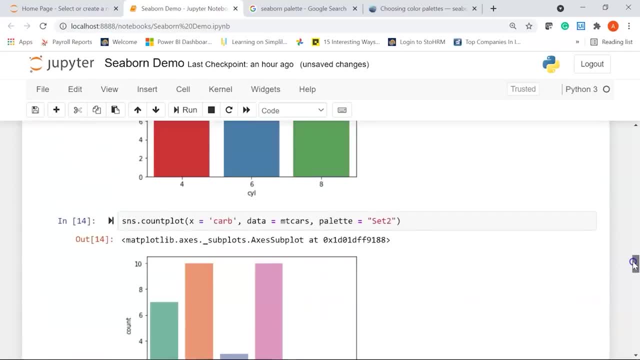 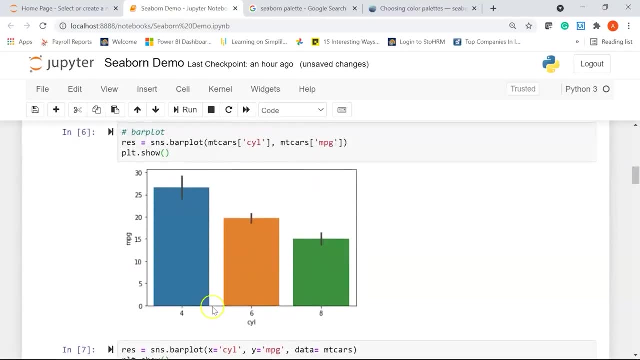 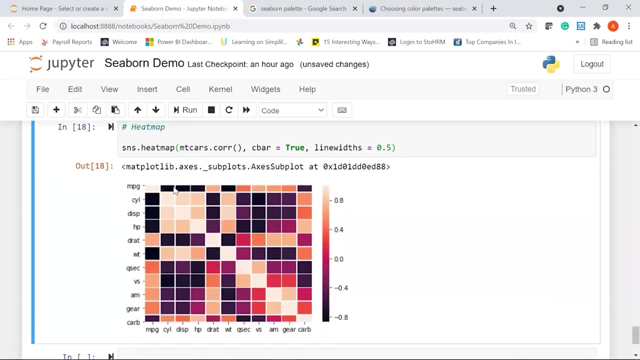 per gallon decreases, and this we also had seen in our first bar plot, this one you can see here: whenever the number of cylinders increased, your miles per gallon had decreased, and this is what has been depicted in our correlation map or the heat map. but if you see for 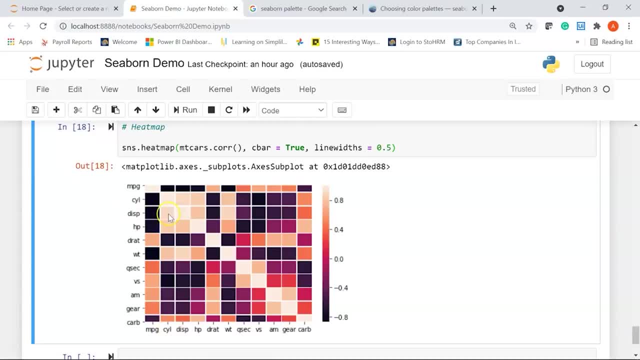 cylinder and displacement, there is a positive correlation which comes around this color bar range. similarly, there are other features in the data set. for example, if you compare for the weight of the vehicle and the number of cylinders, there is a positive correlation which means when the weight of the vehicle increases, the number of 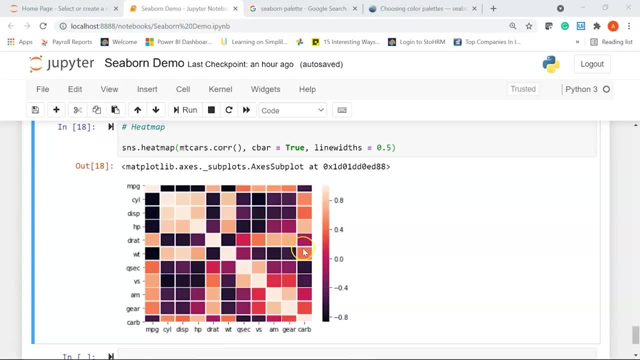 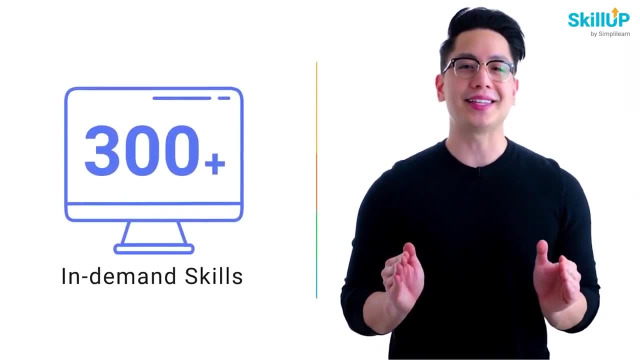 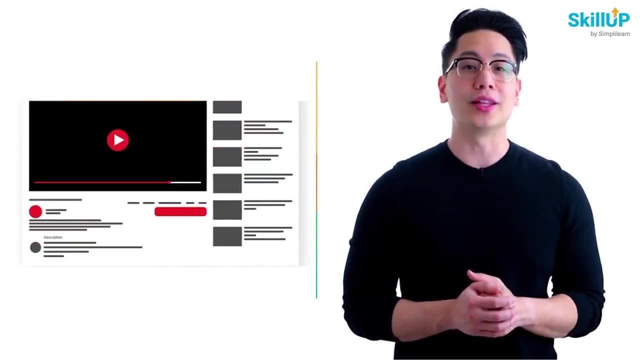 cylinders present in the vehicle also increases, and the others? you can also compare and find out the correlation based on this color bar. choose from over 300 in demand skills and get access to 1000 plus hours of video content for free. visit skillup by simply learn. click on the link in the 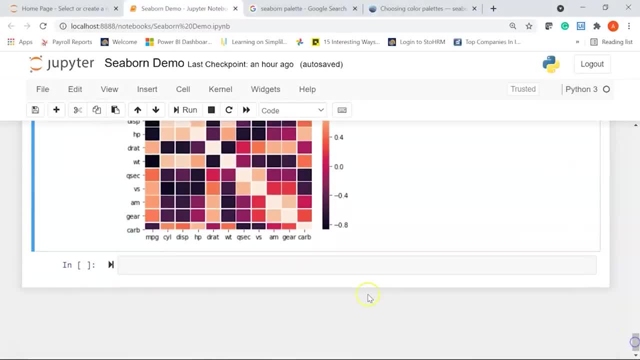 description to know more. ok, now let's move ahead. the seaborn scatterplot function helps you create plots that can draw relationships between two continuous variables. so to understand about scatterplots and other plotting functions, henceforth we are going to use iris plot data set, so let's go ahead. 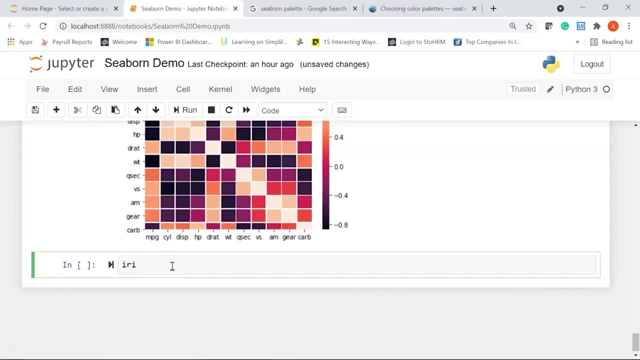 and load the iris plot data set. i will say irish equal to sns, dot, load underscore data set. so this iris plot data set is already inbuilt into the sns or the seaborn library. now we will go ahead and print the first 5 rows from the data set. 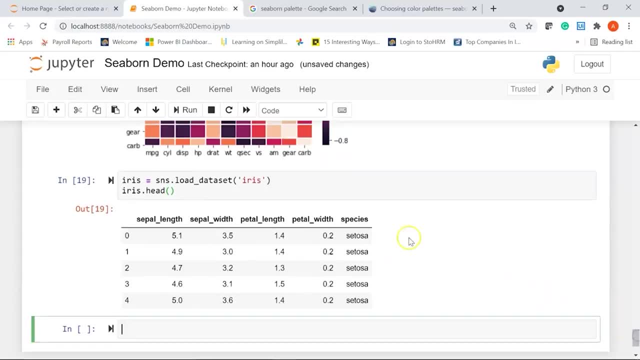 there you go, here you can see here there are total 4 feature variables. you have the sepal length, sepal width, petal length and petal width of the 3 species of flower, that is, setosa, virginica and versicolor. so, using this data set, 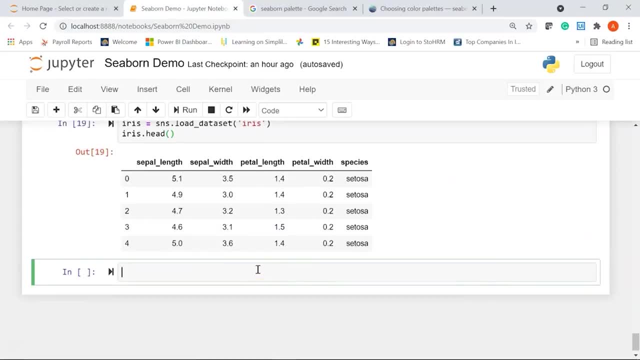 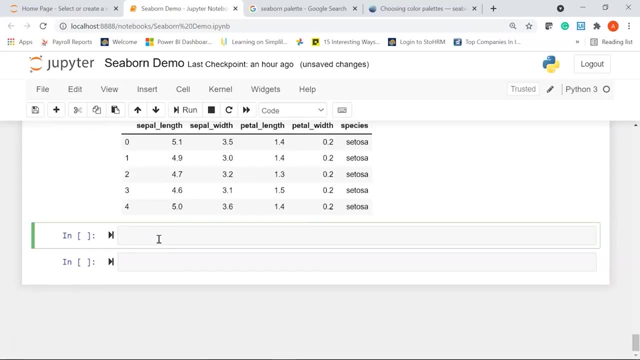 we are going to see the rest of the seaborn plotting functions. first let me go ahead and print the different species of flower and the count for each of the species of flowers that we have in our data set. i will say iris within square brackets. i will pass in the 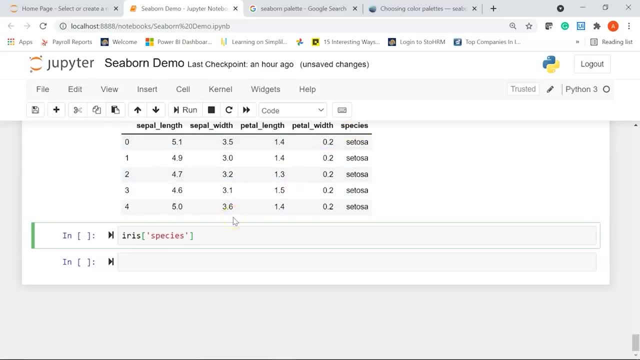 output, or the target variable, that is species, and i will use the function that is value underscore counts. let's run it. there you go. so we have 50 flowers of setosa type, again 50 flowers of versicolor species, and then we have another 50 flowers of type virginica. 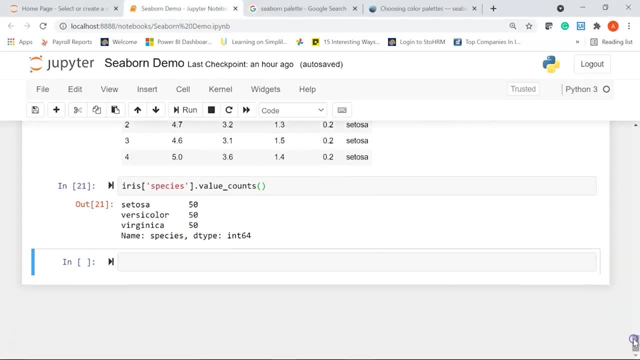 so there are total 150 flowers present in our data set. alright, now we will create a scatter plot to show the relationship between sepal length and petal length for different species of iris flowers. so i will say sns, dot, followed by the scatter plot function. in the x axis i will say: 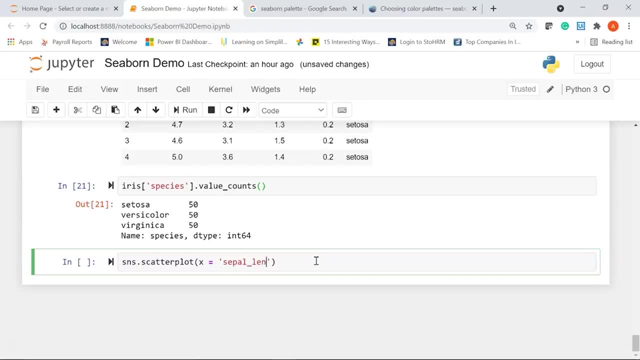 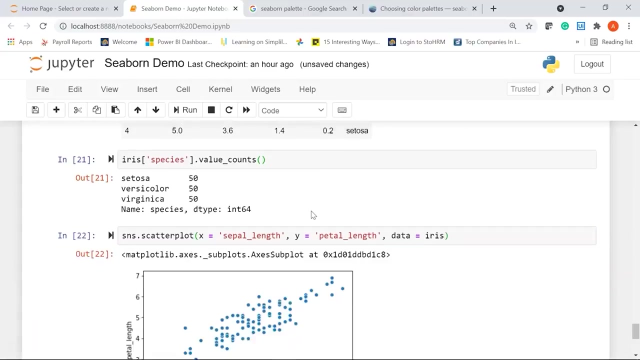 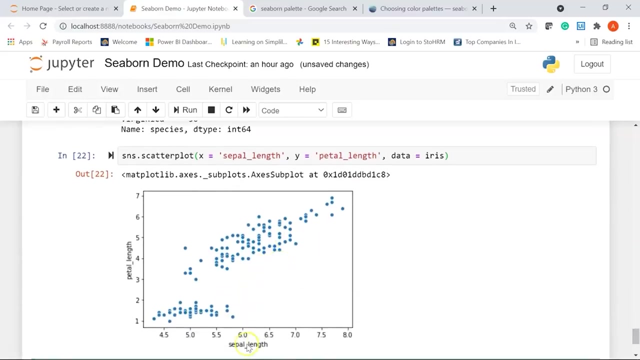 sepal length column. give a comma. i will pass in my y axis with petal length. then i will say: data equal to iris. now let's run it. you can see here: this is my scatter plot between sepal length and petal length. now you can classify the different species of flowers. 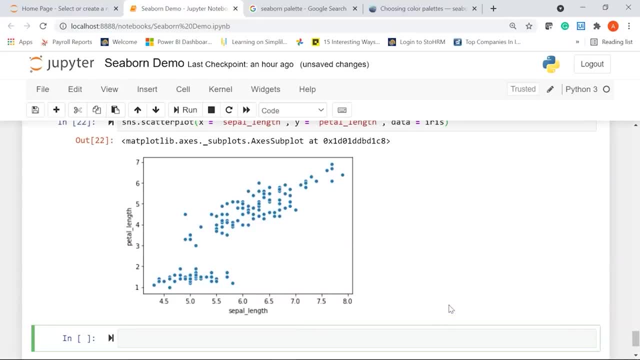 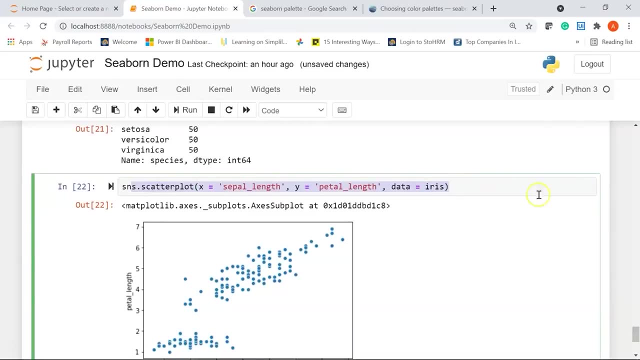 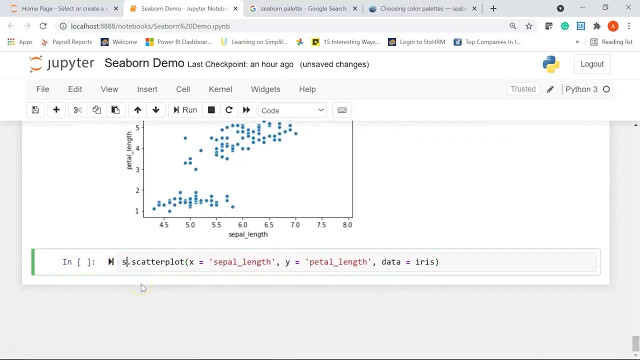 using the hue parameter as species in the function. so what i will do is i am going to copy my above code, i just paste it here and we are going to edit in this cell itself. i will add a last parameter called hue, and this will have my species. 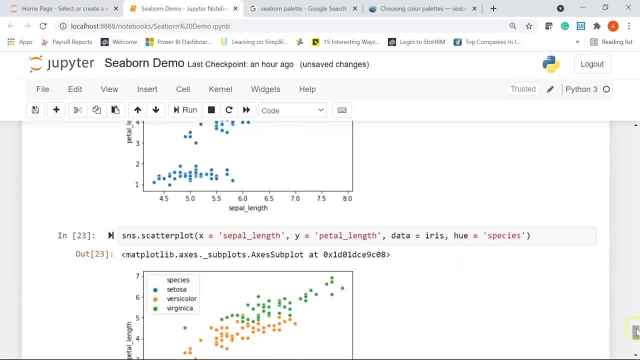 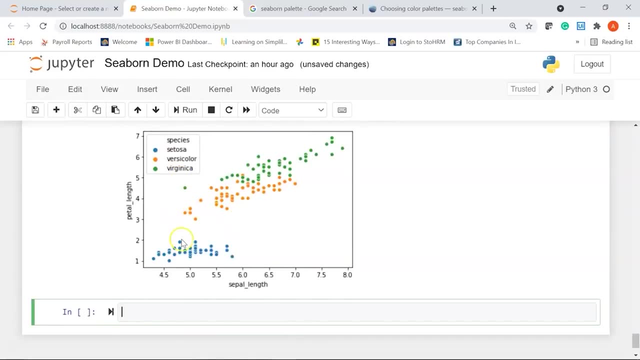 column. let's run it and see the difference. there you go, here you can see we have a nice scatter plot. the blue dots are for satosa, the orange dots are for versicolor and for virginica you have the green dots. from this scatter plot you can see that for virginica. 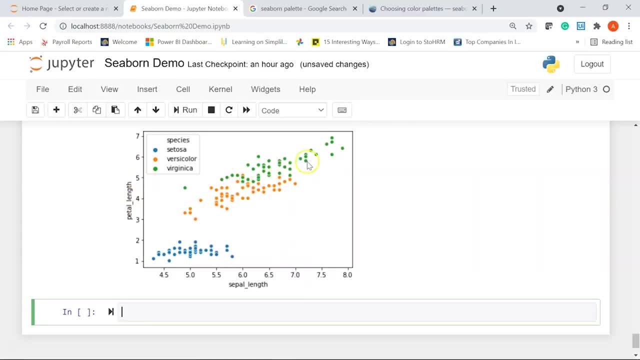 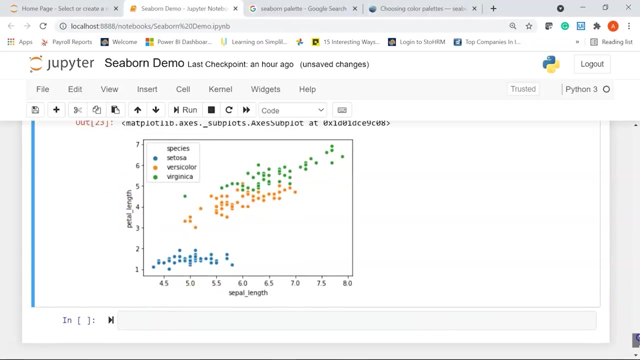 flowers the sepal length and the petal length are higher than your- versicolor and satosa- and this region is completely for satosa flowers, so you can see that the satosa flowers have lower sepal length and petal length. alright, you can also use another. 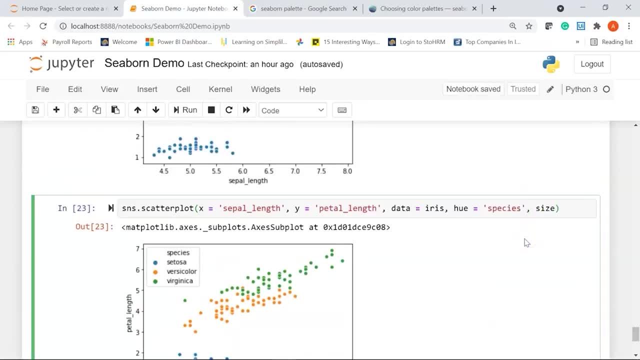 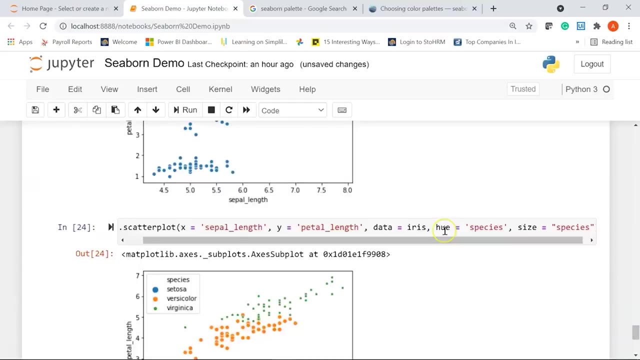 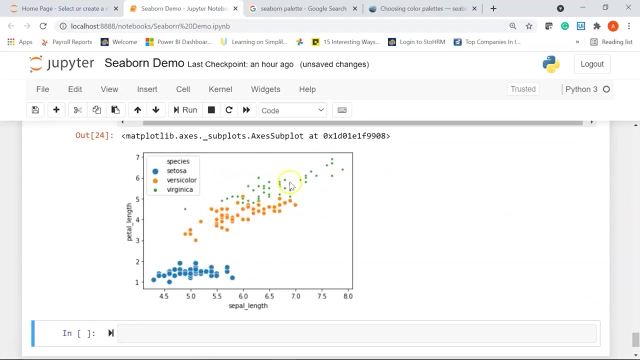 parameter known as the size, that will differentiate the different species of flower in terms of the size of the dots. i will say size as species. let's run it. you can see the result. there you go. so here you can see. the virginica flowers are in green. 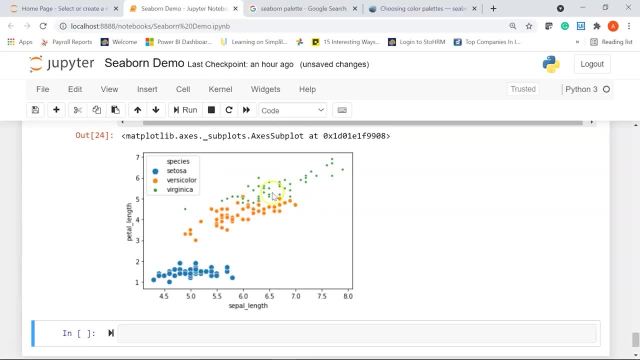 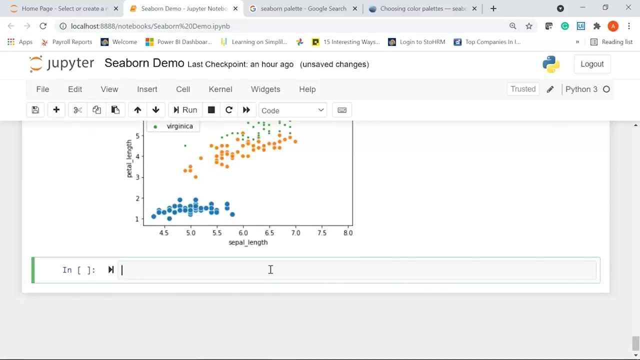 dots, the size is small, followed by versicolor with medium size dots, and then we have satosa, whose size is large. okay, now the python seaborn library lets you visualize data using pair plots. that produces a matrix of relationship between each variable in the data set. so let me show you how. 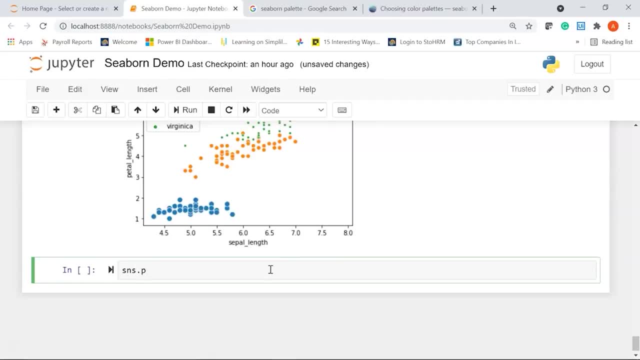 to create a pair plot, i will say sns, dot, pair plot, which is the function that i will pass in my data frame name. that is iris. i will put this iris data frame within double quotes and will run it. okay, there is some error here. lets debug the. 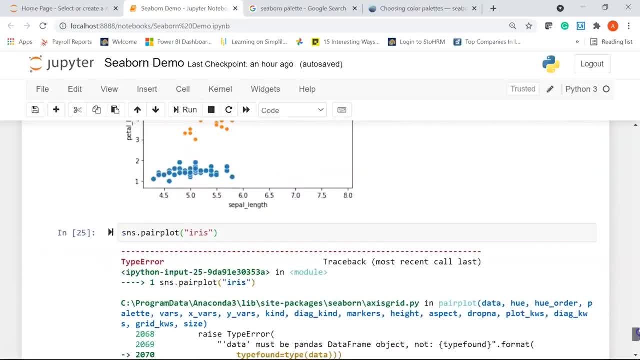 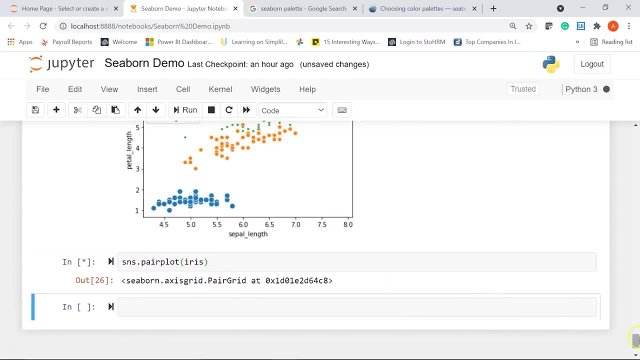 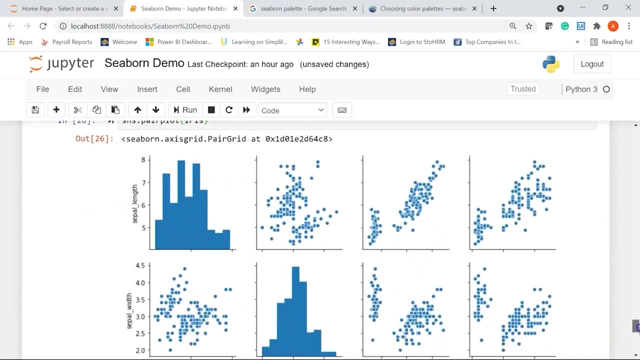 error. data must be panned as data frame. okay, what i will do is i will just remove the double quotes and will run it. this might take some time to create the pair plot, so just wait for a while. there you go, here you can see we have. 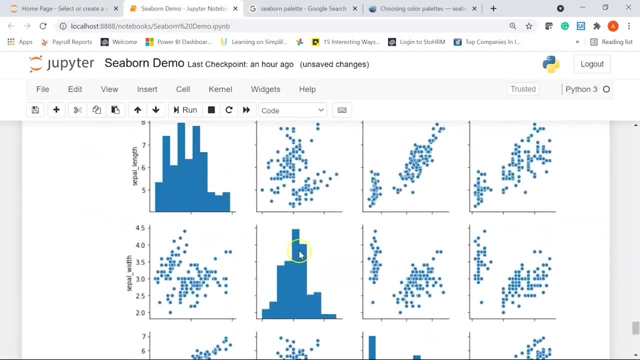 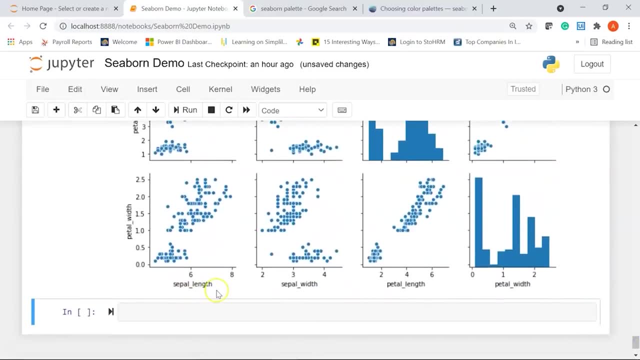 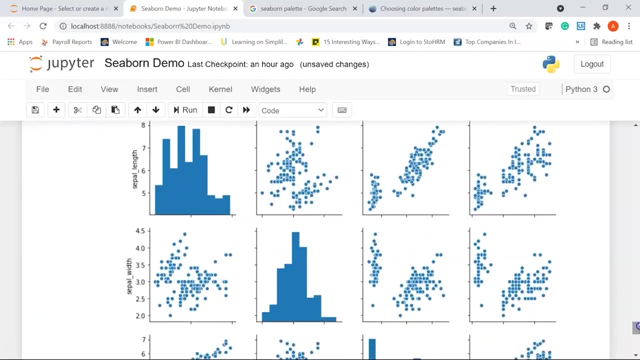 a nice pair plot. on the y axis you have the sepal length, sepal width, petal length and petal width. similarly, on the x axis also, you have the same feature: columns. all the diagonal plots are histograms and the rest of the plots are scatter plots. 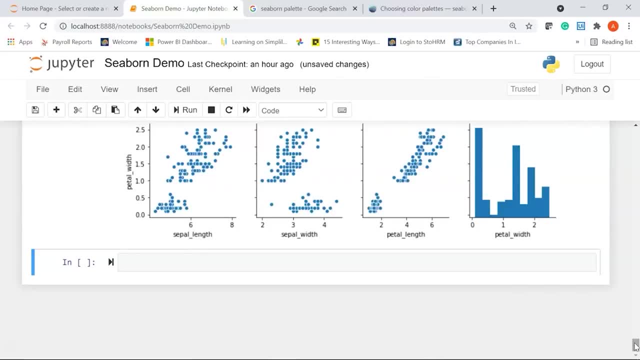 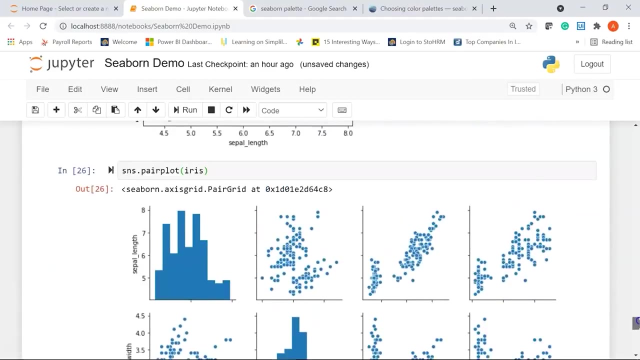 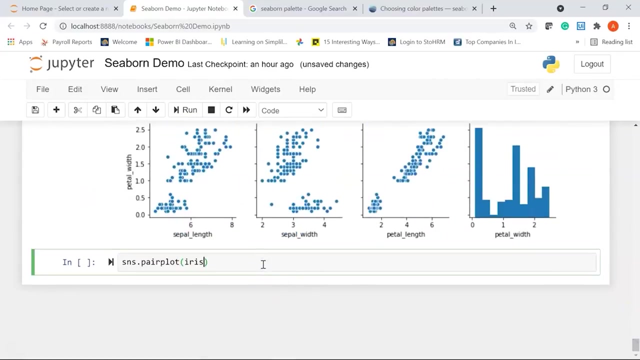 now you can convert the diagonal visuals to kde or kernel density estimation and the rest of the scatter plots using the hue parameter. this makes the pair plot easier to classify each type of flower. so i will just copy this cell of code, paste it here and i will say hue. 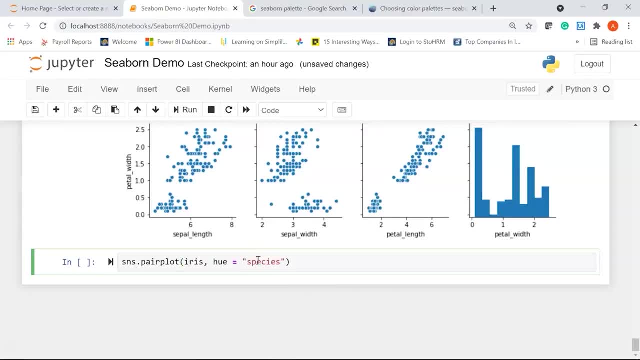 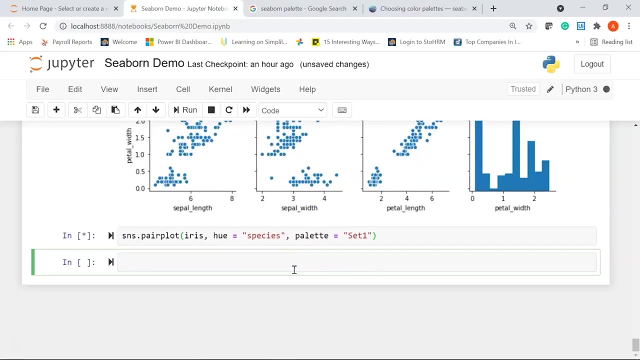 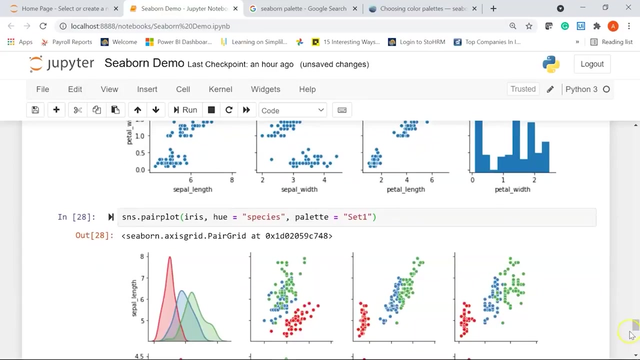 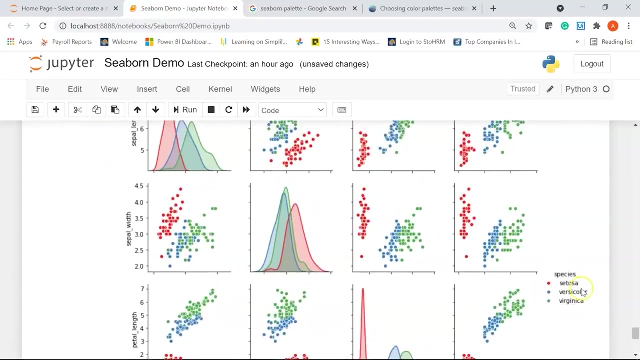 equal to species, then i will say: palette and hue equal to set1. let's run it and will see the new pair plot. now this might take some time. there you go. so here you have the pair plot ready and on the right side you can see the different species. 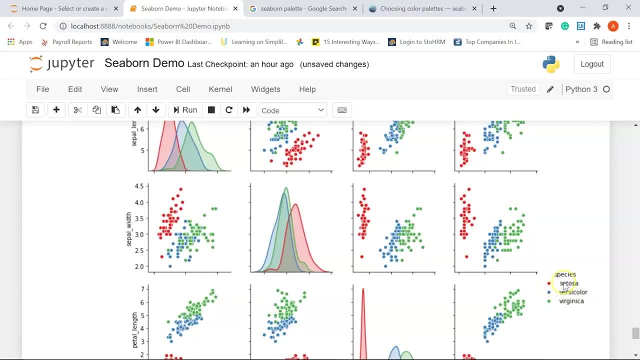 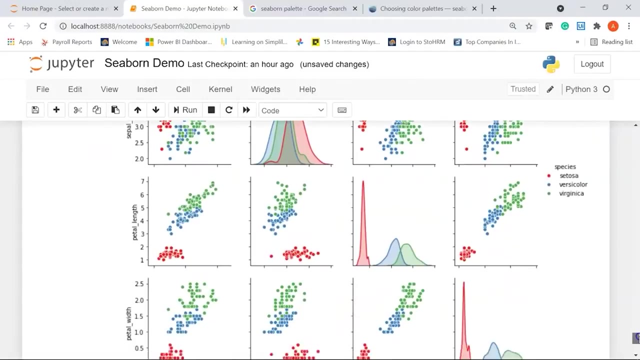 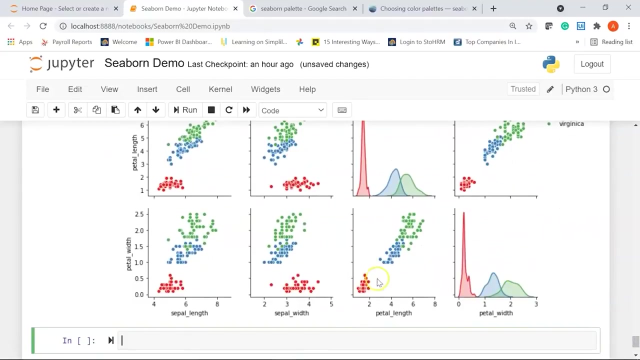 the red color dots represent setosa flowers, the blue color dots represent versicolor and the green color dots represent virginica flowers. now, if you look at this graph, you will find that your petal length is the best feature to classify the three different species of flowers. 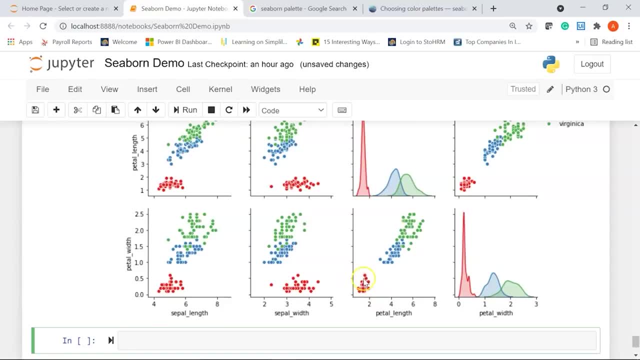 the reason being. you can see here they are very well categorized and they are separated. all the red dots present here in the petal length represent setosa flowers around this range. all the blue dots represent versicolor flowers and the green dots are all virginica flowers. 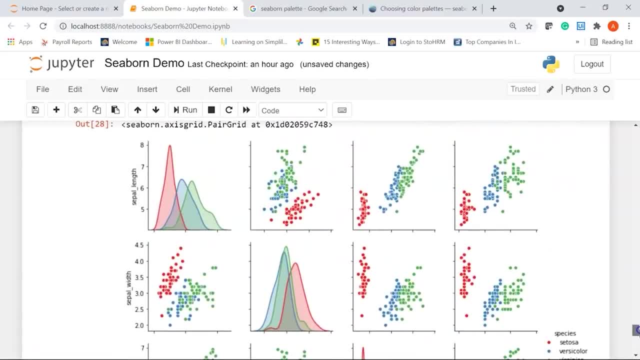 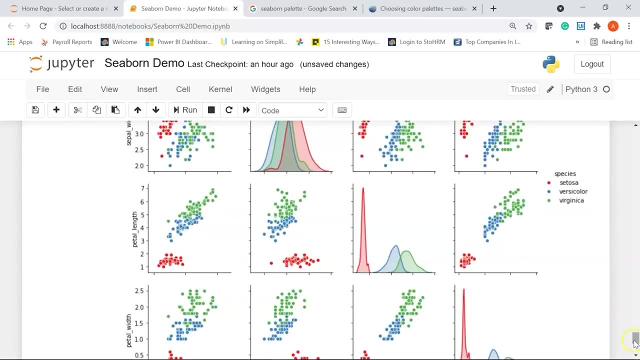 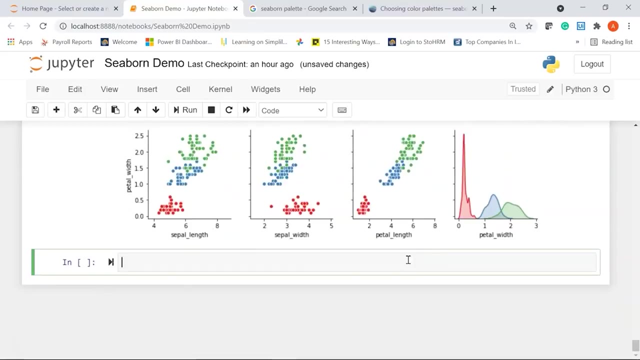 so, out of the four features- petal width, petal length, sepal width and sepal length- you can take petal length as the best feature to differentiate between the three species of flowers. alright, now coming to lmplot function. so the lmplot function in the seaborn library. 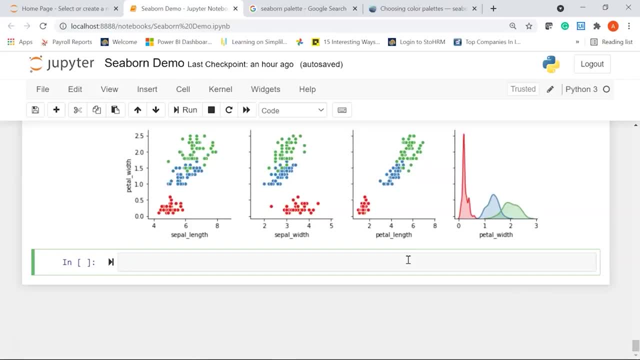 draws a linear relationship as determined through regression for continuous variables. so let's create the plot to show the relationship between petal length and petal width of the different species of iris flowers. so i'll just give a comment here. as lmplot i'll say sns. 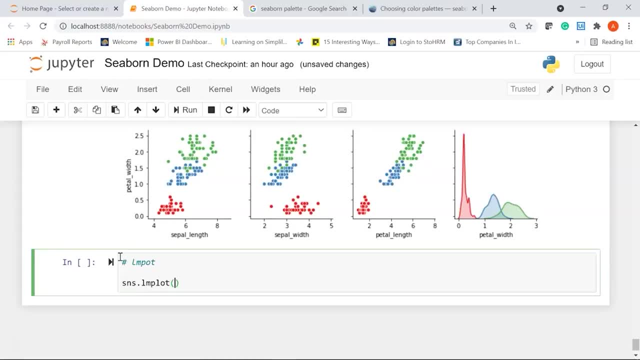 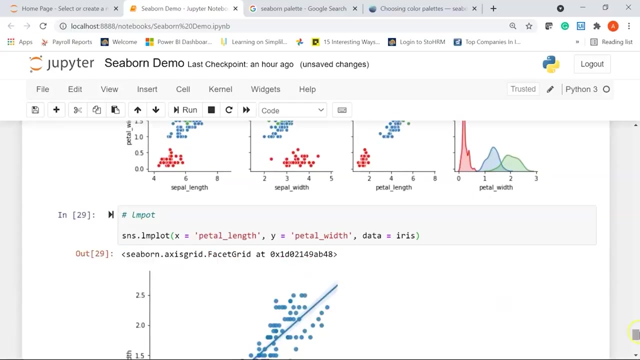 dot lmplot. in the x-axis, we'll have petal length, give a comma. in the y-axis, i'll pass in petal width and i'll pass in my data frame using the data argument or parameter, which is iris. let's run it. you can see it here. 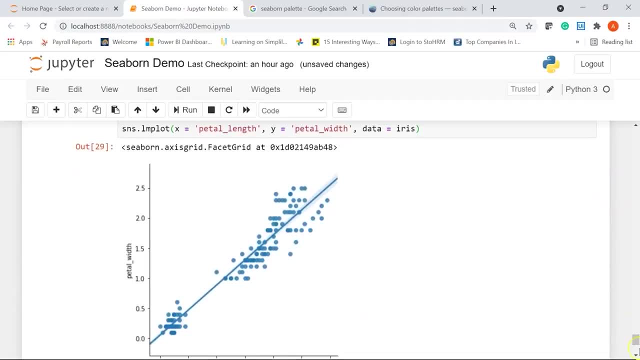 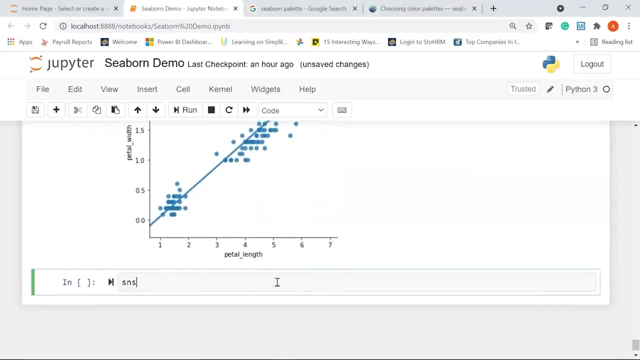 we have a nice plot. the line you see here is a linear regression line. now in this lmplot you can use the hue parameter to differentiate between each species of flowers and you can set markers for different species. let me show you how to do it. i'll say sns dot. 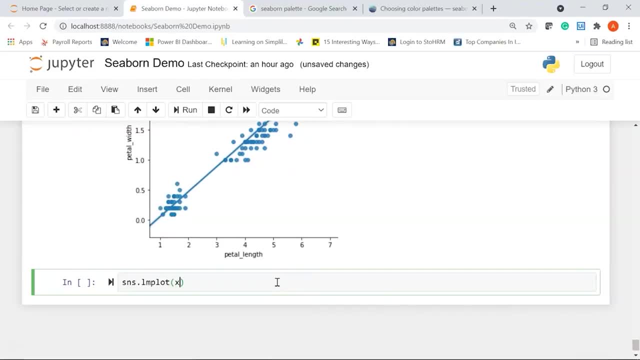 lmplot. we'll say x as our petal length, give a comma. i'll write y as petal width, then i'm going to pass the hue parameter in hue. i'll say my column as species. then i'll give data equal to my dataset name, that is. 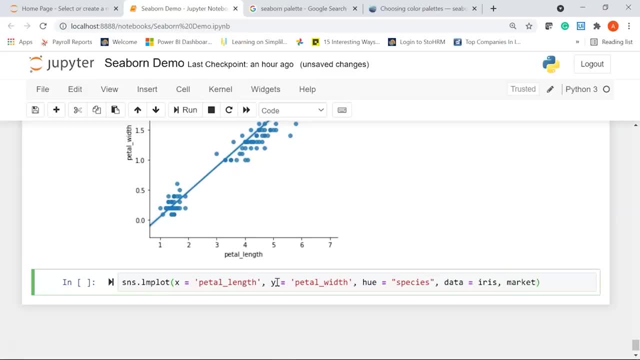 iris, and now you can pass in markers argument to differentiate the different types of flowers. let's say i want to represent setosa with dot or o, then my next species, which is versicolor, should be represented with a star symbol and the final virginica species of flowers should. 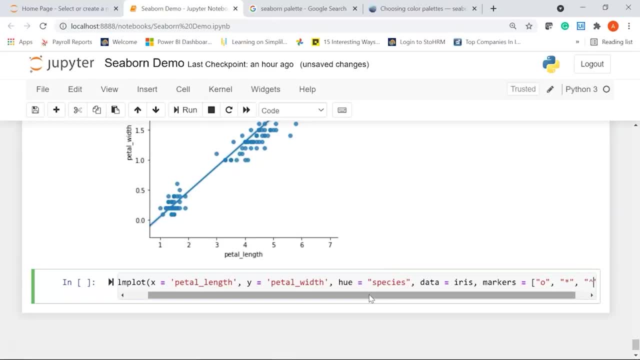 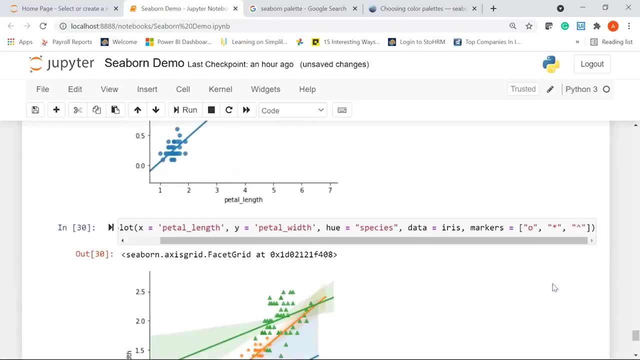 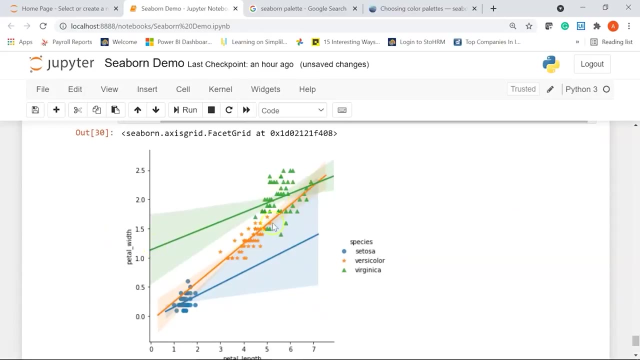 be represented with, let's say, this arrow mark. now let me go ahead and run it. there you go. you have three different linear regression lines, and the circle dots in blue color represent setosa. the orange color stars represent versicolor flowers and the triangles represent virginica flowers. 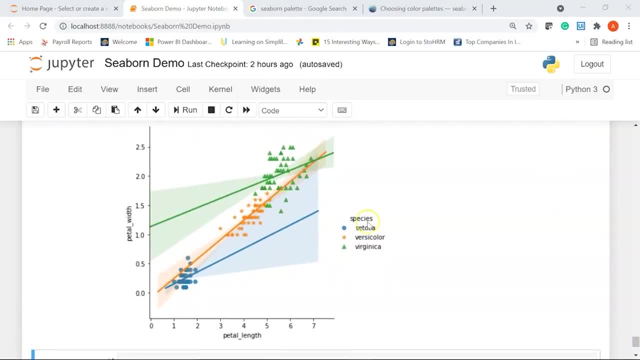 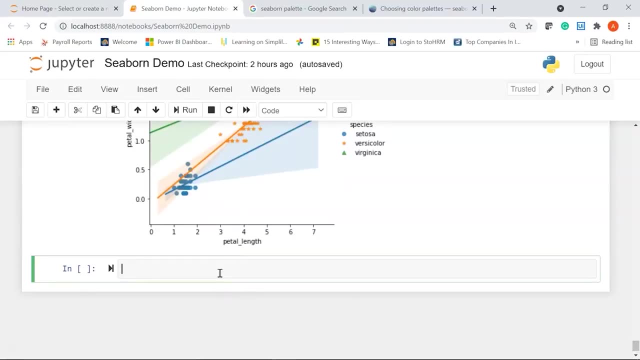 so this is how you create a linear relationship between the different types of flowers using the regression line. alright, now let's take a look at the final plotting function, where we will create a box plot. a box plot, also known as a box and whisker plot, depicts the 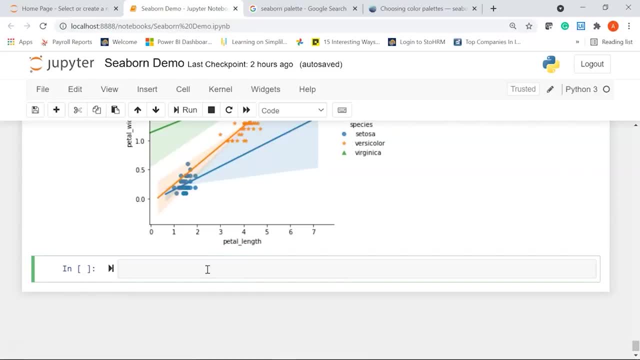 distribution of quantitative data. the box represents the quartiles of the data set, the whiskers, so the rest of the distribution, except for the outliers. now let's see the distribution of the three species of flowers based on their sepal width. just give a comment as box plot. 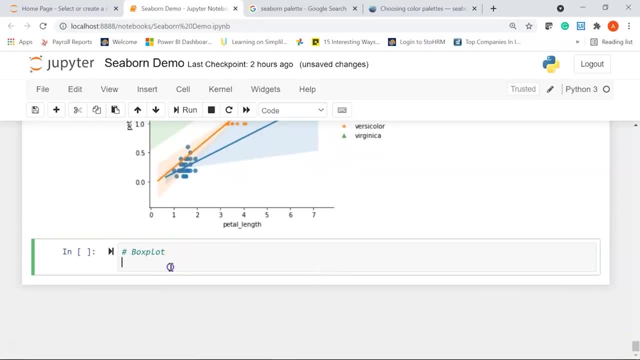 is the final plot that we are going to see in our seaborn demo. I will say snsboxplot. in the x-axis we will have the species column. in the y-axis we will have sepal width. then I will pass my data as iris. let's run it. 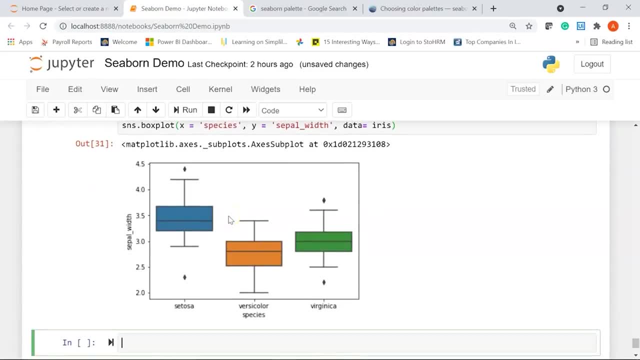 here you go. we have this box plot created at the bottom in the x-axis. you can see. we have the box plot for setosa flowers, orange for versicolor flowers and green for virginica flowers. now this line represents median which is inside the box, so this is also the median for versicolor flowers. 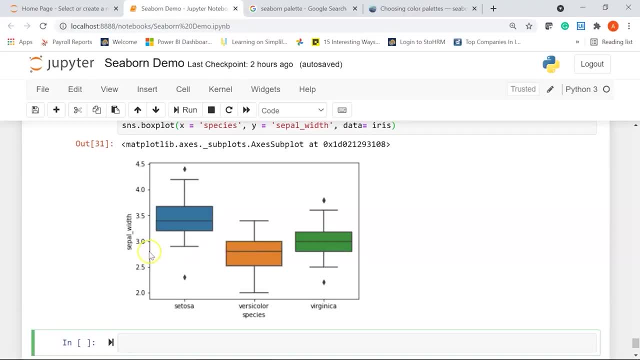 you can compare the median sepal width for each of the flowers from the y-axis. this line represents the maximum sepal width value for setosa flower and this line at the bottom represents the minimum length of the sepal width for setosa flowers. now these dots. 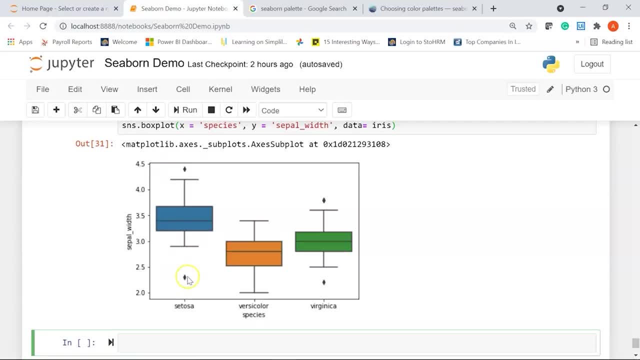 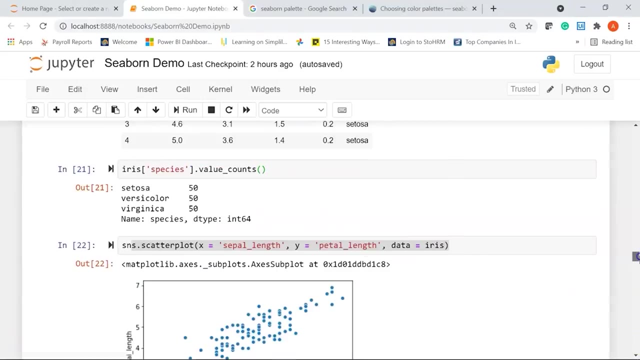 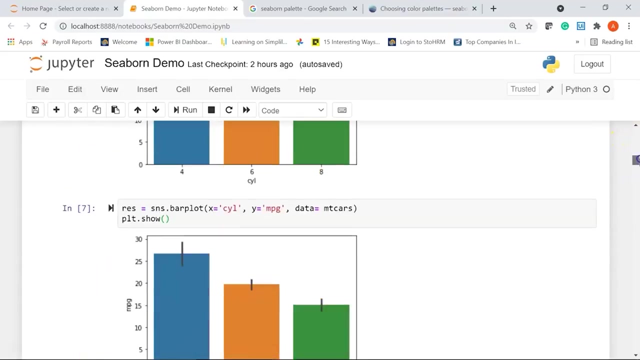 that you see outside the box plot are called as outliers. the extended lines that are outside the box plot are known as whiskers. alright, so that brings us to the end of this demo session on seaborn library in python. so first we imported our empty cars dataset, then we saw how to create. 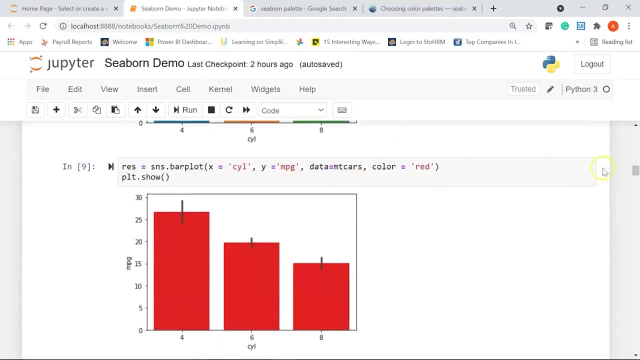 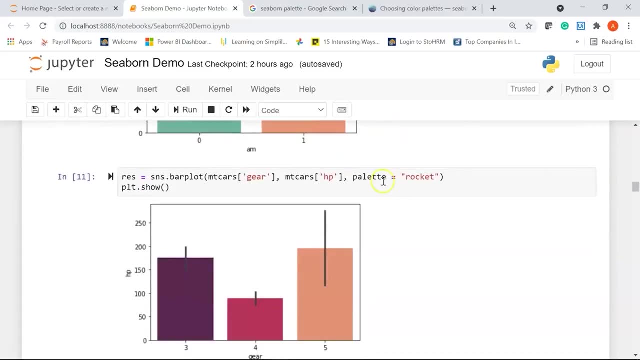 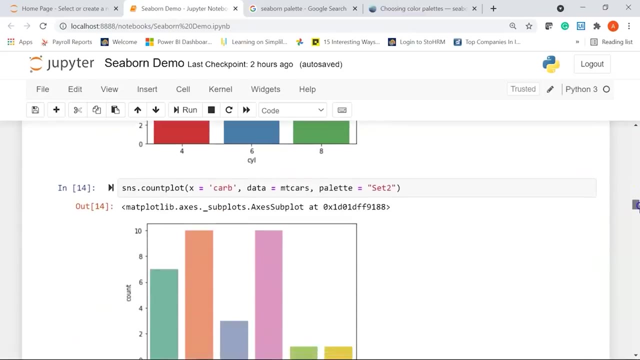 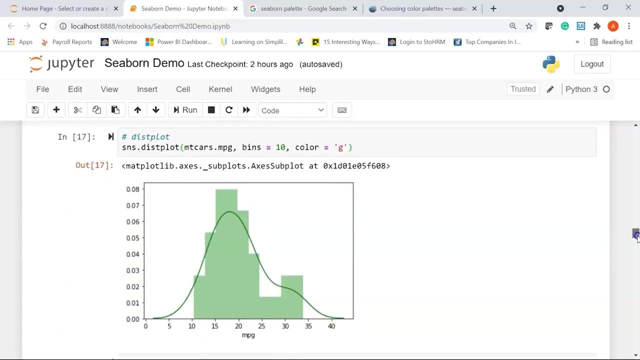 a bar plot, we learnt how to use the color argument or the parameter inside bar plot. we also saw how to use the palette attribute or the palette parameter. then we learnt about creating count plots. then we saw how to create horizontal count plot. now, moving ahead, we saw how 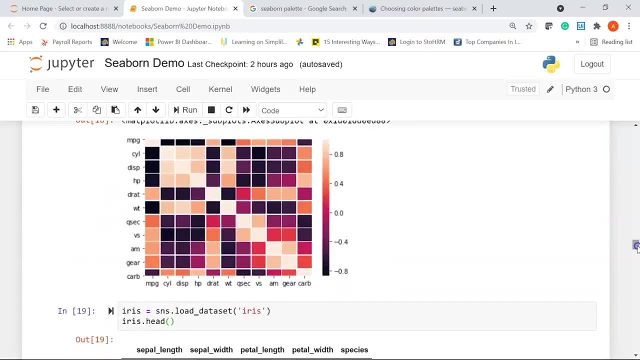 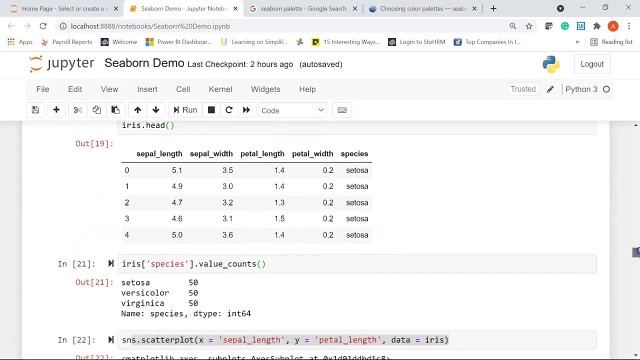 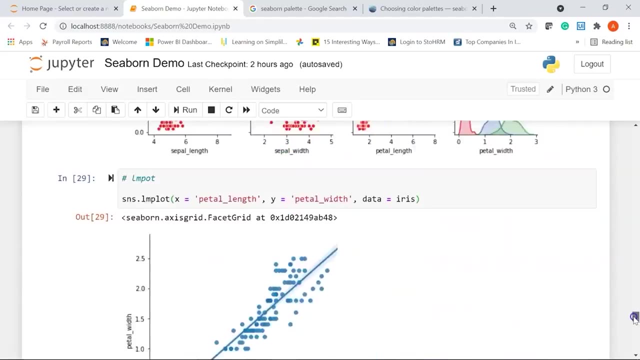 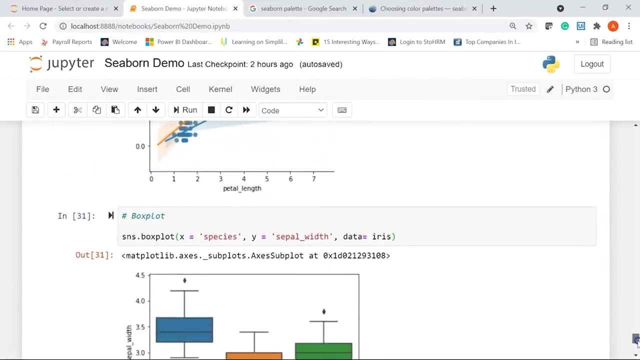 to create distribution plot. then we saw correlation heat map. after that we analyzed the other functions, such as the scatter plot. then we had the lm plot and we had the lm plot for finding the linear relationship, and later we saw the box plot using the iris flower dataset. 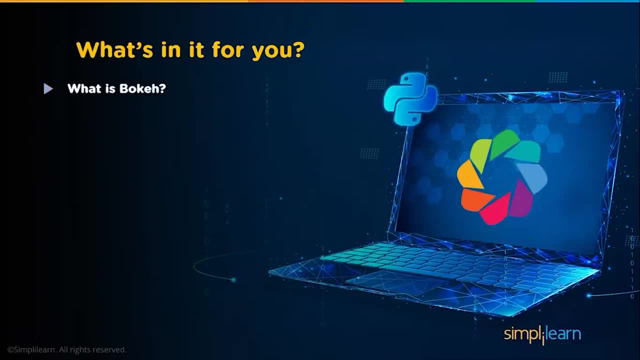 so first we will explain what exactly the meaning of bokeh is. then we will take a look at scatter charts and see how we can implement them in bokeh. next we will understand what line charts are, the scenarios in which they are used and how they can be coded. 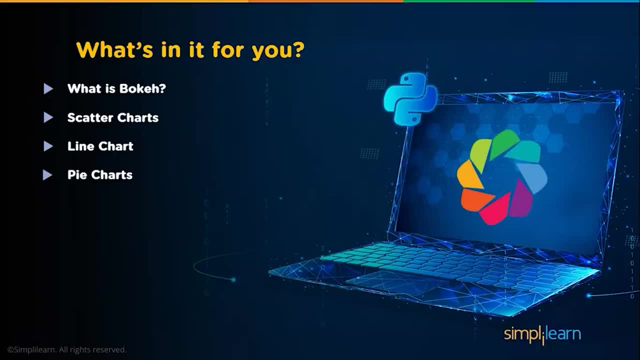 in python bokeh, then we will move on to pie charts and understand how data distribution can be represented using them. next, we will take a look at histograms. then we will move on to bar plot and understand the difference between histograms and bar plots. we will then take a look at 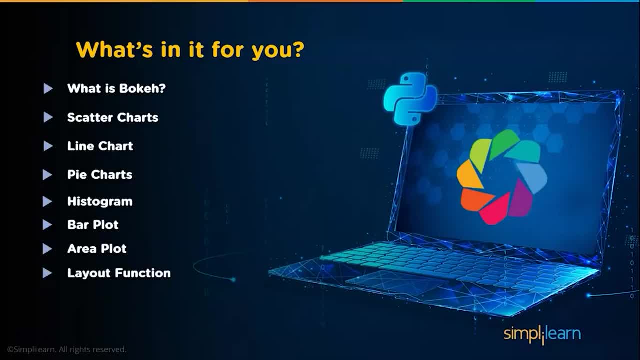 area plot and how to understand them. and then we will move on to the layout function in bokeh, which is used to make interactive web pages. and finally, we will use a dataset to understand how we can make interactive charts in bokeh by using everything that we have already learned in this video. 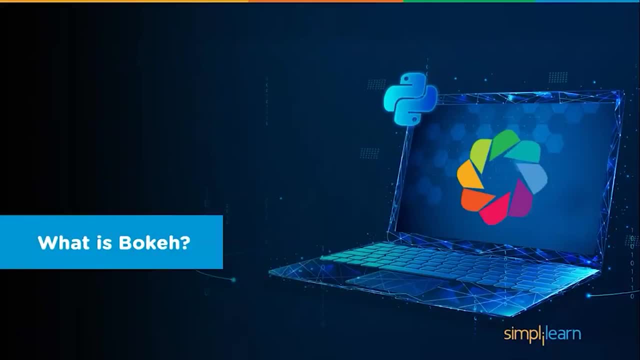 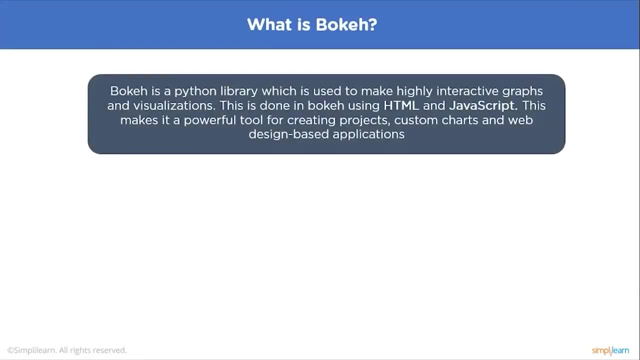 so the first question that probably comes to your mind is: what exactly is bokeh? bokeh is a python library which is used to make highly interactive graphs and visualizations. this is done in bokeh using html and javascript. this makes bokeh a powerful tool for creating projects. 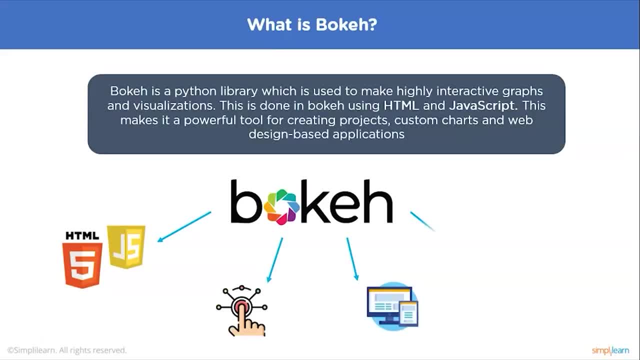 custom charts and web design based applications. now bokeh is a python library for creating interactive visualizations for modern web browsers. it helps you build beautiful graphics, ranging from simple plots to complex dashboards with streaming data sets. with bokeh, you can create javascript power visualizations without writing. 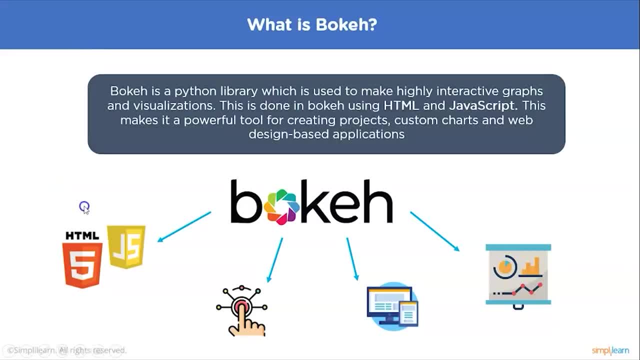 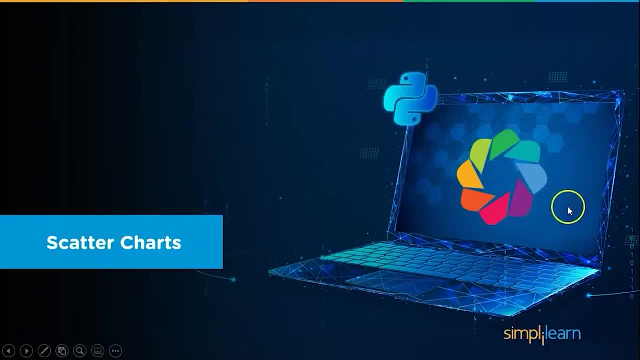 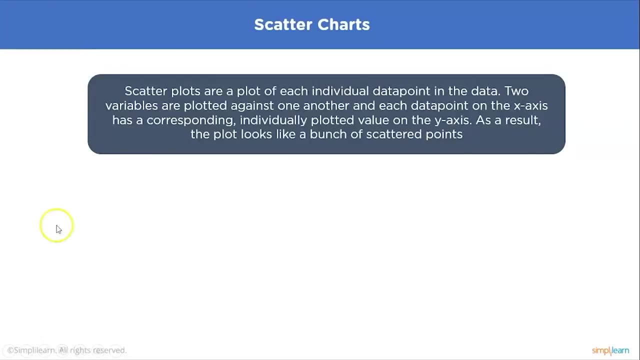 any javascript yourself. this makes it a very powerful tool for data visualization. next, let's take a look at scatter charts and how you can plot them in bokeh now. scatter plots are a plot of each individual data point. in the data, two variables are plotted against one another, and each 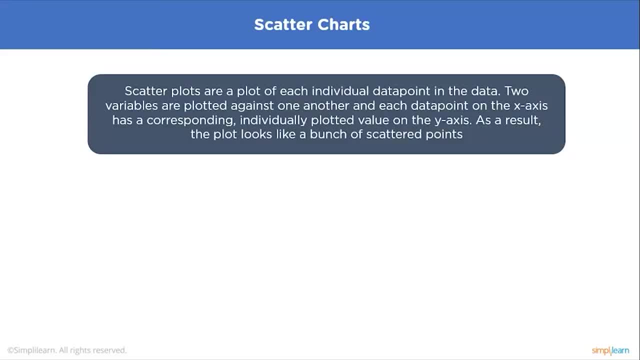 data point on the x-axis has a corresponding individually plotted value on the y-axis. as a result, the plot looks like a bunch of scattered points. these are some examples of scatter charts. here, each point on the chart corresponds to a value on the x-axis and its 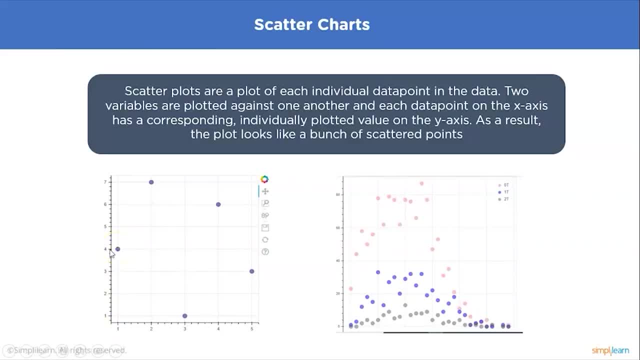 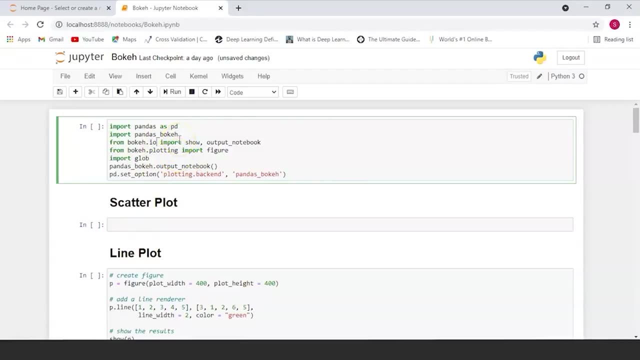 respective value on the y-axis. using scatter plots, we can see how two different variables correspond to each other. now let's see how we can plot scatter charts using bokeh. so the first thing that we are going to be doing is importing all of the necessary modules. 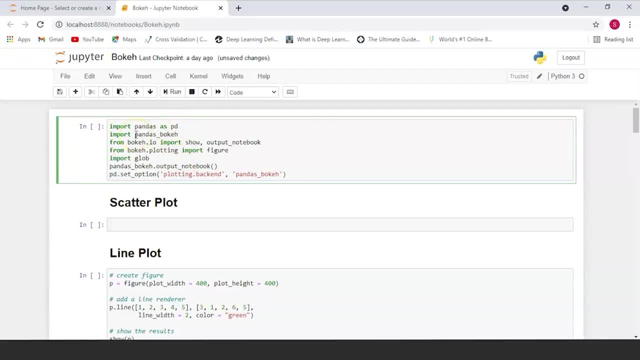 for our python project. the first module that we are going to need is the pandas module, which is used to work on data frames. next, we will also be importing the pandas bokeh module, which is used to implement bokeh on pandas data frames. next, we will import bokehio. 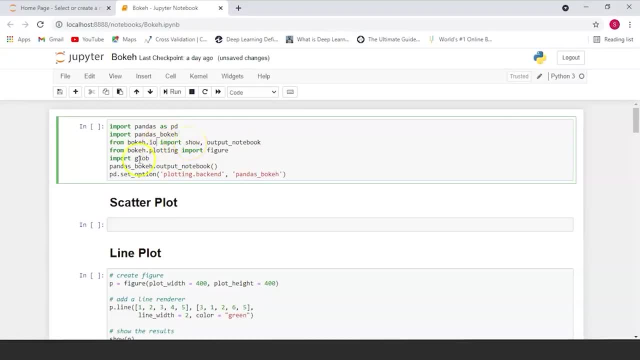 which we will use to show the various graphs that we are plotting. we will also import bokehplotting, which will help us in plotting all of the various graphs that we are going to be looking at. we will also import glob, a module which will help us. 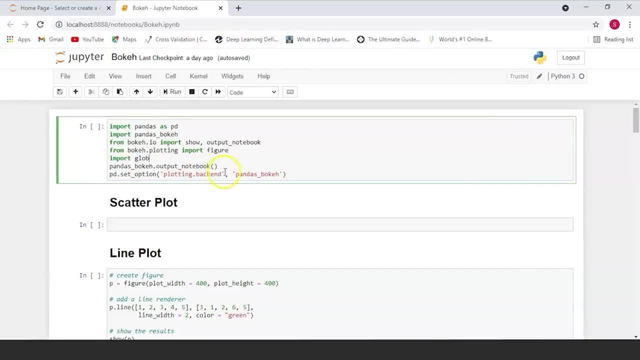 merge our files and get them in the required format. so the first line of code that we are going to be writing is pandas underscore bokeh dot output underscore notebook. this is basically just a line of code which will help you see your output in the same notebook itself. 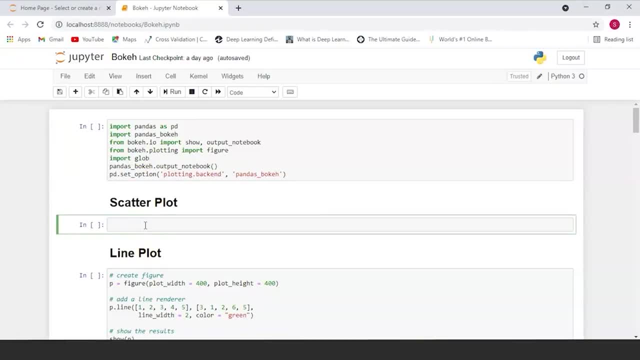 now let's see how we can plot scatter plots in bokeh. we already have imported the figure function from bokeh dot plotting. the figure function contains most of the plots that we want to plot, such as line plots, scatter plots, bar charts, etc. so this is what we are going to be using. 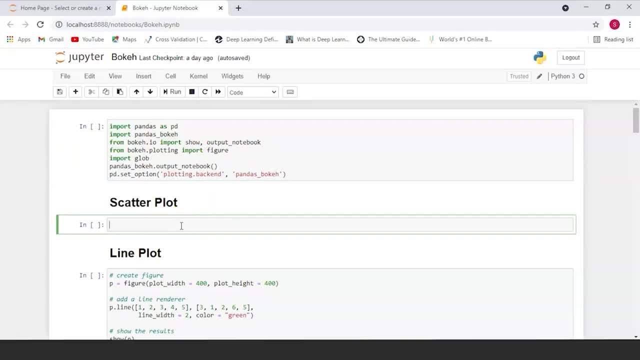 the first thing that you are going to need to do is create a figure. so how do we do that? let's create a random variable, p, and this we are going to be initializing to the figure function. now, within this figure function, we are just going to add a couple of 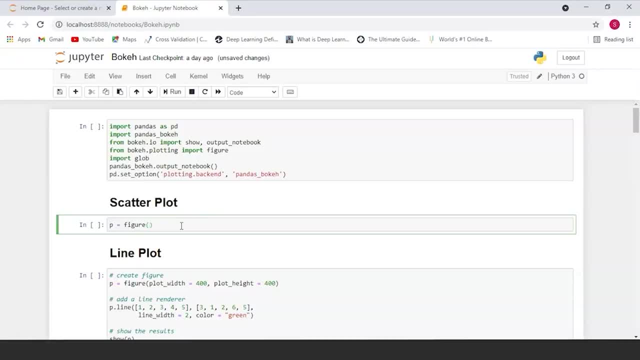 parameters for our figure itself. so let's say we want the plot width to be equal to 400 and the plot height to be equal to 402. we are going to be plotting a scatter plot in the form of a square here next. we know that a scatter plot is nothing. 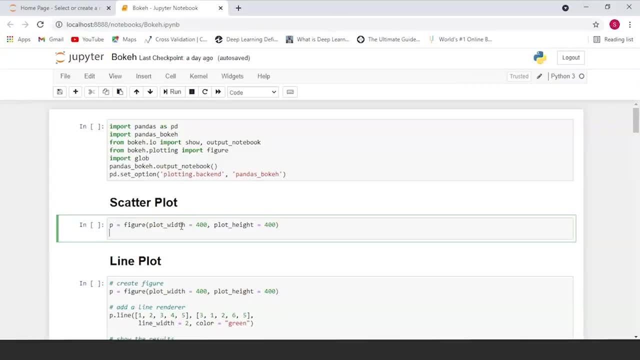 but various circles which are plotted on top of our graph. so that's what we are going to do. we are going to be plotting circles at certain coordinates which are going to be given by our lists. so the first coordinate is going to be the x axis and the next list that you are passing. 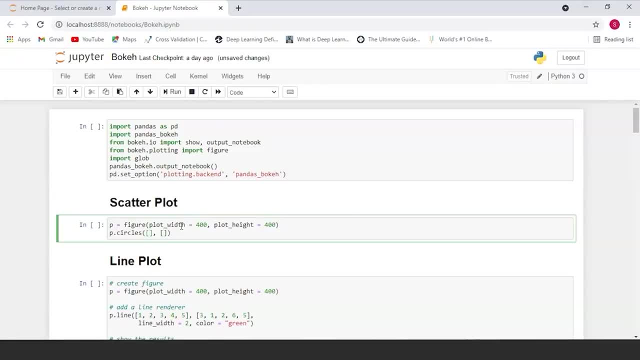 in is going to represent the y axis coordinates. so over here, let's just plot this as one comma, two, three, four and five, and over here let's start with four, seven. these are all just random points. this is just to show you how exactly you can plot a graph in bokeh. 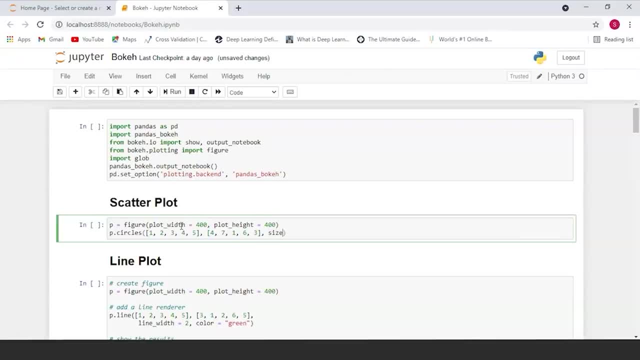 and now let's just say that we want the size of the circles to be equal to 10 and the color of every circle to be navy. we are also going to give a random parameter called alpha and equate that to 0.5. this will just act as a place holder. 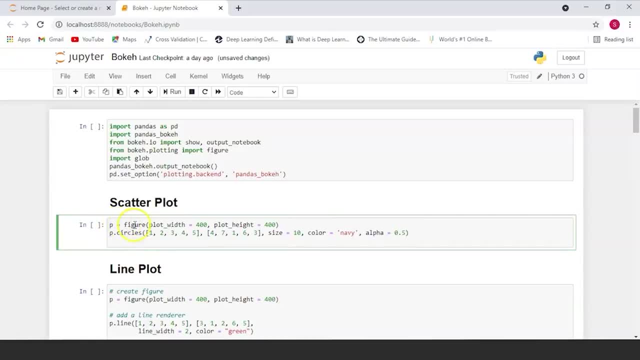 now over here, you have initialized your figure function and given it certain parameters, and, using this figure function, you are calling the circle attribute of it passing in other parameters such as the x axis coordinates and the y axis coordinates, the size of the circle, the color of each circle and 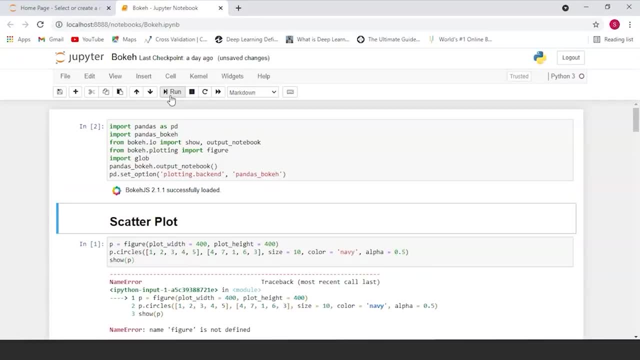 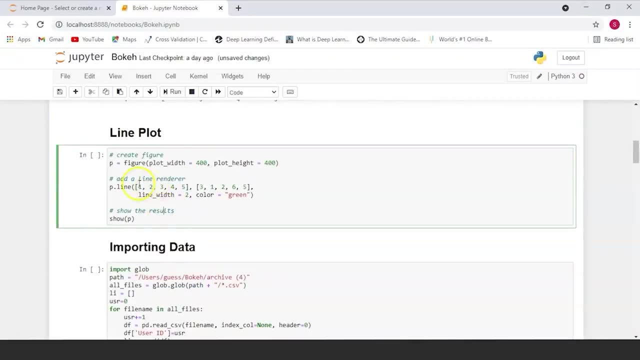 a random parameter called alpha. so now we have imported all of our modules, and this is how you plot a scatter chart in bokeh. the same thing can be done when you look at the line plot. all you have to do is initialize your figure function and call. 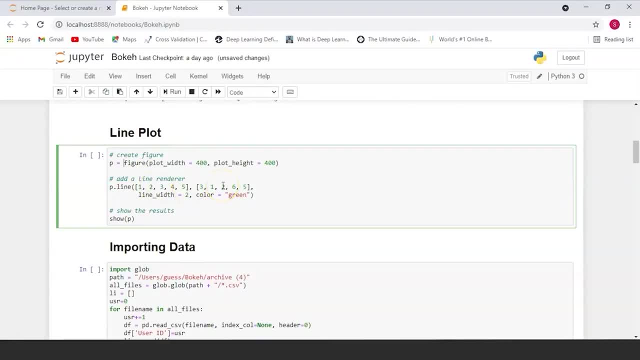 the line attribute of it, passing your x axis coordinates and your y axis coordinates, maybe passing a couple of other parameters that are required, such as the width that you want the line to be and the color that you want the line to be, and, finally, all you have to do is show the plot. 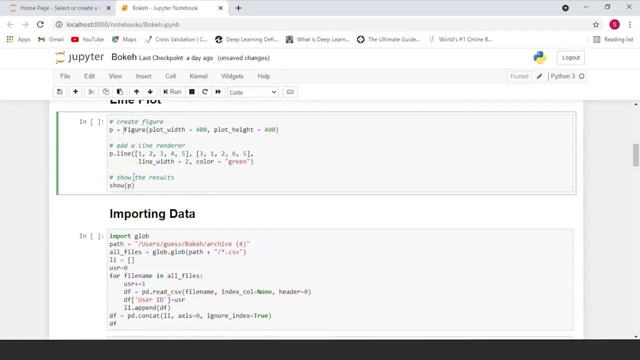 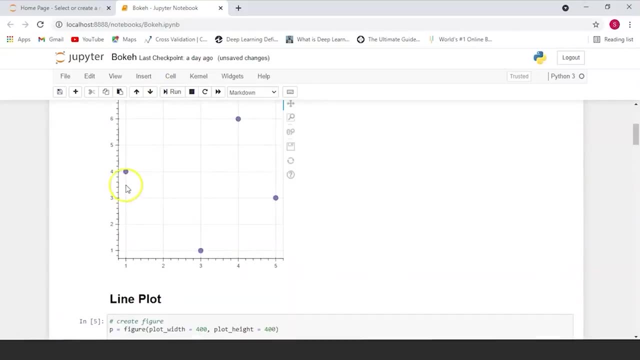 this is a basic overview of how you can use bokeh to plot graphs, and here we have a line plot. so the main difference between the scatter plot here and the line plot here is that the line plot has various different points which are connected to each other. 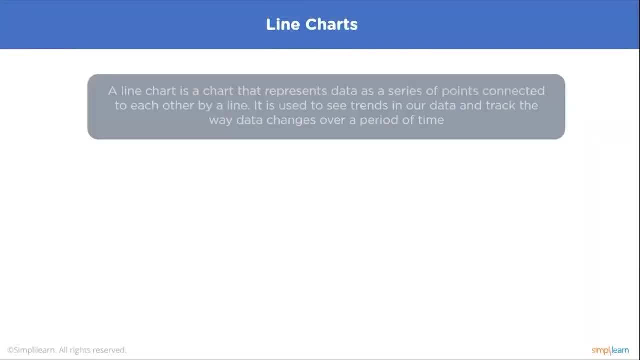 with the help of a line. so again, what exactly are line charts? a line chart is a chart that represents data as a series of points which are connected to each other with the help of a line. it is used to see trends in our data and track the way data changes. 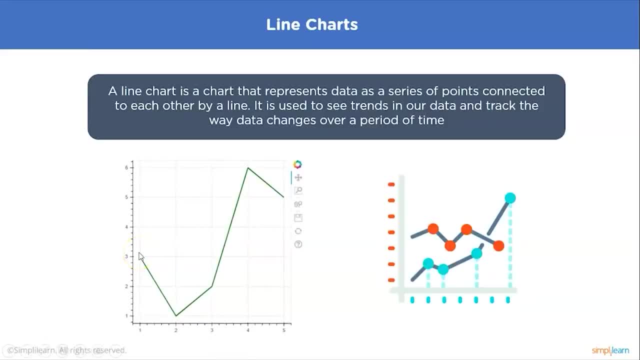 over a period of time. so this is the same chart that we just plotted using bokeh right now. so, as you can see, the parameters that you know were passed in were 1,2,3,4 and 5 on the x axis and 3,1,2. 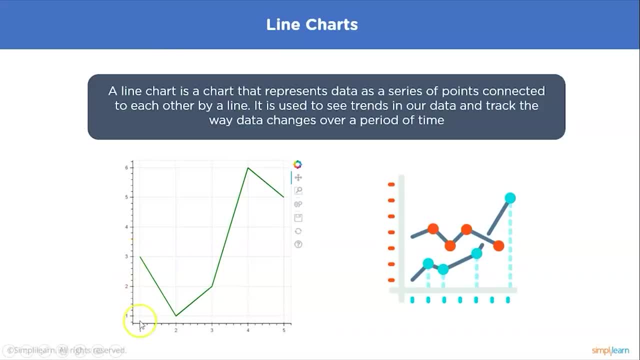 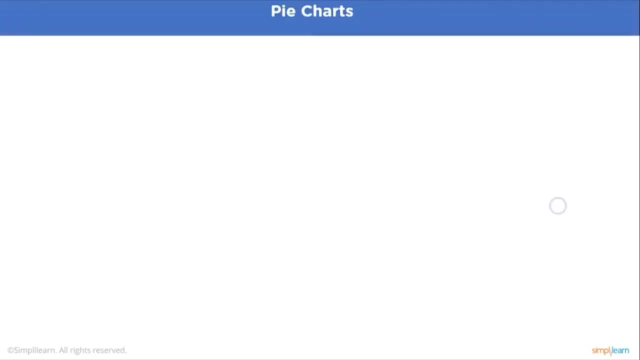 6 and 5 on the y axis. so how exactly the line chart is plotted is that you plot each of these points and then you connect them using a line. next, let's take a look at pie charts and how they can be implemented in bokeh. 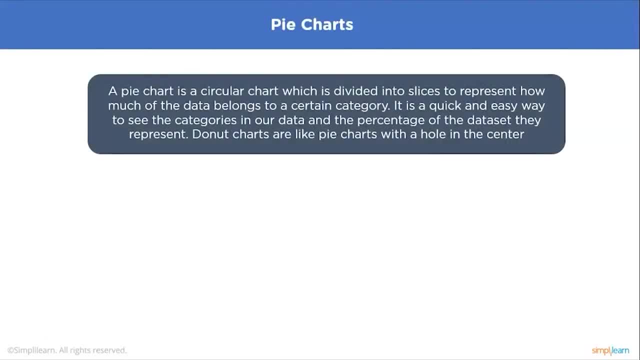 but first, what exactly is a pie chart? a pie chart is a circular chart which is divided into slices to represent how much of the data belongs to a certain category. it is a quick and easy way to see the categories in our data and the percentage of the data set that they represent. 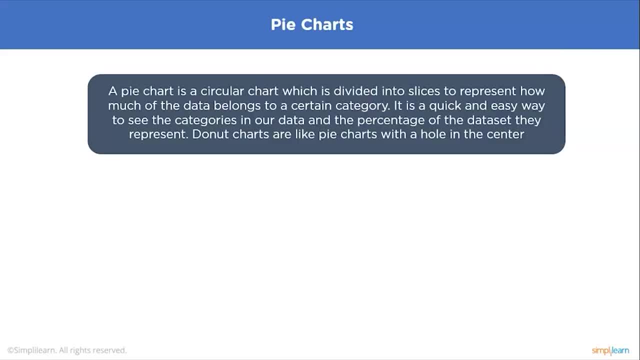 on the other hand, you have another type of chart called a donut chart. donut charts are like pie charts with a hole in the center, and in this hole you can use it to represent extra data, or you can draw a pie chart within that hole itself. so this is an 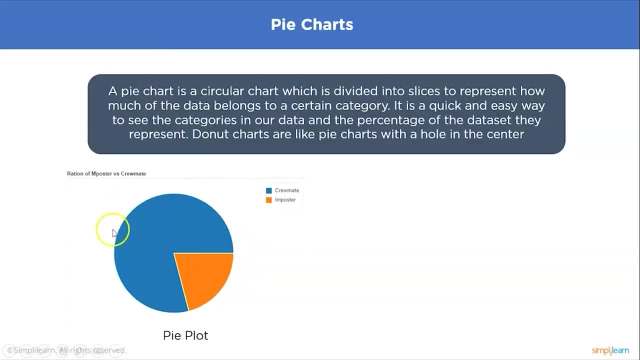 example of a pie chart. using this, you can easily get to know the various categories that our data is divided into and the percentage that each of these categories contribute towards our data. like over, here, we have a pie chart which represents crewmates and impostors in a game called among us. 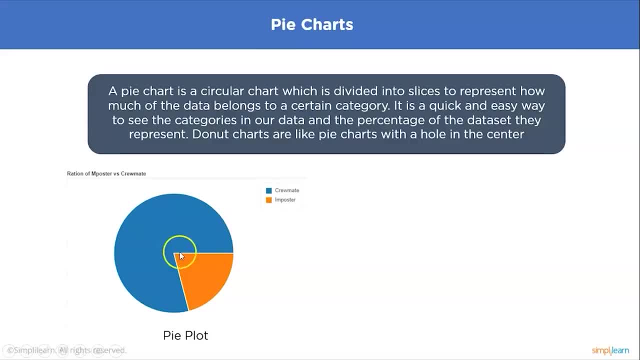 so, using this, we can just say that around 75% of our data is crewmates and 25% of it is impostors. on the other hand, you have a donut chart, which is almost exactly the same as a pie chart, except the middle portion. 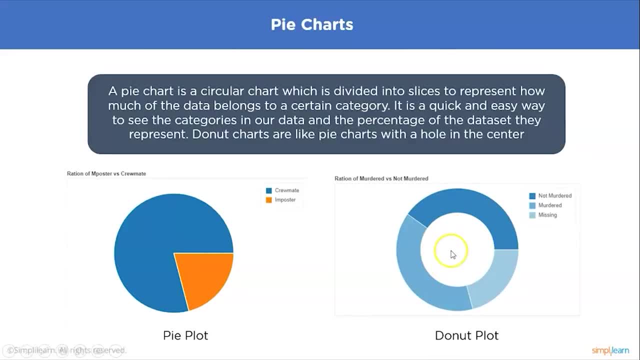 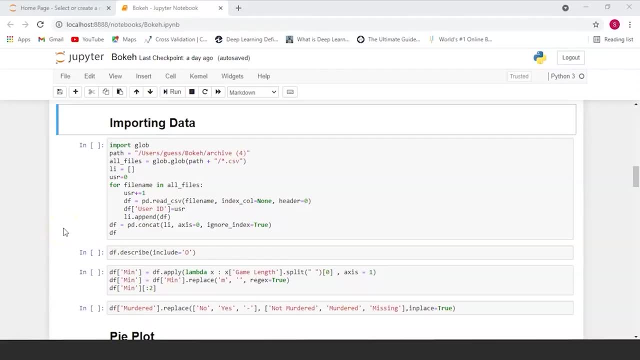 is missing values, and in this middle portion you can do other things, such as plot a pie chart or represent other data within it. so now let's see how we can plot our pie plots using python bouquet, but first we need to import the data that we are gonna be using to plot. 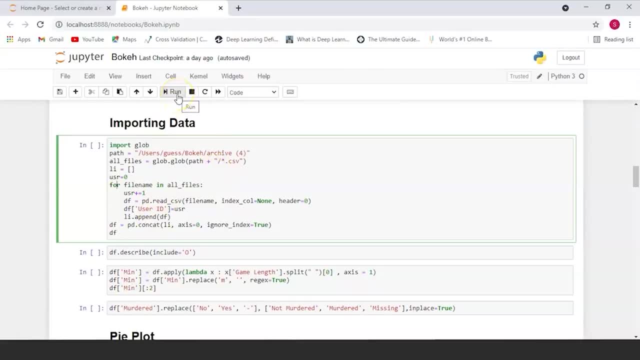 all of this. so the data that we are gonna be looking at is the among us data. among us, as you might know, is a game that caused quite a frenzy in the past 2 years, so the data that we are gonna be working at is the among us data set. 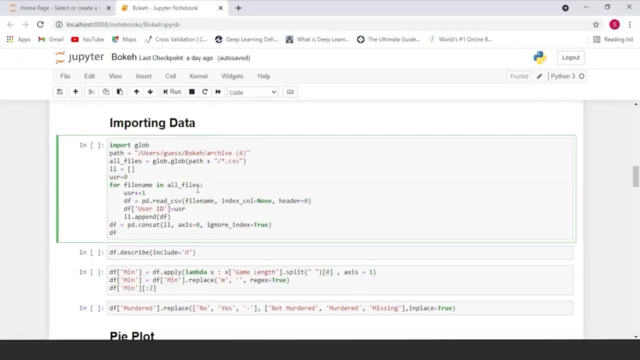 that you can find on kaggle among us was the new craze for people playing mobile games. that suddenly exploded in popularity and became a hit video game during the pandemic. now among us is basically a multiplayer game where 4 to 10 players are dropped in an alien. 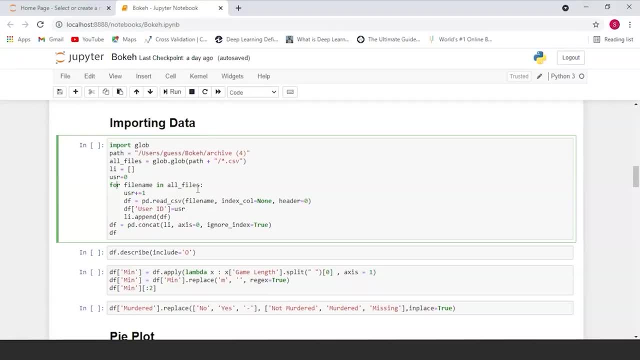 spaceship. each player has their own role of imposter or crewmate. the task of the crewmate is to run around the spaceship to complete various tasks which are assigned to them and also to not get killed by an imposter. players can be voted off the ship. 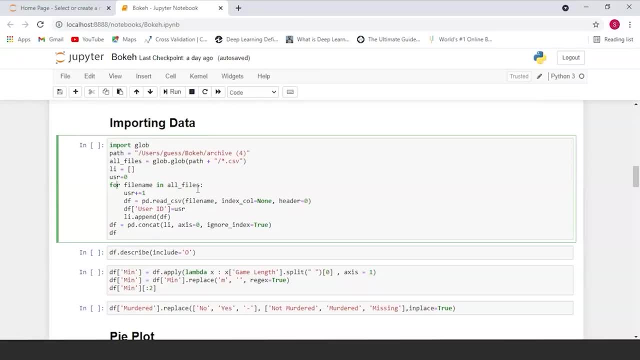 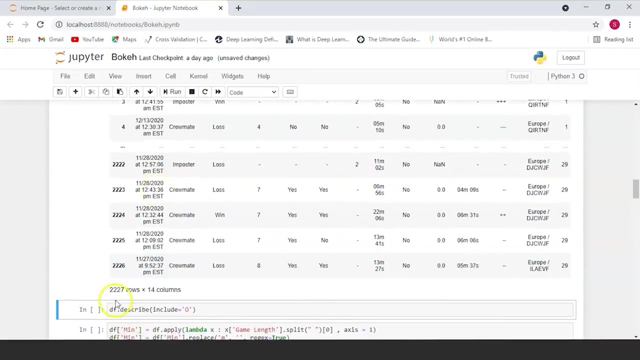 so each game becomes one of survival. so let's load this data set and create more features. so now we have imported our data set. as you can see, our data set has over 2000 rows and 14 columns. the first column that i want to show you: 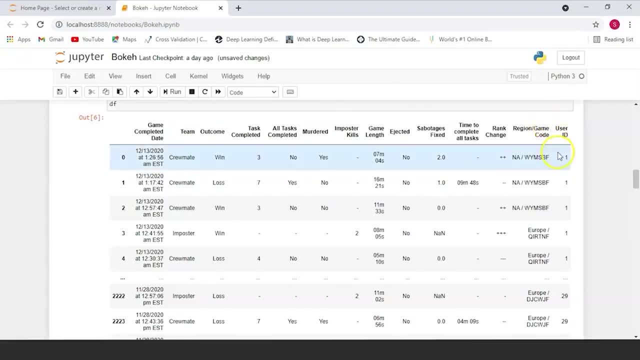 is the user id column. the user id column tells us which user the game data was collected. from now there are 14 columns. the game completed data tells us the date and time of game completion. the team tells us if the player is an imposter or a crewmate. 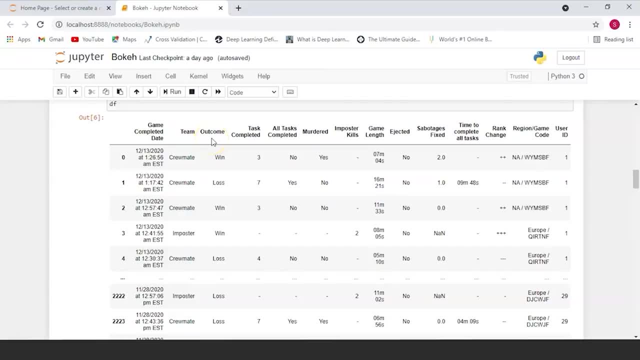 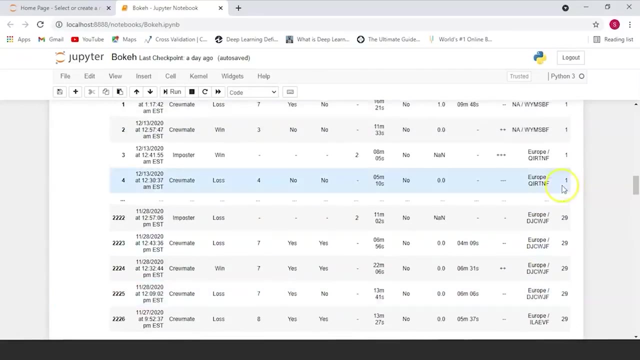 the outcome tells us if the game was won or lost, and so over here, this is each game that a certain user has played. user id is used to represent the user who has played the game and, as you can see, we have collected data from 29 different people. 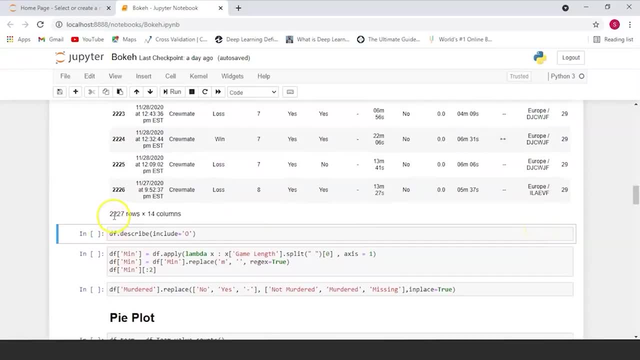 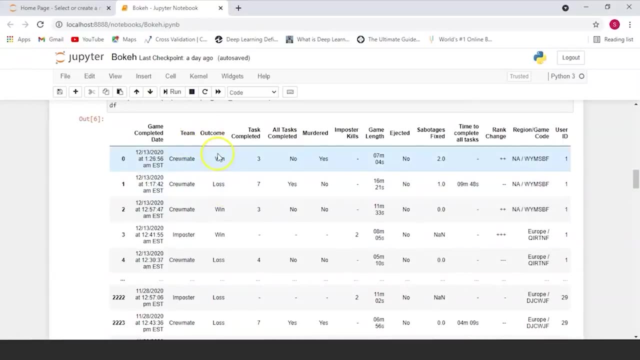 and the number of games that these 29 people totally have played is over 2000. the outcome tells us whether the user has won or lost in this game. the task completed tells us how many tasks was completed by the user in this game. all tasks completed tells us whether the 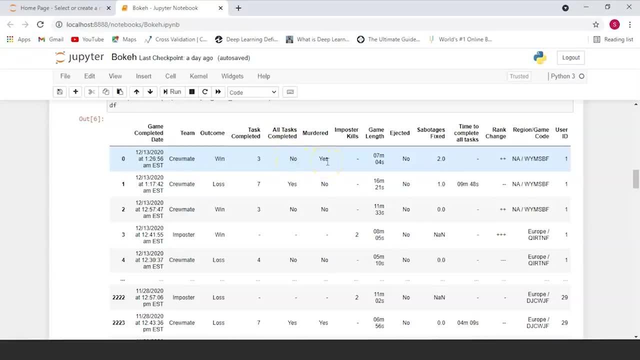 user was able to finish their tasks. murder tells us if the user was murdered and imposter kills tells us the number of kills by the imposter. so if the user was not an imposter, we do not have data on how many kills was committed by the imposter during that particular game. 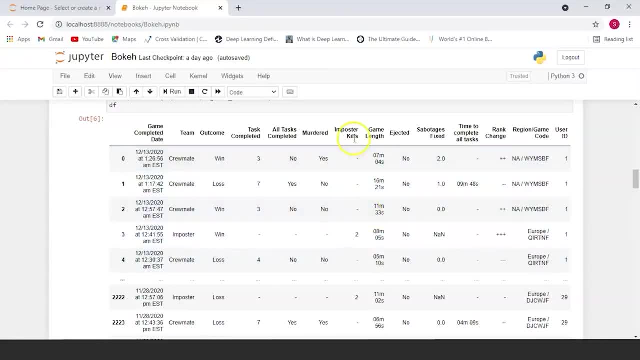 that's why this column has a lot of missing values. gameline tells us the total duration of the game and ejected tells us if the player was ejected or thrown off of the spaceship by their fellow players. sabotages- fixed is basically the imposter within the game can create. 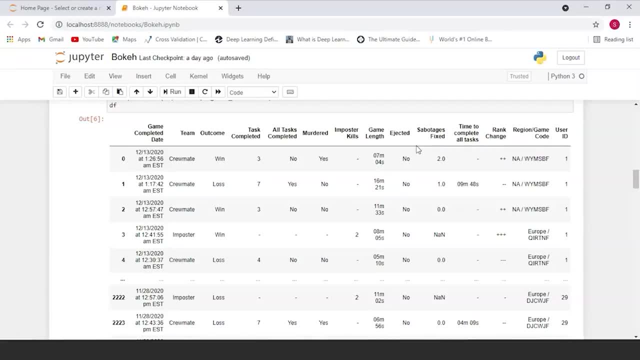 sabotages and it's the crewmates duty to fix them. so this tells us the number of sabotages which was fixed by this particular crewmate. time to complete all tasks tells us the duration taken by the crewmates to complete all the tasks and the rank change. 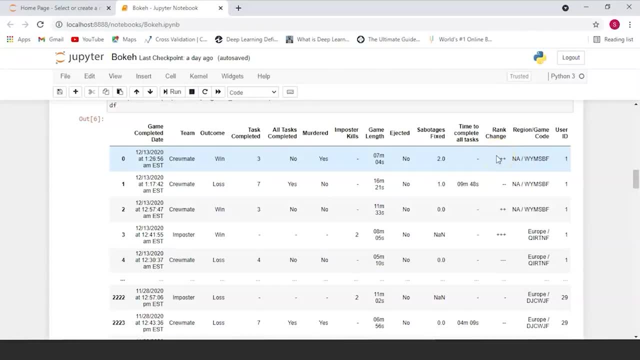 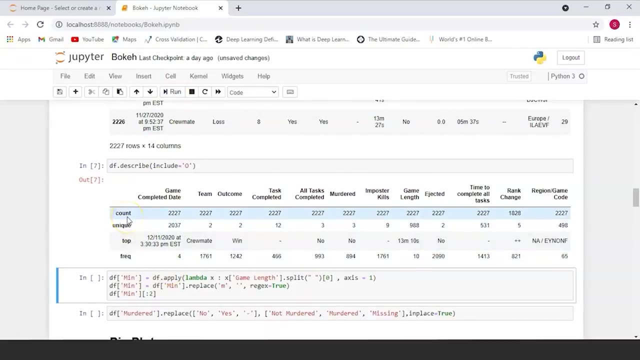 tells us the change in rank after win or losses of the game, the region or the game code tells us the server and the game code. now, first, let's just see how exactly the data is distributed. so this tells us how many counts each column has. so, as you can see here, 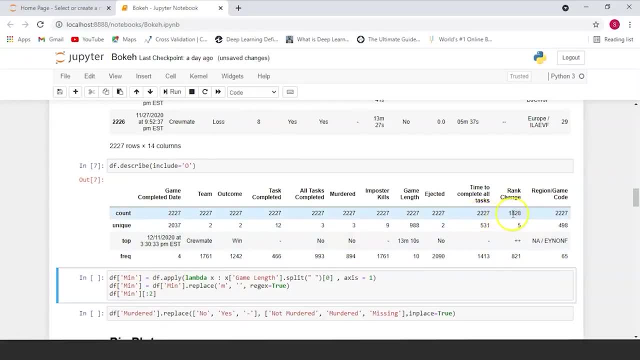 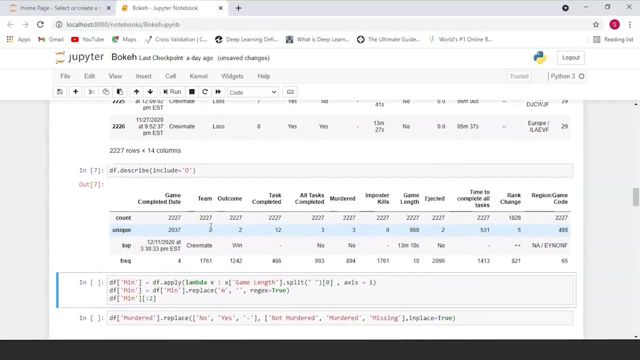 most of them have the same number of counts, except rank change, which has a couple of missing values. unique tells us how many unique values exist in each column. so, obviously, team there will be two, because there are only two possible outcomes: you can either be a crewmate or you can either be an imposter. 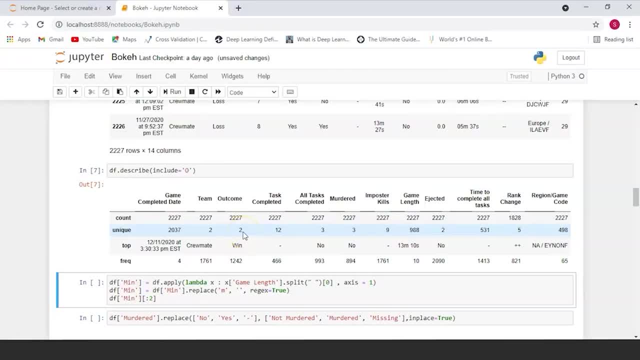 outcome also has only two unique values, because you either win a game or you lose a game. task completed has 12 different values and this is because the number of tasks which have been completed probably range from 1 to 12. all all tasks completed has three values. 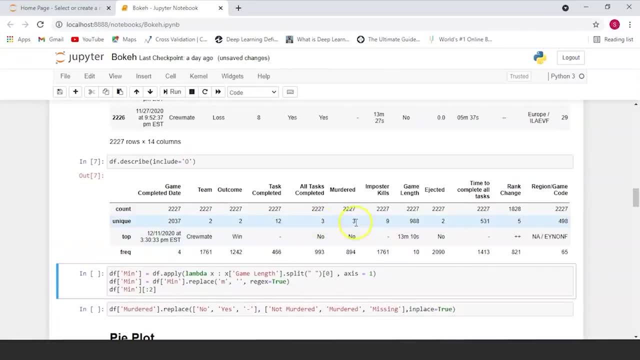 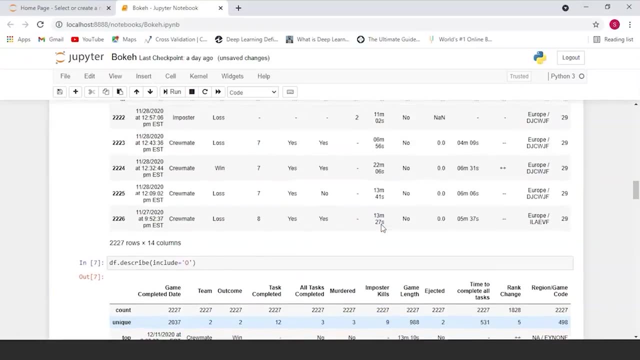 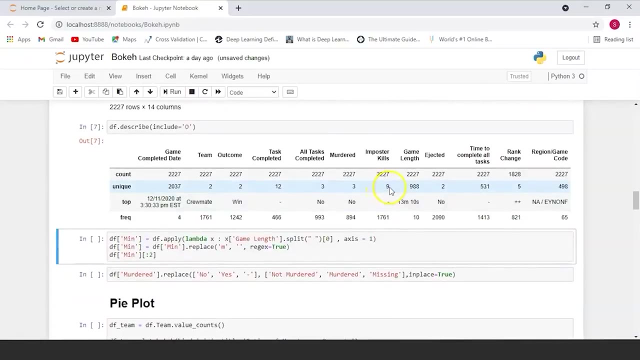 which is yes, no and missing data, and the same goes for murdered. you have yes, no or missing data. imposter kills tells us how many kills the imposter has made. so in this case, the most kills that the person has made is probably 9 game length. there are 988. 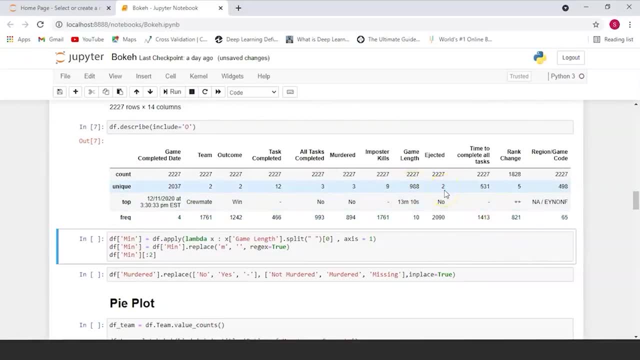 different values and ejected again. there are only two values, because you can either be ejected or you can either stay in the game. now. the top value tells us the most frequently occurring value and the frequency tells us the frequencies of all of the top values. now let's create a feature. 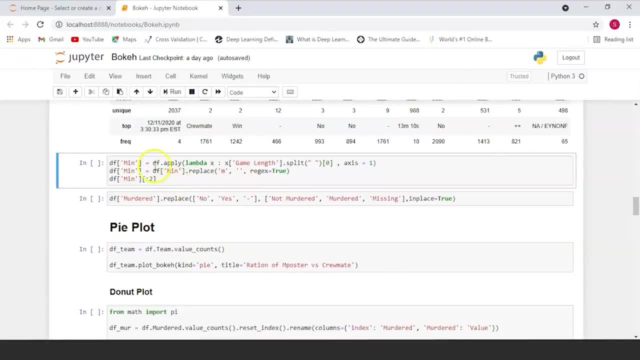 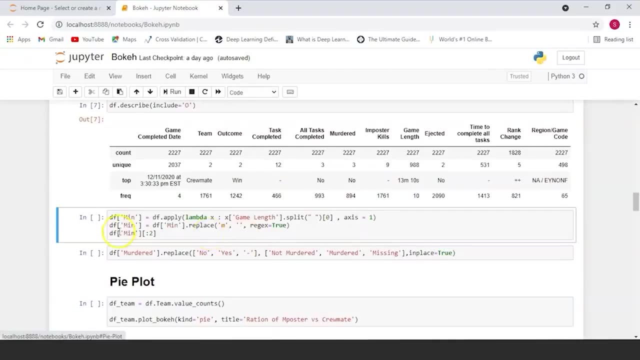 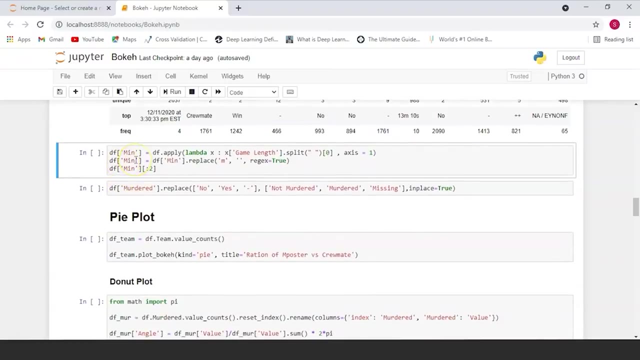 called minute and extract data from game length. so we're going to be splitting the game length column, which is this column, and we're going to be converting it into minutes, and then we're going to be using that data and creating a separate feature column called minutes. 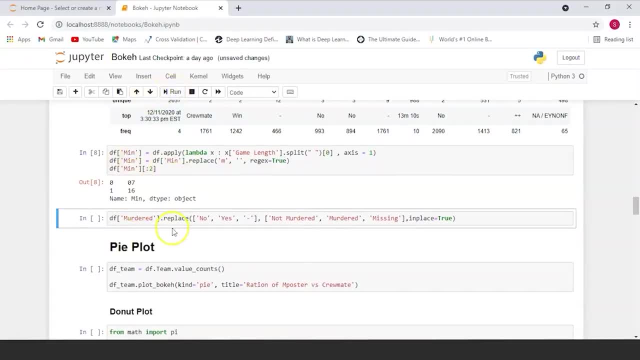 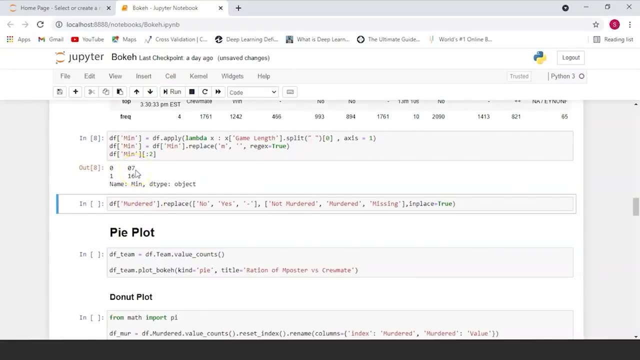 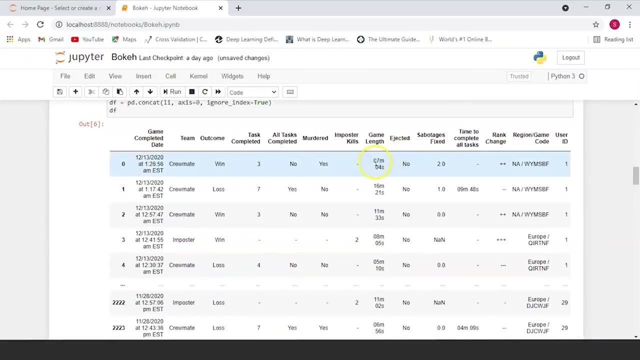 out of it. so let's do this. so these are the first top two values of our minutes, of our new minutes column. the zeroth value is 7, because the first game length that you see here was of 7 minutes. so all that we're doing is. 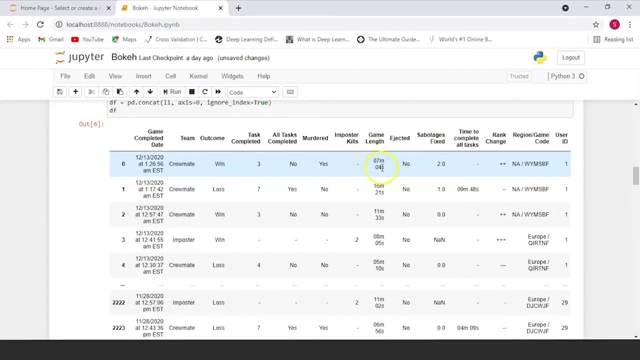 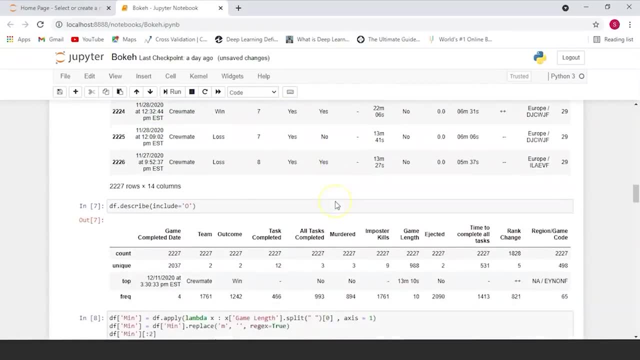 that we're going to be splitting this value, which is 7 minutes 4 seconds, and we're going to be keeping only the first value, which is that of the minutes. the second minutes value is 16 minutes and that corresponds to the second value in our 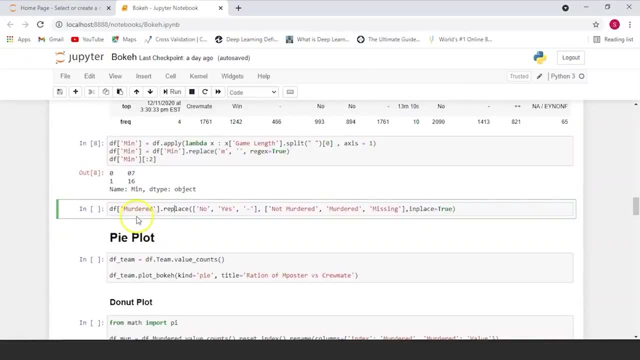 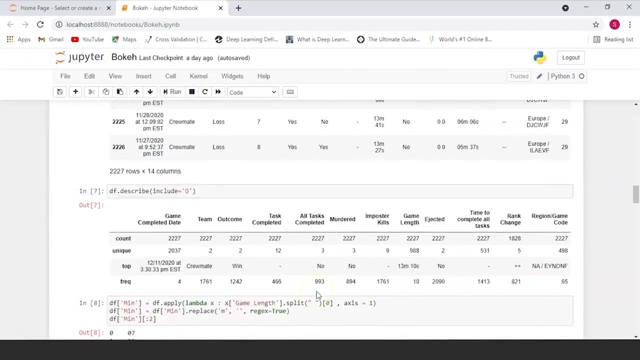 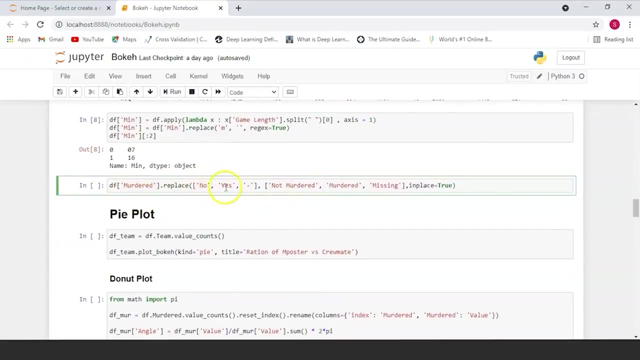 minutes feature variable. now let's take a look at the murdered column. the murdered column has yes, no, yes, no values and missing data set and missing values. so let's change those. we're going to be replacing no values with not murdered, yes values with murdered, and the 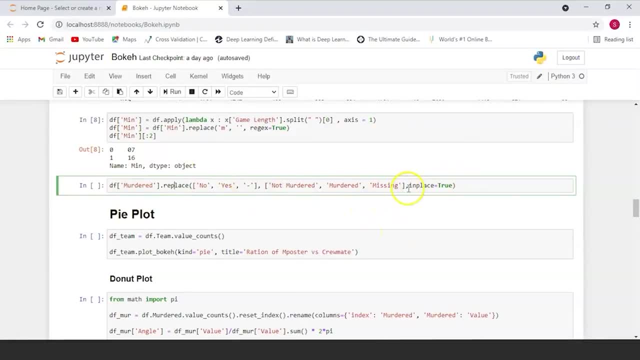 simple dash with missing, and we're going to be doing this in place, which basically means that this is going to make a change to our main data frame. so this is done. let's take a look at our data frame now. this is what our data frame looks like. 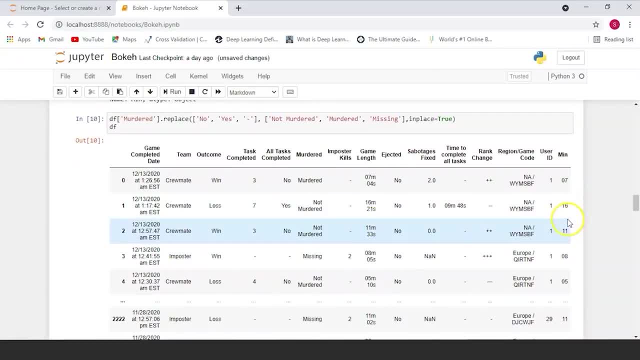 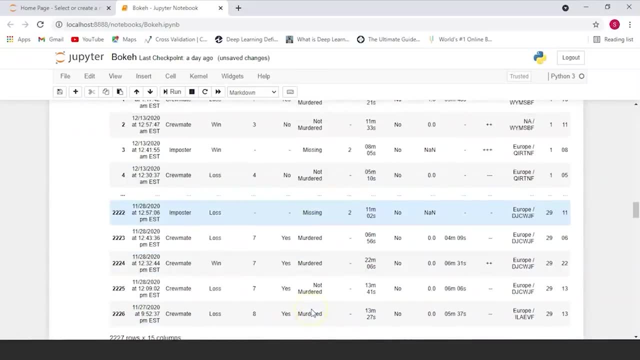 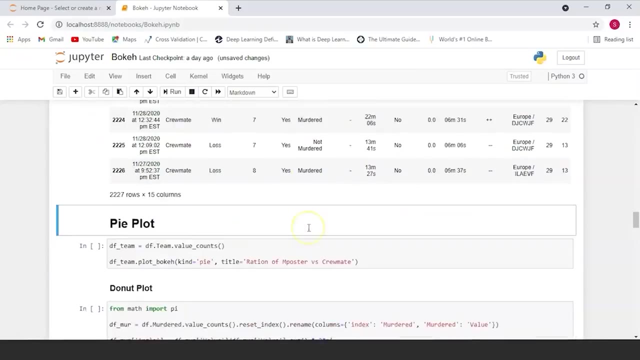 we have a games length column, we have a minutes column and we also have made changes to our murdered column, which is represented here. so now we don't have any missing values or dashes in our murdered column. we have all of it represented as categorical data and this is one of the main columns that we're. 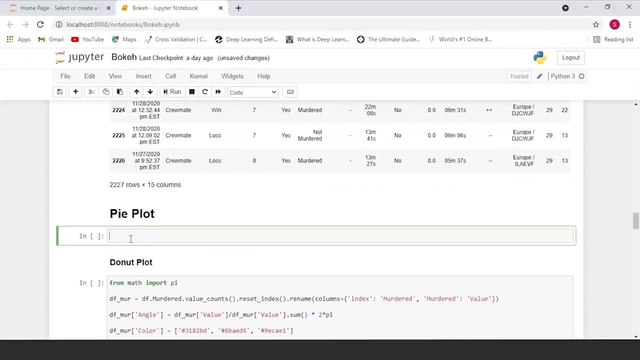 going to be using to plot our pie plots. so now let's see how we can plot a pie chart. the first thing that we're going to be doing is that we're going to be getting the total value counts in our team column here. so we're going to be 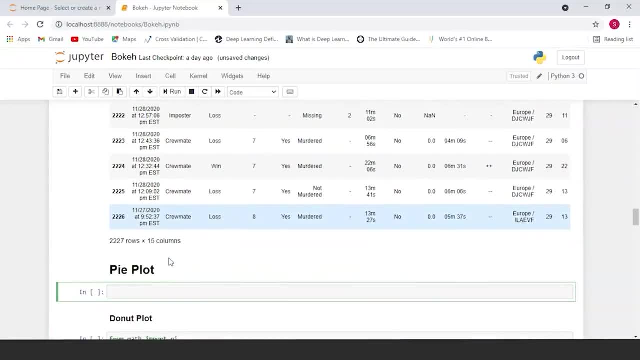 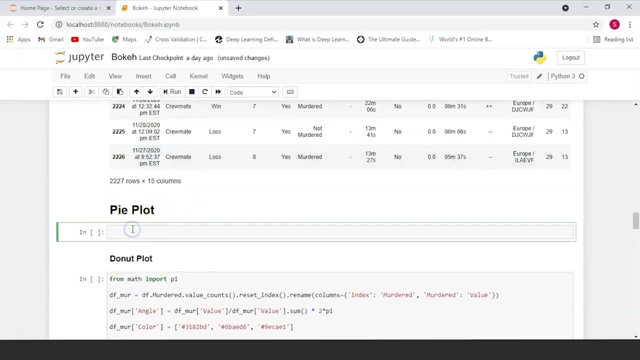 plotting a pie chart with the help of this team column and we're going to be getting the value counts of each unique value in the team column. so let's, you can do this with the help of the value counts function that pandas data frames, provides us with 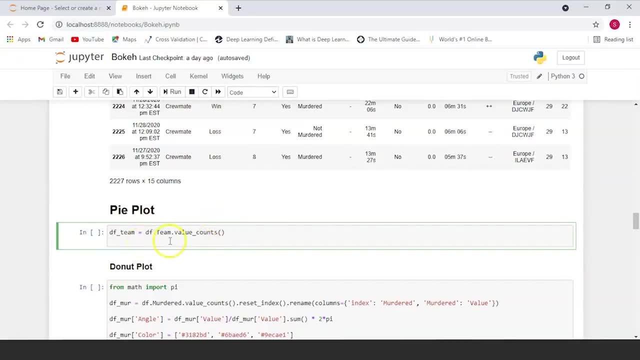 and now that we have the value counts of each unique value, which is present in our team column, let's plot it in the form of a pie chart. we're going to be doing this with the help of the plot bouquet function and the type of chart that we want to plot. 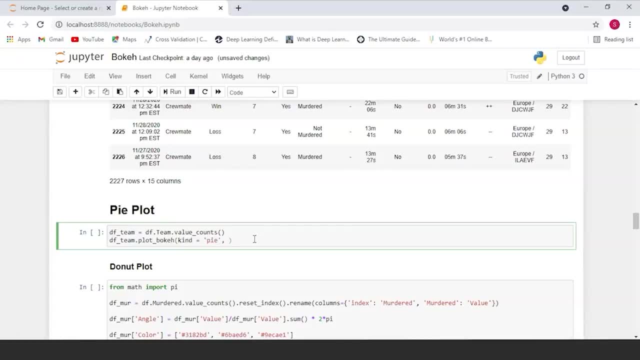 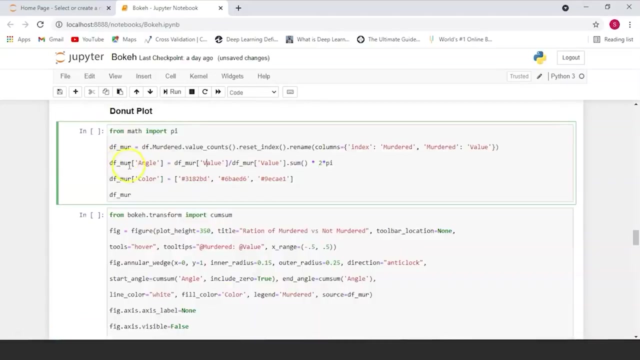 is a pie chart. let's give it a title as ratio of imposters versus crewmates, and let's run this now, and this is what your pie plot looks like after you've plotted it. so now the same thing can be done to plot a donut plot. 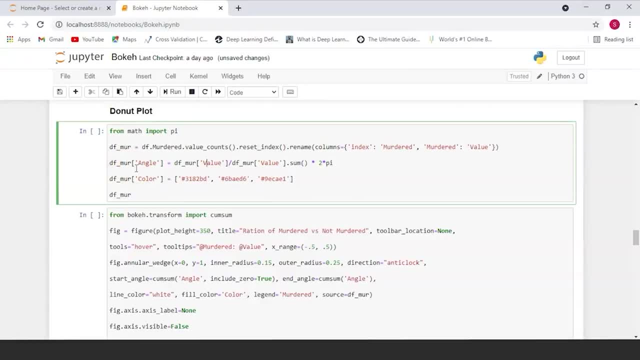 the first thing that we want to see is if there are more crewmates or imposters, murdered or not, in the game. to do this, we will add two more features- angle and color, which are going to be used in the chart. so to get angle, we're going to be importing pie. 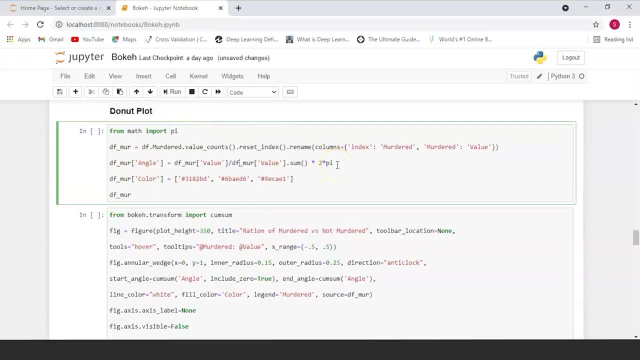 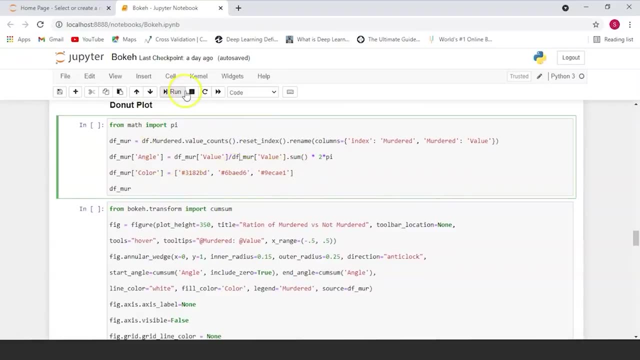 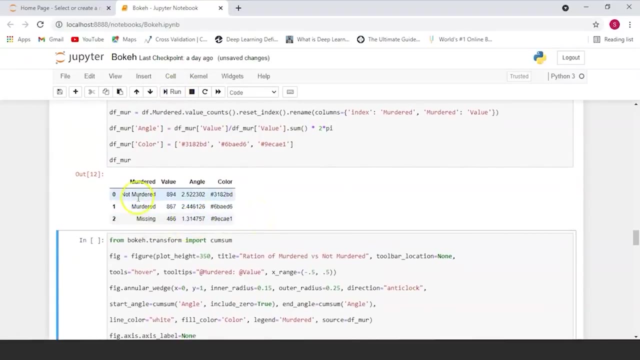 from math and we're going to be converting our angle in the form of radiance. and as for the color feature, we're going to be having three different shades of blue. so this is basically what our murdered data frame looks like. so, over here, you have not murdered. 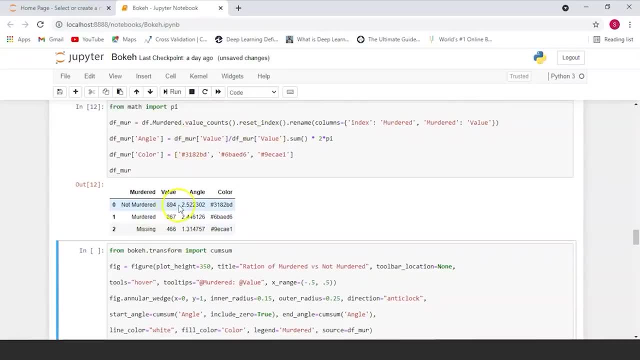 the total value counts of which is 894, and the angle that this gives us is 2.522302, and this is the corresponding color. the same goes for murdered, which is 867 values, and we've converted that into an angle in radiance and given it. 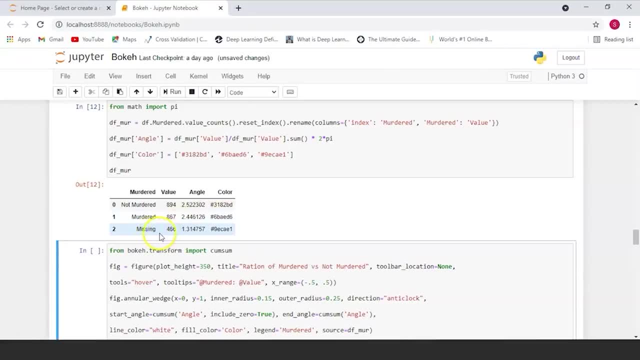 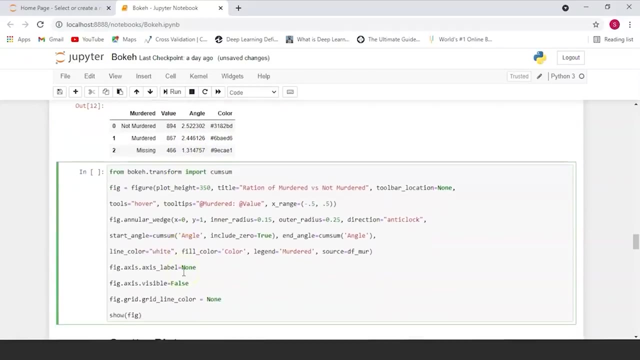 its own color. and finally, we also have missing values, of which there are 466. the angle is 1.314756 and it has its own corresponding color. so this is a data frame that we're going to be using to plot our donut chart. so, from 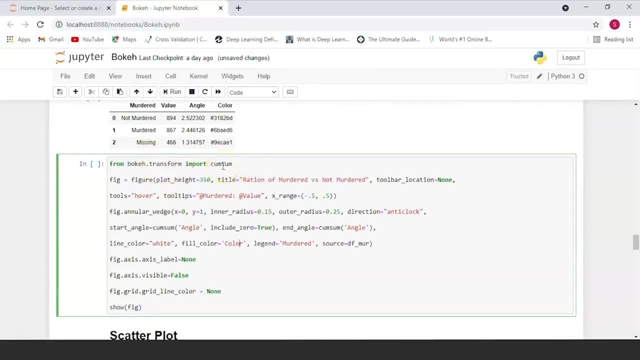 bouquettransform, we import cumulative sum and the cumulative sum is what we're going to be using to find the start of our angle, or basically to find, or basically to find how much portion of our donut chart is going to be occupied by the angle. so the donut chart can. 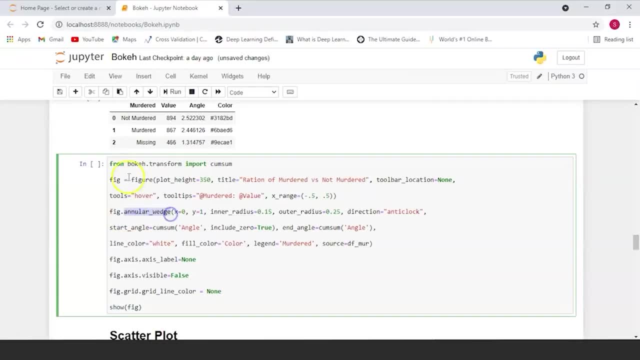 be plotted using the angular wedge function from figure. so the x axis here is 0 and the y axis is 1. the inner radius is the radius that you are going to be giving to the inner smaller circle and that we've given as 0.15 the outer radius. 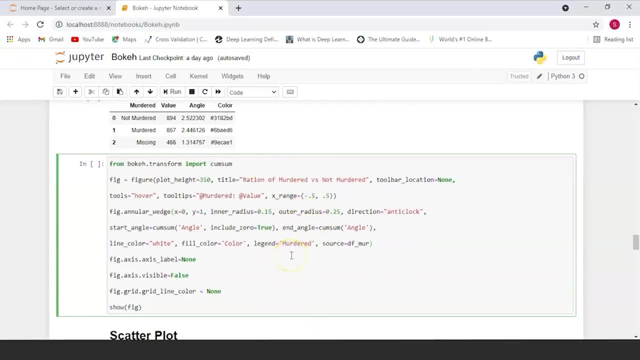 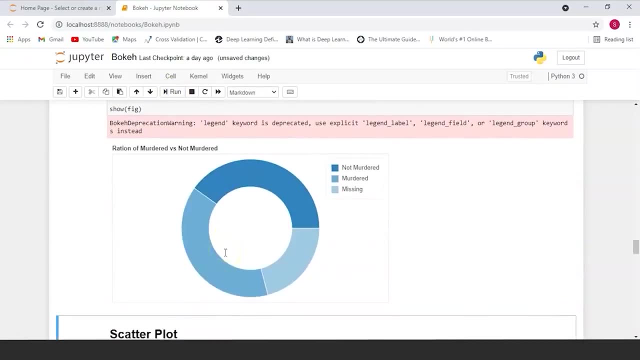 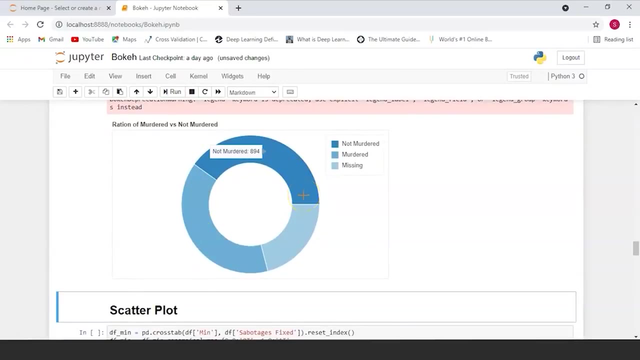 is the radius of the bigger outer circle, and the direction in which our data is going to be plotted is in the anti-clockwise direction. so let's run this, and this is what our donut chart looks like. so the not murdered is this dark blue color. 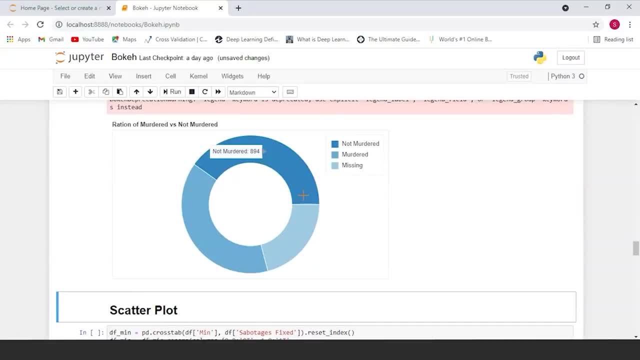 portion of our donut chart and when you hover over it, you can see how many values are present in the not murdered column. the same goes for murdered, and, because we've plotted our data in the anti-clockwise function, this is how it's being plotted. so murdered, not murdered, and then finally. 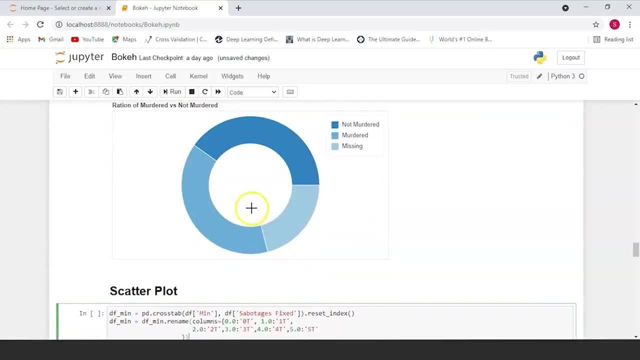 you have the missing values. the way that you can interpret this graph is that you can say that most of the people were murdered during the game, but most of the data is missing, so we can't say for certain whether the majority of the people were murdered during the game or not. 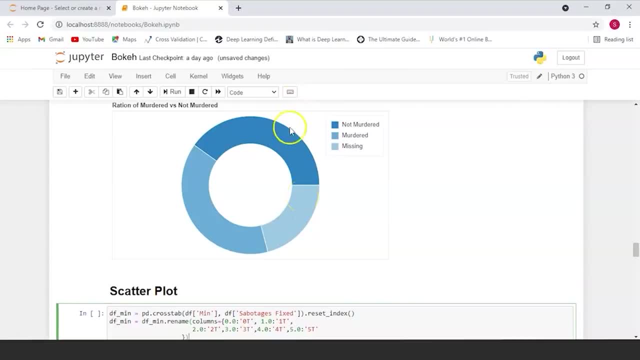 because the number of missing values can make a huge difference and the number of people who were not murdered and the number of people who were murdered are very close to each other, like their total values are very close to each other. next, we will create a data frame of: 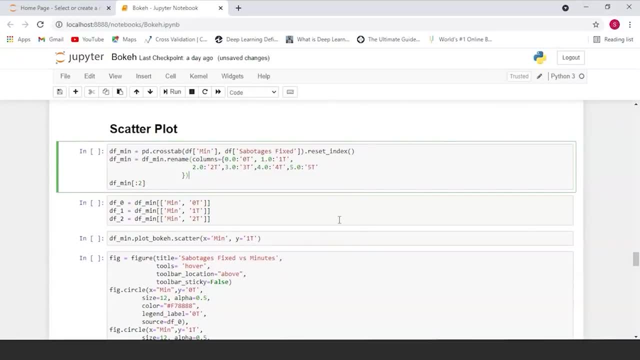 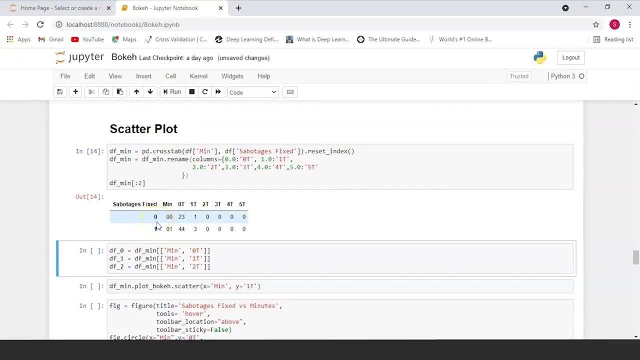 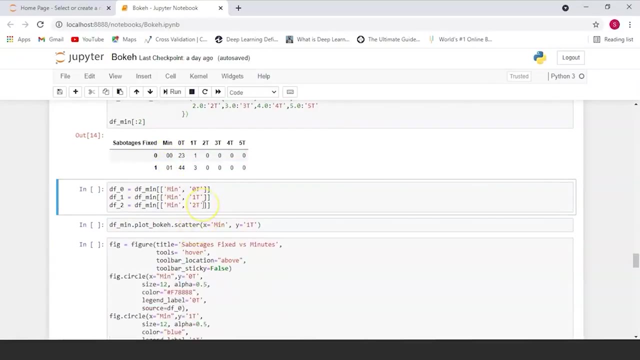 sabotages fixed and minutes and change the column name and add t in them. so this is basically what we're doing. we've created a data frame which has the number of sabotages fixed and the minutes. now let's just take the sabotages which were fixed. 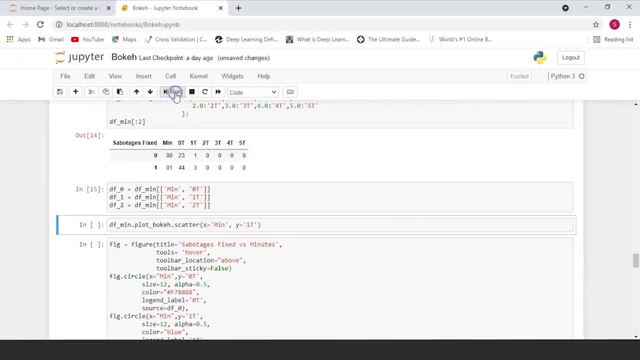 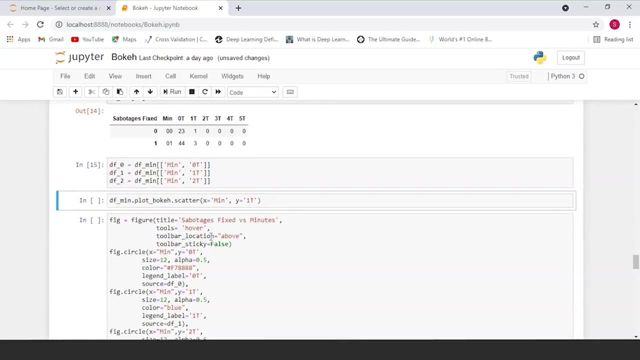 which is 0,, 1 and 2, and create a data frame out of all of these. so each of these individual data frames just contains these individual columns. to make a simple scatter plot with only one legend: we can pass the data and use scatter to make the charts. 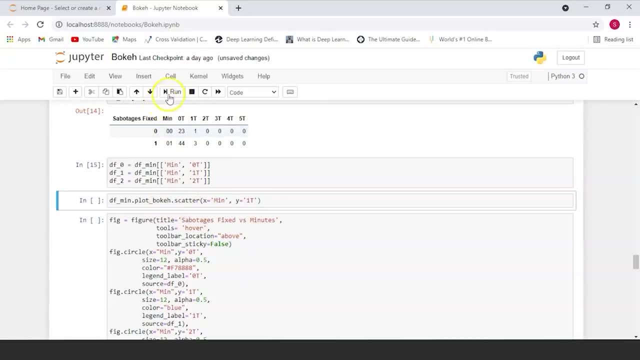 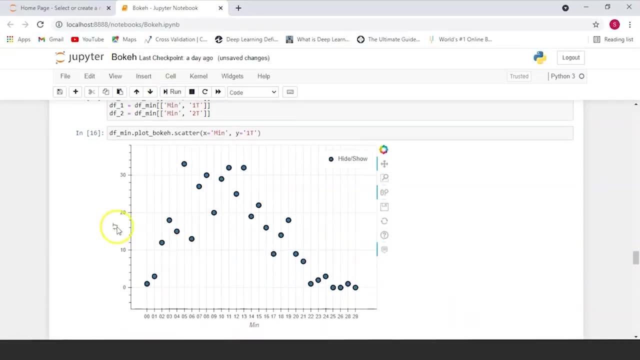 so basically we're just plotting the scatter chart in Bokeh here and this is what our minutes scatter chart looks like. now we're plotting this for 1 t. we're plotting the minute at which one sabotage was fixed. and another cool thing about Bokeh charts is that 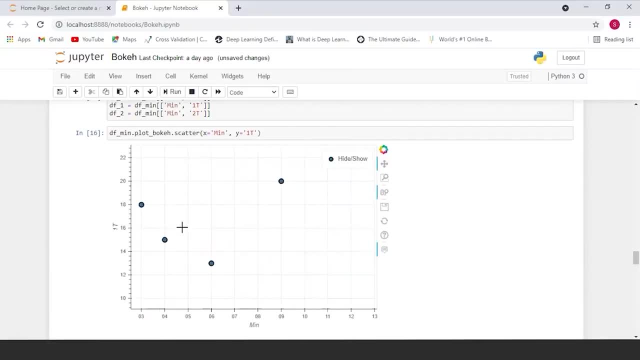 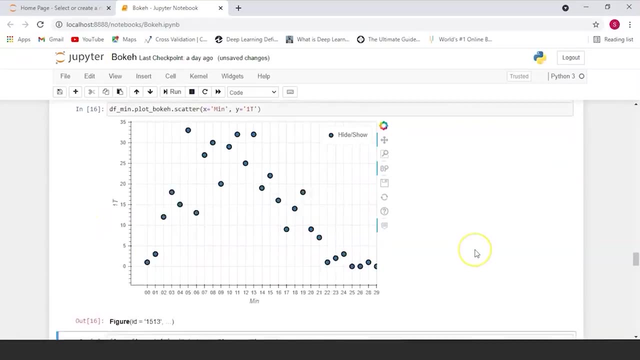 you can always zoom into them or zoom out of them to better see where your data is plotted. so this is a scatter chart which has only one variable, which is 1 t, and the minute at which it was plotted. to make a scatter chart with more variables. 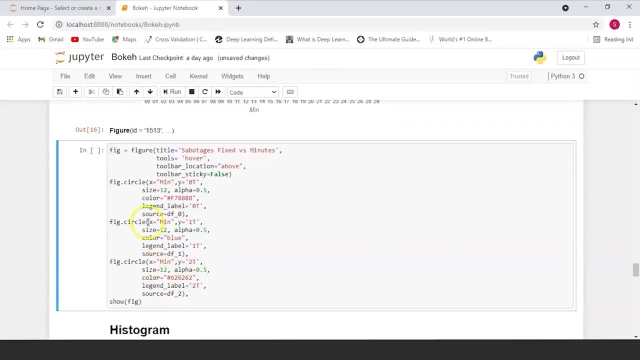 we are going to need to use circle, which is a method of figure object which we've already seen before. the circle is one of the many plotting styles which are provided by Bokeh. you can also use triangles or many more. you don't have to make each point. 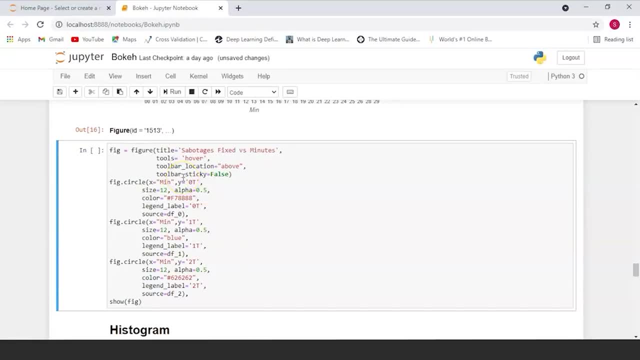 a circle. so we're gonna be plotting. so we're gonna be plotting the sabotages fixed and the minute at which they were fixed, and we're gonna be plotting 3 different circles of 3 different colours and each of them correspond to how many sabotages. 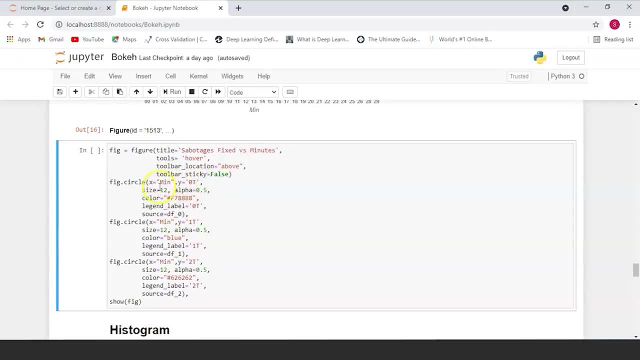 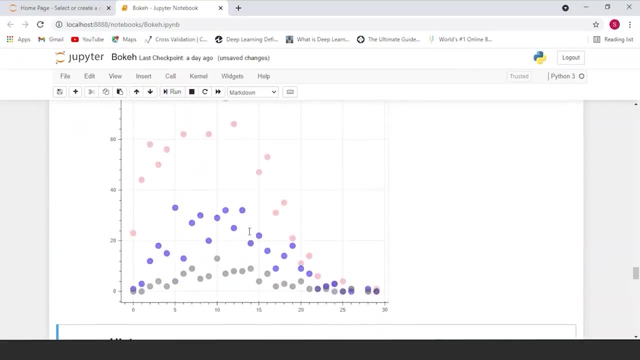 were fixed at what time. 0 sabotages at what time, 1 sabotage at what time and 2 at what time. so let's run this so, as you can see here, when 0 sabotages were fixed, these were the times when 1 was fixed: this. 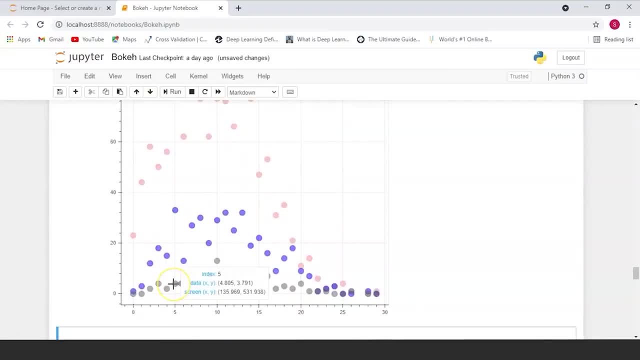 was the time at which it was fixed and when 2 was fixed. this is the time that it was fixed at, so the x-axis is our minutes and the y-axis is the sabotage. when you hover over it, you can see various information about where each circle is plotted. 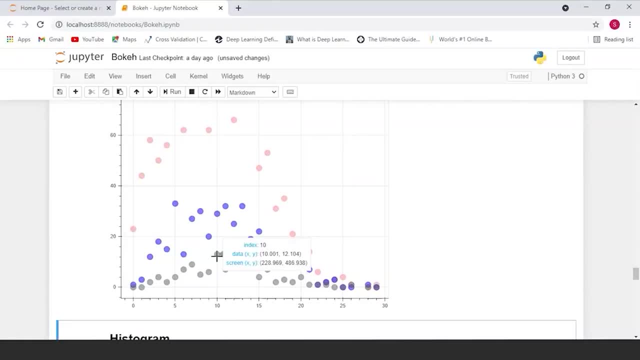 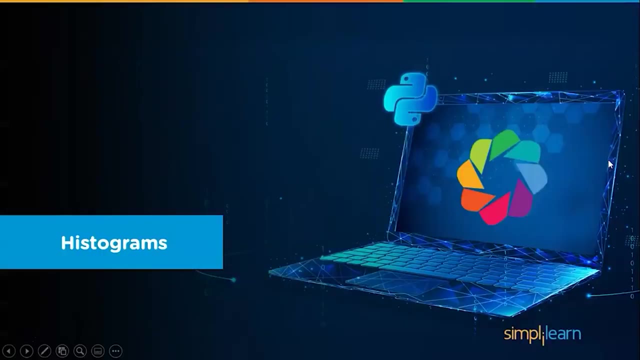 so this has an index of 10. the data xy will tell you the exact x coordinate and the y coordinate, and the screen xy will tell you the screen pixels on which it is plotted. so now we've taken a look at pie charts, let's move on to histograms. 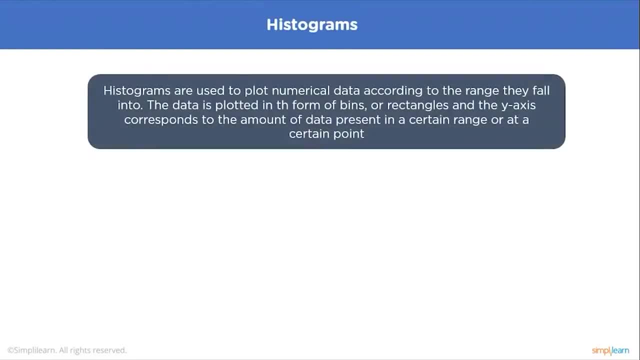 so what exactly is a histogram? histograms are used to plot numerical data according to the range that they fall into. the data is plotted in the form of bins or rectangles, and the y-axis corresponds to the amount of data present in a certain range or at a certain point. 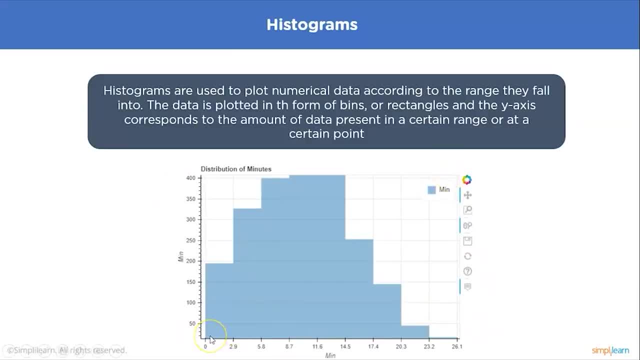 so this is what a histogram looks like. this is a histogram of the distribution of minutes, so the x-axis has the range within which this data falls, like over here the first range is from 0 to 2.9, and second one is from 2.9 to 5.8. 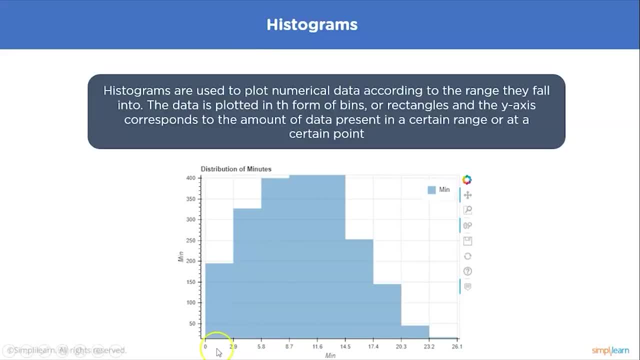 each range has a value of 2.9 and the corresponding y-axis, or the height of the bins, tells us how much data is present within this range. so this is how you can read histograms. now let's see how we can plot them using python bokeh. now let's see the. 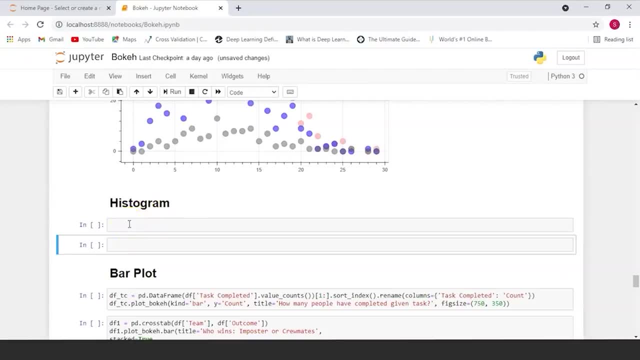 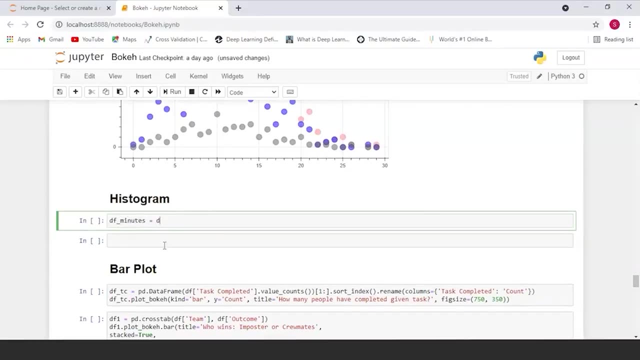 distribution of minutes in the among us game, we will use hiss to plot a histogram. so basically, we're just going to be plotting the minutes of our game. we're gonna be using the df min column for this and we're gonna be converting it into an integer. 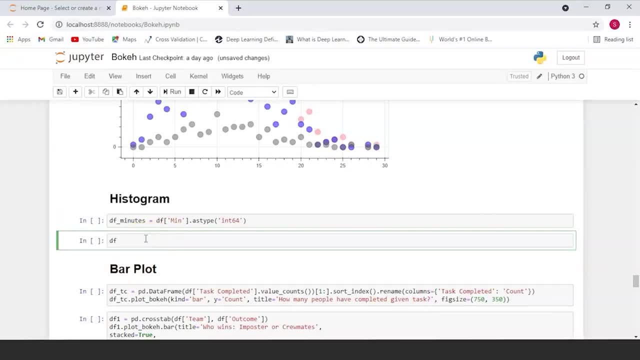 so this is the column that we're gonna be plotting. let's plot this again. we're gonna be using the plot bokeh function here because it makes plotting data frames very easy. the kind of data frame that we're gonna be using is the histogram, or hiss. 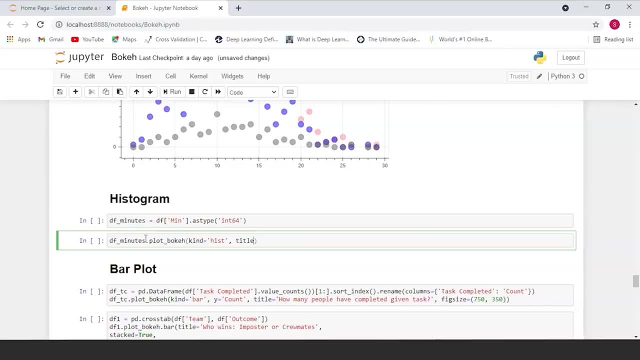 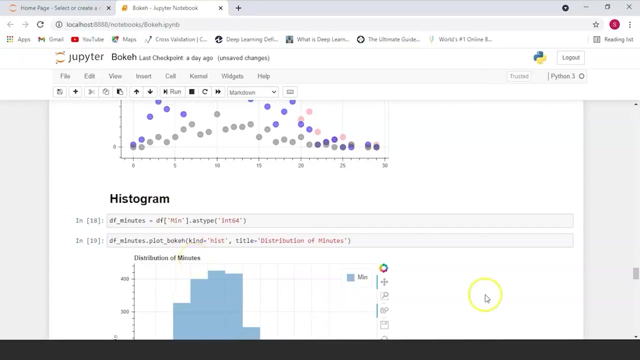 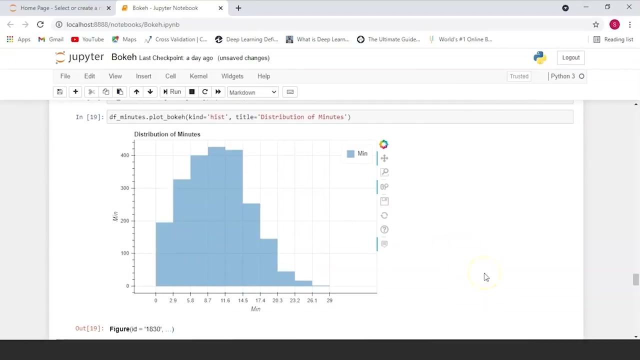 and the title of our graph is going to be distribution of minutes. so let's run this now. this is what our histogram looks like now. this is when we've only plotted one variable, which is minutes. yes, so another thing that you can plot is a stacked histogram. 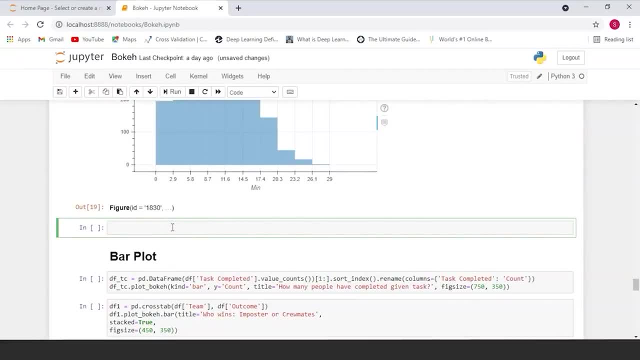 a stacked histogram is when you plot various histograms on top of each other. so let's see how this works for a stacked histogram. we want to see if the game length has a correlation with the amount of imposters and crewmates in our game. so to do, 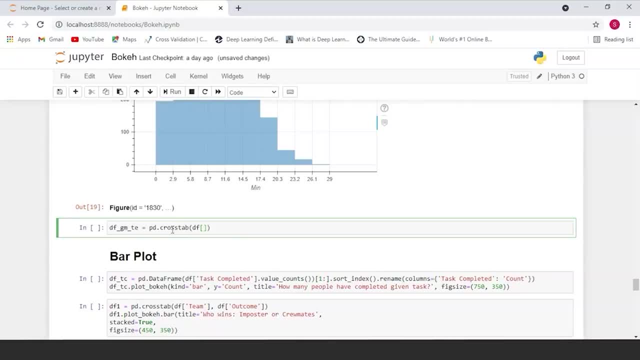 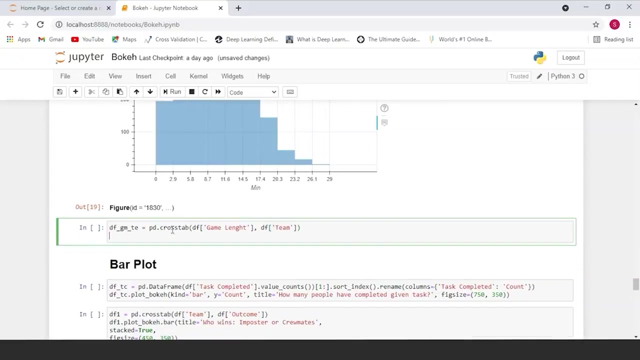 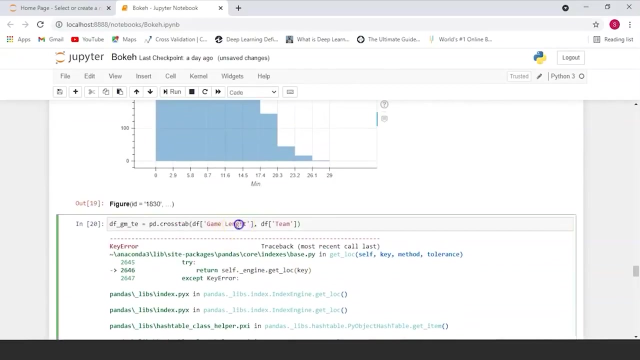 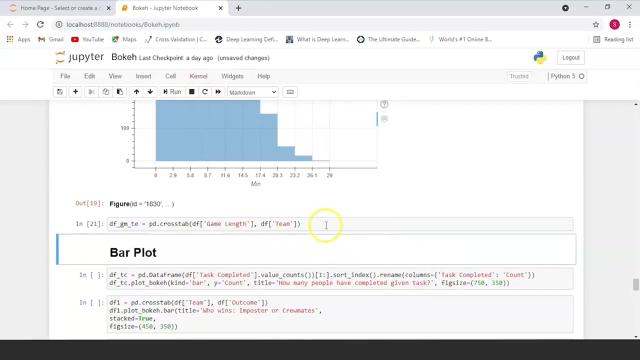 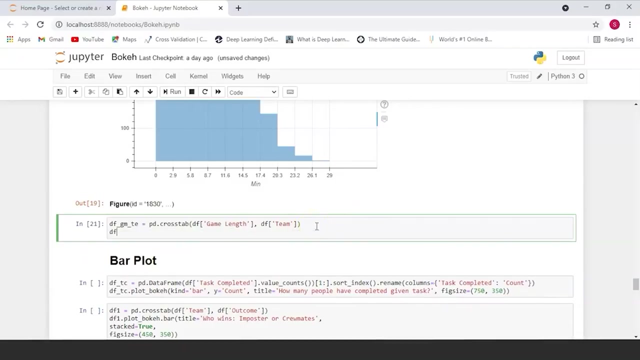 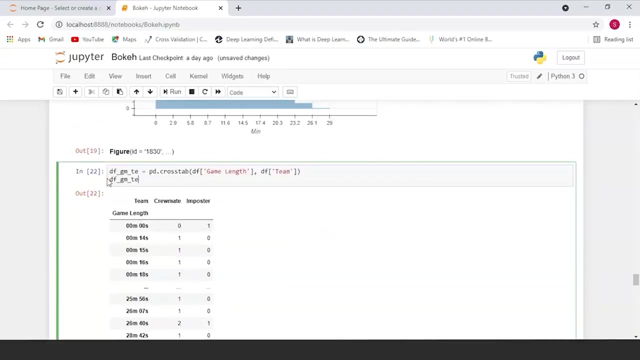 this. we're gonna be creating a small data frame which has the game length and the team columns combined. so let's do that, and this is what this looks like. so all you have to do to plot this in the form of a stacked histogram is use the hiss function again. so 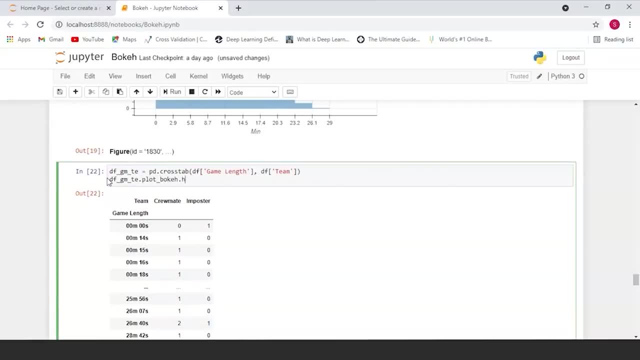 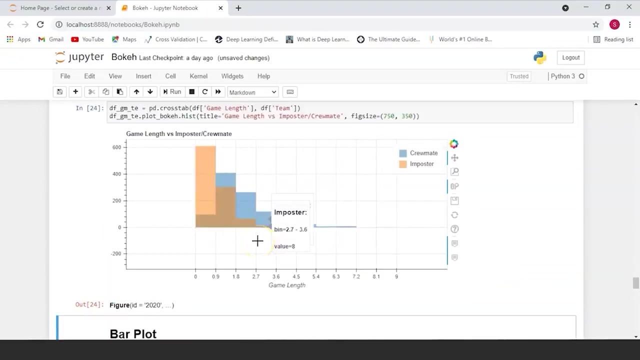 let's see how that is done. and let's give this figure a size of, say, seven percent, and let's give this figure a size of, say, 50 comma 350. so let's run this again and this is the stacked histogram that you get. we have two different columns which are plotted. 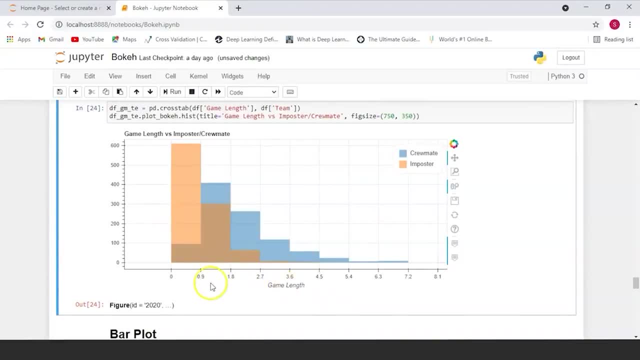 on top of each other versus the game length. so basically, this tells us that when the game length was between 0 to 0.9 minutes, the number of imposters was way higher than the number of crewmates, and the longer the game went on, the number of imposters. 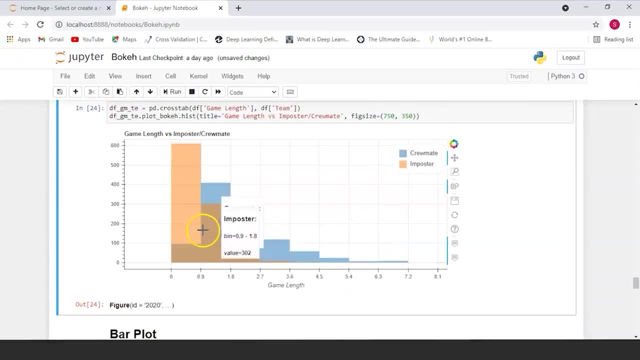 decreased and the number of crewmates just kept getting longer and longer. now, obviously, you can say that the number of crewmates is decreasing as the game goes on too, but this is because the imposters would have killed off most of the crewmates. as you can see here, towards the end, there are 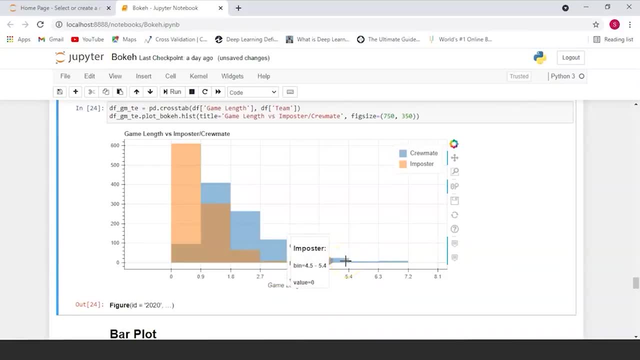 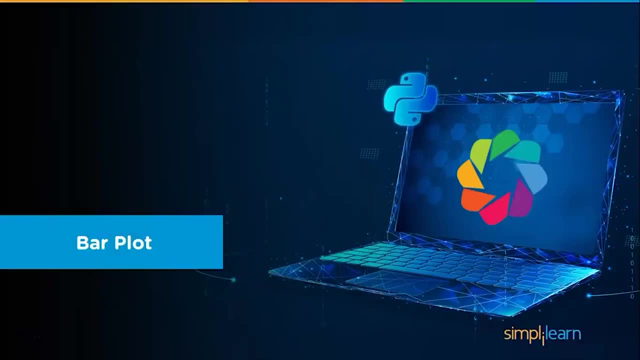 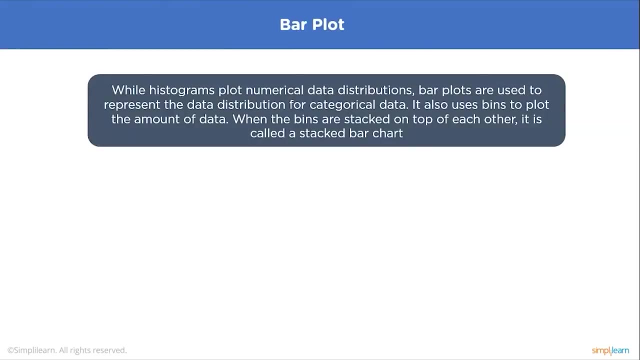 no imposters, which means that most of the imposters were ejected and the crewmates won. so now we've taken a look at histograms. let's move on to bar plots and understand how exactly they are different from histograms. so in histograms you have plotted numerical data distributions. as of yet, 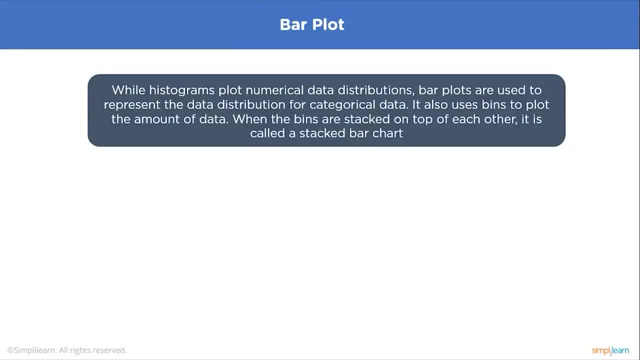 in bar plots, you plot for categorical data. it also uses bins to plot the amount of data when the bins are stacked on top of each other. it's called a stacked bar chart. this is basically what a bar chart looks like. the difference is this does not have its own range. 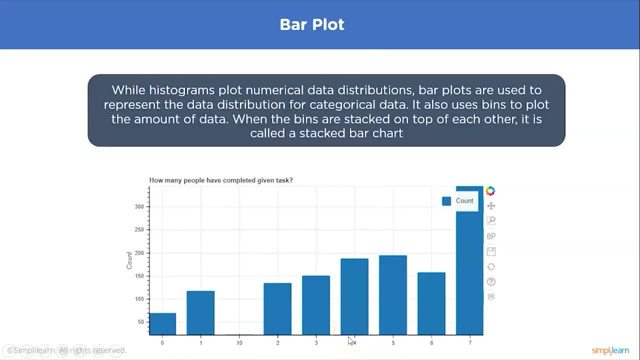 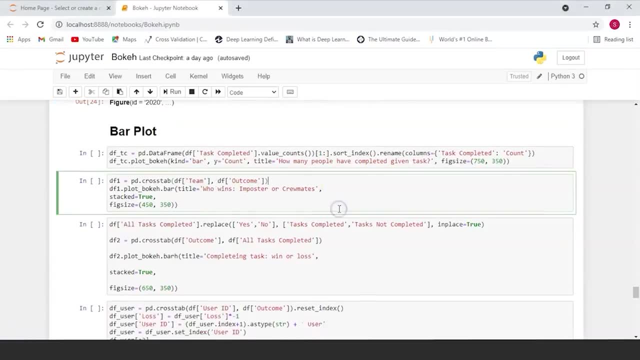 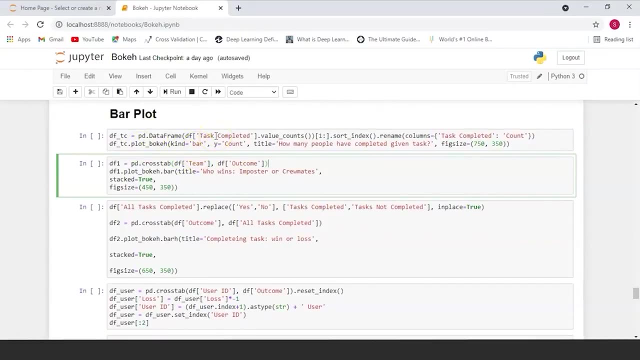 each bar is used to represent a categorical data, and the height is used to tell us how much of that categorical data is present. so now let's see how we can plot a bar plot. so again, we're gonna be making a small data frame of the task completed. 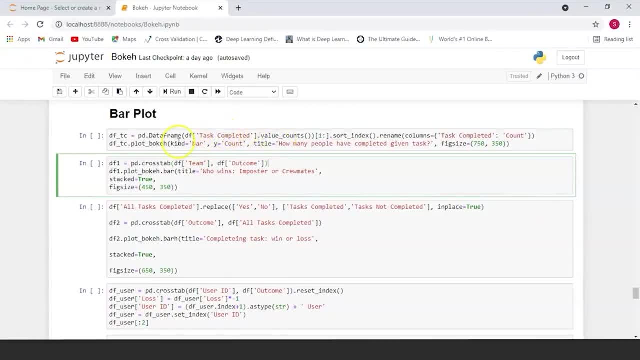 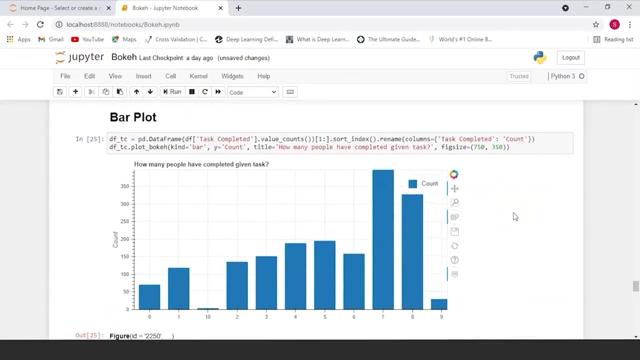 and the value counts of how many tasks have been completed. to plot a bar plot, we're gonna be using plot bouquet again, and the kind of plot that we want to plot is bar, so let's run this and see what we get. so here is your bar plot. 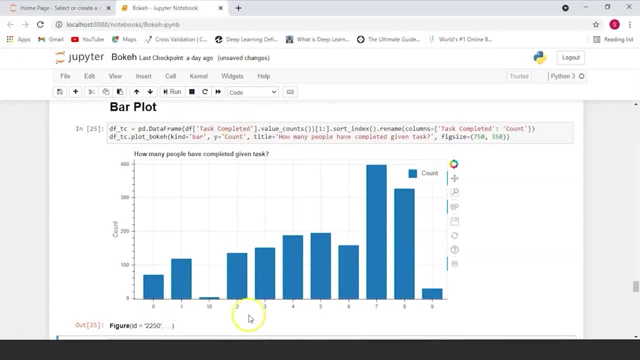 the task completed in this case is categorical data and the counts basically tells us how many value counts fall into each category. so 0 tasks completed are 69, 1 task completed is 117, 2 tasks completed is 10 and so on. from this bar chart you can say: 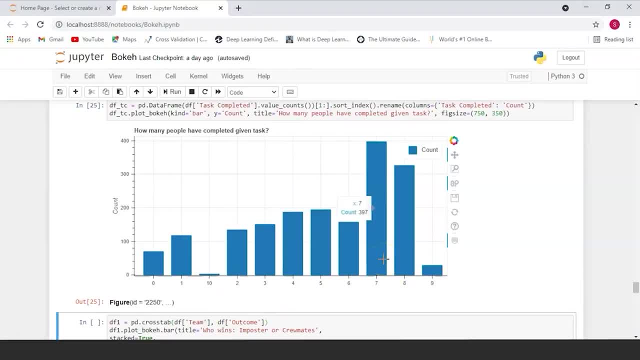 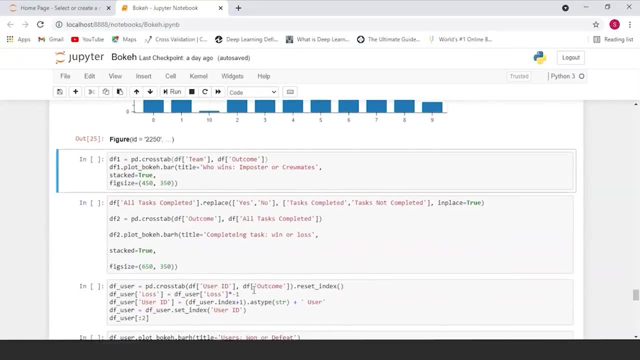 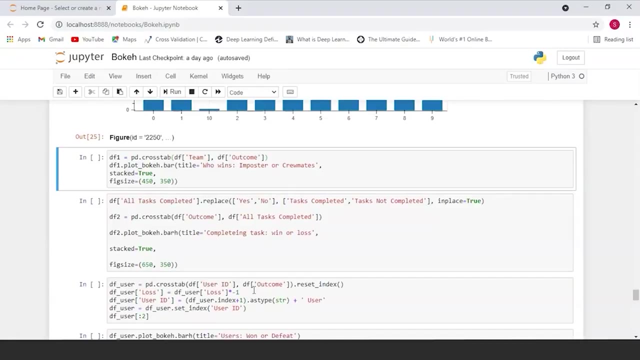 that the most number of tasks completed is 7 and the least tasks completed are 10. now let's create a stacked bar chart and let's see who wins- imposters or crewmates to create a stacked bar chart. what we're gonna be doing is that. 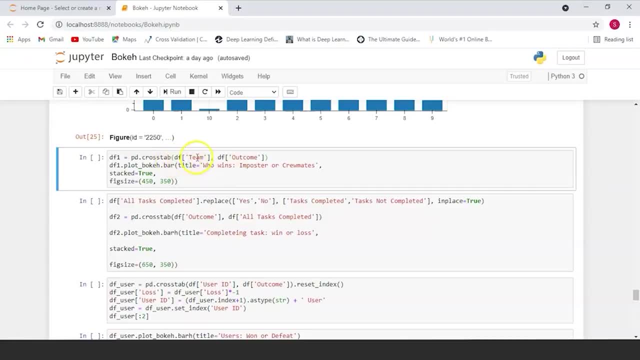 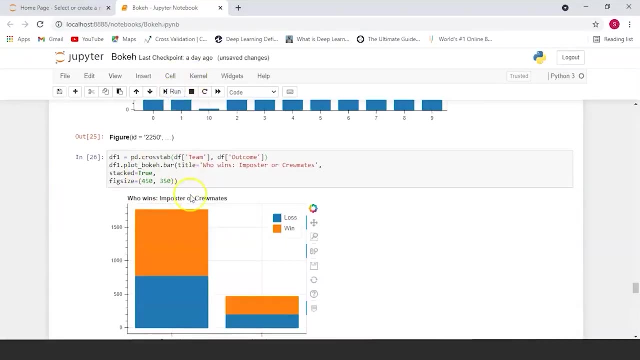 we're gonna be creating a different, smaller data frame of team and outcome. to make sure that the bar chart is stacked, all you have to do is include a stacked attribute in your bar function and change its value to true. so let's run this and see. and here you can see. 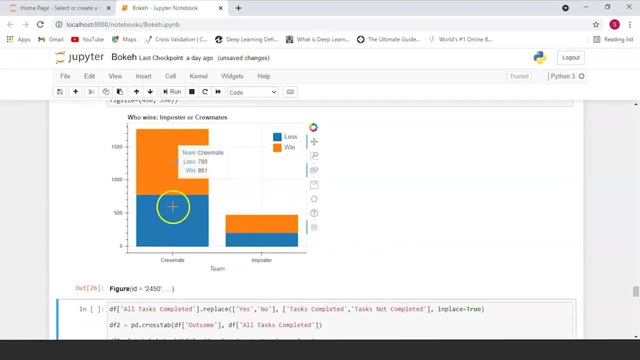 that we have a stacked bar chart, so you can see that crewmates, who have a lot more data, have won 981 times and lost 780 times, while imposters have lost 205 times and won 216 times. so the crewmates have won significantly, far more than the number of. 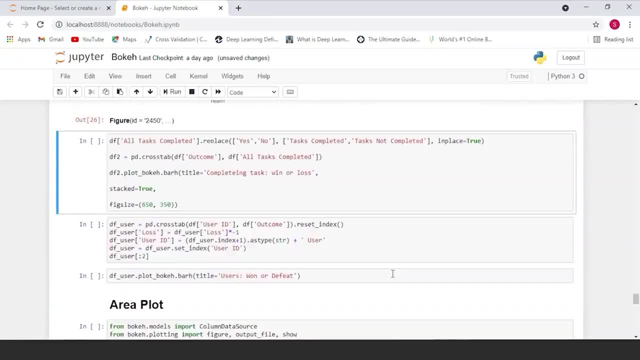 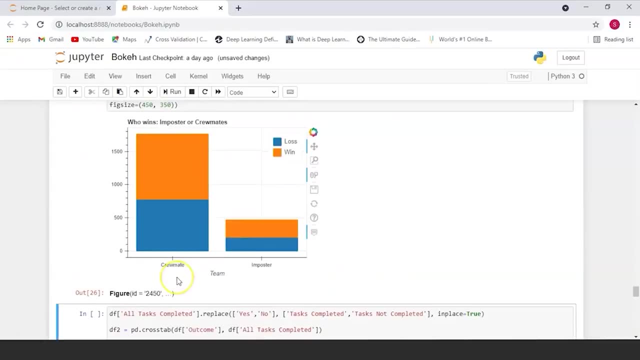 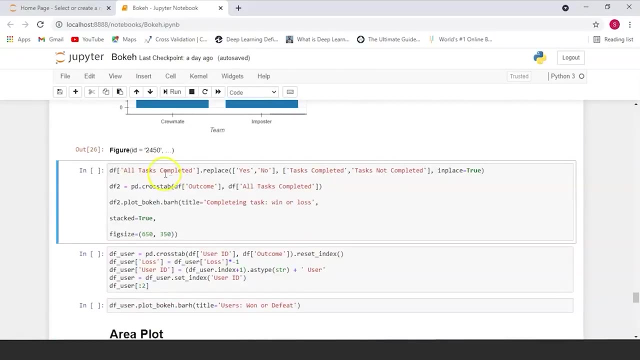 times imposters have won. now let's take a look at stacked vertical bar charts. so so far, the bar charts that we've been looking at have been horizontal, which means that the data goes upwards. for a vertical bar chart, we're gonna be seeing if all tasks have been completed or not. 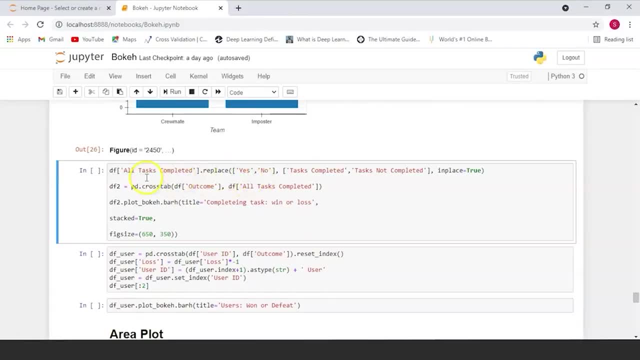 so in the data frame column all tasks completed, we're gonna be replacing the values of yes and no with tasks completed and tasks not completed. we're also gonna be creating a smaller data frame of the outcome column and the task completed column to plot a stacked vertical bar chart. 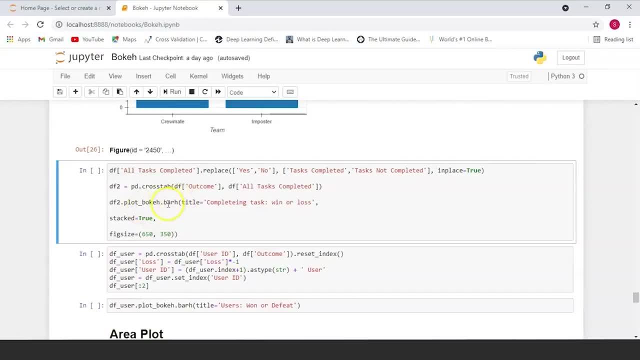 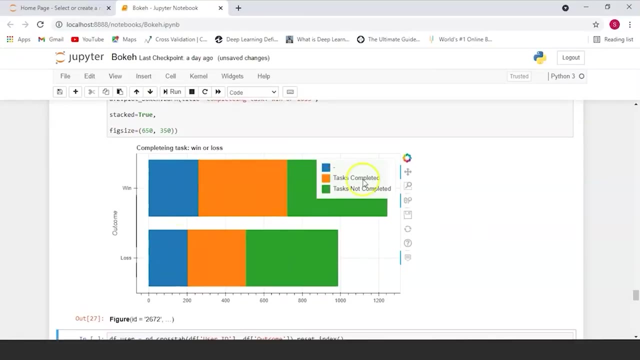 you're gonna be using python bouquet dot bar h function and you're gonna be changing the stacked attribute to true. this is what a stacked horizontal bar chart looks like. so over here we can see that the missing values is represented by blue, tasks completed by orange and tasks: 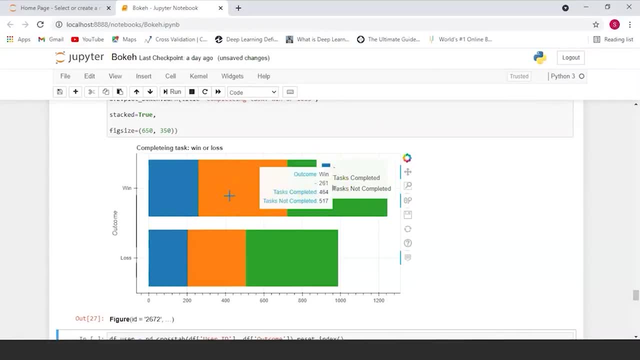 not completed by green. here you can see the total outcome. you can see how many wins, how many tasks are completed and how many tasks are not yet completed, and the same goes for losses. you can see how many losses have occurred, how many tasks are completed and how many. 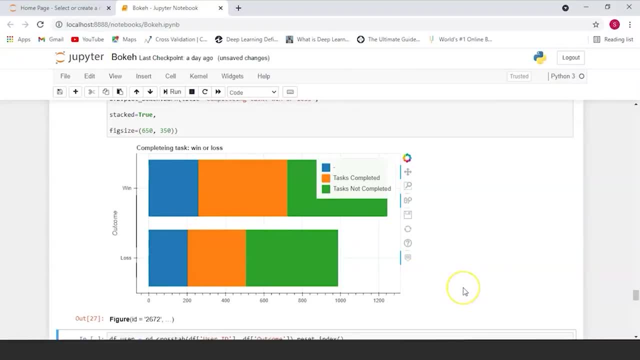 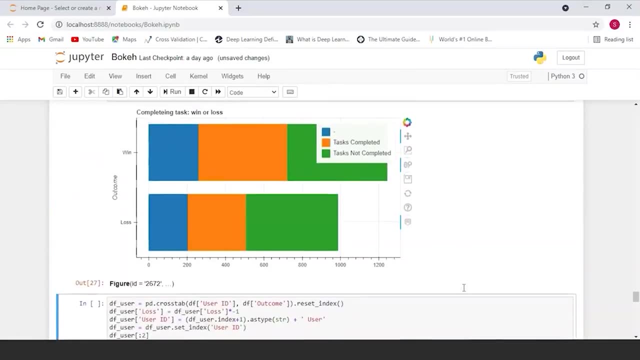 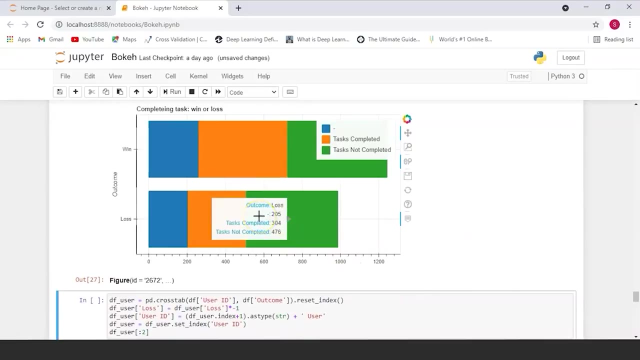 tasks were not completed. this is a very good way of representing a lot of data in a relatively smaller area. now the way we can interpret this graph is that we can say that finishing the task will automatically ensure that the crewmates have won. there's a higher number of people. 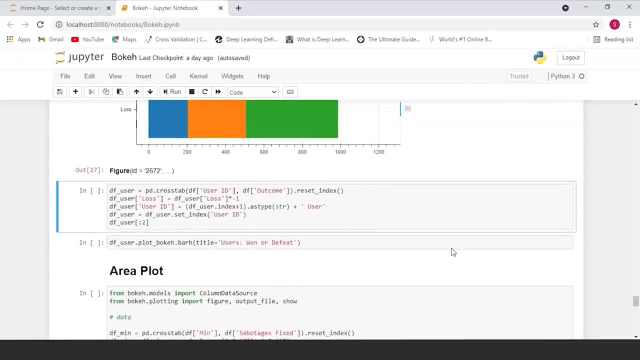 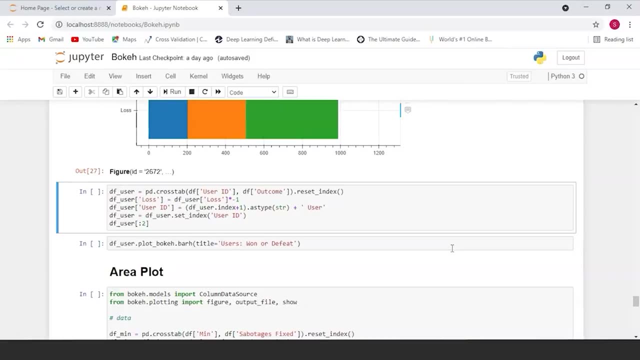 who need to complete the task to win the game. another very unique type of bar chart that you can have is a bidirectional bar chart. so let's plot a bidirectional bar chart in which the bars will be going both ways, to the left and to the right. we're gonna be. 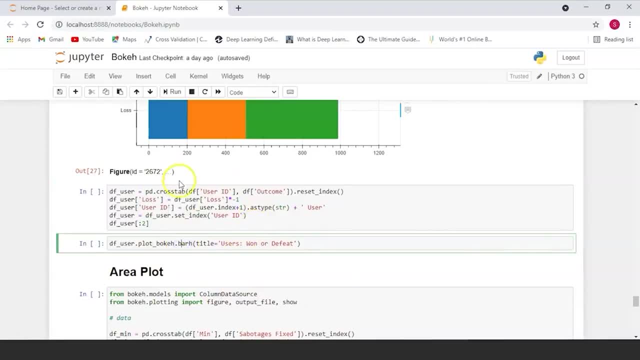 plotting a horizontal bar chart over here to make it easier for you to see. to have a bidirectional bar chart you need positive values and negative values. the center is going to be at zero. so here we're gonna be making the loss features negative by multiplying the loss feature with the. 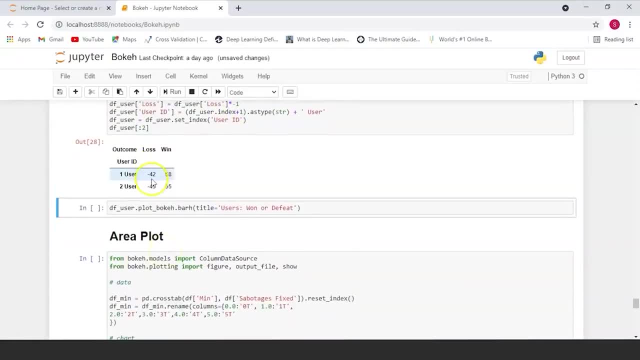 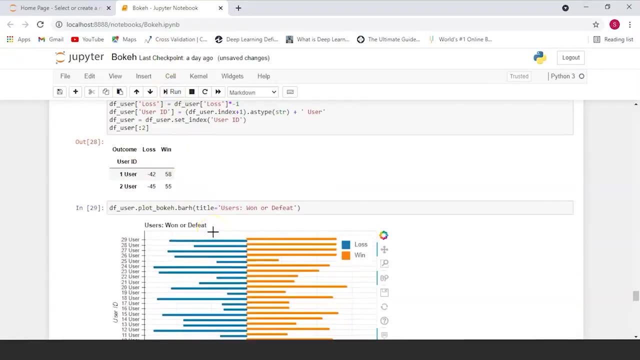 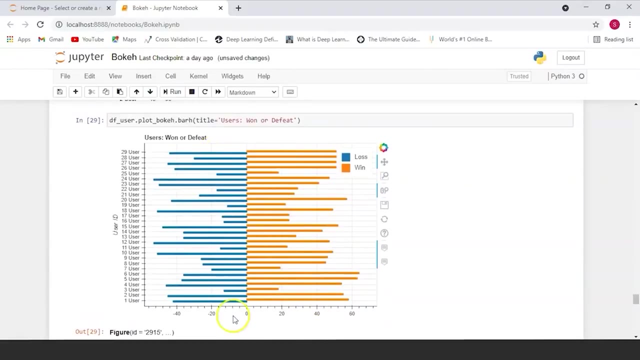 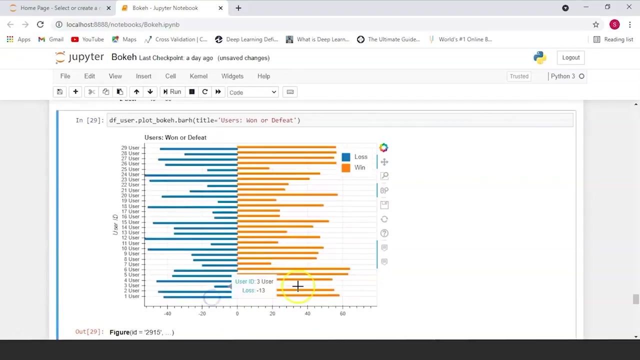 minus one value. so here we go: the losses are all negatives and the wins are all positives. right now let's run this and see how many losses and wins have occurred for each user. so user one has 42 losses and 58 wins, but you can easily. 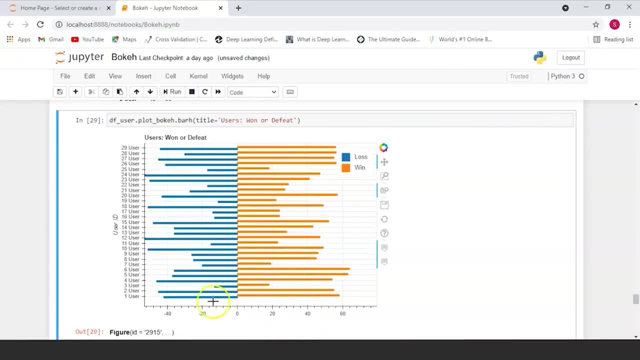 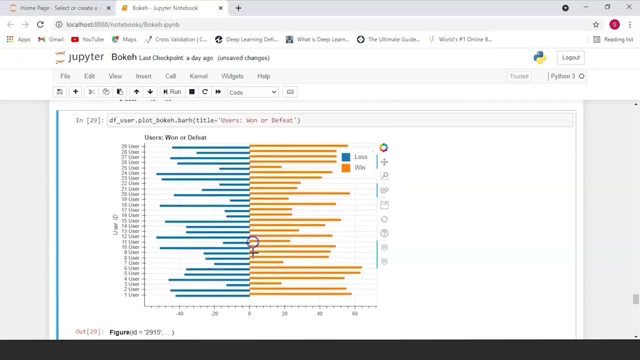 see whether they have won more or lost more by comparing the height of the bars for the wins and the losses. so we can easily say that in this scenario, user one has won more times than they've lost. the same can be said for user two, where the wins bar 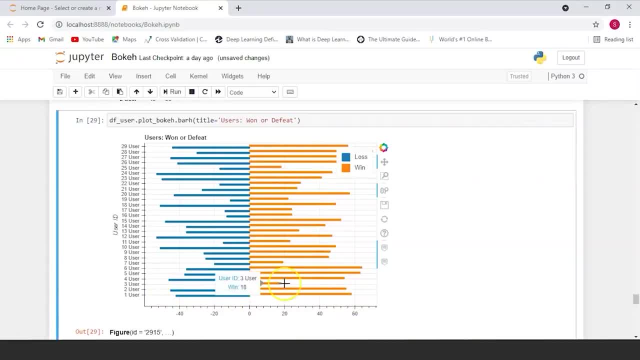 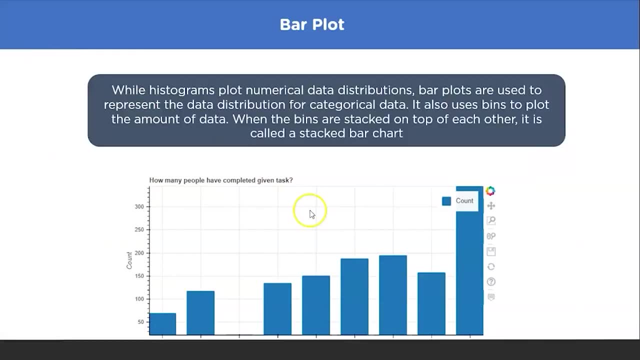 is significantly higher than the losses bar. so this is how you can plot and understand a bidirectional bar chart. so we've taken a look at how we can plot bar charts and the various types of bar charts that are available to us in python bouquet. now let's take a look at area plots. 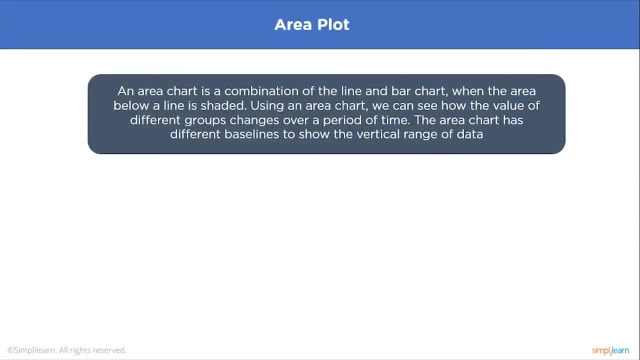 area plots is a combination of the line and the bar chart. when the area below a line is shaded using an area chart, we can see how the values of different groups change over a period of time. the area chart has different baselines to show the vertical range of data. 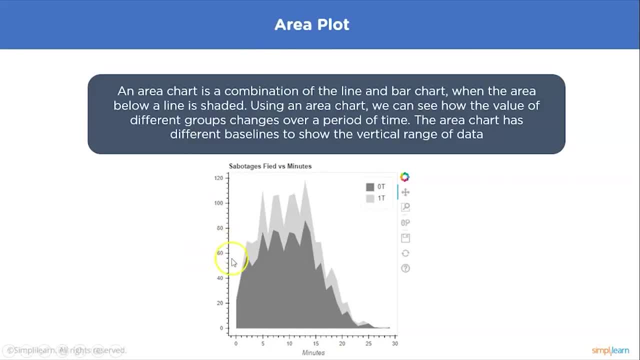 here we've plotted the sabotages fixed versus the minutes at which they were fixed at. so these are the minutes, and the sabotages fixed are of two types: 0t and 1t. so the number of minutes that we're considering here is somewhere around 28. 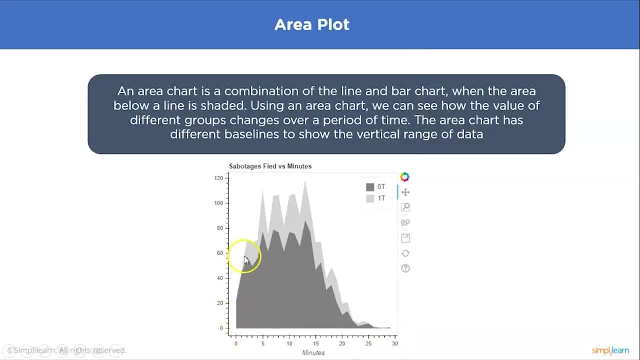 ish and 0t, as you can see, has a way higher value. so one really good thing about area plots, especially in this case, is that they have two ranges and they have another range on the y-axis which tells us how the number of sabotages fixed is ranging. 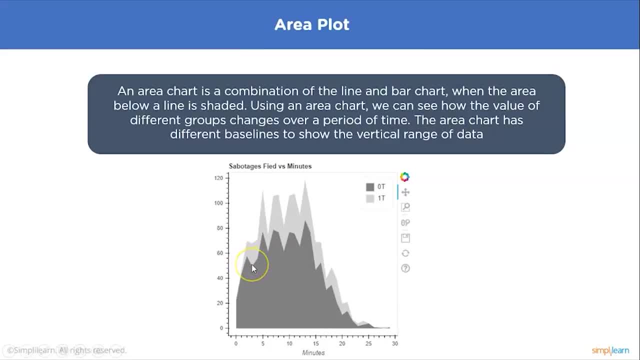 so 0 sabotages fixed. you can see how the value keeps fluctuating and how the value changes for different minutes, and the same can be said for 1t. now 1t has a baseline which is over here, which is just above the 0t baseline. 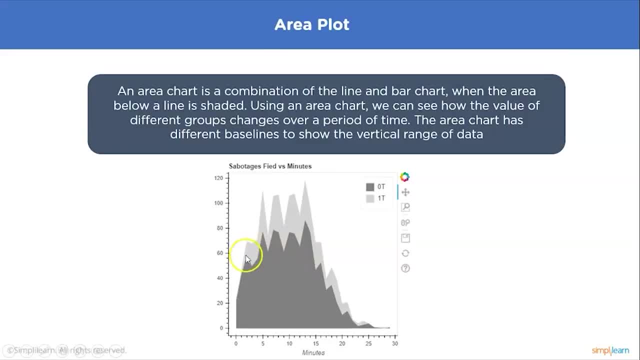 this doesn't necessarily mean that this is where 1t starts and this is where it ends. this just means that it ranges from 0 all the way here, and we can compare very easily how 0 sabotages fixed and 1 sabotages fixed range or change. 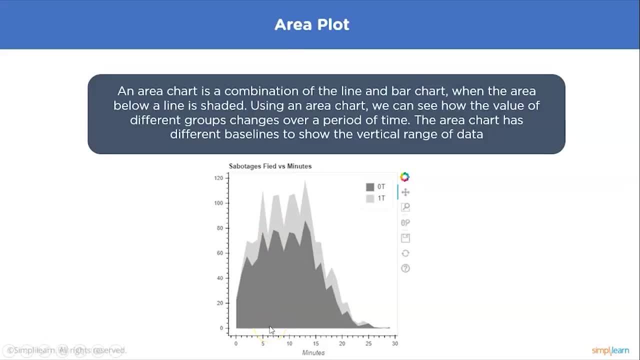 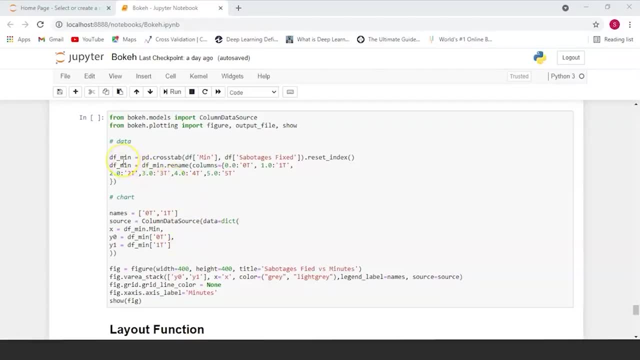 with respect to each other at the same time. now, the first thing that we're gonna be doing to plot our area chart is that we're gonna be creating another data frame- this is called df minutes- which is going to be comprising of the minutes column of our 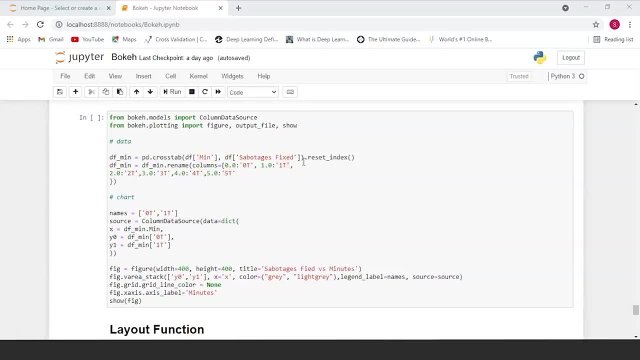 data frame and the sabotages fixed column of the same data frame for df min. we're gonna be renaming the columns to 0t and 1t and the only columns that we're gonna be considering, out of the five different columns that we have, are the 0t and the 1t column. 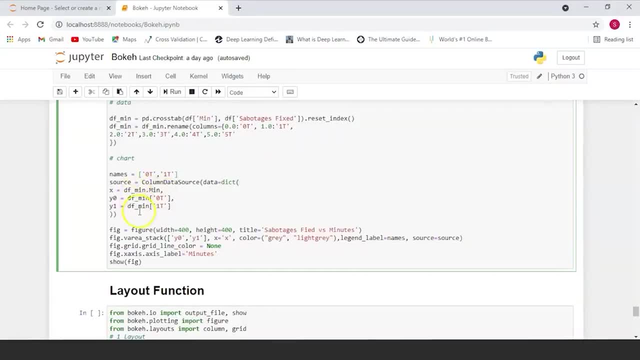 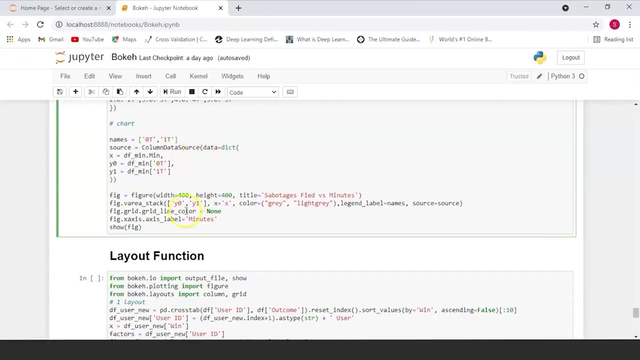 we're gonna be combining all of these together in a format which can be plotted by using bokeh, and column data source helps us do this. it helps us convert our various data frame columns into lists. next, we're gonna be using the figure function and we're gonna 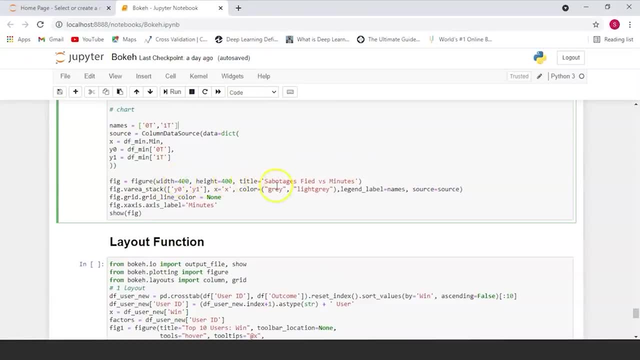 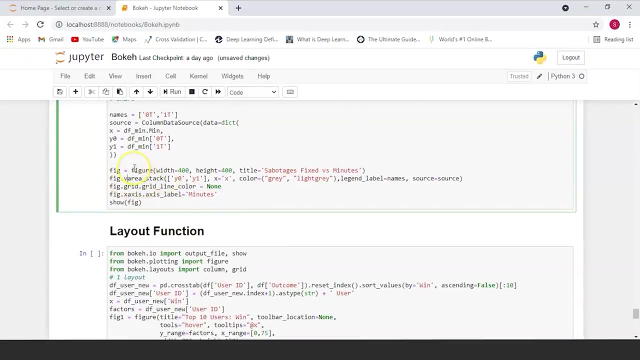 give our figure a width of 400, a height of 400 and the title of sabotages fixed versus the minutes at which they were fixed at. to plot a stacked area graph you're gonna be using var underscore stack function from the figure module you're gonna be passing in your y parameters. 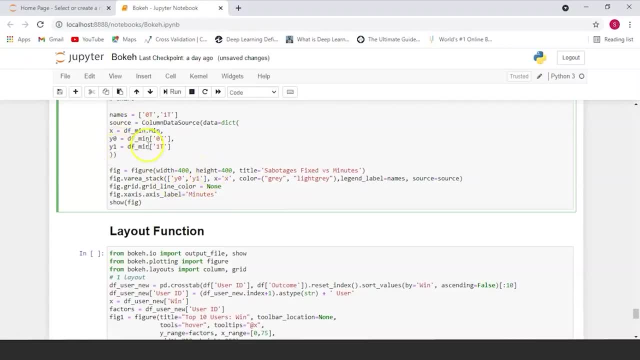 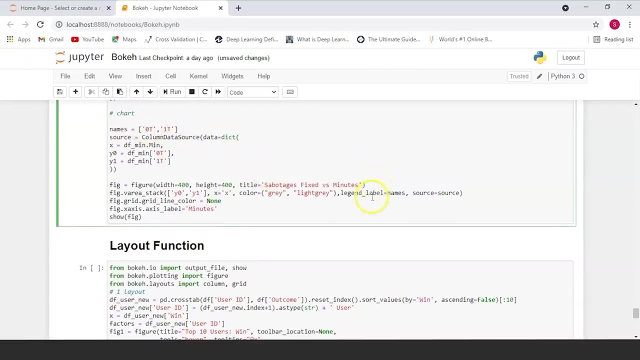 which is y0 and y1, because we have two different y parameters here and the x parameter, which is df minutes. the color that you're gonna be using is gray and light gray. the legend labels are the names that you've already put here, which is 0t and 1t. 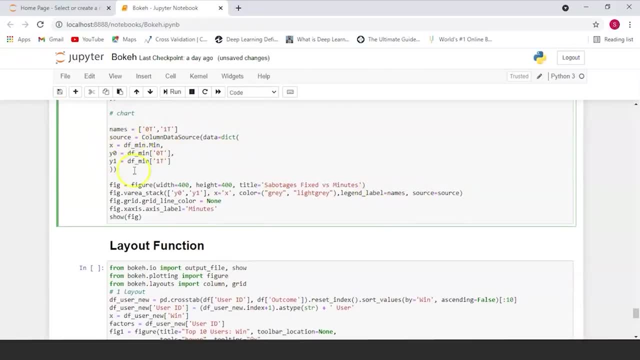 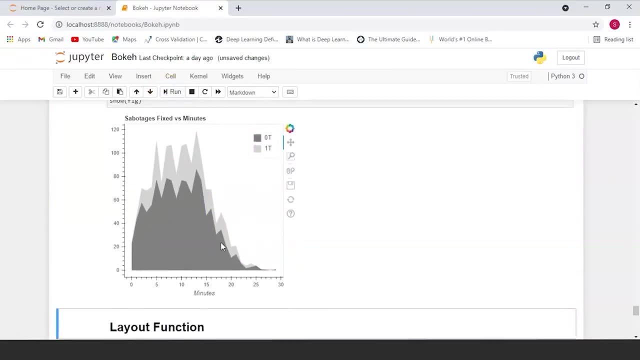 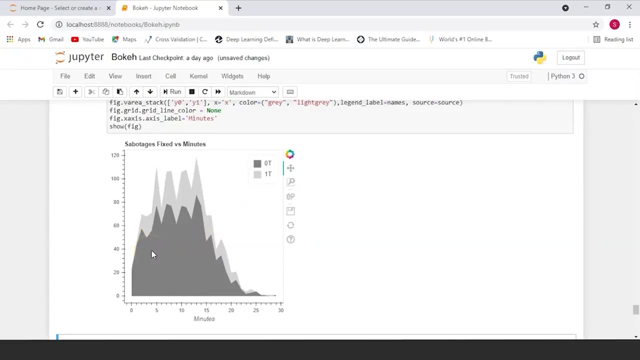 and the source of your data is going to be this column data source. now let's run this and see how our area chart looks. so this is our area chart. we've gotten two different sabotages here and two different times at which they occur, which is 0t and 1t. 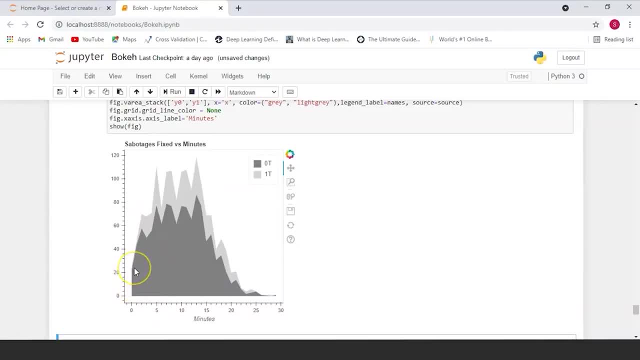 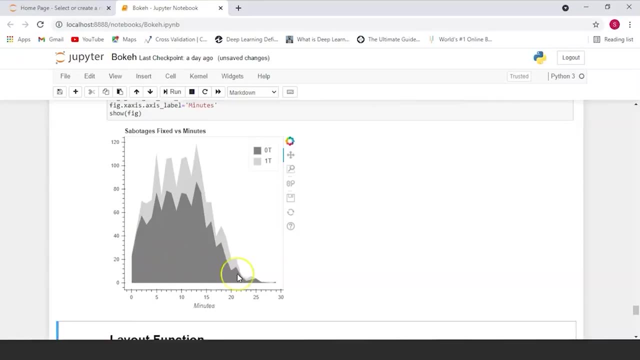 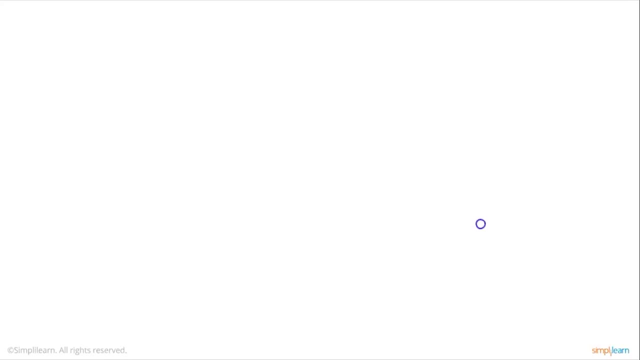 the minutes tells us how many sabotages were fixed at each time, basically how long it took to fix a sabotage and the minute during the game at which they occurred. now let's take a look at the layout function of our bokeh library. the layout function will let us 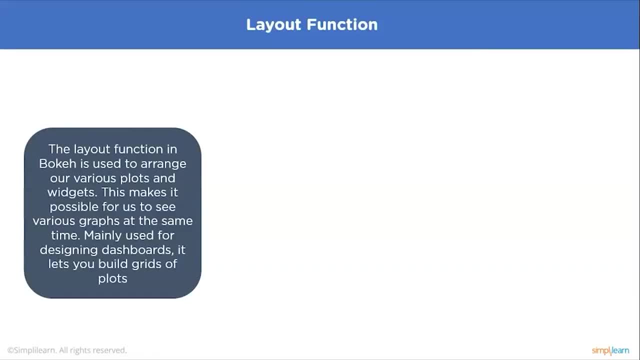 build a grid of plots and widgets. we can have as many rows and columns or grids of plots in one layout. using the layout function, we can see various graphs at the exact same time. mainly used for designing dashboards, it lets you build grids of plots. so this is basically. 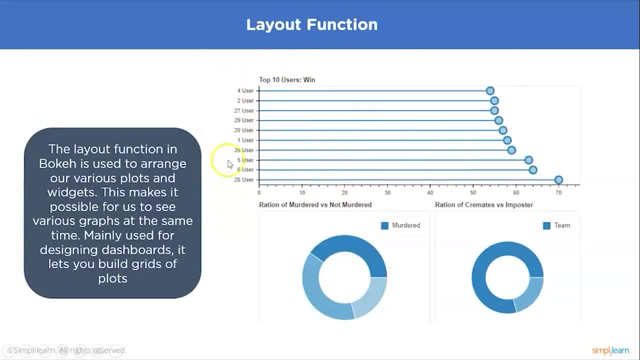 what your layout function will help you do. this is going to look very good in a website, because it's going to arrange our plots in a way that we can easily see all of them and understand all of them without any loss of data. this is also arranged very neatly, which is exactly. 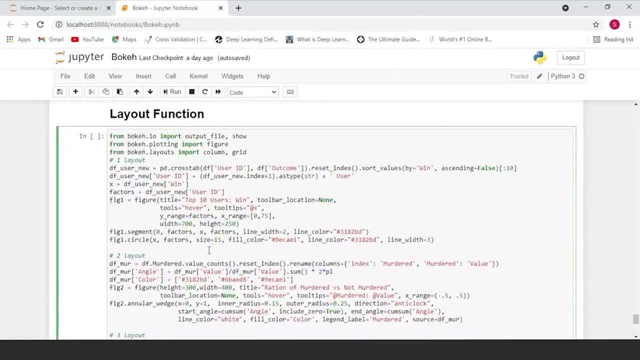 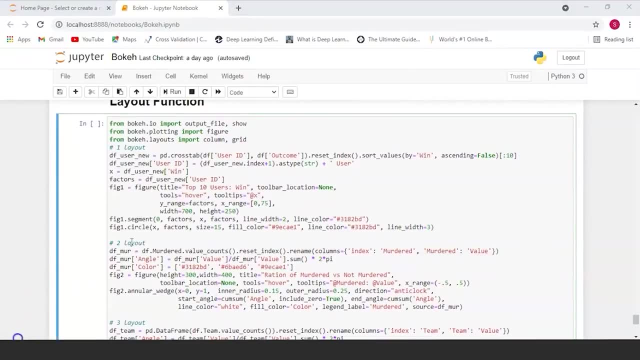 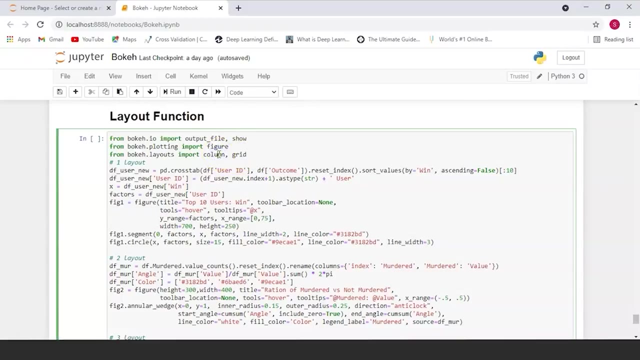 what the layout functions allow us to do. so now let's take a look at how the layout function can be implemented in python bokeh. now of the layout functions, there are many different layout options which are available. you have the column function, which allows you to display. 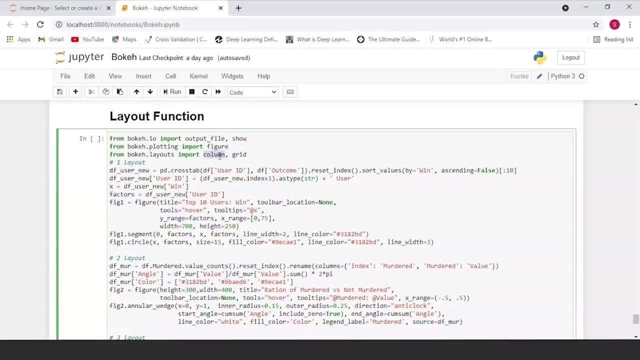 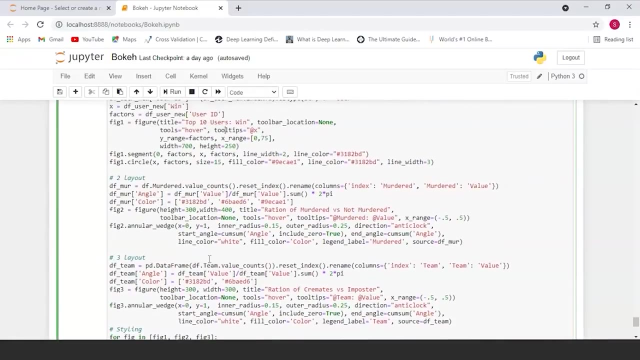 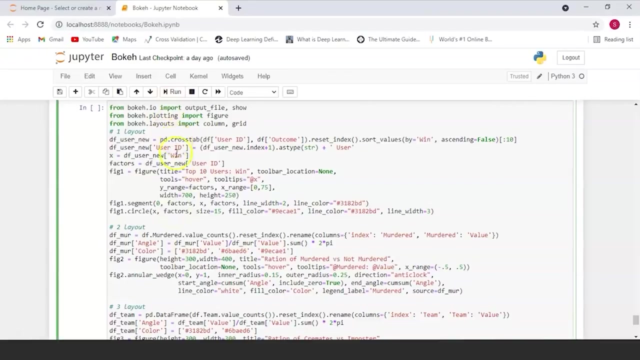 plots vertically and you have the grid function, which lets you display plots in the form of grids. now, for example, let's say that we want to make a dashboard layout in bokeh. we are going to be considering three different charts. the first one that we are going to be 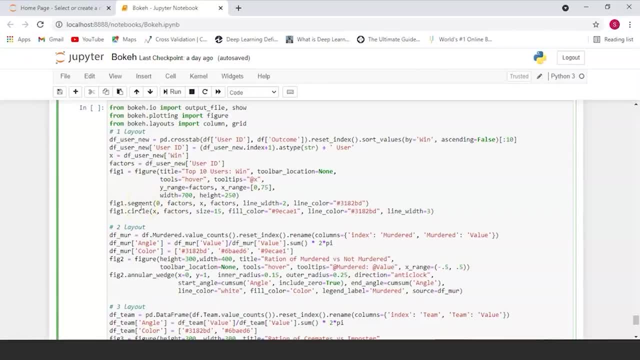 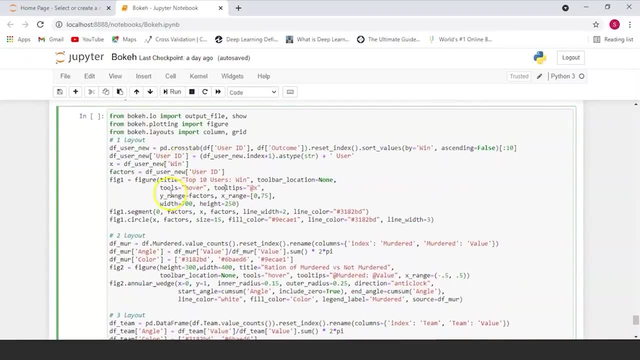 considering is a lollipop chart, which is done here. the next one that we are going to be considering are two pie charts, so this is how you plot a lollipop chart, and i will show you what exactly a lollipop chart is in just a minute. the first thing that you need: 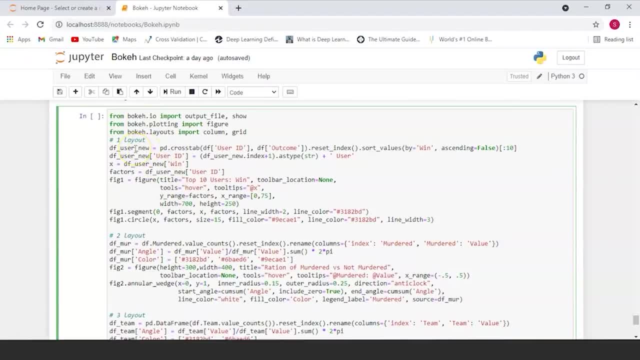 to know is that the first graph that we are going to be plotting is the graph is going to be a graph which has the user id versus the outcome of the games plotted on it. so what we are going to be doing here is that we are going to 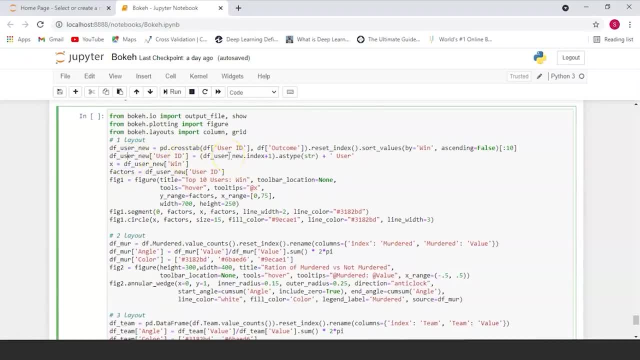 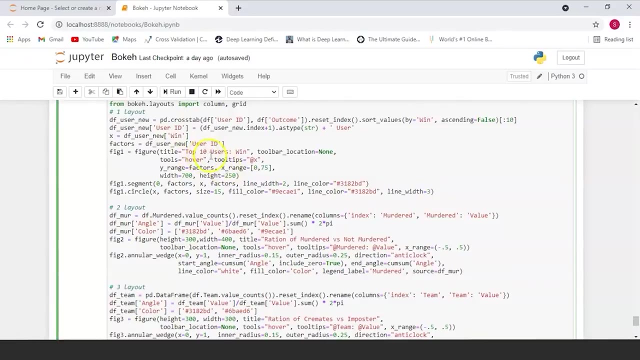 be creating a single data frame which has all of the user ids present in it, along with the user and the wins that the user has obtained. now, using this, we are going to be plotting it in the form of a plot in decreasing order, where we have the top 10 users who 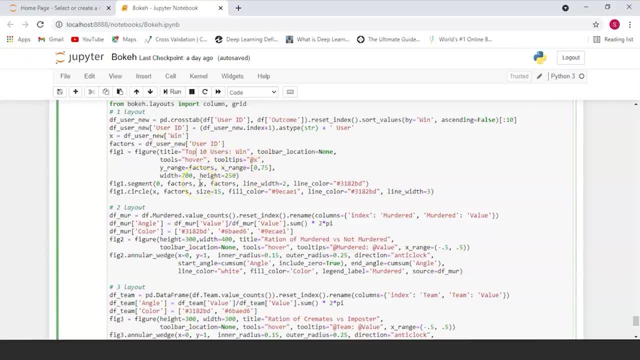 have won, which basically means that the users who have won the most number of games out of all the users in consideration. so figure one segment will basically help you plot a line which has a width of 2 and a circle will be at the circle, at the very top of this. 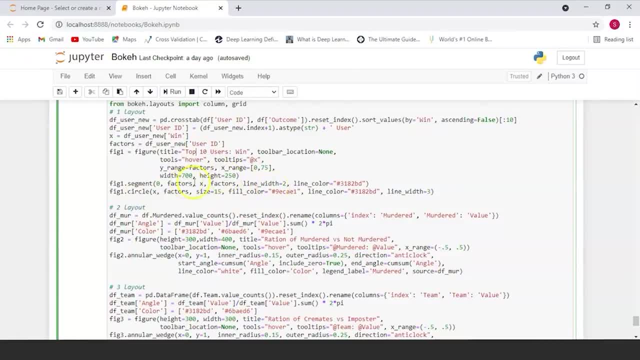 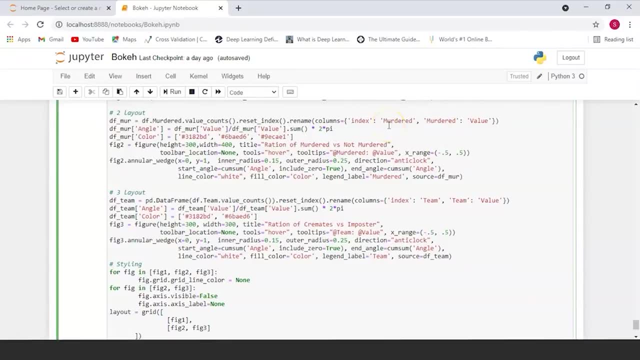 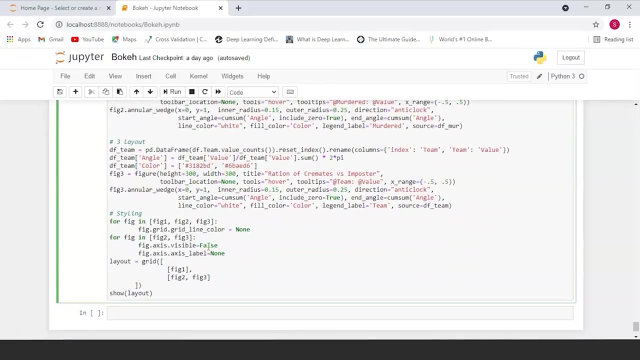 segment. so lollipop chart is going to be a horizontal line with a circle at the very top. so the next graph that we are going to be plotting is going to be a murdered and missing values pie chart, and the last thing that we are going to be plotting is: 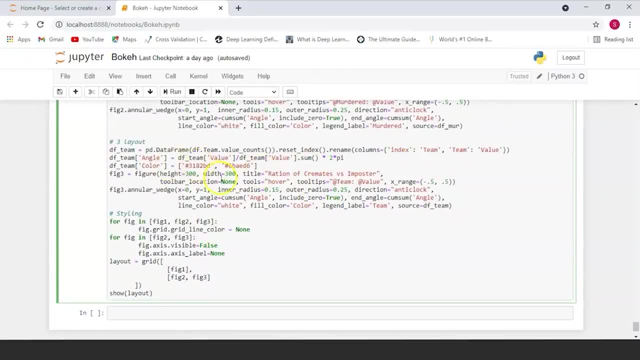 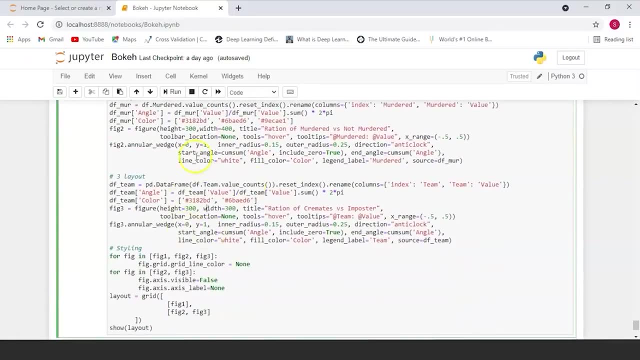 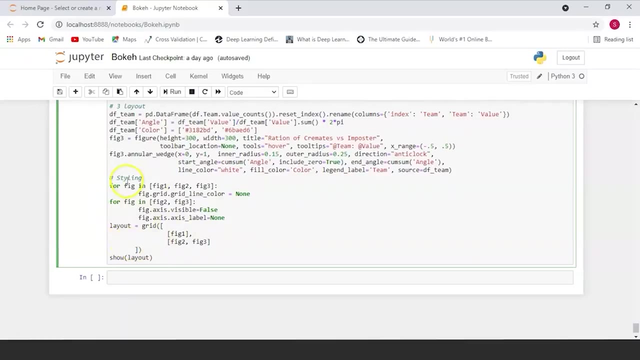 a donut chart of the teams and the values within them. so these are the three different graphs that we are going to be plotting, and these are just us creating the graphs and plotting them. the main logic is over here. the main logic is that you want to set. 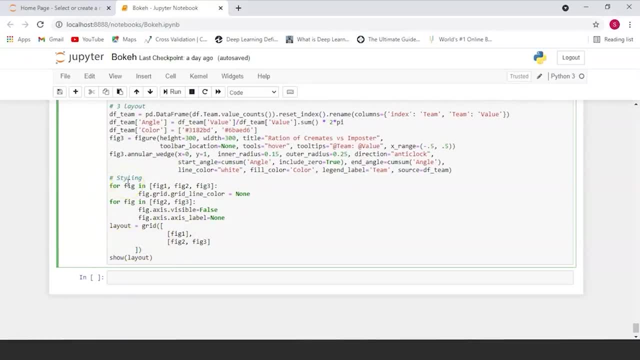 a layout in bokeh as to how you want to see the charts. so the layout that we are going to be looking at is that we are going to be having a lollipop chart at the very top and two smaller pie charts at the bottom right. so 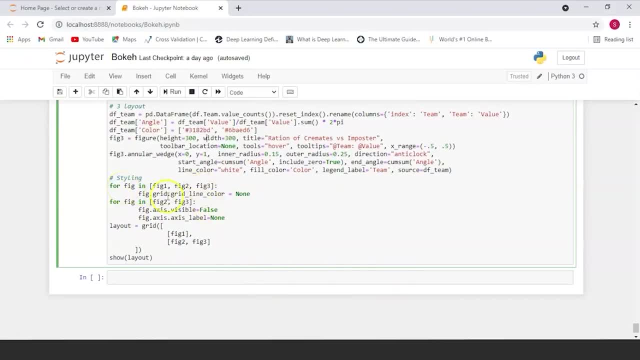 we have three figures here, and the first thing that we are going to be doing is that we are going to be giving these figures a line color of none. the axis is not going to be visible and the axis labels are not present for these figures. this is. 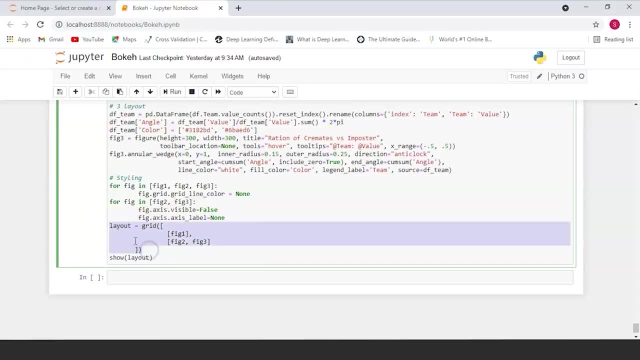 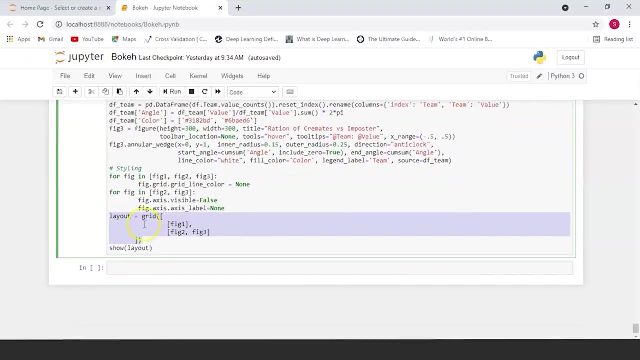 the main function that you are going to be looking at. this is your layout, using the grid layout function that you have imported here from bokehlayouts. you are going to be creating a grid, and how does the grid know where the figures are? so you have divided the grid into two. 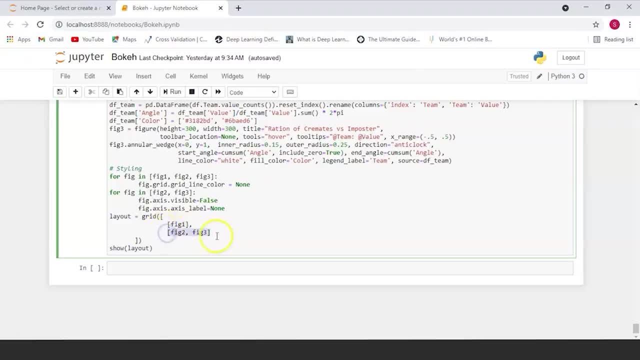 this is evident because you have two figures, two main figures here, which are separated by a comma. so this tells the grid that the page is going to be divided into two. the first figure, which is on top, is going to be figure one, and the figure at the bottom are 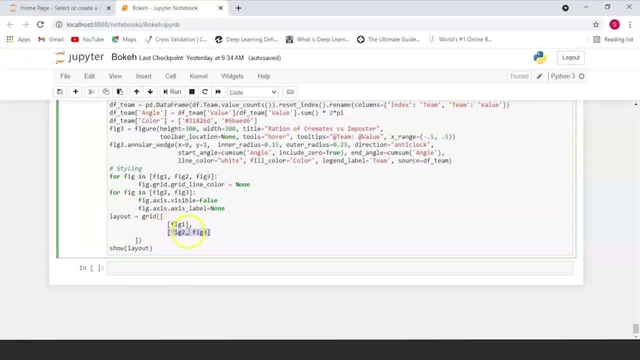 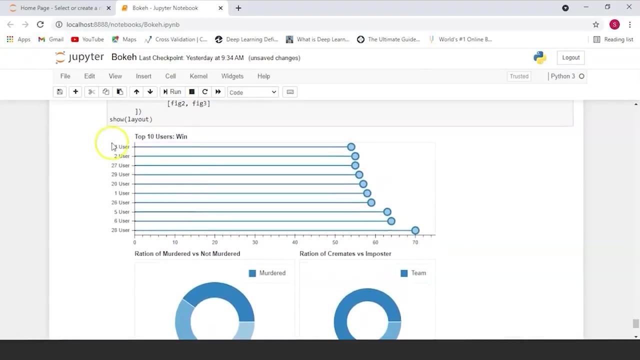 figure two and three. this means that the bottom half is going to be further split into vertically. lets run this and see what our layout looks like. so here you have it. your entire page is divided into two. the first one has one, the figure one, which is the. 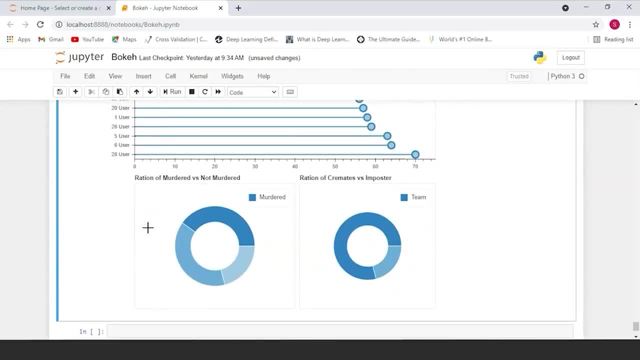 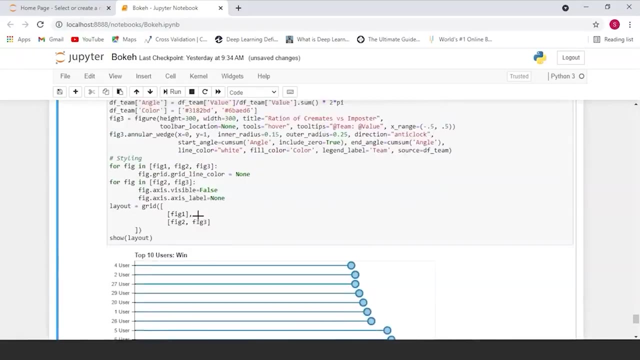 lollipop chart, and the bottom half of our page has two figures, which are the two donut charts. the bottom half is divided exactly into two, as you can see here. this is because that is the grid layout that we wanted, so this is how you can use the layout. 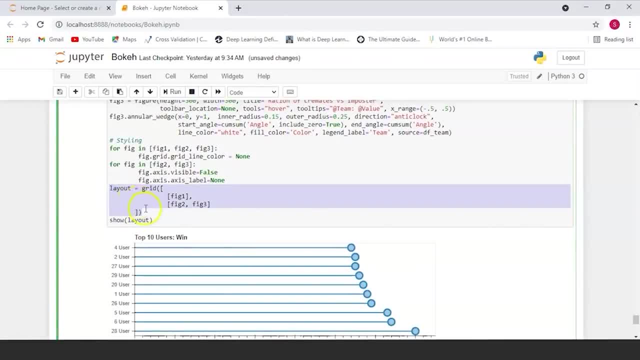 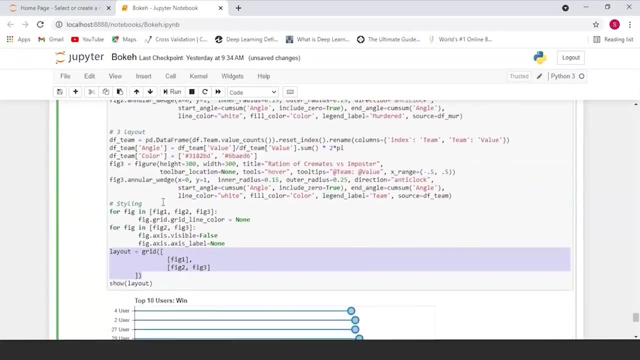 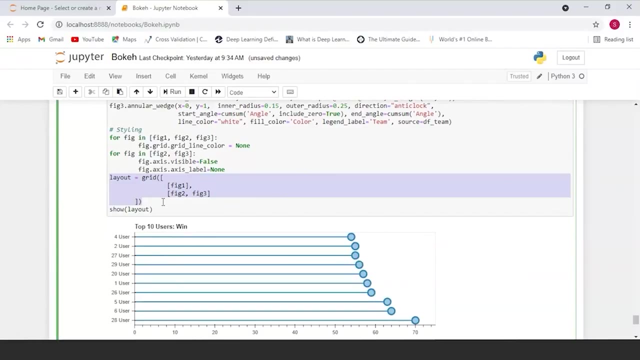 function in python bokeh. it is extremely easy. all you have to do is create a layout by using the grid function, or you can also use the column function. the column function will plot it in the form of a single column vertically. using the grid function, you can plot figures vertically. 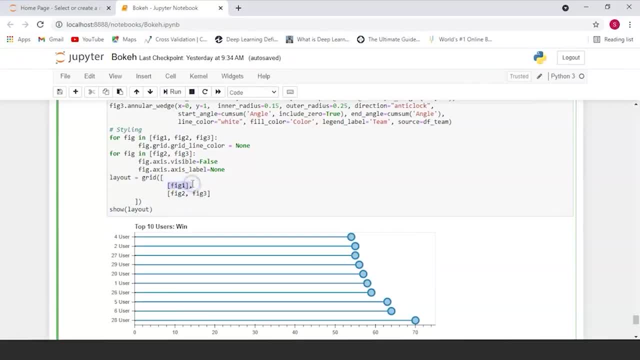 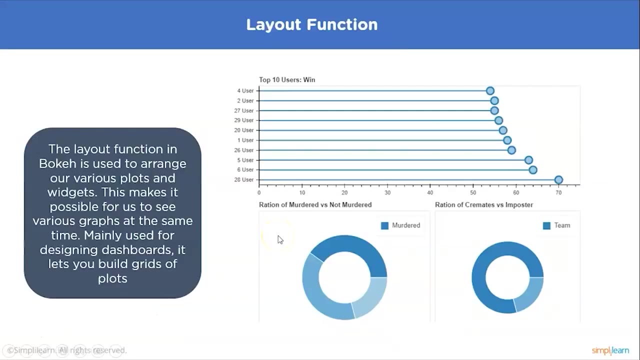 as shown here. so when you separate them by commas with respect to each other, they will be plotted vertically, and when you group them together and separate them with commas internally, they will be plotted horizontally. so now we have taken a look at how we can use the layout function. 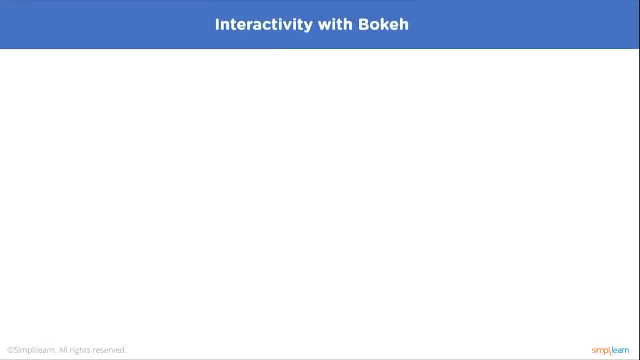 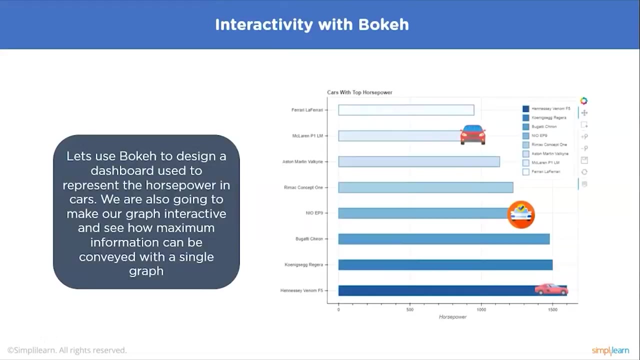 now lets see how we can make interactive graphs with the help of bokeh. over here we are going to be using bokeh to design a dashboard which is used to represent the horsepower in cars. we are also going to make our graphs interactive and see how maximum 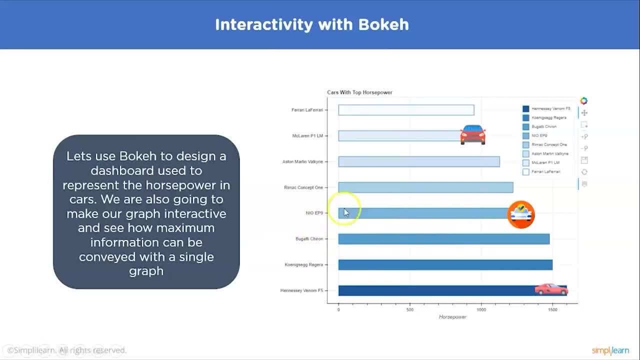 information can be conveyed with the help of a single graph. so here we have multiple different cars, and along with the cars, we are also going to be given their horsepower, a little bit of other information about them and their images, and over here, as you can see, we have a very simple 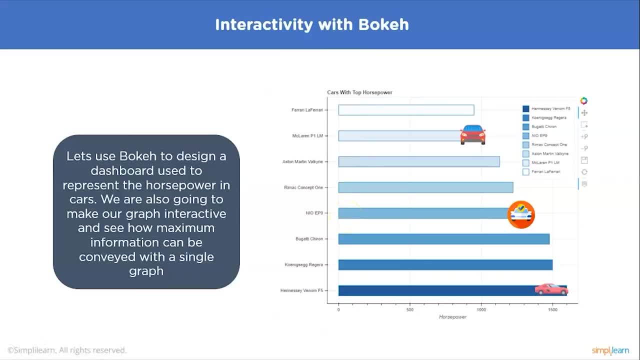 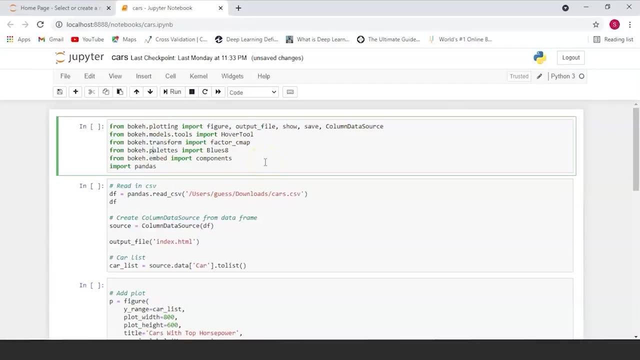 vertical bar chart, but lets see how we can make it interactive and convey all the information that we have in our single data set on this one bar graph. so the first thing that we are going to be doing is importing all of our important, necessary modules. we are obviously going to have the pandas. 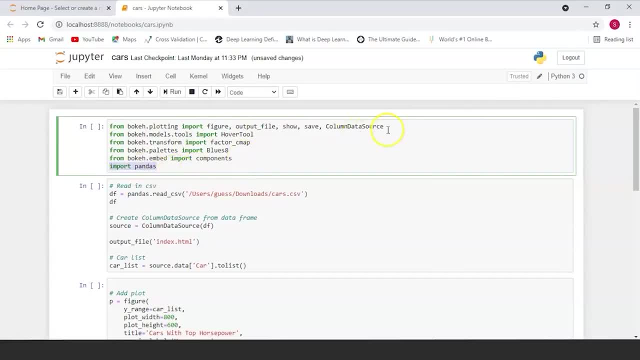 modules, which is going to be imported to work with the data frame that we have given. apart from this, we are also going to be importing figures output files: show, save and column data. source from bokehplotting. we already know that the figure function is used to. 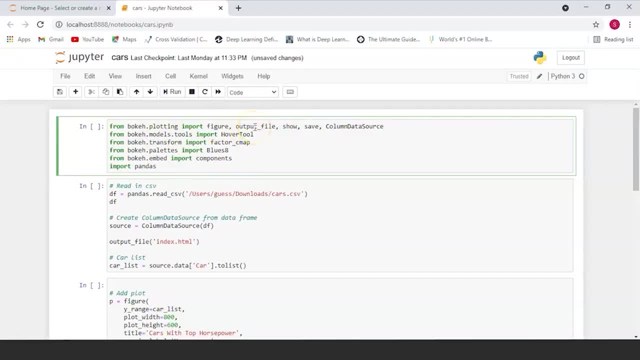 plot different types of graphs which are given output. file is just used to see our file. the show is used to display our graphs and save will help you save your graph now. the column data source is the core of most bokeh plots. it provides the data to the glyph of 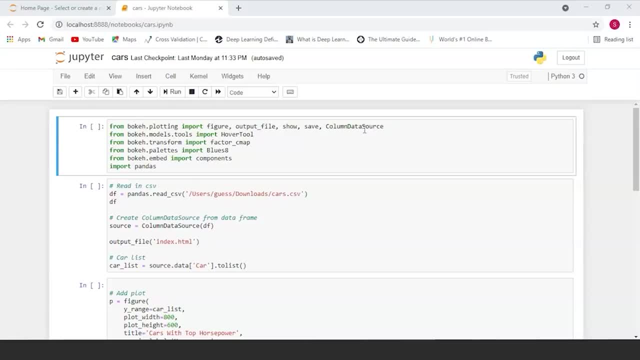 your plot. when you pass sequence like python lists or numpy arrays to a bokeh render, bokeh automatically creates a column data source with this data for you. so this is basically what you are going to be using to pass data onto your bokeh glyphs. apart from this, 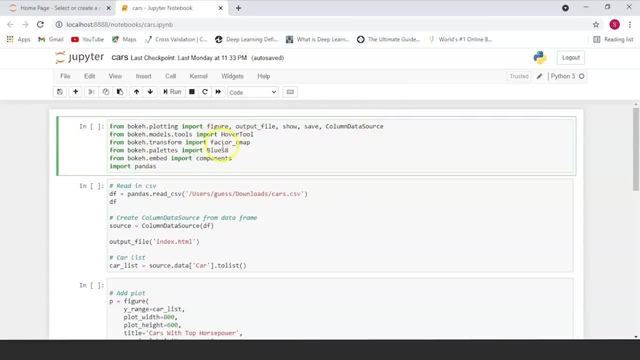 we are also going to be using a hover tool function and, from the transform function, we are going to be importing factorCMap. we are going to be importing a palette color, which is going to be various shades of blue, and we are going to be importing components from the embedded 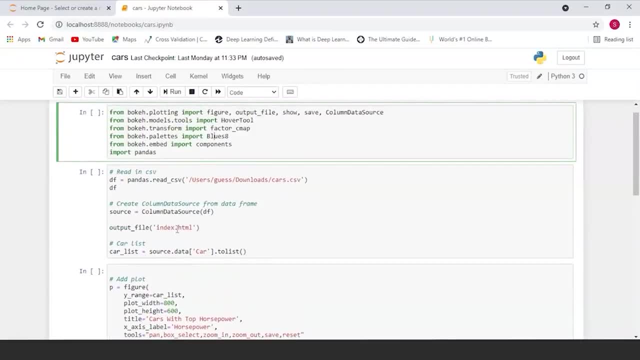 function of bokeh. lets just see how we can use all of these and the different things that they do. the first thing that you are going to be doing is reading in your cars data frame and creating a column data source so that you can easily pass this data onto your 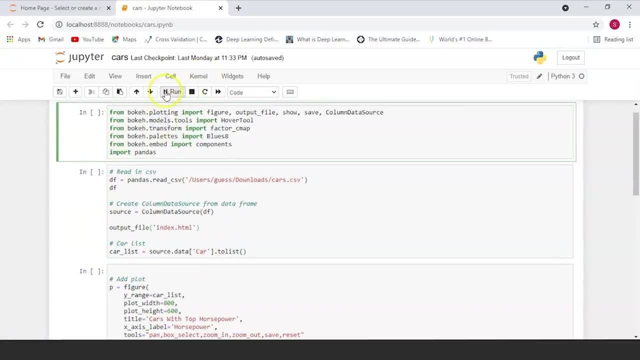 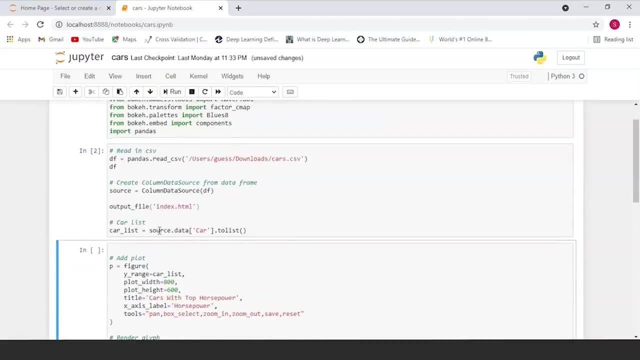 bokeh glyphs. so lets run and import all of our various required functionalities and import the data as well. so this is what your data set looks like. we have 8 different values in our data set, which are the names of different cars, their horse power, their price. 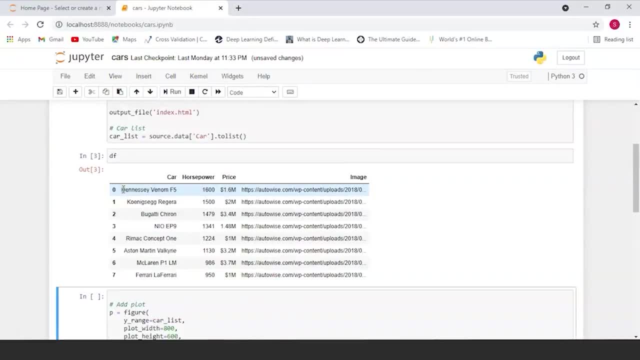 and a hyperlink of an item. so this is what your data set looks like. we have 8 different values in our data set, which are the names of different cars and image. this is what our data set looks like. we have only 8 columns. so, using this data set, we are going to be. 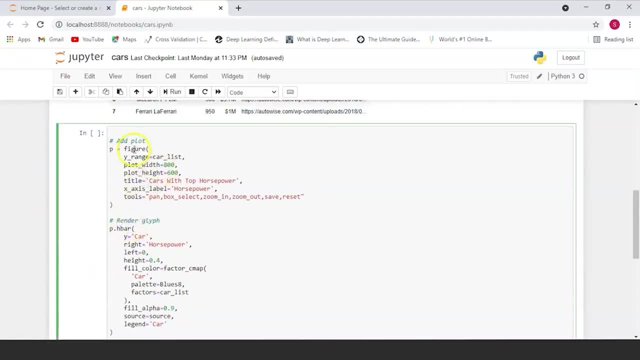 plotting a horizontal bar graph. again, we are going to be calling our figure function and we are going to be giving y range to our car list. the y range is basically just going to have the different values which are going to be present on the y axis. we have given the plot a width of 800. 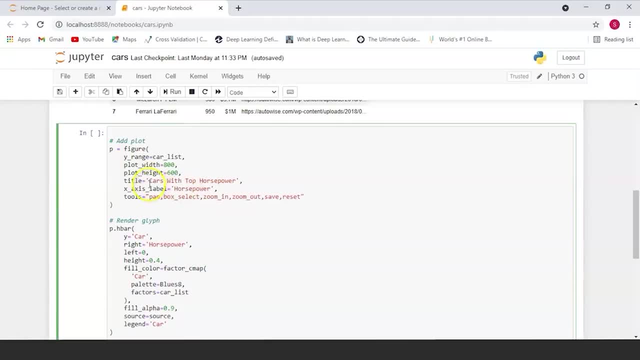 and a height of 600. the title of the plot is cars with top horse power and the x axis label is horse power. the tools that we are using here is pan box, select, zoom in, zoom out, save and reset. so these are tools that you are going to be getting. 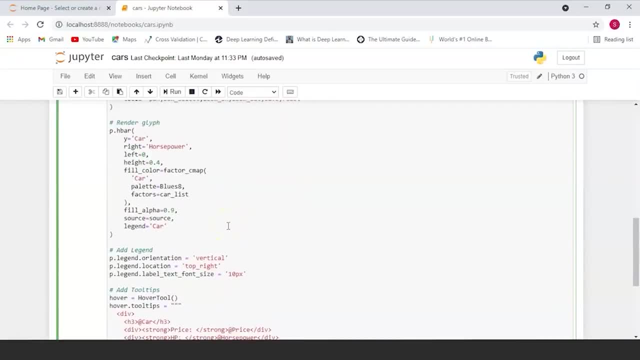 on the right side of your plot. now let's render our glyph, or render our graph. the graph that we are going to be using here is the horizontal bar graph, so the y axis is going to have cars and the right or basically the height of the entire bar. 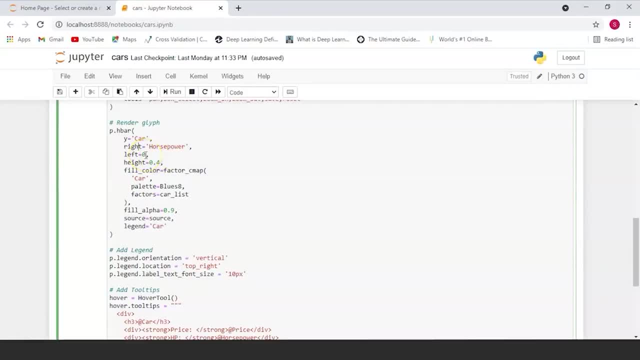 is going to depend on the horse power. the left is going to start from 0 and the height of each bar is going to be 0.4. the color that we are going to be giving is going to be a pallet of blue, so each different. 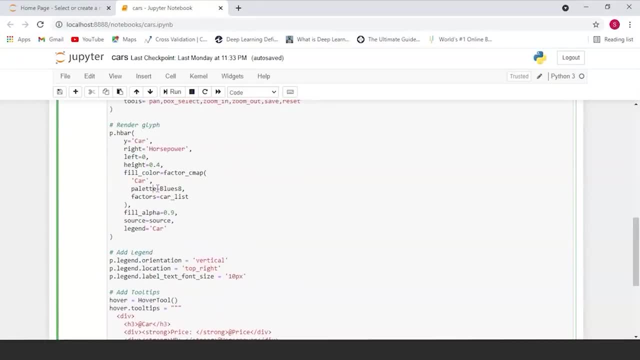 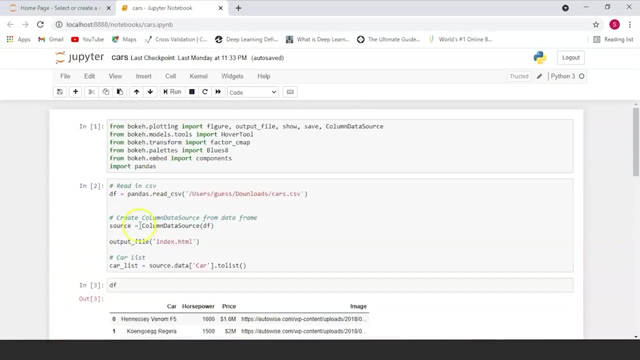 car will have a different color of blue associated with it, and the color of blue which is associated with it will depend on the car list. now fill alpha 0.4, 0.9. the source is your source data that you have over here, which is the column data. source of our data. 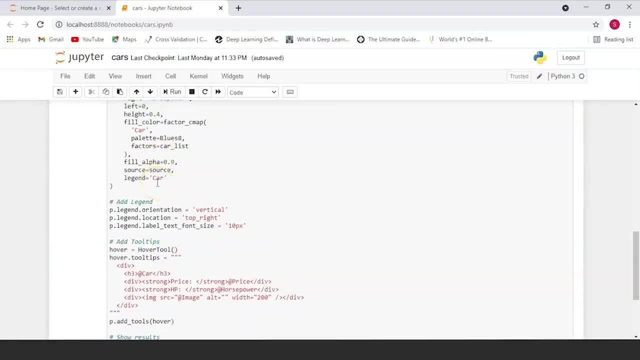 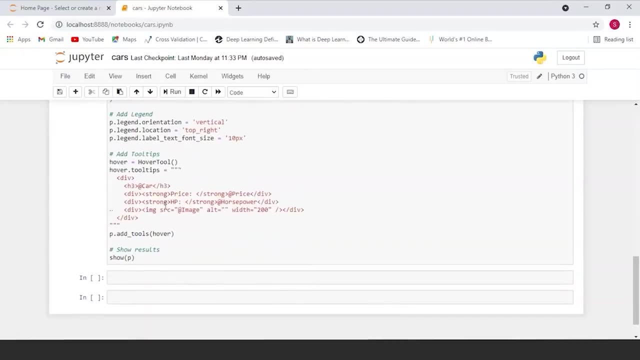 frame and the legend is going to be car, which basically means that your entire plot is going to have the legend of car. now we are going to be adding the legend. this is us giving the legend its orientation. so the legend is going to be vertically oriented. the location is going to be on the 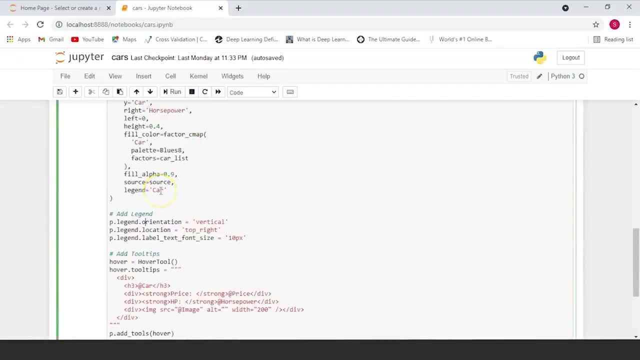 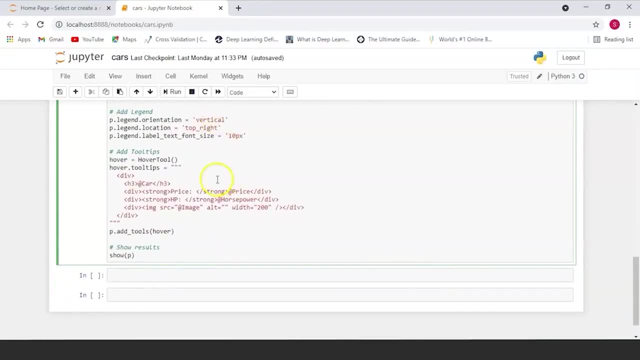 top right and the font size of the text car of our legend is going to be 10 px or 10 pixels. we are also going to be adding a hover tool inside this hover tool, this hover tool tips will basically tell you what you are going to be seeing. 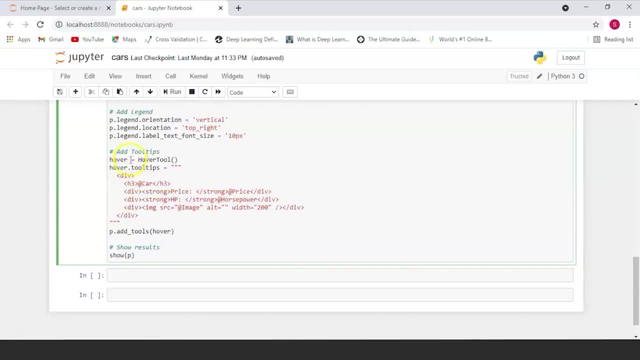 in the hover tool box, so we are going to be creating this with the help of an html format. the first thing that you are going to be seeing is the name of the car. the next column will have the price of the car, the horsepower of the car. 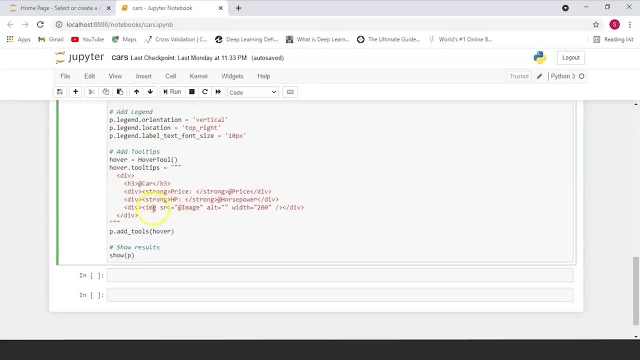 and the image. now, the image is in the form of a hyperlink and this is going to be auto populated in your hover tool. the width of the image is going to be 800, so we are going to add all of these hover tools to our p image and we are finally going to 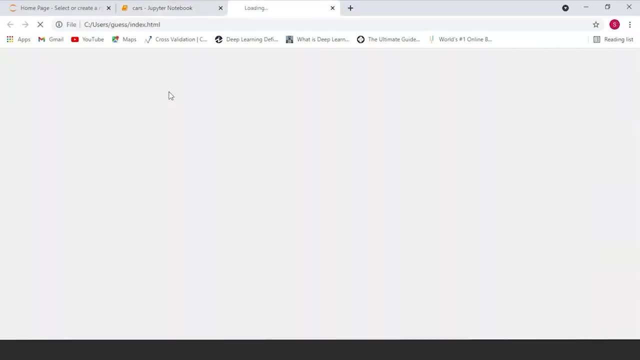 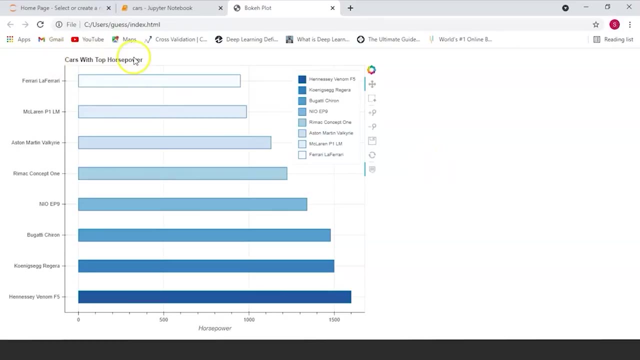 be showing you the graph and what it looks like. so this is your bouquet plot. here, the name, the title of the plot is cars with top horsepower. this is your legend, which is cars. the name of each car is given here, along with the color which is associated with it. 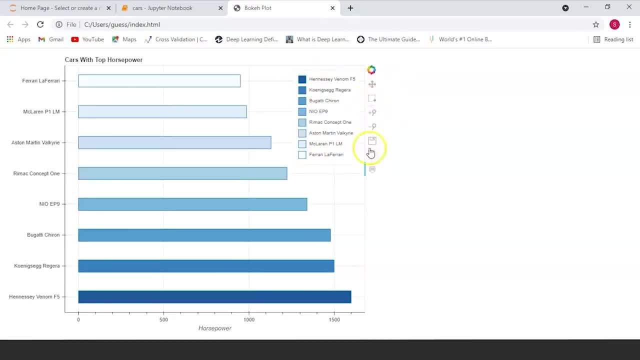 here are the different tools that we have. you can save this, you can reset it, you can zoom out, you can zoom in, you can select the boxes and you can pan your image. so here we are zooming in, here we are zooming out. if we save this, 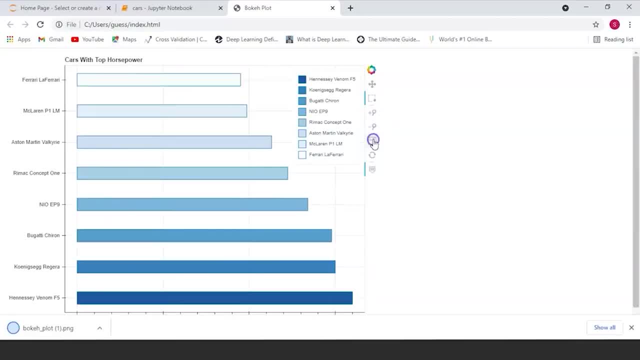 the plot automatically gets downloaded in your system and if you reset it, the image goes back to exactly what it looked like when it was first opened. now, here you have the names of the different cars on the y axis and you have the various horsepower on the x axis. let's take a look at.